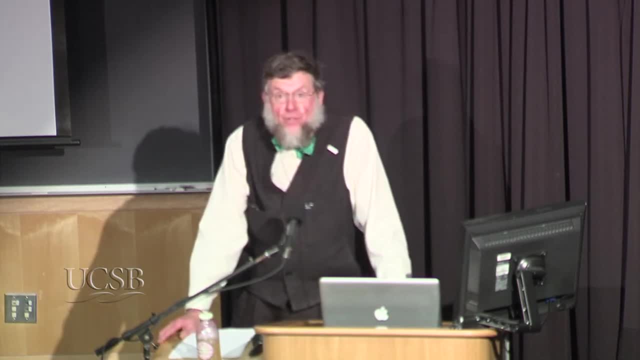 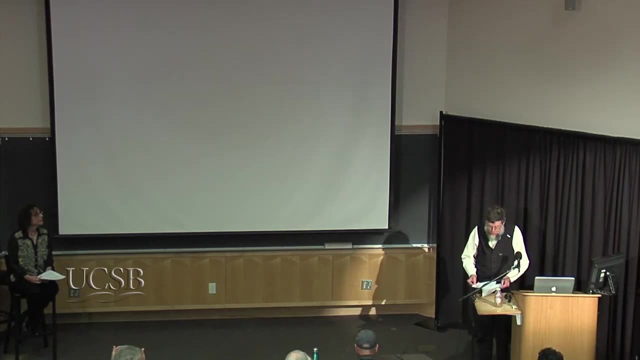 illustrate the reality of current sea level rise that help us envision its future in a presentation entitled Figuring Sea Level Rise: Interactive Visioning. Now, those who are in the room today are largely here because we see environmental change as a critical issue. This choir does not. 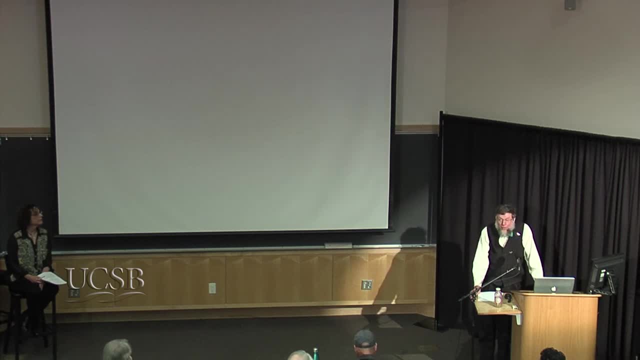 need the sermon of the problem. It does, however, I think, need one of effective outreach. It is clear that a tremendous amount of work is being done to improve the environment, but it is also clear that the greatest number of our fellow citizens are either unconcerned or misinformed about. 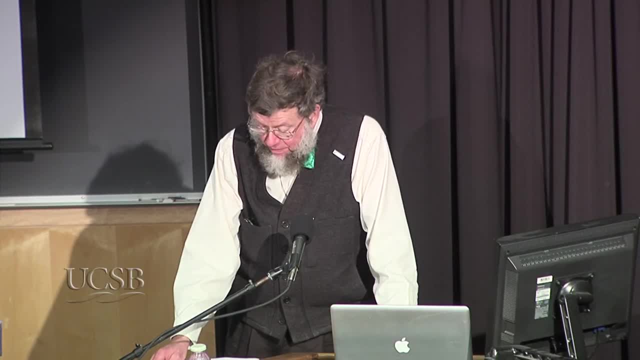 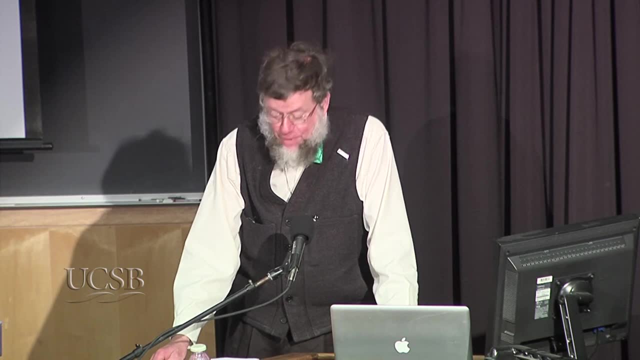 the threat of environmental and social destabilization that is posed by climate change and the resulting sea level rise. If you wonder where the misinformation rises, one has to look very much further than Oreskes and Conway's recent book Merchants of Doubt. Some misinformation is not an accident. 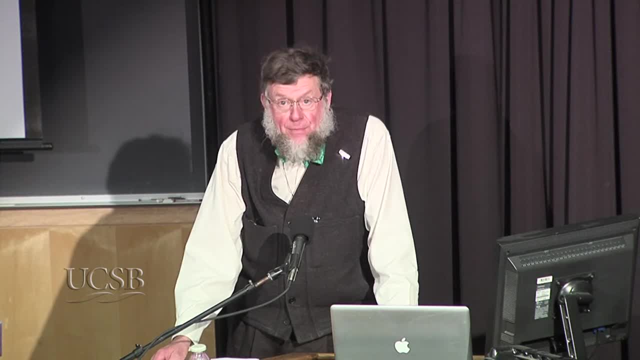 It is organized and it is financed. This needs to be addressed and countered. But beyond that, there's also a population of individuals who has an awareness but turns aside because they've already given up. It's too frightening, It's too challenging, It's too depressing, And indeed, some of what is now in motion in terms of planetary 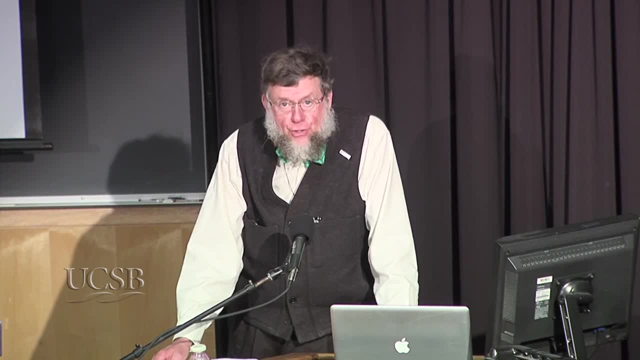 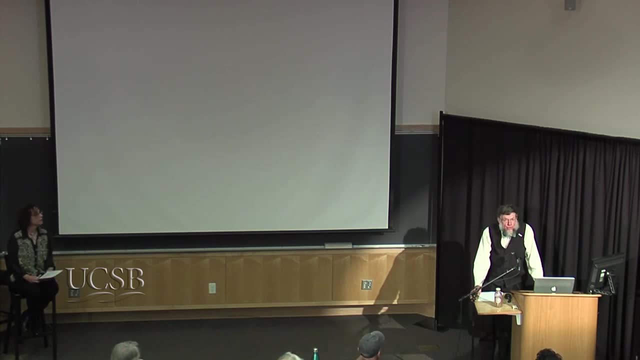 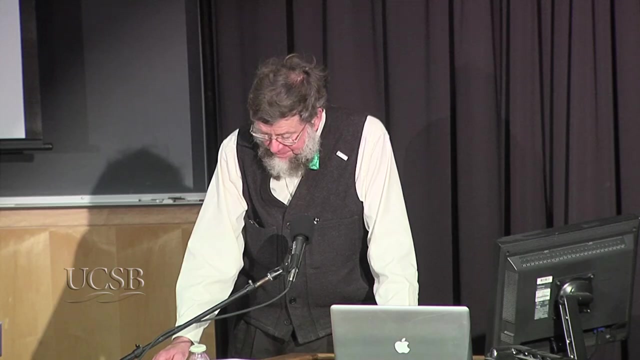 change is not going to be derailed But, given the inertia of human affairs, we need to get on this as soon as possible. We must quickly inspire new thinking and real world solutions to a planet that is in the process of transformation. How do we command that attention and correct misinformation? We all need to. 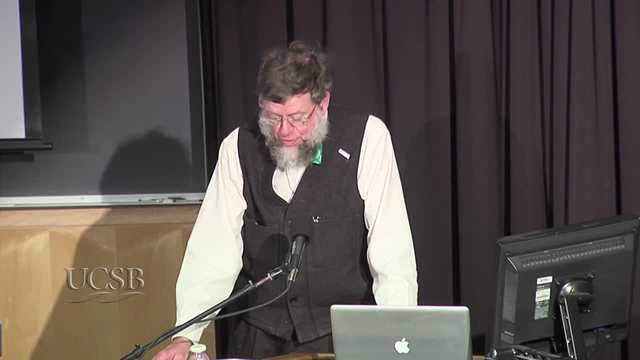 have value in this fight, and it is a fight- And none of us, willing or concerned, or unwilling and in denial- really has a choice. The planet is finite. We're all on the train to gather and it's underway. We need to make sea level rise a. 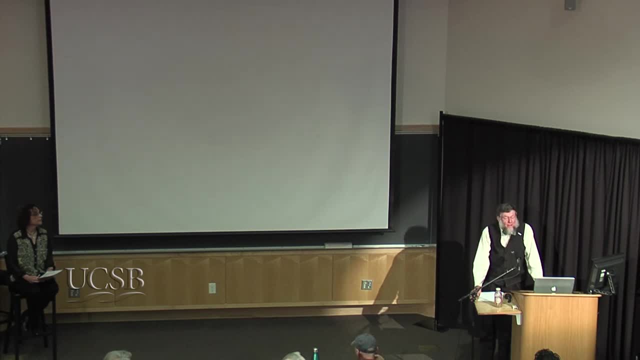 critical issue in America, not just in this room. There's much we can do, but we need to begin And we think that with today's discussions we can talk about using some tools to address this. In today's presentation, we'll explore through: 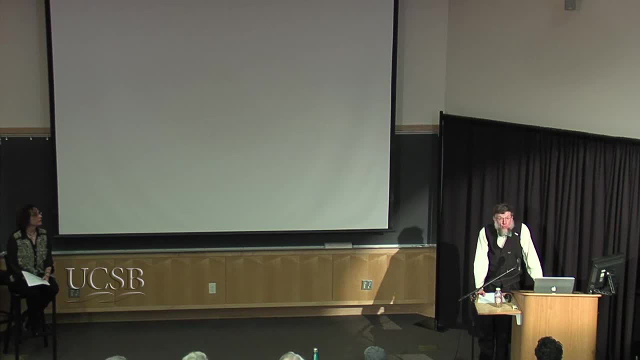 interactions and expertise. We're going to talk about climate change. We're going to talk about climate change. We're going to talk about the opportunities of our speakers and our audience. This is a two-way process. It is not coming from here and going. 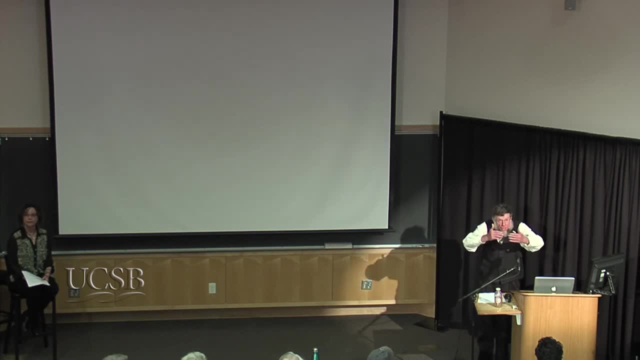 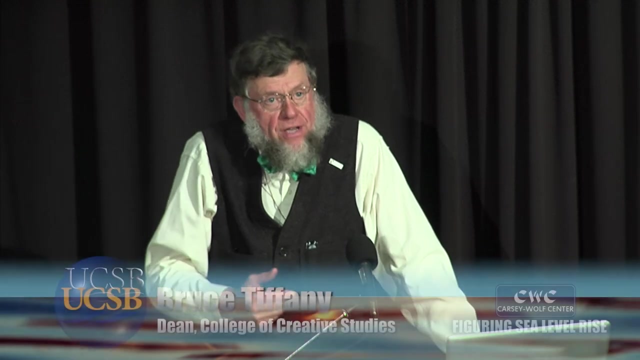 there, The room is full of experts, various aspects, and we want to have that interflow of ideas How we can effectively integrate some of the really sophisticated and visually challenging, visually loaded with impact imagery that scientists have generated in the process of understanding sea level rise and global change. We want to take those tremendously. 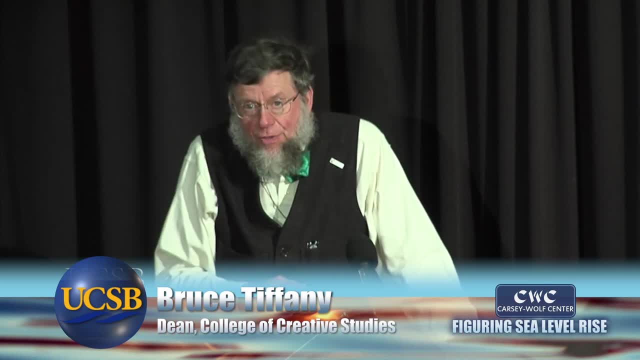 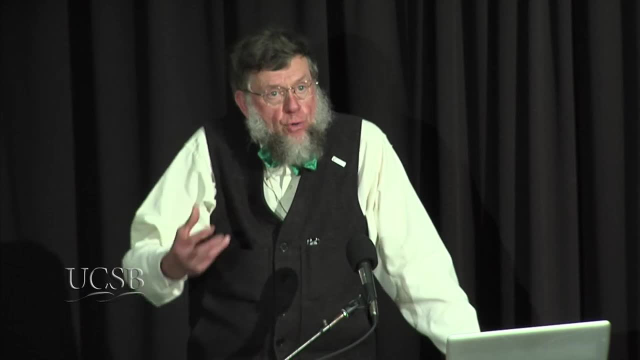 powerful visual units And integrate them. we hope, with the abilities of those who are experts in film, who are experts in writing, who are experts in public communication, How can we work together to achieve, to bring this message to the public at large? So our focus today is not on the science, It is on 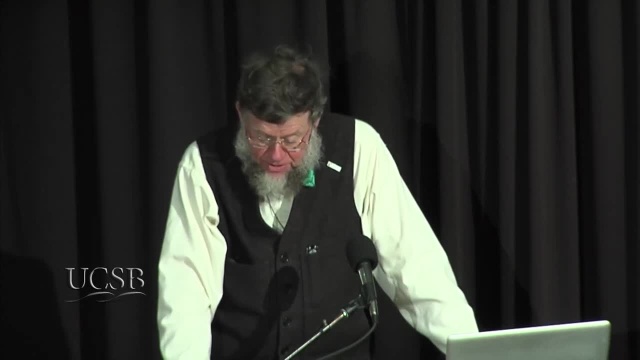 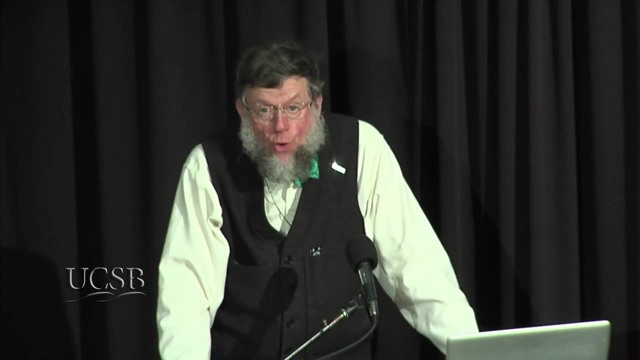 communication, How to bring our collective abilities as specialists and citizens to alert and involve the public at large. All communication is story, So the bottom line is: this is a crucial story of our times. How do we tell it effectively? I here want to recognize the 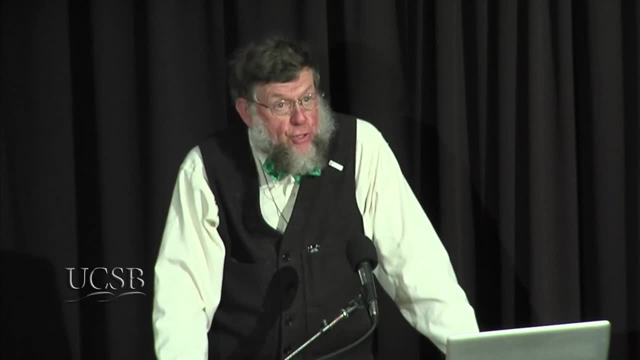 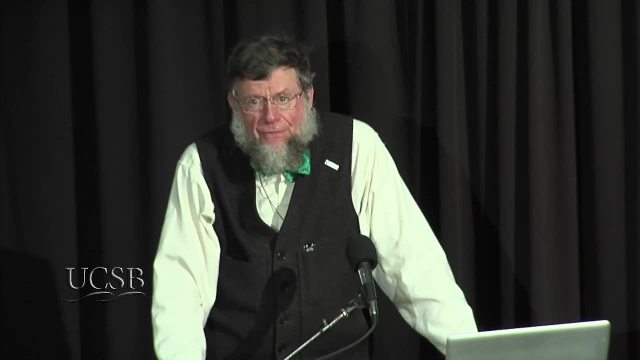 vision of the College of Letters and Science in establishing this critical issues in America sequence And the support that it has offered to this undertaking, which has been phenomenally exciting, I think, to those of us who are participating in it across disciplines, And I particularly want to. 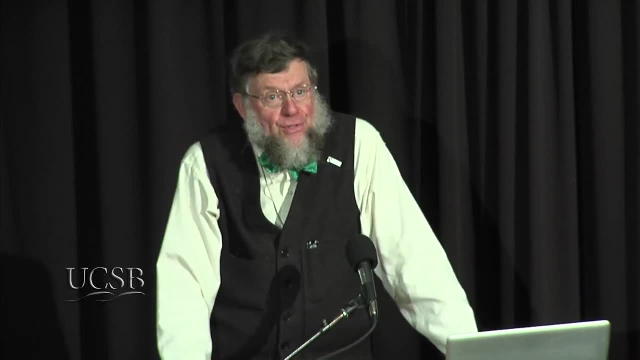 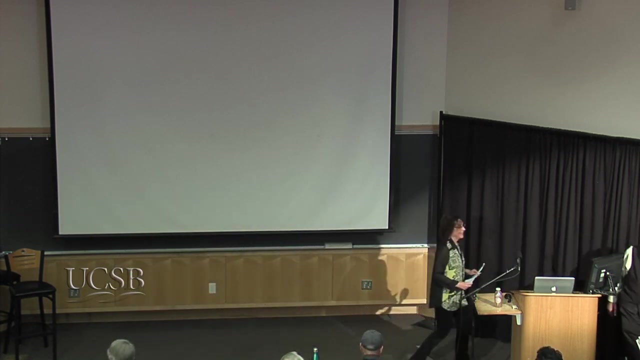 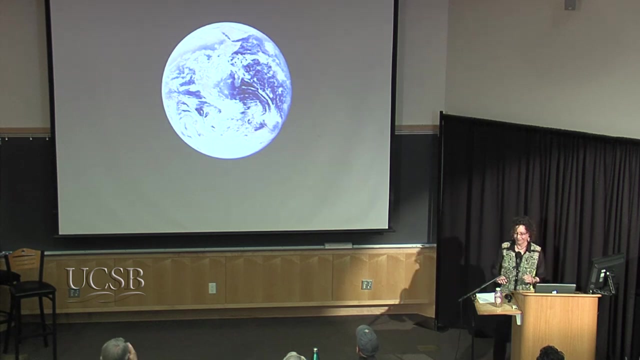 thank Janet for being our leader, our fearless leader, our chief among equals, who has been the inspirational leader and has held us online and made this really happen. So, Janet, thank you And thank you all for being here. Thank you, Thank you so much. Let me bring up my PowerPoint somehow. 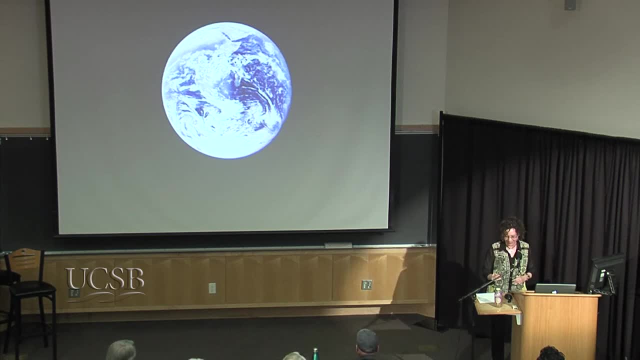 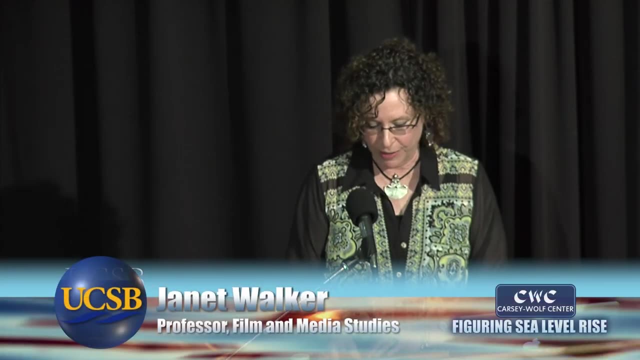 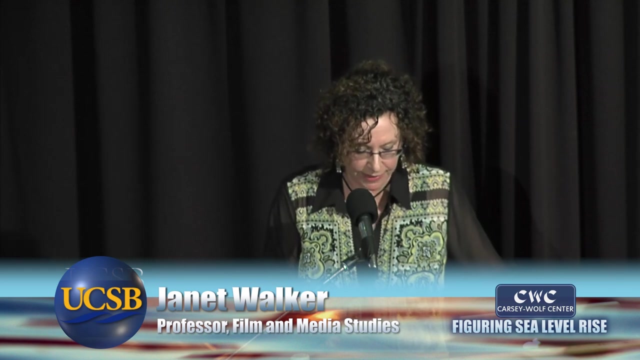 There's never a way to have no light on the screen, yet light to communicate with each other. So anyway, thank you very much, Dean Tiffany. Indeed, I'm the one who's been inspired to be working alongside my colleagues on the core team, Professors Josh Schimmel, Mary Hancock, Annalise Llewellyn. 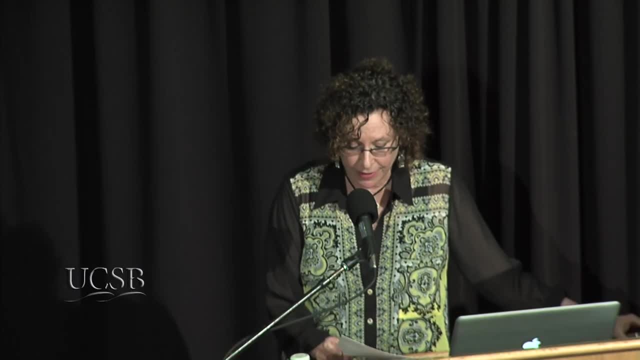 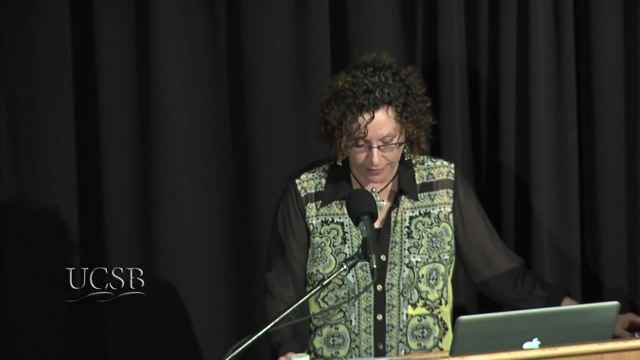 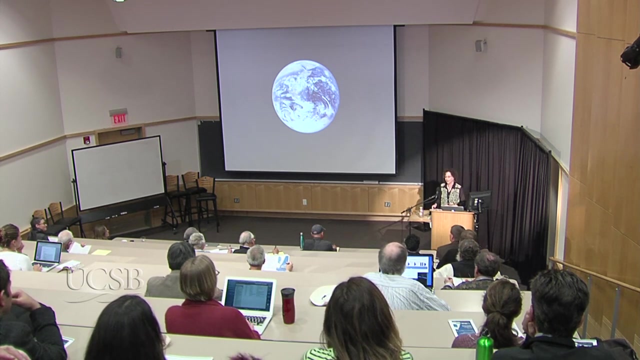 John Forn, Stephanie Lemonajar. Together, we come from all three divisions of the College of Letters and Science, And we are joined by additional colleagues, including from engineering and the Bren School of Environmental Science and Management, whose names and areas of research you can read in the 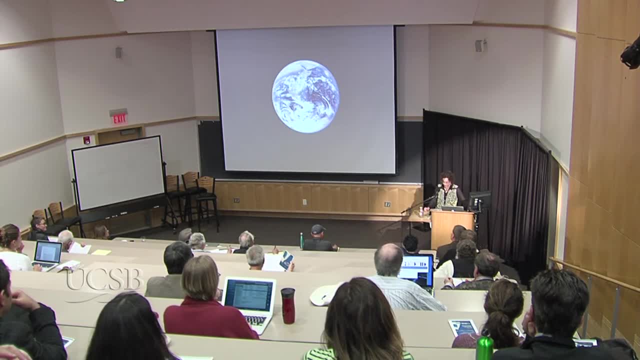 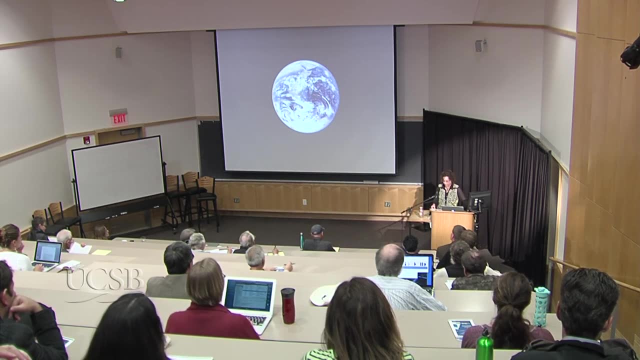 program and on our website. All hands on deck will be required if we are to comprehend what's going on and, importantly, if we are to respond to what's going on. As our fall quarter speaker, Earth and Planetary Scientist Gary Griggs, put it, and he was linking our California coast to regions around the world- 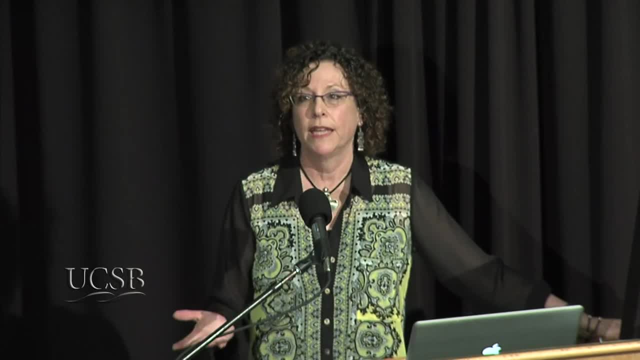 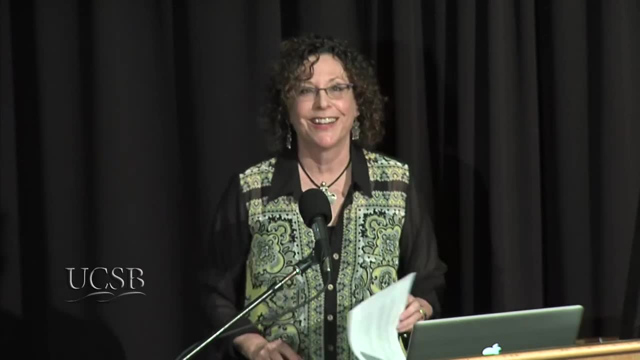 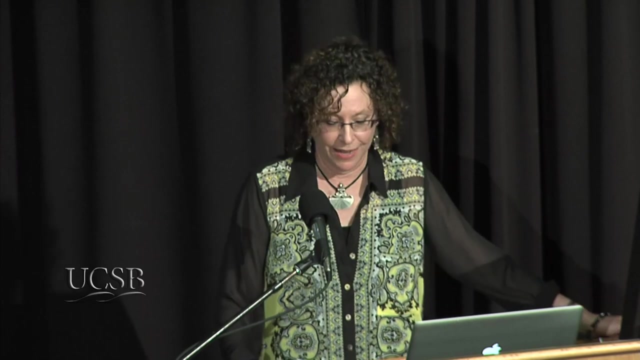 we have three choices and they overlap: Mitigation, adaptation, suffering. Now I'm guessing just about everybody here has a choice. Everybody here has seen Davis Guggenheim's and Al Gore's Oscar-winning documentary film An Inconvenient Truth. 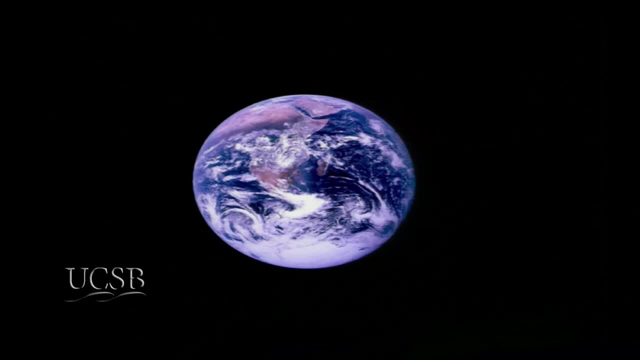 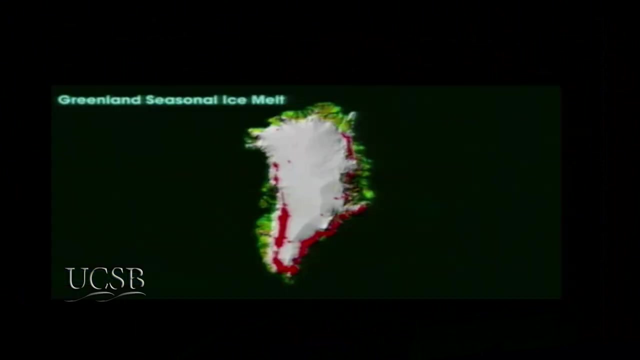 So, even though we're wildly interdisciplinary, we may well have this film in common, As you will likely remember, the sea level rise sequence. this is what would happen- and the famous hockey stick, of course- If the land-based ice on Greenland were to break up. 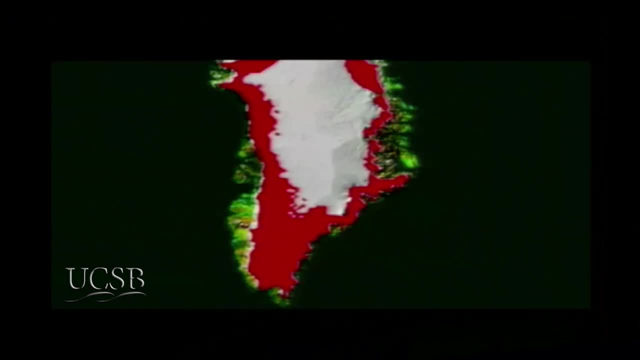 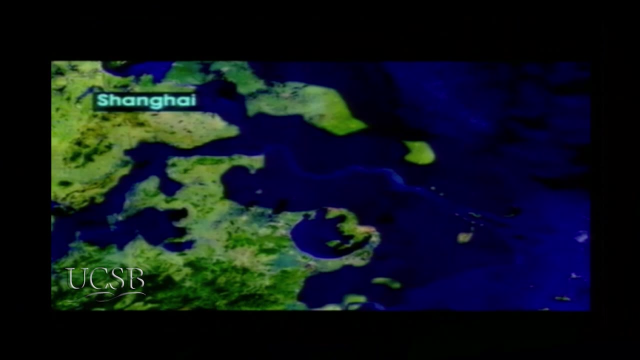 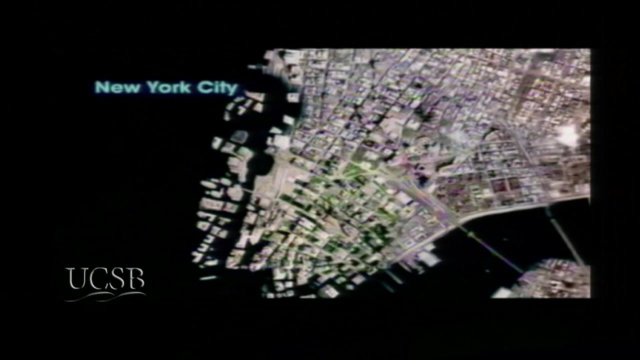 Or if half of Greenland's ice and half of West Antarctica were to break up. The imagery was very striking at the time and now seems even more prescient in the wake of Storm Sandy. Actually, to create this sequence, Guggenheim and Gore called on a Hollywood visual effects guy who had worked on District 9, Avatar: Tron Legacy. 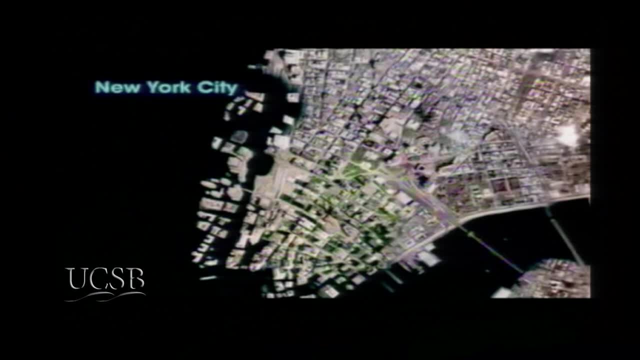 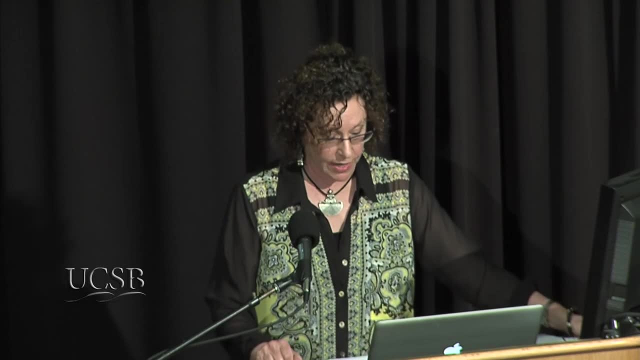 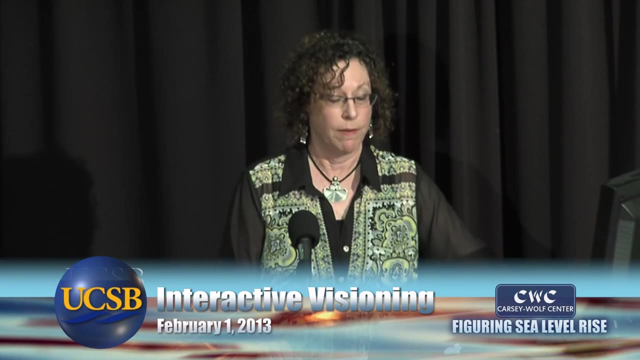 but could have been drawn in a different way. But could have been drawn from one of the proliferating interactive visioning sites, such as the Digital Coast Project of the National Oceanic and Atmospheric Administration, NOAA, designed to enable the user to toggle up sea heights to what they might be at some future date. 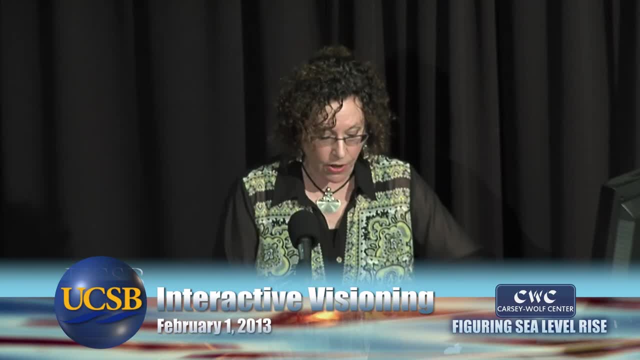 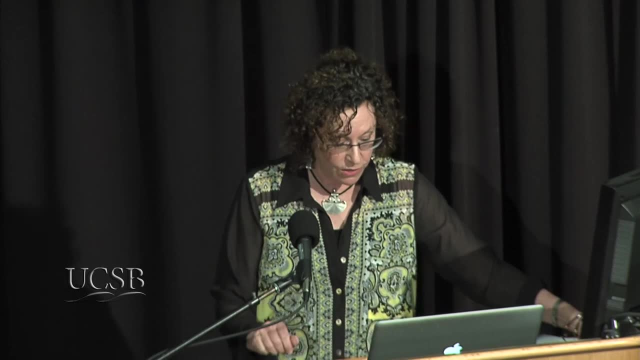 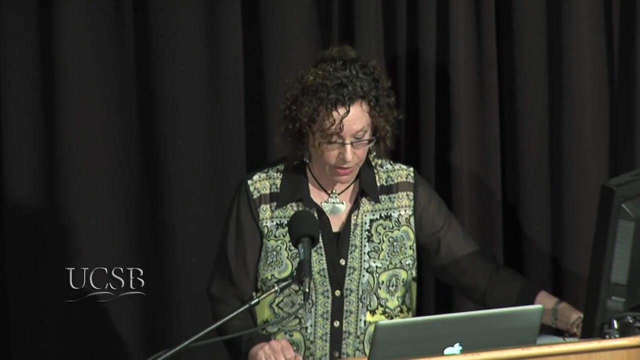 Today we're very fortunate to have with us our keynote speaker in the first session, Doug Marcy, the man behind NOAA's Sea Level Rise Viewer, And in the second session, Dr Jeremy Weiss, creator of the Climate Gem Tool at the University of Arizona. 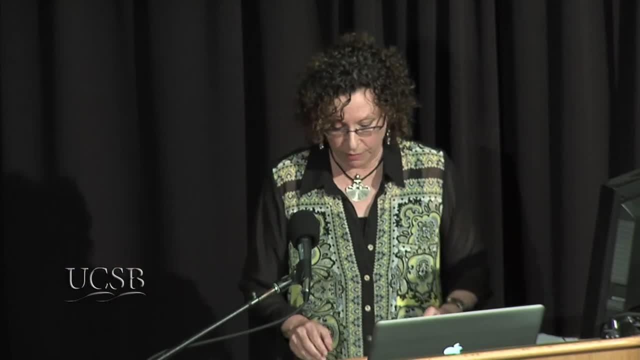 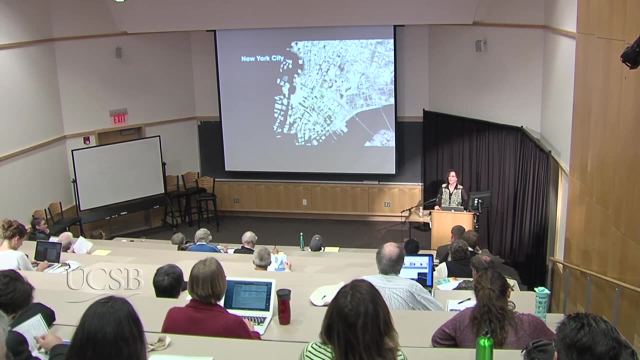 Dr Weiss is joined on the panel for the second session by three other visioneers who have imaged and imagined environmental change in technologically and media-rich manners of their own design. Each of these speakers will be introduced when we convene that second session. 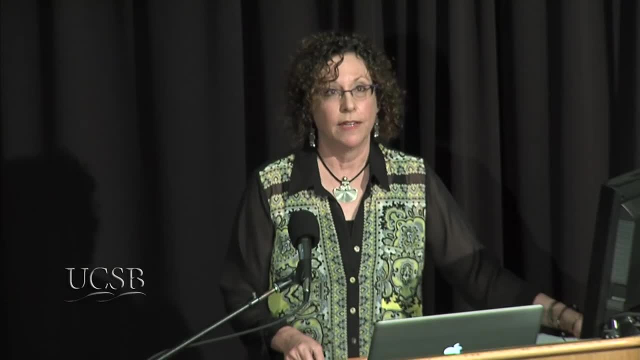 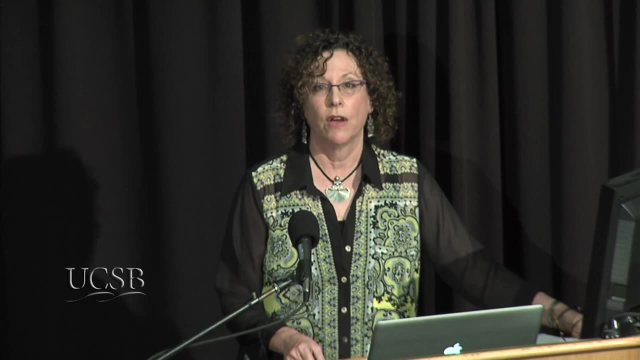 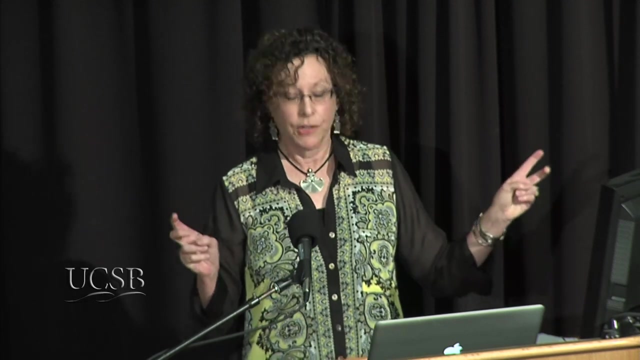 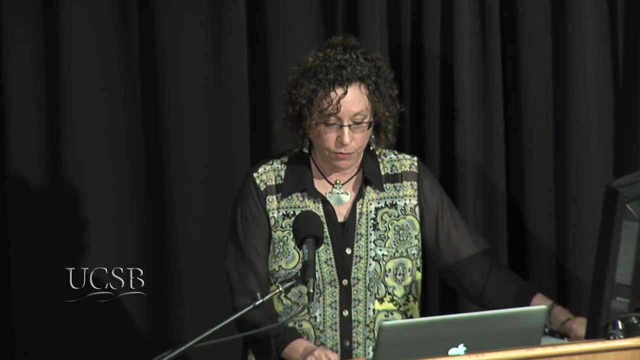 At the magnetic center of our initiative is the realization that sea level rise research is not only communicated, but also conducted and projected through highly mediated means. Our symposium on interactive visioning therefore entails a kind of conceptual toggling up from environmental documentaries to mediated sites such as map overlays, technologies of remote sensing. 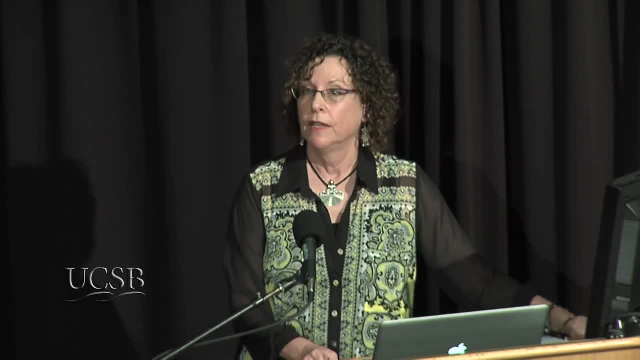 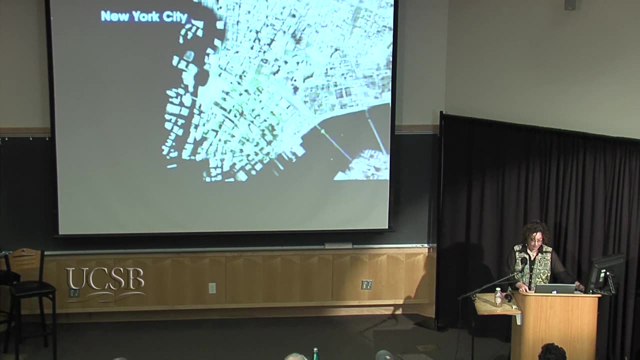 and forms of digital distribution that themselves constitute media and environment as entities that, in the words of Professor Constance Penley, influence, shape and inhabit one another. The geographer Catherine Youssef states that the catastrophe of climate change is upon us. 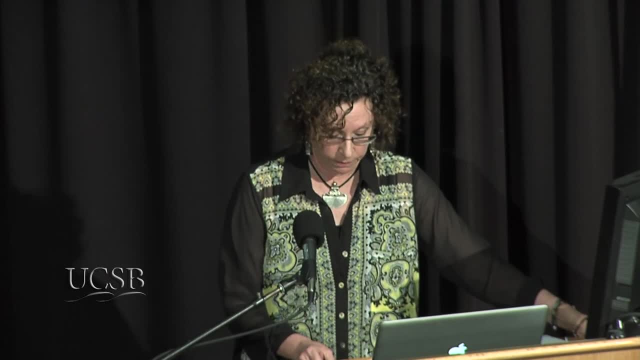 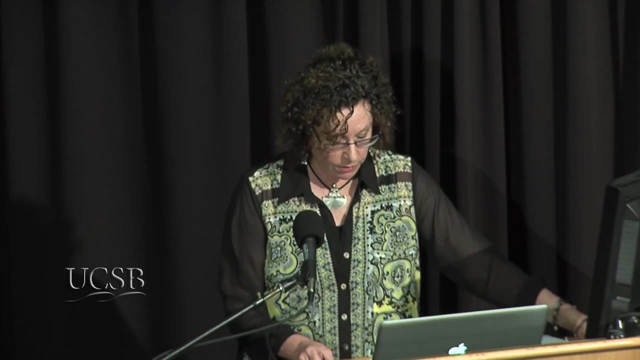 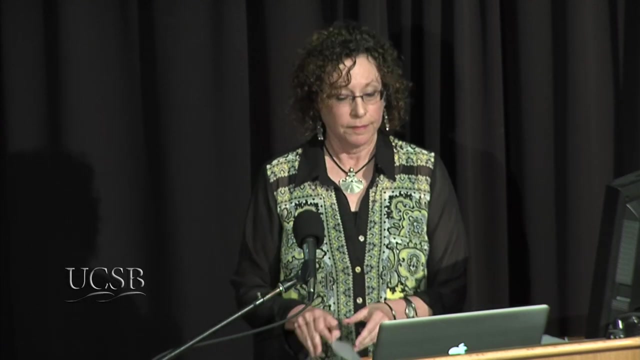 and that it is Earth, writing writ large, Taking cognizance of her harrowing perception. focusing on sea level rise. this symposium is designed to explore the potential of media as a means of Earth re-writing And speaking of Constance Penley. 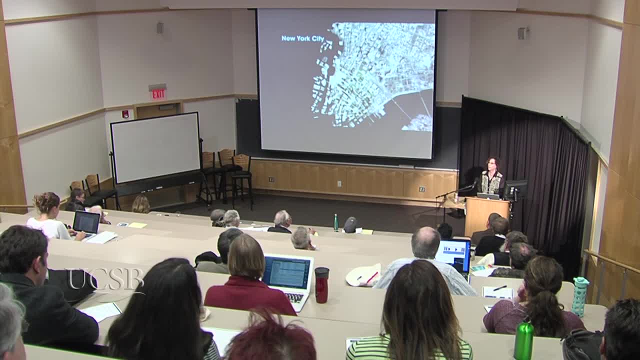 I'd also like to acknowledge the terrific boon of our being produced by the Carsey-Wolf Center, which is led by Executive Director Richard Hutton, with co-directors Ron Rice and Constance Penley and Associate Director Leanne French. 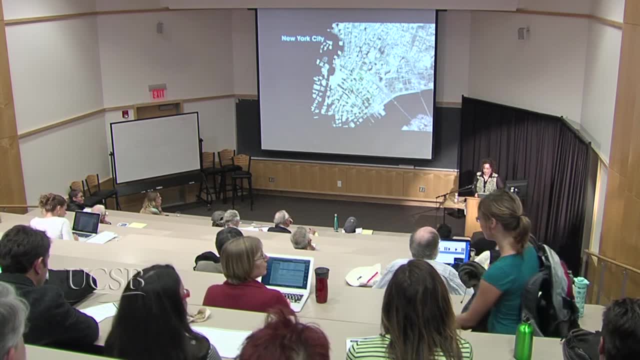 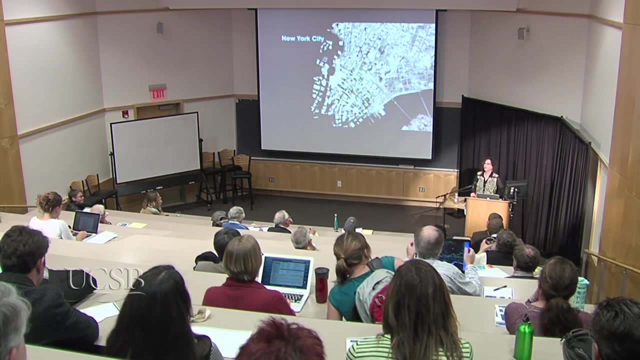 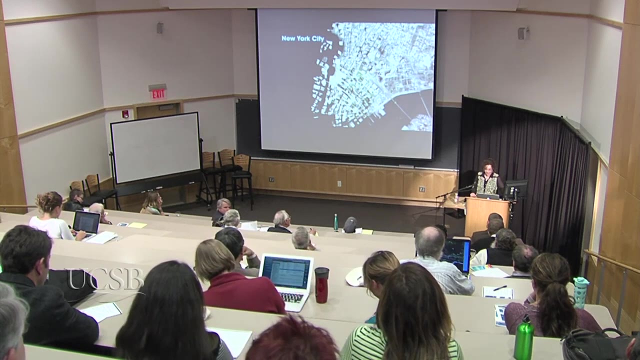 Leanne is a key member of our team. with an MA from the Bren School and incredible knowledge, energy and diplomacy, She's really the main person who has figured out figuring sea level rise. Dean Tiffany mentioned the College of Letters and Science as our inaugurating sponsor. 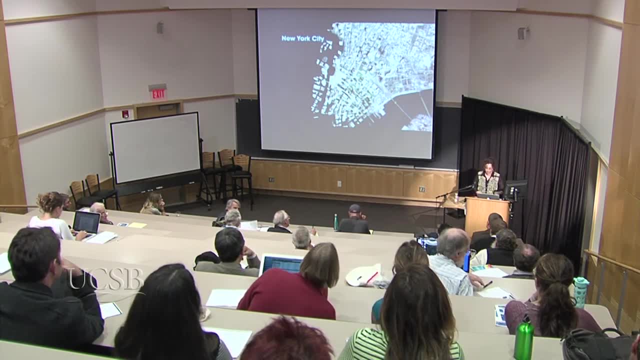 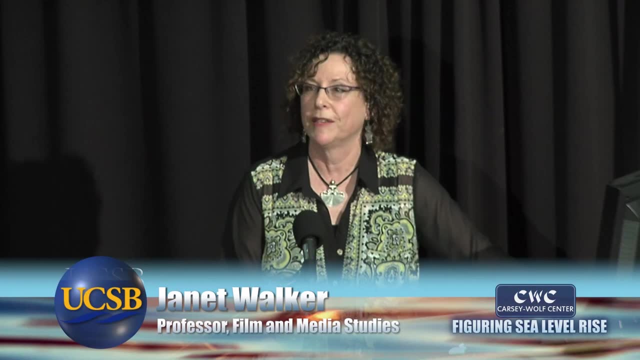 The Center for Information and Technology, led by Lisa Parks, contributed in particular to this day, And please do consult the printed program with thanks to our superb assistants, Erin Hannan and Madeline Fitzwater, for the long list of co-sponsors. 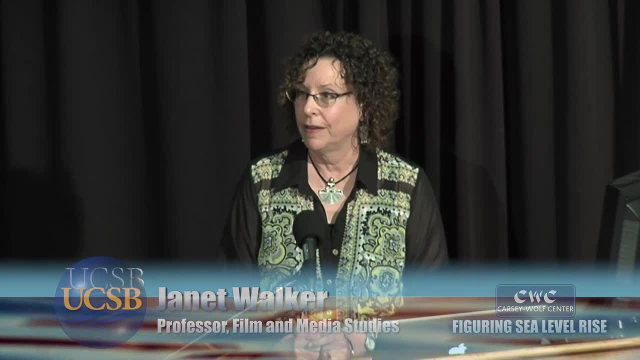 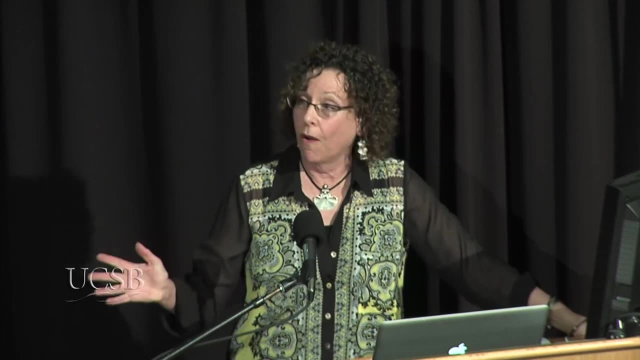 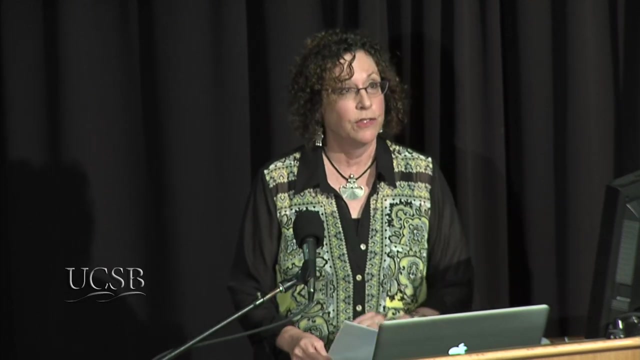 The whole is great, but the sum of the parts is pretty impressive. Today's symposium will unfold in two sessions. The first session: we are honored to welcome our keynote speaker, Doug Marcy, Coastal Hazards Specialist with NOAA. I am obliged to report that our other slated speaker, 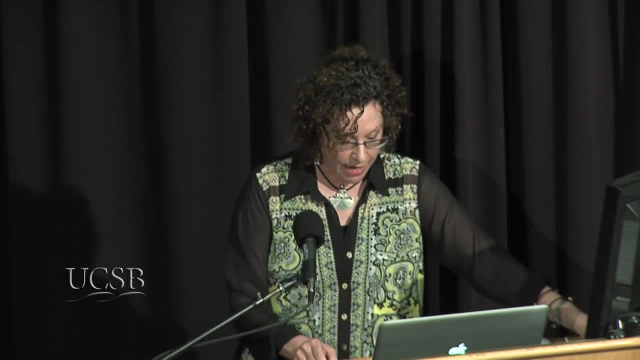 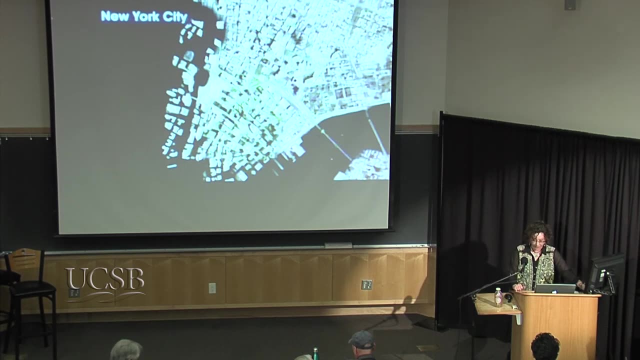 Mike Lemenick of Climate Central came down with the flu and wasn't able to fly out to join us today. but Doug Marcy has graciously agreed to delve into a few more areas and it's really great that we'll have time to engage with him. 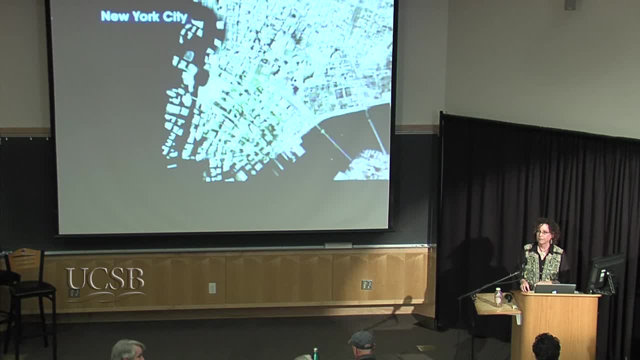 in the question and answer session following the talk. So we'll have Doug Marcy's talk and then we'll take a break and we'll reconvene for a panel presentation of six lightning or Pecha Kucha style talks and a discussion with the author. 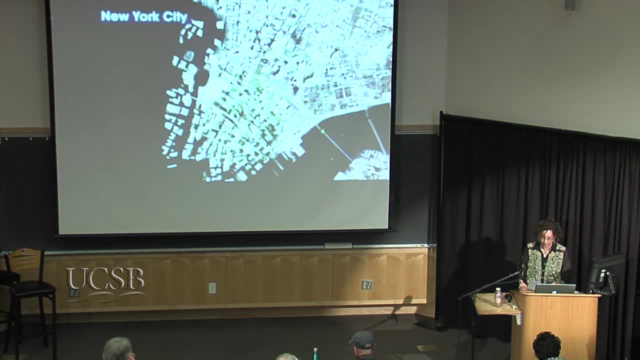 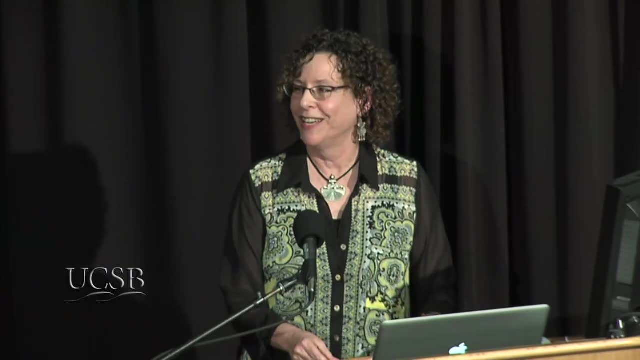 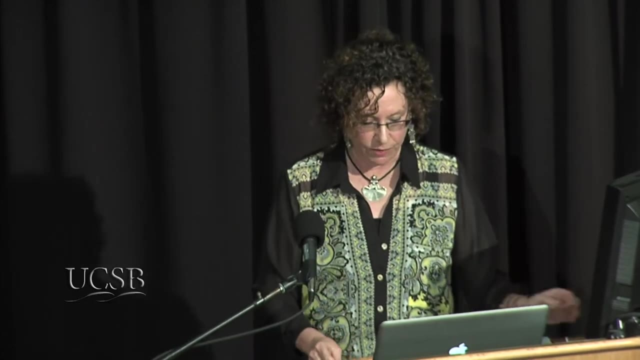 and the audience moderated by Professor Lisa Jevrat, And she will go ahead and introduce the panelists and the whole session when the time arrives. So it's my great pleasure to introduce Doug Marcy at this point. As I said, Coastal Hazards Specialist with NOAA. 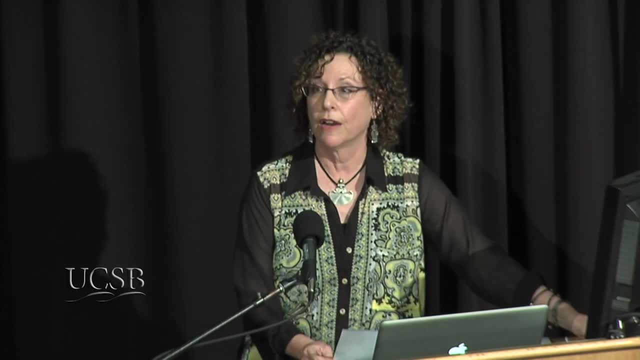 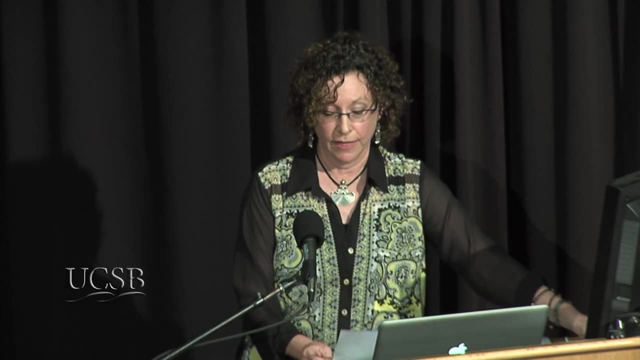 National Ocean Service and Coastal Services Center in Charleston, South Carolina. He's been with CSC for over 10 years, working on enhancing coastal inundation products and GIS capability, storm surge assessments and coastal hazards assessment projects, contributing to more disaster resilient communities. 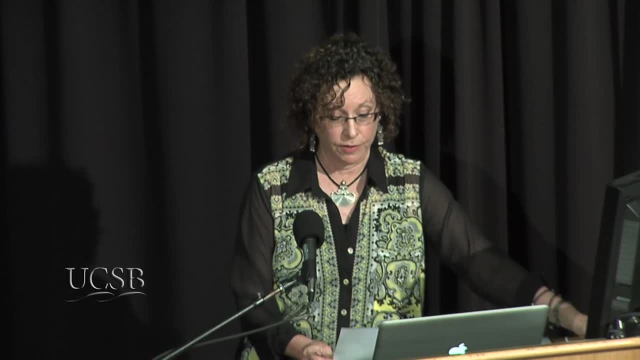 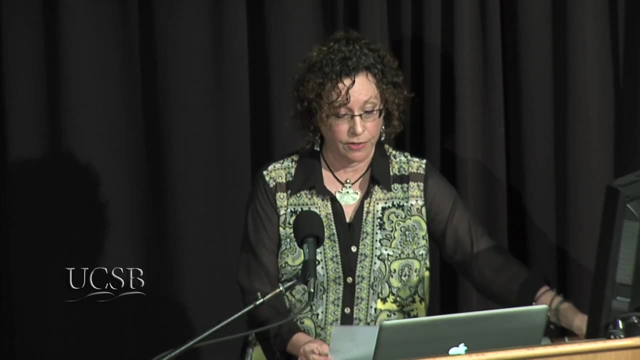 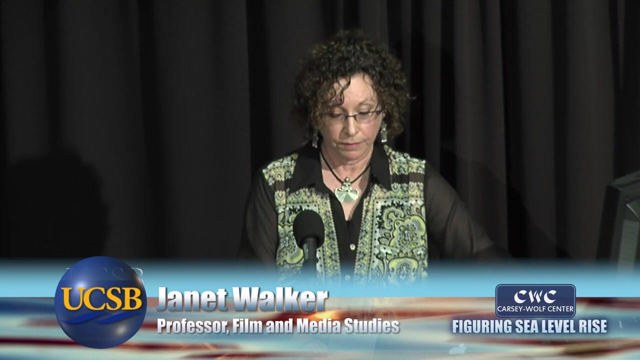 He has received both the Department of Commerce Bronze Medal Award and NOAA Administrator's Award for contributions to hurricane response and climate change science. Before coming to NOAA, Doug worked as a hydraulic engineer with the US Army Corps of Engineers. He has an MS in coastal processes. 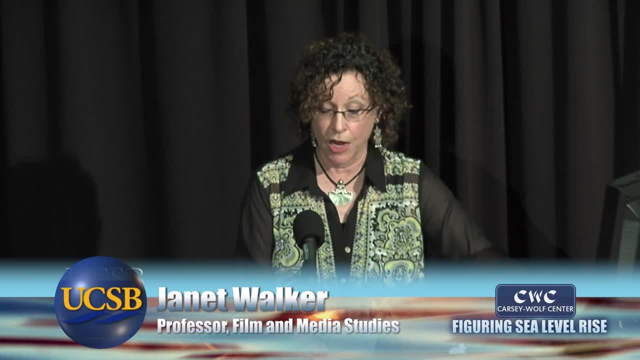 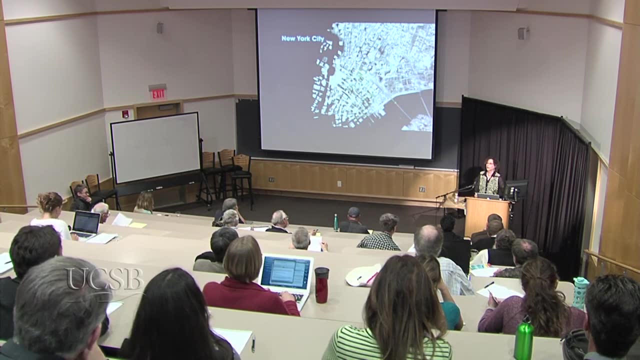 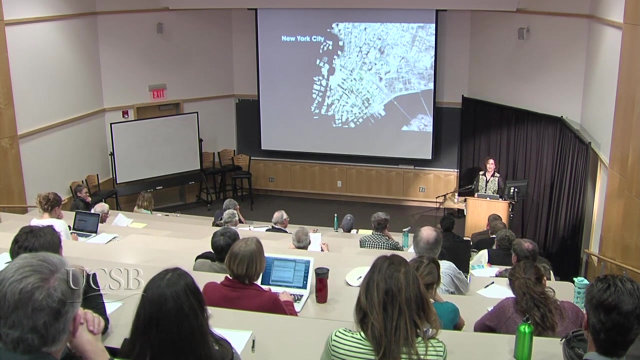 from the University of North Carolina at Wilmington and a BS in geology. His current interests, as you will see, include using GIS technology with meteorologic, hydrologic and coastal modeling to enhance inundation forecasting, mapping and risk assessment. 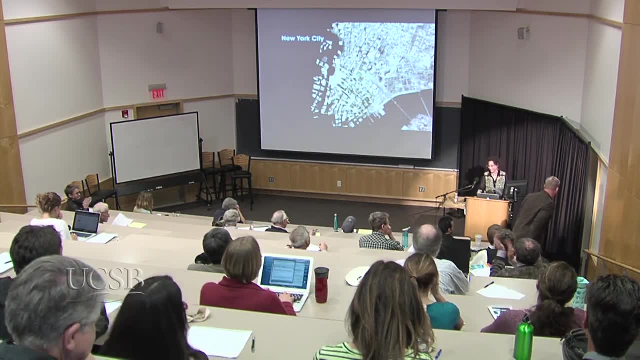 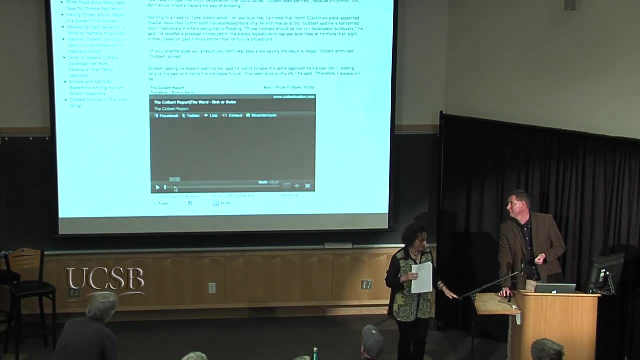 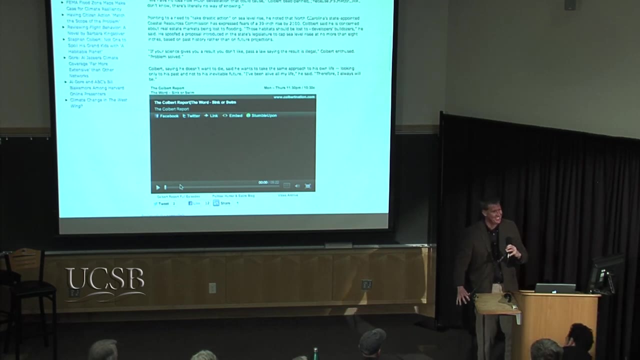 So I now welcome Doug Marcy. Okay, Thank you, Janet. I'm 6'5", so I've got to do this. Yeah, Did I write that whole bio? Geez, I should have cut that down a little bit. 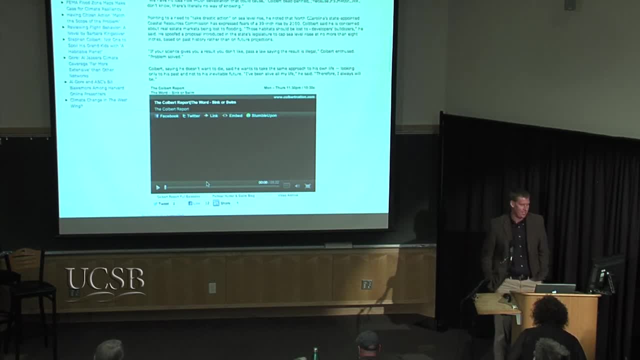 Thank you very much for inviting me out here to speak with you guys today. This is a subject matter near and dear to my heart. We've been working in the past. Like I said, I've been with NOAA 10 years. I was with the Corps before that. 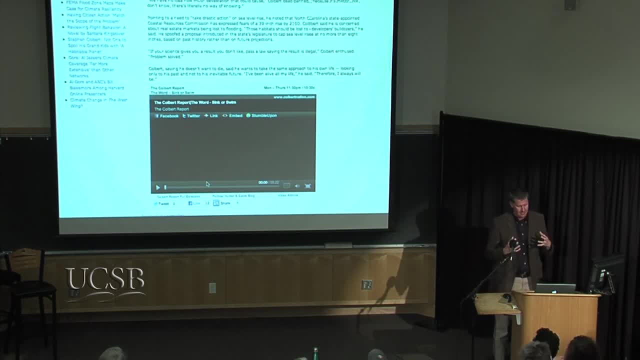 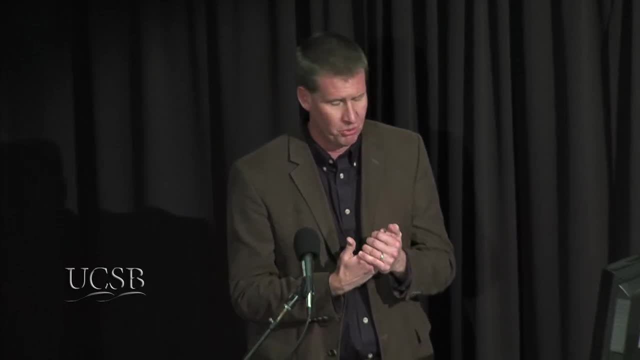 really trying to translate And what our office does is translate. NOAA is pretty much a science agency and we produce a lot of really good data. We have a lot of good modelers, But we fall short sometimes on actually communicating that important information to the public. 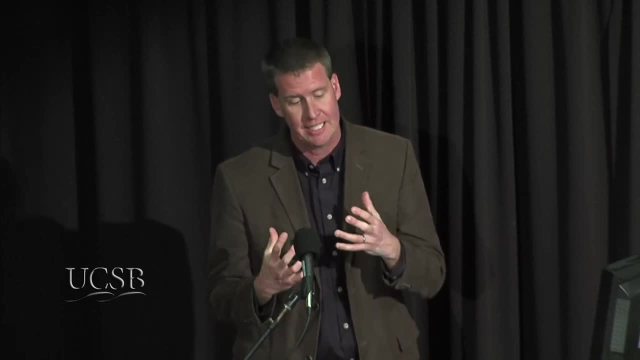 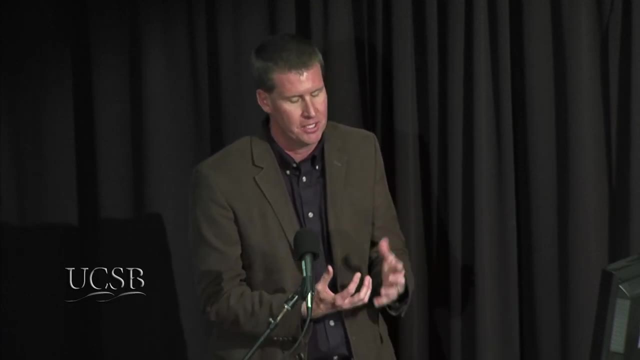 and also to decision-makers. So we really concentrate on trying to translate that science in meaningful ways through mapping and through visualizations, so people can actually use that to make decisions. So I'm going to be going over that a little bit in my presentation today. 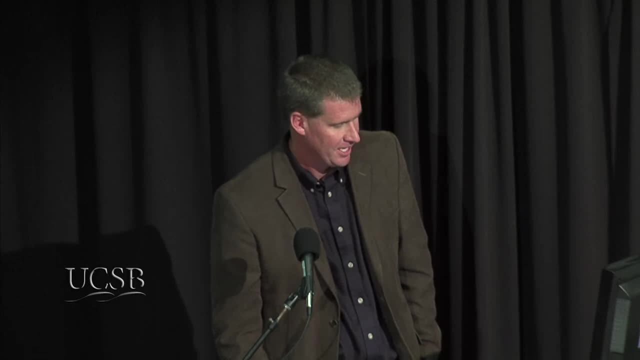 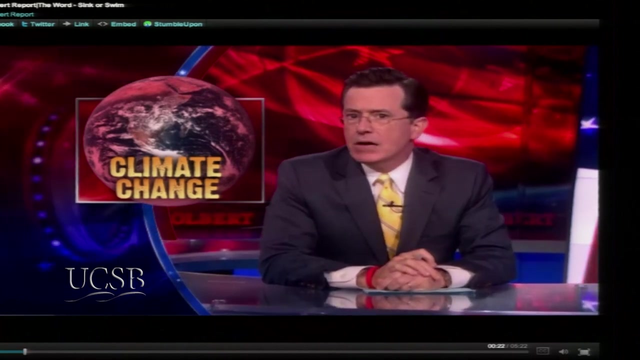 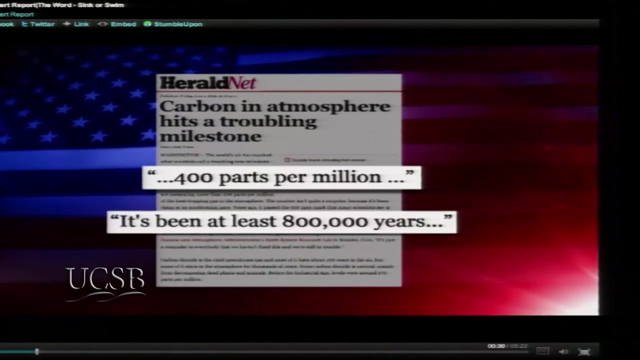 But first I thought I'd start out with something that can get this kicked off pretty good here. Troubling news from the so-called scientists. Now they're saying that the CO2 levels in the air have surpassed 400 parts per million for the first time in 800,000 years. 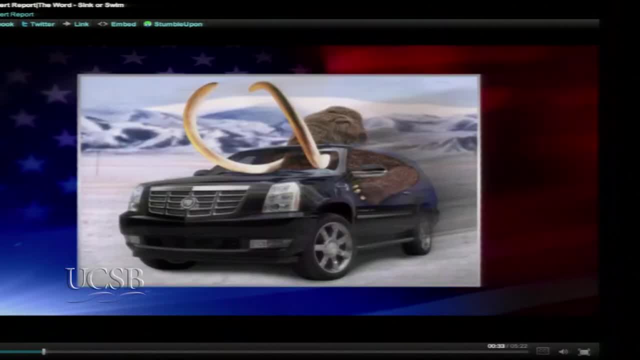 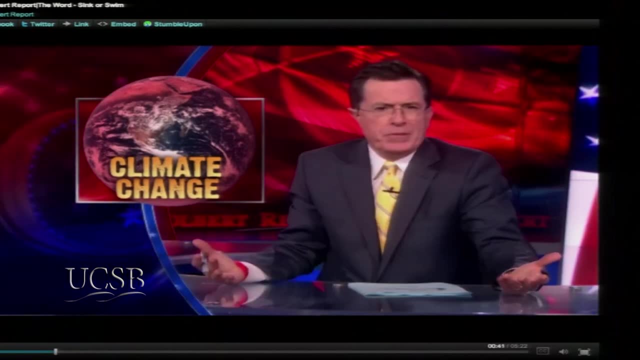 when woolly mammoths roamed the Earth in escalades. But, folks, I don't buy it. First of all, what do they mean? 400 parts per million? Air's only got two parts: The breathy part and the part that makes balloons go up. 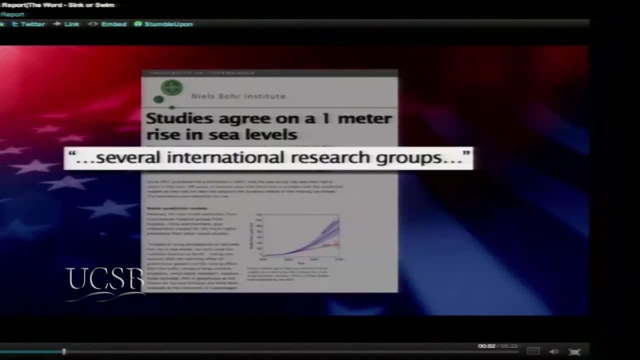 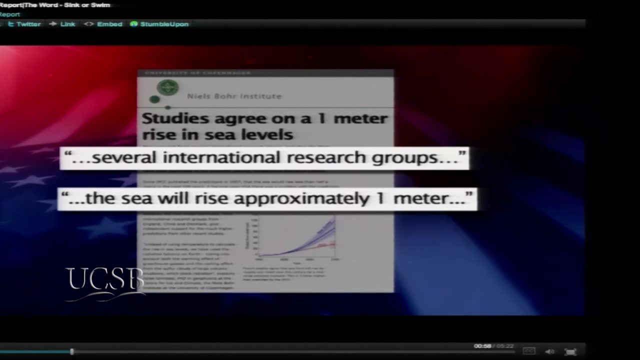 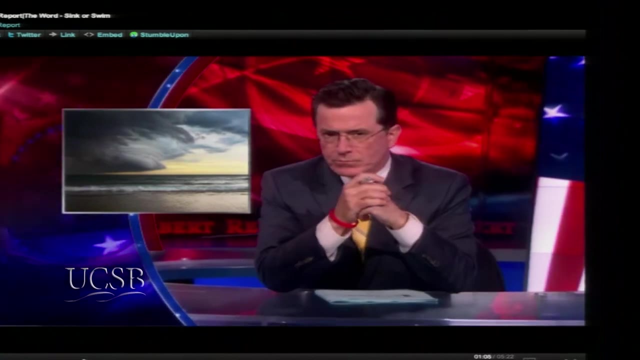 But these alarming climate numbers have led international research groups to predict that in the next 100 years, sea levels will rise by approximately one meter. We have no idea how much devastation that could cause, because it's metric, But We don't know. 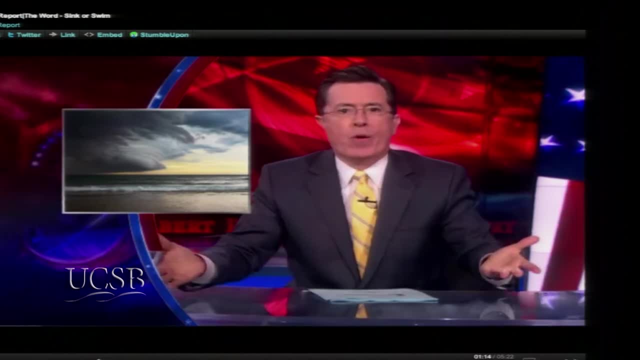 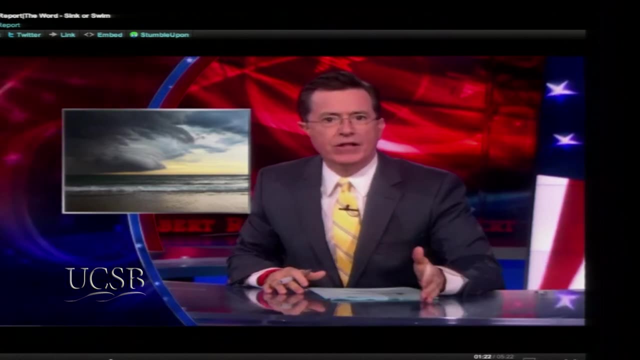 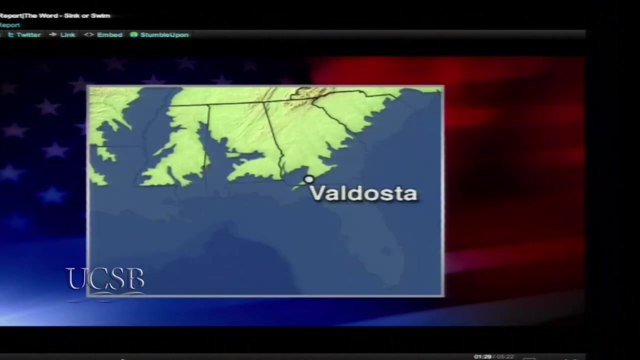 No way, There's. no, There's literally no way of knowing. But theoretically it could cost coastal communities billions of dollars in damage and lost development. Plus, who's gonna want to watch MTV Spring Break from Valdosta Georgia? 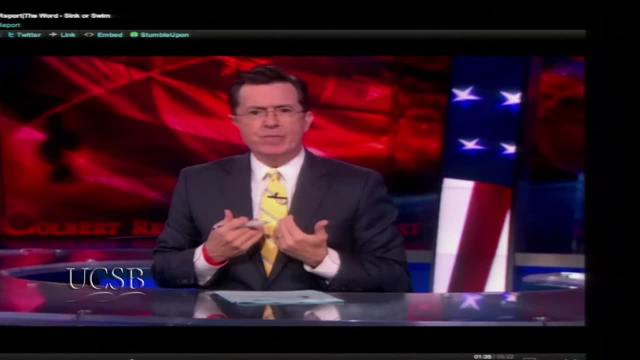 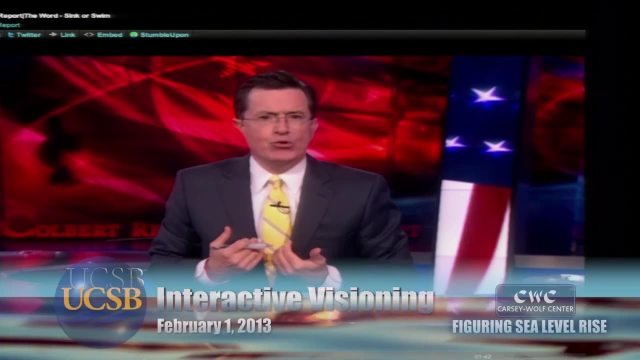 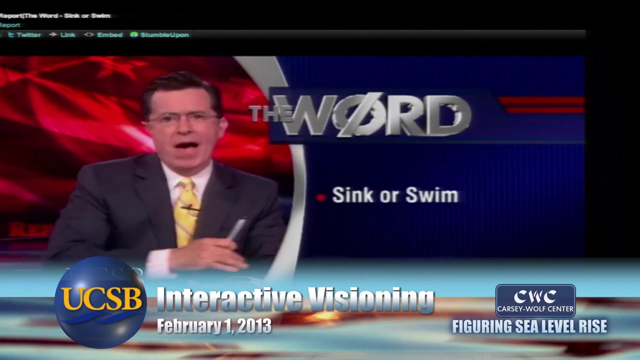 Nation. this issue is near and dear to my heart and, more importantly, near and dear to my beach house in South Carolina. So it is time to take drastic action. and that brings us to tonight's word: Sink or swim folks. 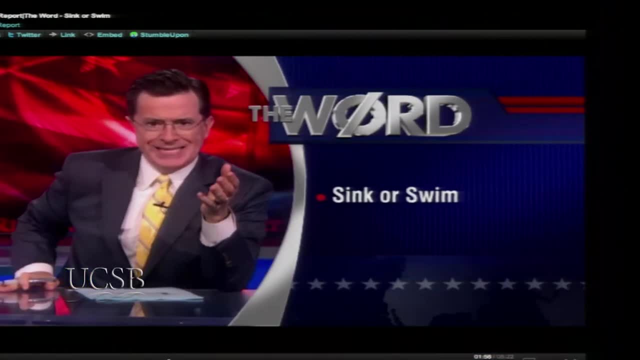 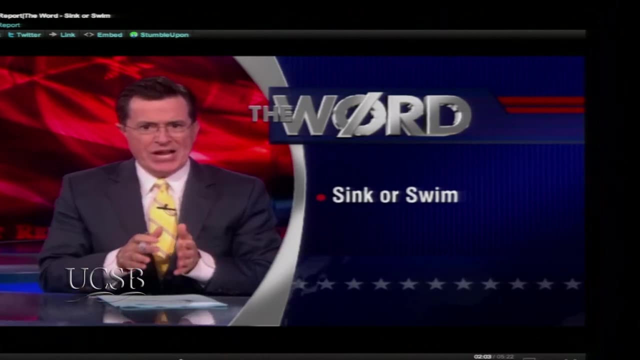 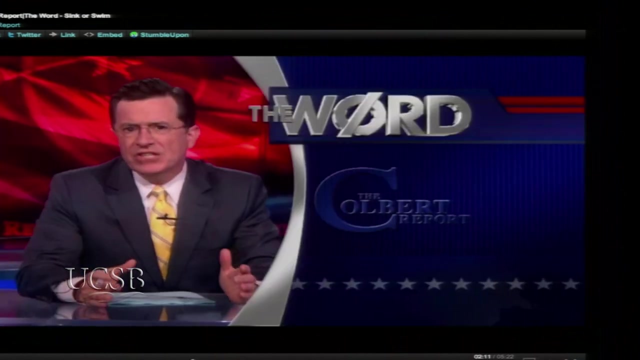 Now, I'm from the Palmetto State, but South Carolina's neighbor, North Carolina, is also worried Because their state-appointed Coastal Resources Commission has projected a 39-inch rise in sea level by the year 2100.. That would devastate the coastal real estate market. 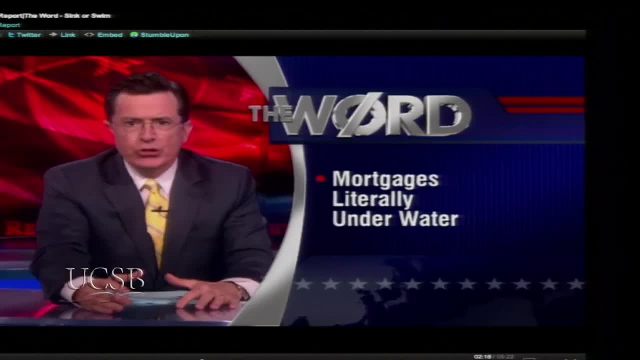 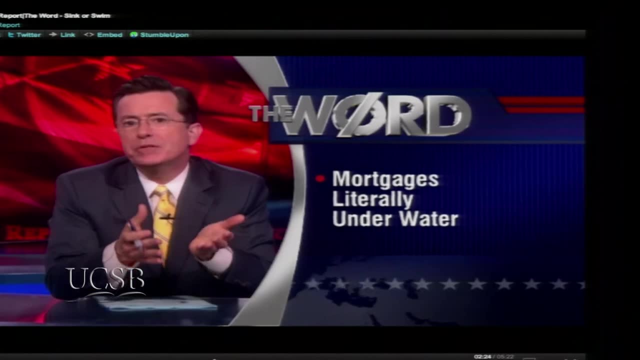 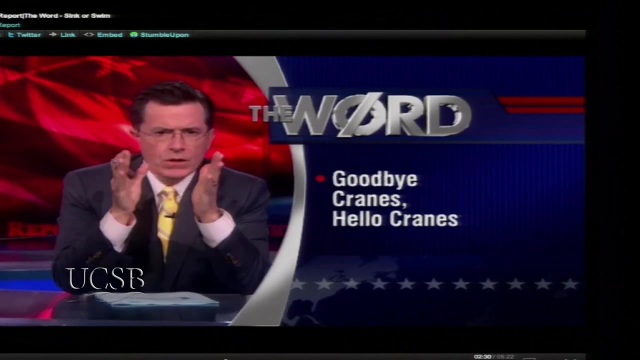 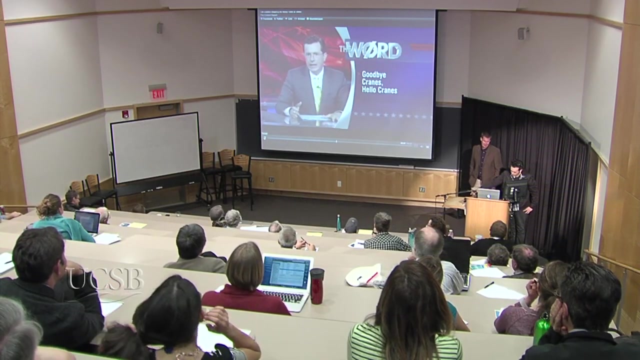 And folks. it would be a tragedy to lose precious coastal wildlife habitats to flooding. Those habitats should be lost to developers' bulldozers. Now, Folks, Fortunately, fortunately, folks. North Carolina Republicans have drawn a line in the soon-to-be-underwater sand. 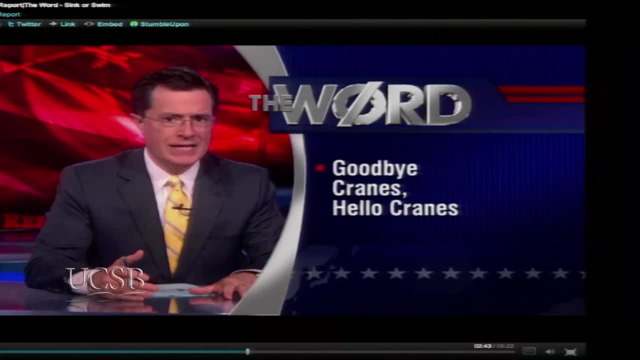 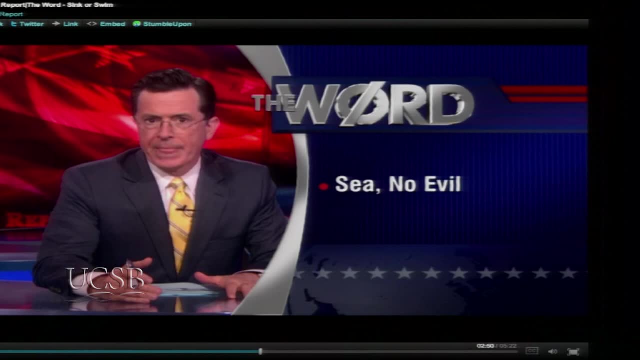 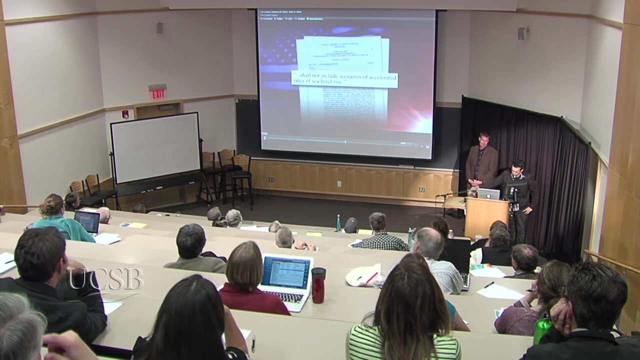 They have written a new bill that would immediately address the crisis predicted by these climate models by outlawing the climate models. Here's how it works. Here's how it works. The law makes it illegal for North Carolina to consider scenarios of accelerating rates of sea level rise. 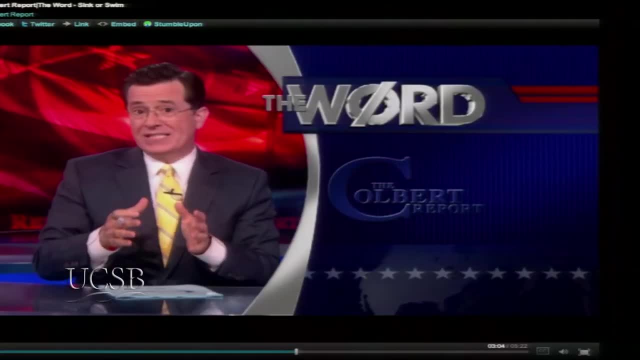 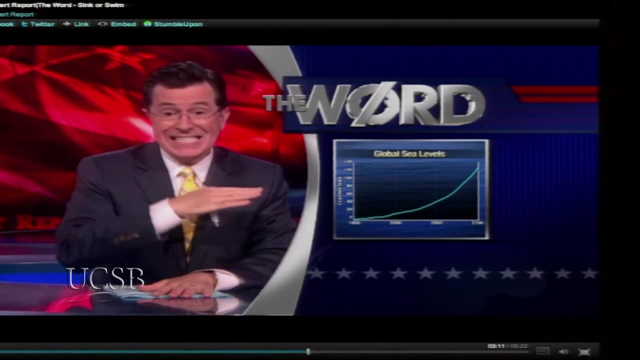 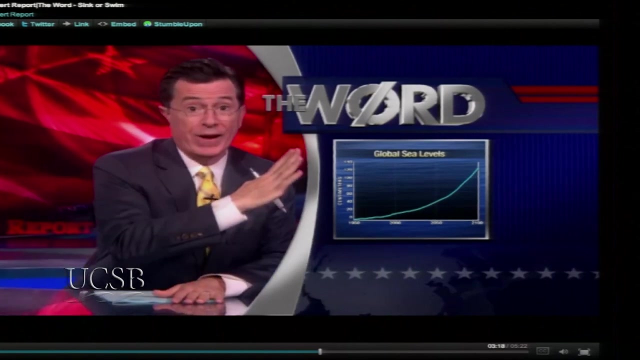 due to global warming. You see, right now, all the scientists' sea level predictions look like this: That steep curve, that's bad. That ski jump to hell there. that's predicting that things are gonna get worse and worse in a feedback loop that accelerates. 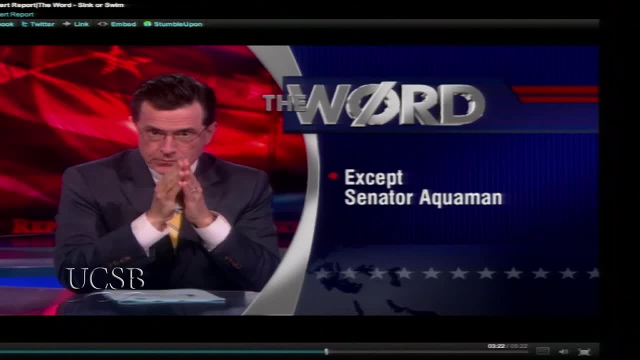 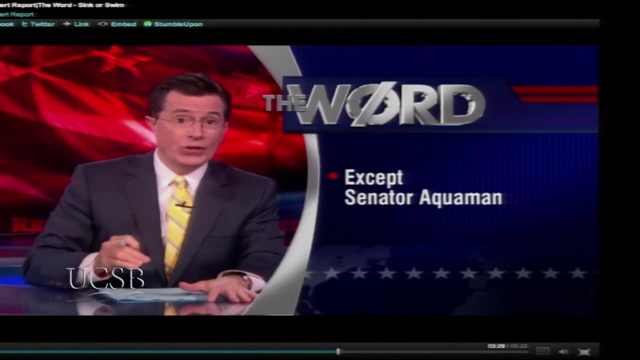 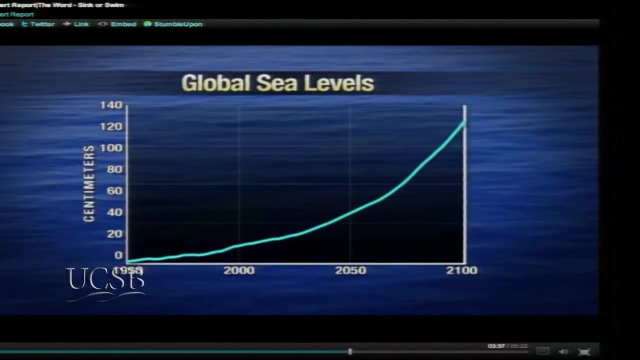 No politician wants that. So to fix, to fix that problem, GOP lawmakers want the state to consider only the sea level rise over the last hundred years, then predict that's what will happen in the future. That makes that scary chart get all better. 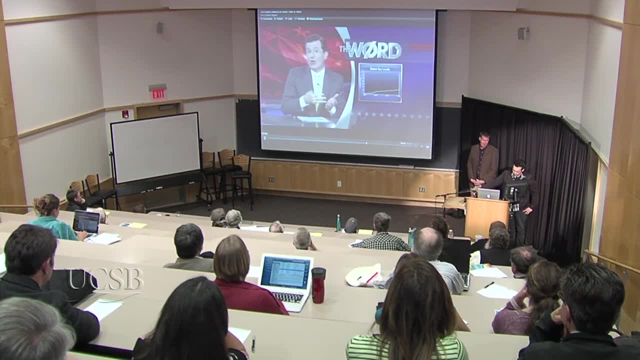 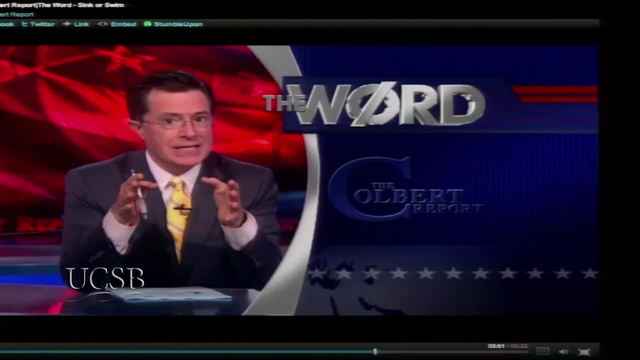 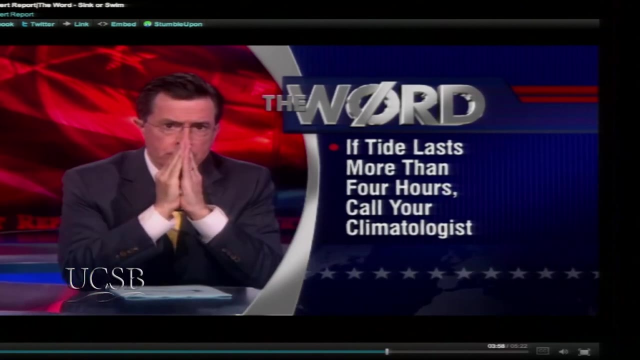 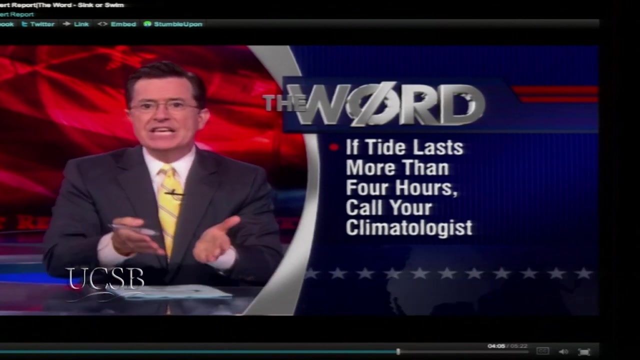 Now, instead of the economy destroying 39-inch rise, the law makes it a rise of only 8 inches, And that shrinkage makes sense because the water is cold. Now, folks, I think this is a brilliant solution If your science gives you a result that you don't like. 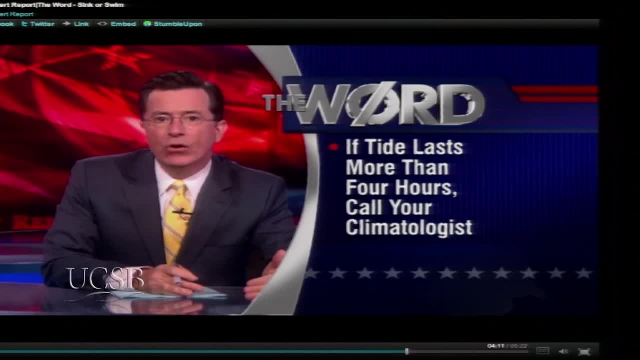 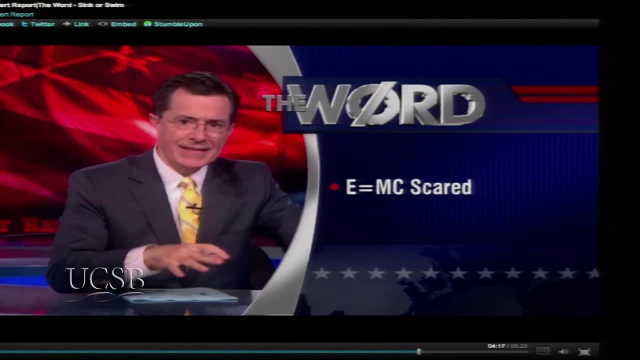 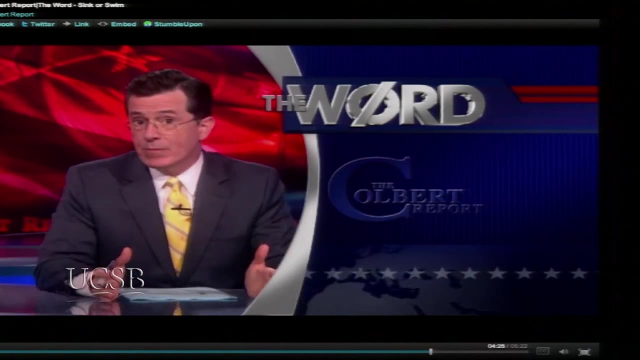 pass a law saying that the result is: illegal Problem solved Now, in fact, I think we should start applying this method to even more things that we don't want to happen. For example, I don't want to die, But the actuaries at my insurance company. 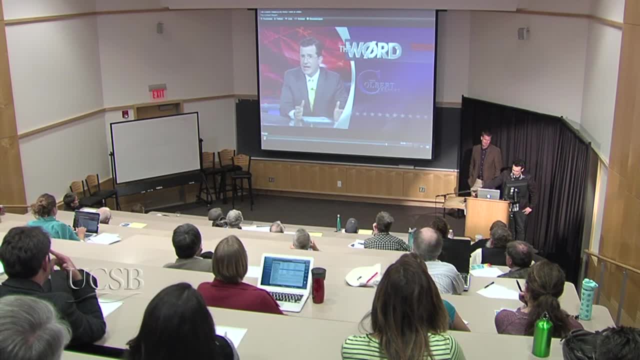 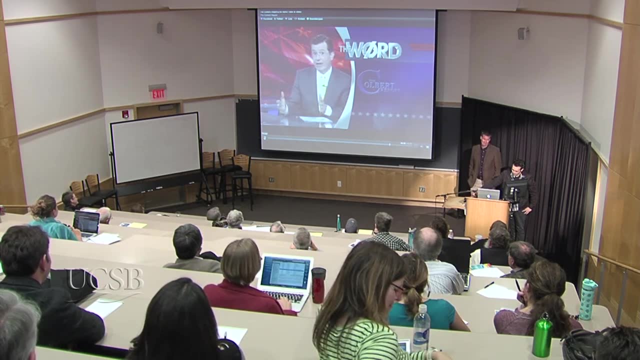 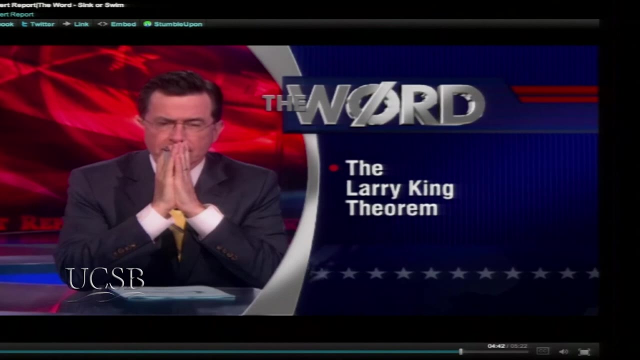 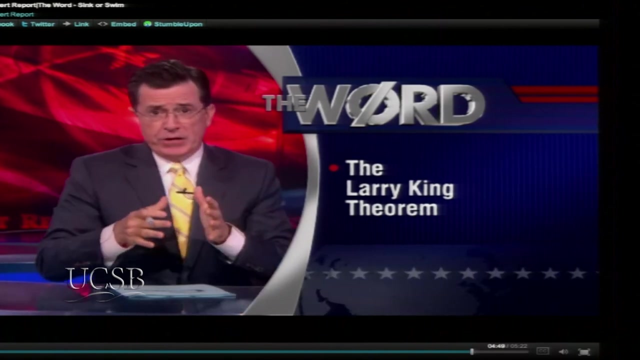 are convinced that it will happen sometime in the next 50 years. However, if we consider only historical data, I've been alive my entire life. Therefore, I always will be, And. And if you extrapolate my life from the critical periods of age 8 to 18,, 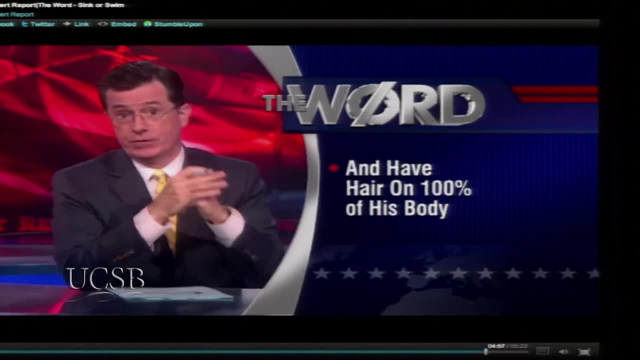 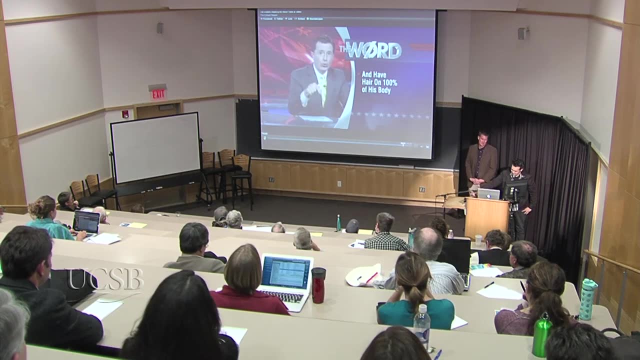 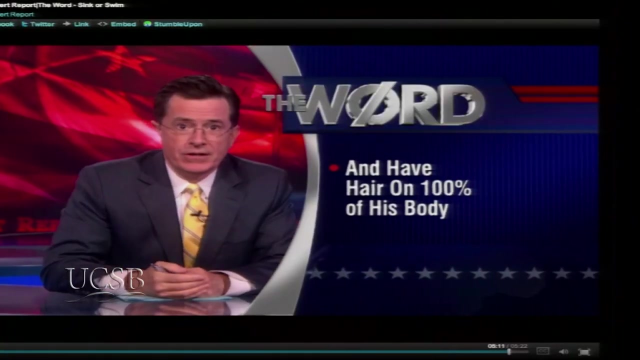 I will grow to be over 20 feet tall, So I say: bravo, North Carolina. By making this bold action on climate change today, you're ensuring that when it actually comes, you'll have plenty of options, Or at least two. 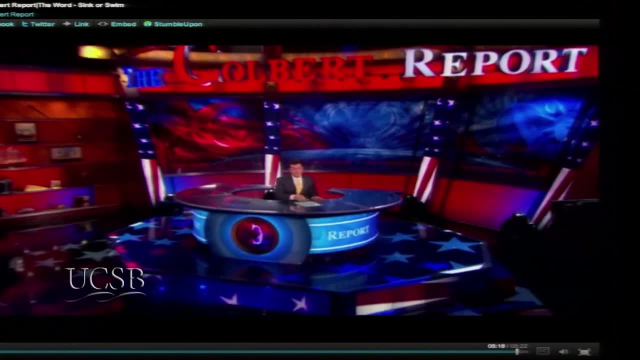 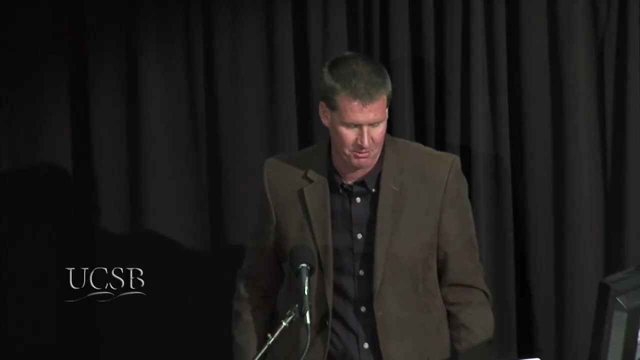 And that's the word. We'll be right back. So now we want to get into- I thought it was a good opener- making light up something that is, you know, pretty close to where I live in Charleston, and we're getting ready to do some products. 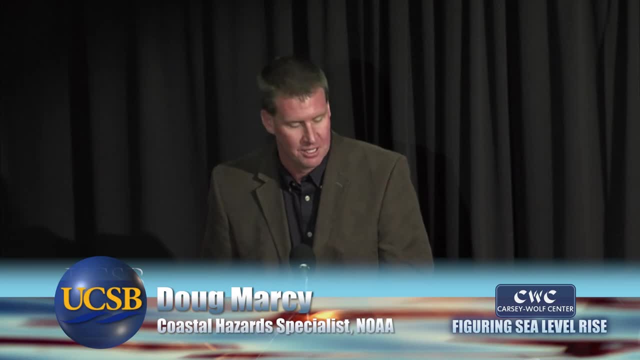 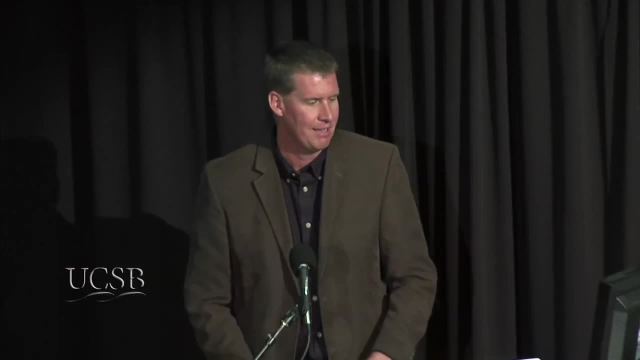 that I'll show you today in North Carolina. So at the time we were like, well, maybe we should wait a little while before North Carolina figures this out. So when it comes to visualizing sea level rise, and I'm going to talk about it in kind of two ways- 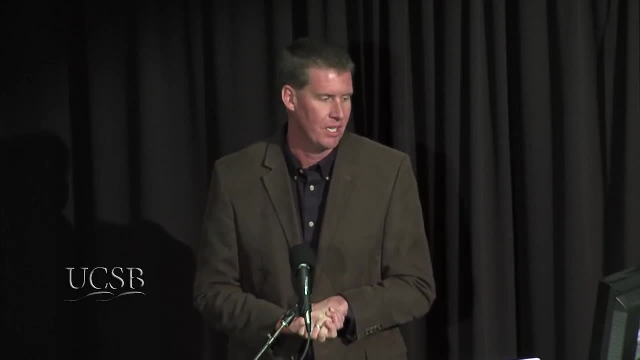 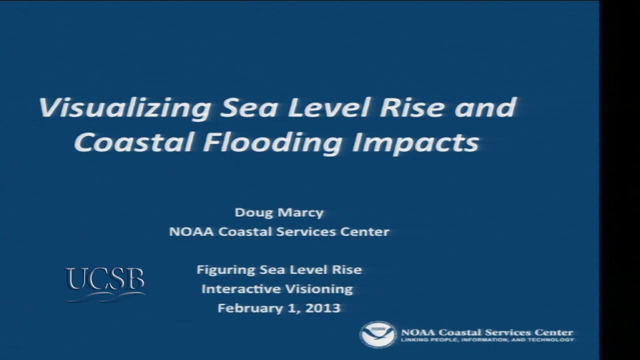 Sea level rise, yes, but also we're really concerned about the coastal flooding too that comes along with it, And that means the episodic events that we get, the storm events- those are really what cause the high water levels that impact us. 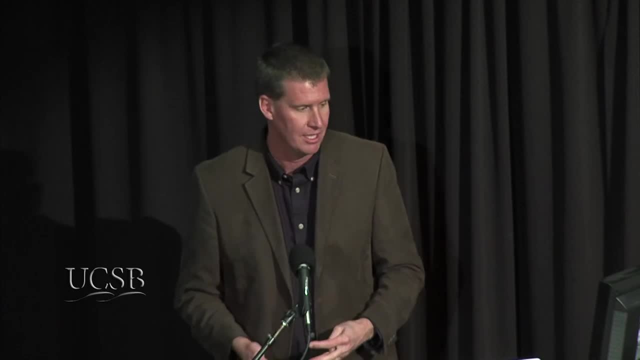 and those are just going to become worse and more frequent when sea level rise. So sea level is almost just an increase in the overall signature of the water levels. and then we have our storm events on top of that. So the old adage comes in. 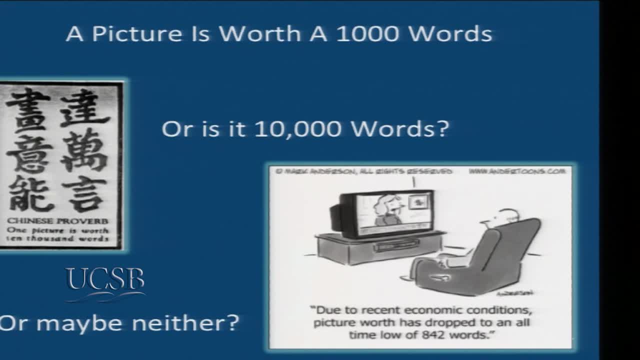 probably overused, but a picture's worth a thousand words. I started to research this. It's actually based on a proverb, a Chinese proverb. that was actually: one picture is worth 10,000 words. but then I found this pretty cool cartoon. 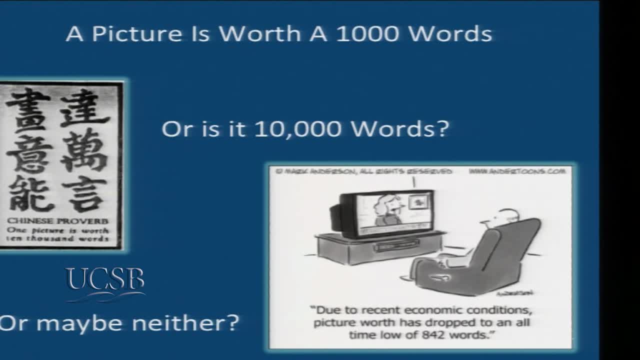 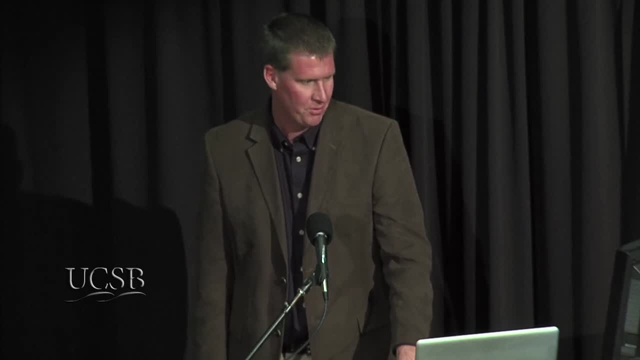 Maybe it's neither. Due to recent economic conditions, picture worth has dropped to an all-time low of 842 words, So apparently we're not getting our value on pictures, but hopefully we will. today At our office, we've been working a lot. 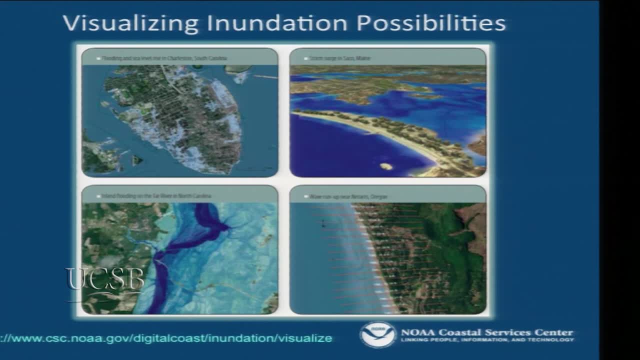 on not just sea level rise but also other types of coastal flooding and even riverine flooding. So we've been doing a lot of work with visualizing storm surge using storm surge forecasts from some of the modeling projecting what that looks like over the land. 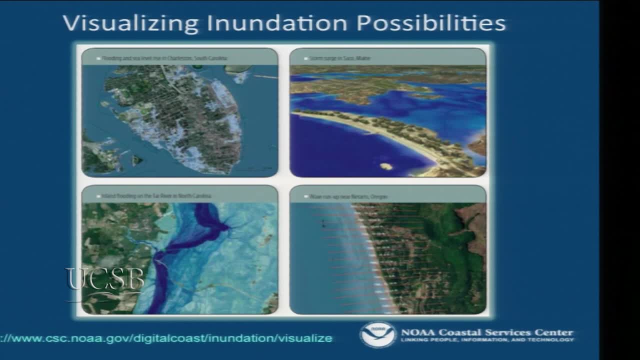 how deep the water might be. We've done some work on wave run-up. Wave run-up is a big issue on the West Coast, Not so much storm surge but the wave setup and the run-up causes a lot of issues. And then, of course, the rest of the country. 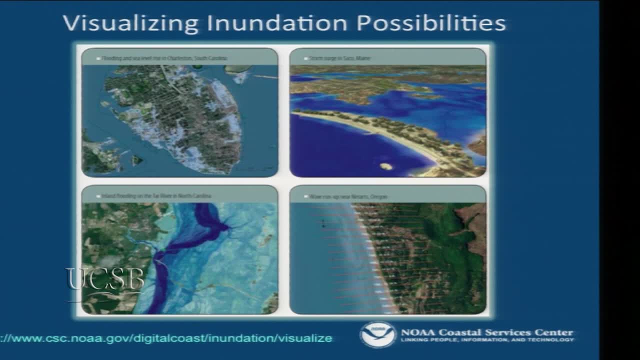 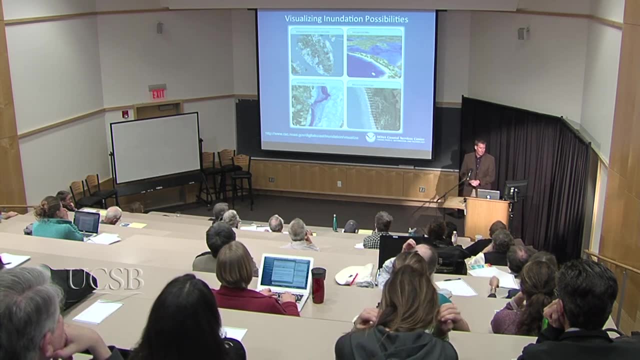 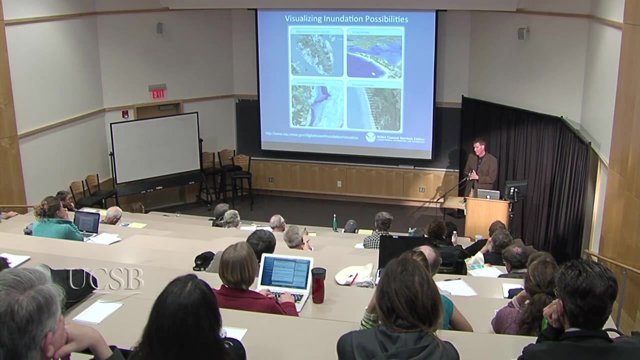 flooding is a major part of you know, in spring, thaw from snow melt. Especially on the Mississippi, we get riverine flooding. So in the past, basically, we had forecast information that was in a text-based format. The National Weather Service would put out these: 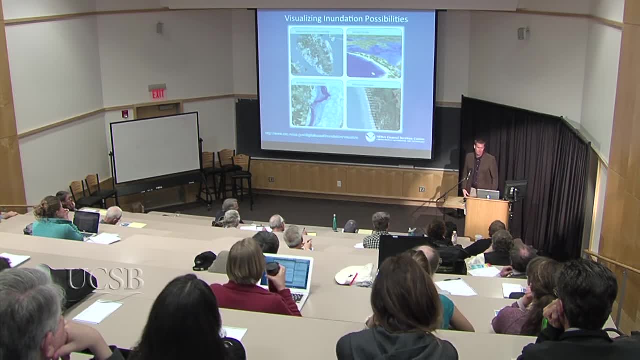 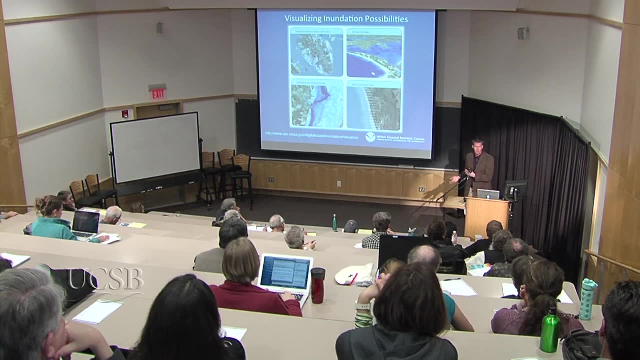 you've probably seen them all capital text format and it's very hard for people to understand. And if you're not from that area, it may say that this river's going to crest to 12 feet. What does that mean? So we can take that information. 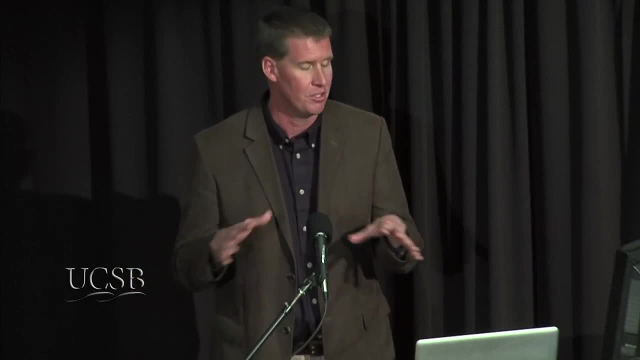 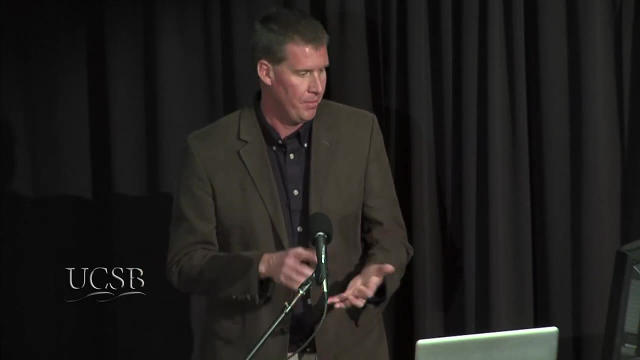 and put it into the GIS- environment geographic information systems- and start to map what is actually going to be impacted And once you do that, we can start doing analysis overlays to figure out how much property is that going to affect and what is the economic cost going to be. 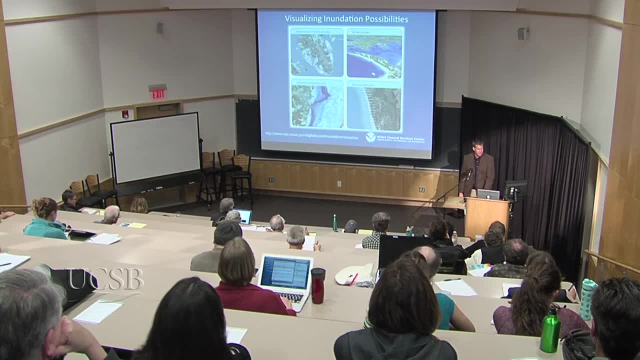 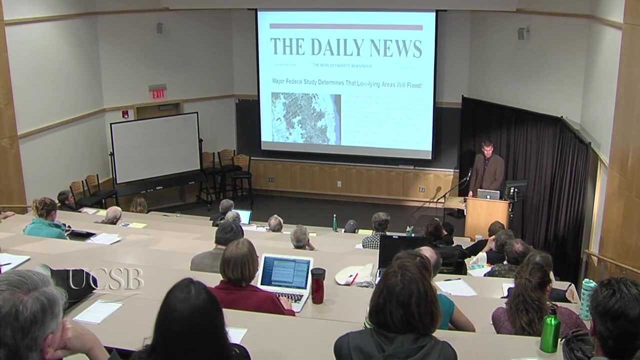 And then I'll talk a lot about some of the sea level rise visualizations and ways we can try to communicate that this is becoming a more frequent problem. But what it all comes down to, This is my favorite. I had a colleague of mine make this. 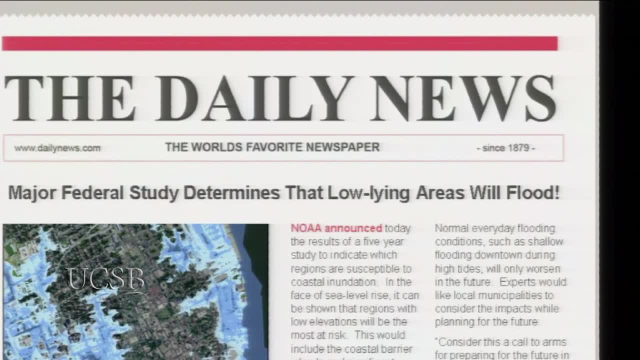 This is all we're trying to do. We're trying to tell people that they live in low-lying areas and they're going to flood. That's what we're boiling this down to, And in many cases it's like you have to try to get people. 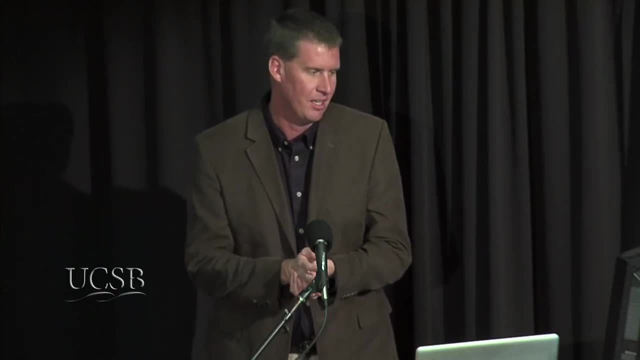 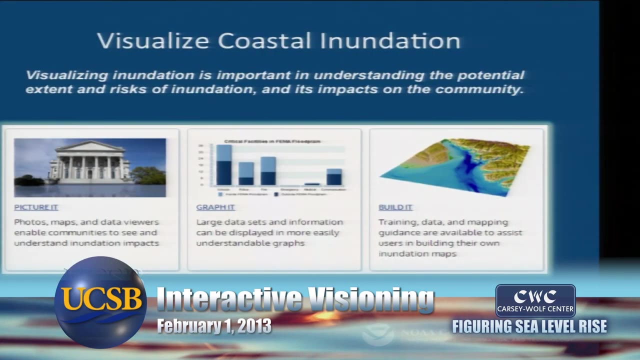 you hit them over the head with the same information a lot of different ways, and that's what I'm going to try to talk about today. So visualizing inundations it's an important thing, and that's because we need to understand the potential extent and the risk of inundation. 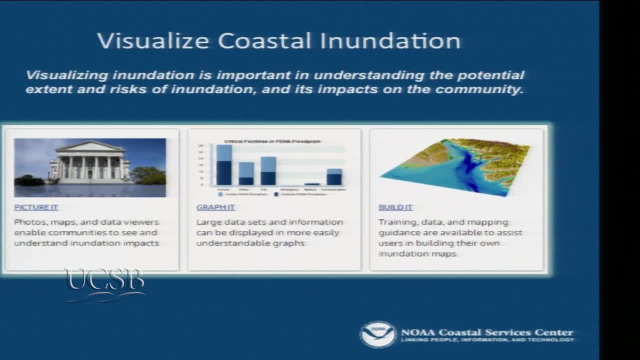 and the impacts on the community. So if you're a true engineer- which is sort of the background I came from working at the Corps of Engineers- is the risk equation is probability, times, consequences and it's really the probability of an event occurring. 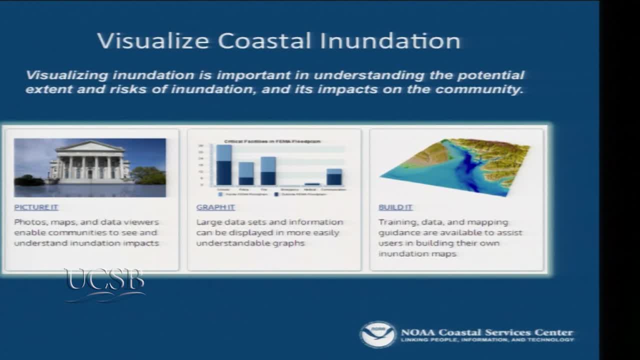 but it's also what is going to happen. So it's not just map the risk, it's not just show an inundation layer, but overlay that on something and determine how much of loss is going to occur. So I'm going to go through three different ways of doing this. 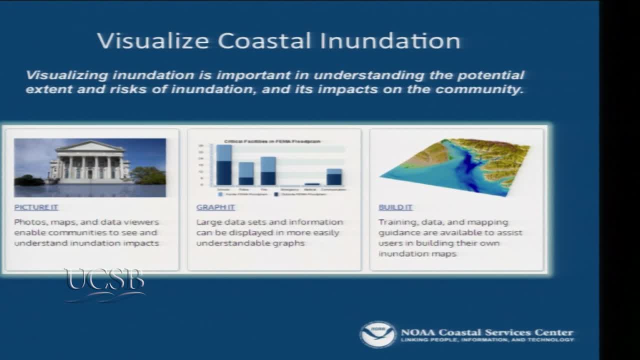 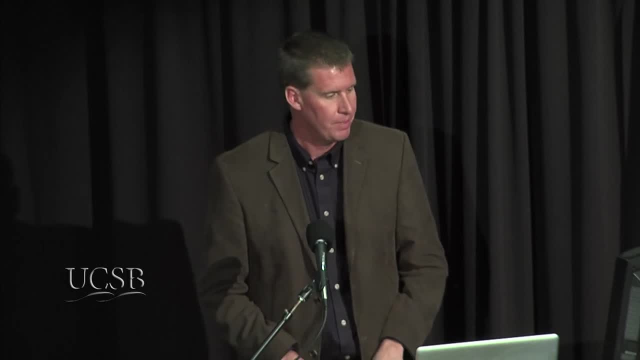 We can picture it, We can graph it And we can build it, And this is building off of kind of information we have, and Janet mentioned our Digital Coast page and it's a website that has a collection of resources there and data. 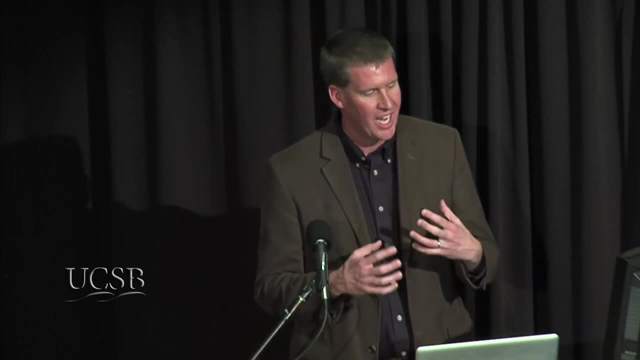 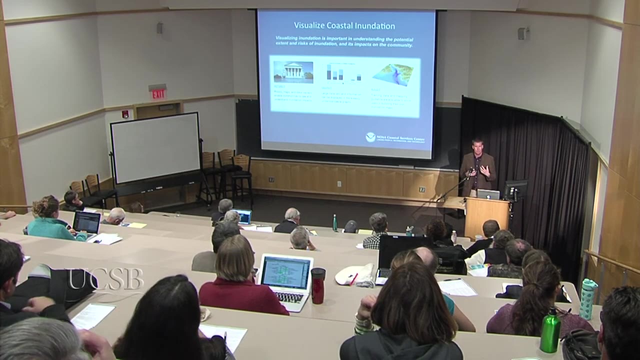 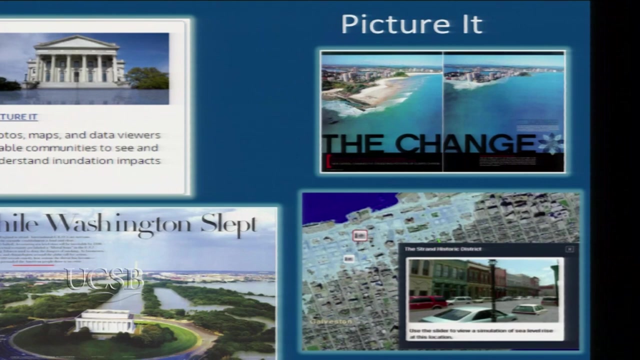 but we have what are called Apply It pages, and this one deals with coastal inundation and it kind of leads you through the process of trying to visualize inundation. So let's start off first with Picture It. Okay, So this brings it down to home for people. 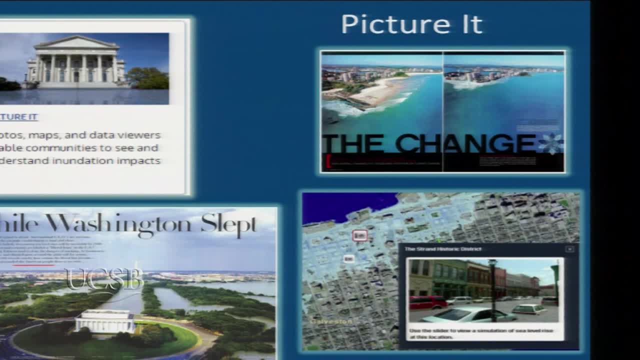 They want to be able to see the impacts at locations that they're familiar with. Okay, Using photos and using maps and using data viewers enables the community to really see their impacts, and it always helps to have it in their community, not just an example from somewhere else. 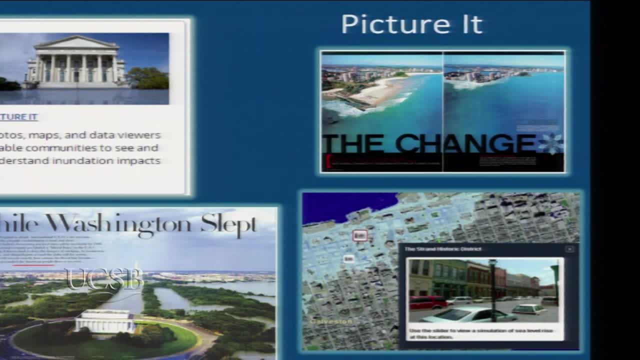 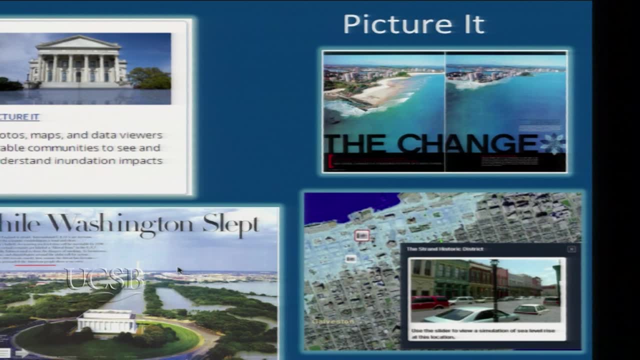 but in actual their community. Some of the things that have been in the literature you know, kind of sensationalize this effect. You can see while Washington slept. this was the Bush administration. This is where it came out. You can see the mall there. 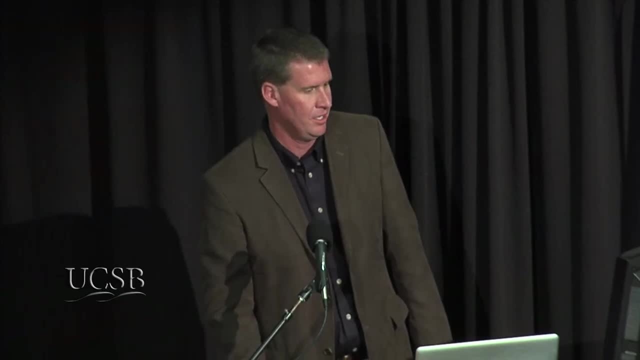 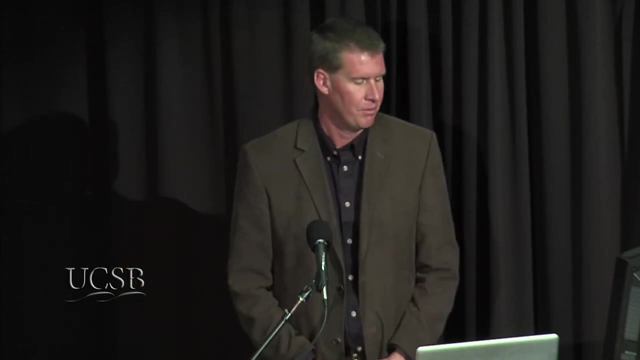 You have simulations of flooding up here. This is one in Australia. I don't know if that's Sydney or if that's Melbourne, but that's showing, you know, the impacts of sea level rise in some of our major cities. And then I'll go into some examples that we have. 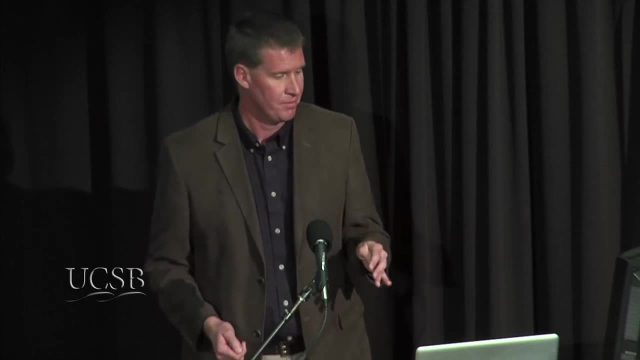 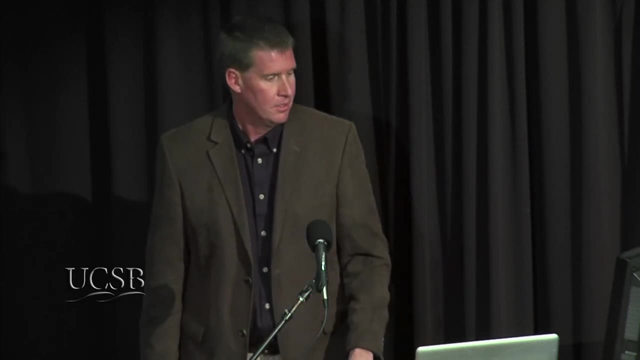 and I'll show you a tool, after I go through some of this, that tries to bring all of these together: the maps, the graphs and the photographs. How many of you have been here? How many of you have been to downtown Charleston? 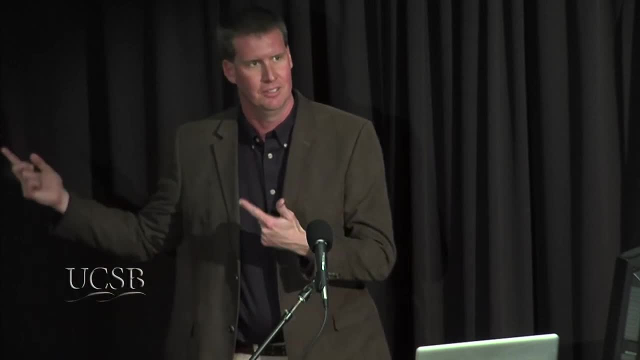 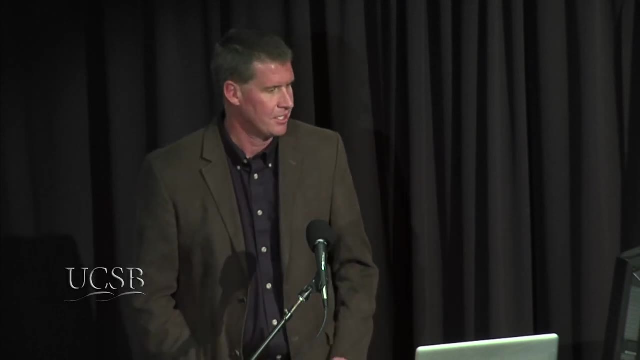 South Carolina You have. Do you recognize this building? This is our customs house. See, this was built back in the late 1800s and actually the initial design was for it to be bigger. They ran out of money. 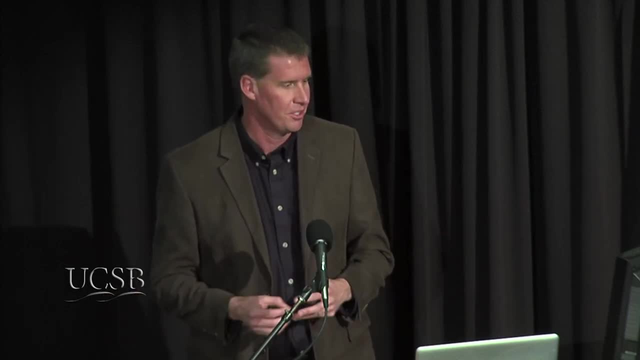 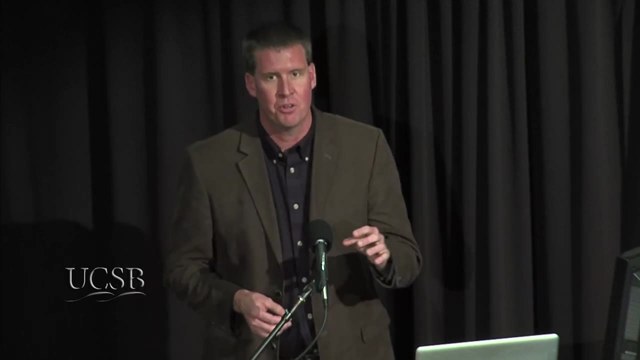 so actually the government stopped back then. The same thing that just happened two years ago: They were going to shut the government down. They actually did back then. so we haven't figured out our problems, obviously, But these guys knew what they were doing. 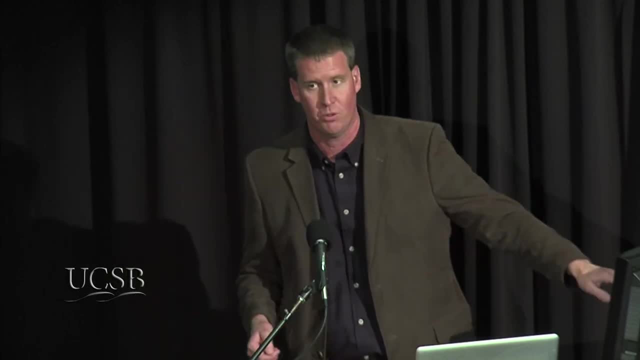 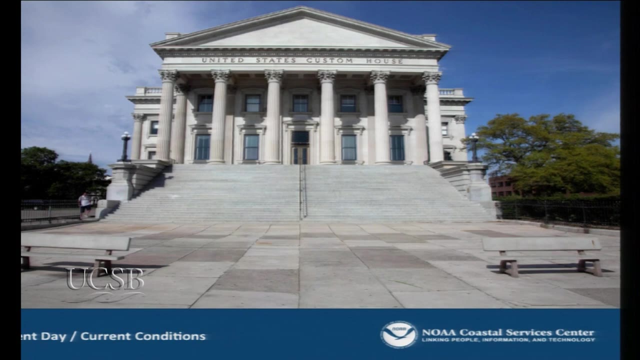 when they built this right, So this is the highest structure. The first floor elevation of this is about the highest first floor elevation we have in Charleston. It's too bad. the rest of the city didn't build to this height, so they're going to be okay. 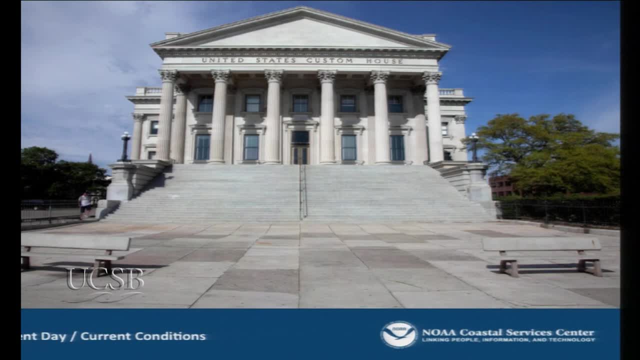 But we can take information like this. We can take a photograph and we can superimpose If we know- for instance, if you've ever been there, there's actually a. does this have a laser pointer on it? Yeah, there we go. 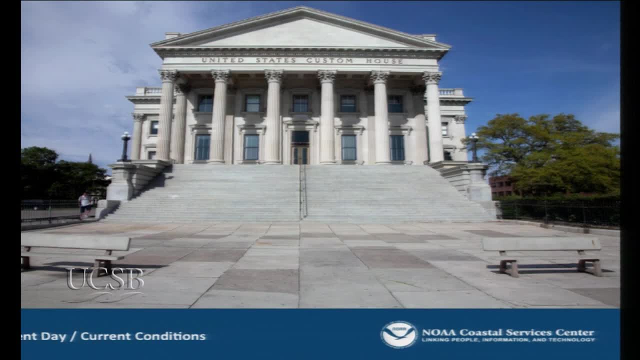 Down in the right-hand corner. if you ever go there, you can check this out. There's actually a geodetic survey marker so we know the actual elevation of that, Those steps, So we can estimate based on water levels. Oops, wrong direction. 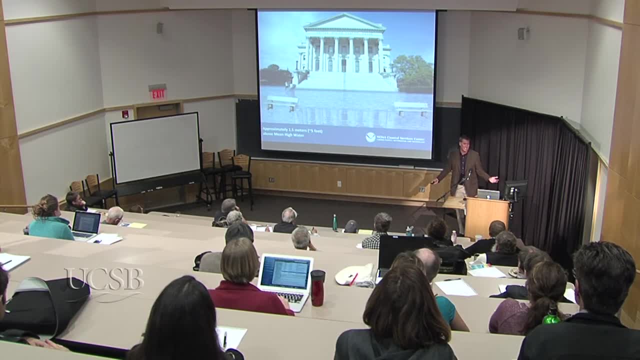 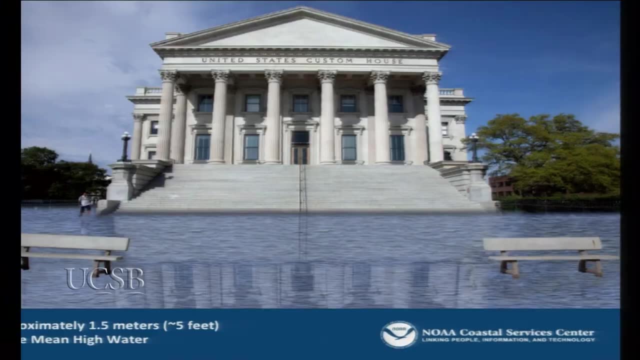 Using some photo scaling techniques. This is, you know, this is easy, right? Oh, it's pretty easy to do that. There's a guy standing here. You can use him for scale. He didn't get out of the way when the water came in. 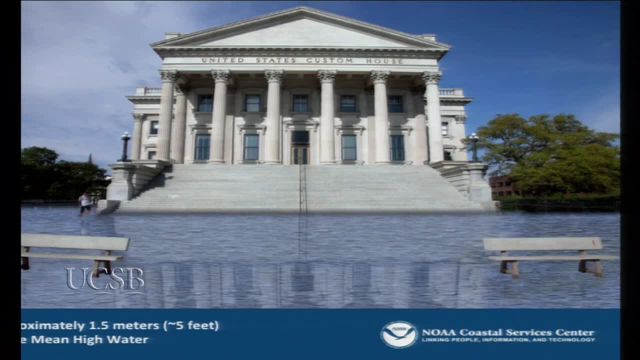 and they didn't move the park benches either. But this is a really neat tool. It's called Canviz. It's something that we make available on our website. It's a platform. It's a partnership with the Agroforestry Center. 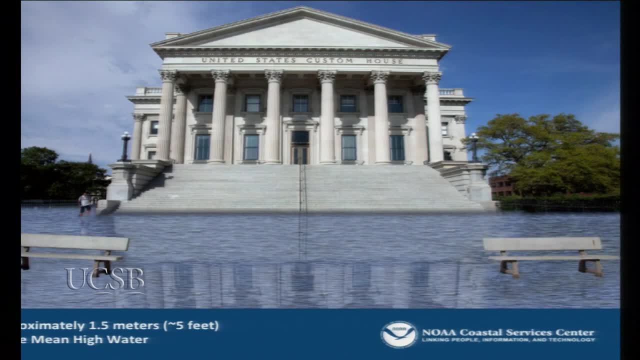 of the US Department of Agriculture, And the tool is- I call it- like Photoshop light. It's very easy to use and you can do these simulations pretty easily. So look it up. It's C-A-N-V-I-S Canviz. 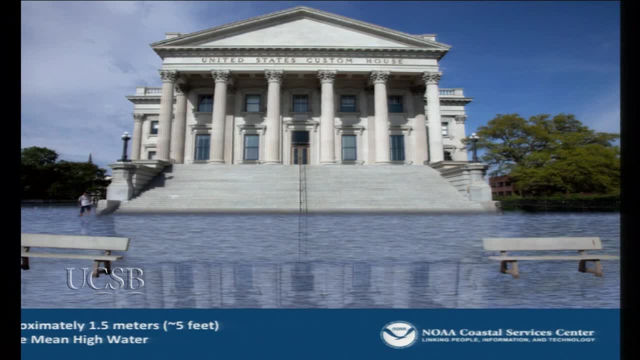 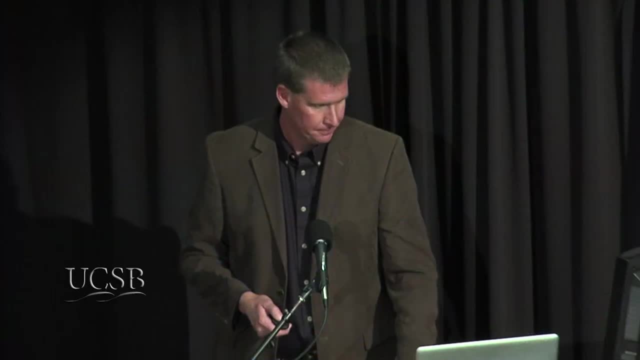 and you can download it So we can do photo simulations like this to show people this is what's going to happen. This is with approximately 1.5 meters of water at that location. So we had photographs. We can also. Scientists love graphs, right. 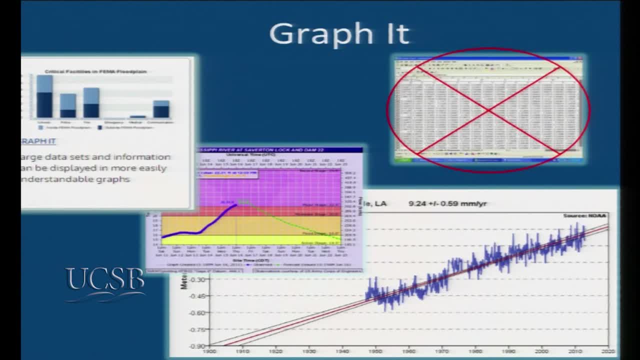 Well, actually, scientists love these Big, long tables of numbers, And this is what we have to deal with with climate data especially. We're going back so far and we have so much data. We can play with our tables all day long. 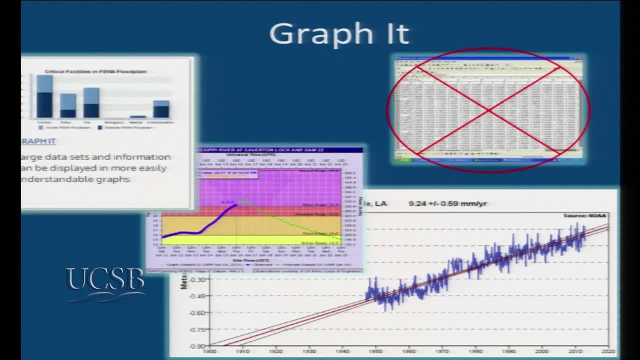 and so what do we try to do? We try to make that information a little bit more user-friendly. so we put it in graphs to show trends. So graphs are very effective at large data sets and information can be easily displayed. Here's a couple examples. 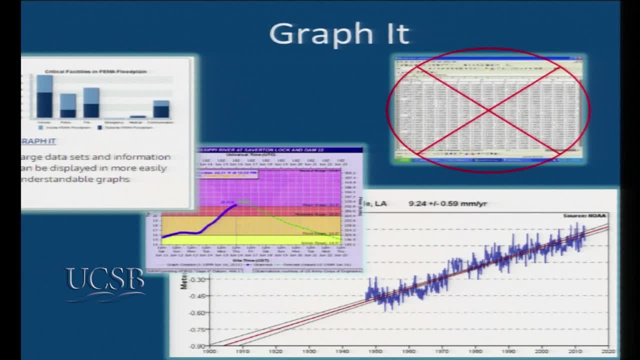 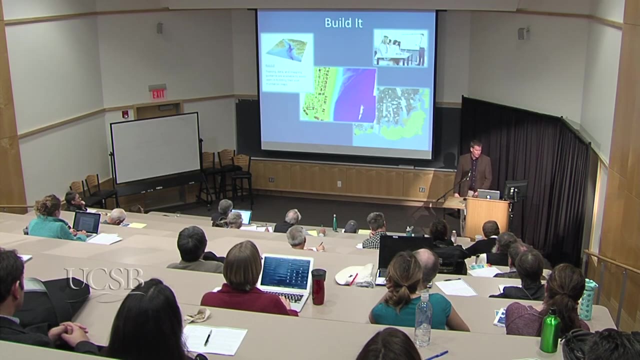 This is a hydrograph from National Weather Service. This shows you the observed river height information, and then here's a forecast. And then there's a lot of these out there for tide-gauge stations. These are sea-level rise trends. Then the other one is to build it. 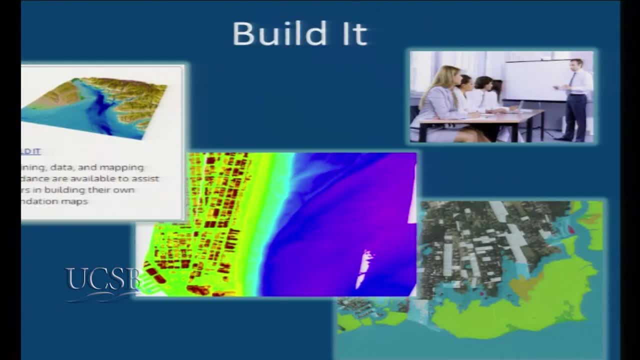 and that's actually getting the data, the base data you need, and doing your own mapping and then training other people how to do it so they can build their own maps. And that requires going out and collecting elevation data- Most of the elevation data that we're collecting now. 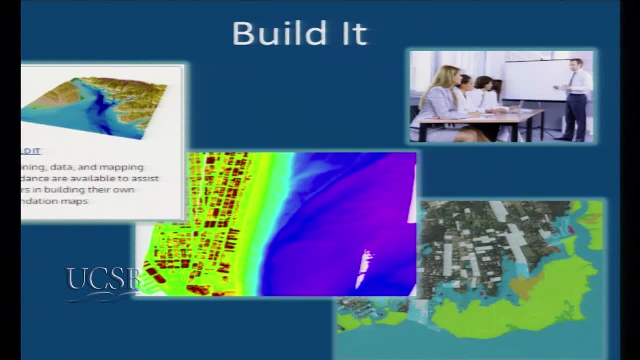 is from airborne-based. it's called LIDAR light detection and ranging and it's actually a laser that's mounted onto a plane and it measures the distance to the ground and, based on the wavelength of the laser, you can determine the elevation. 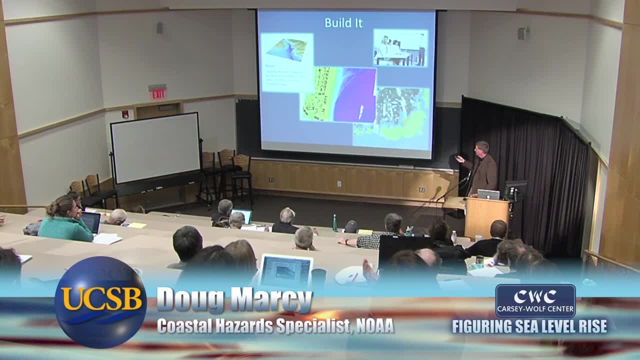 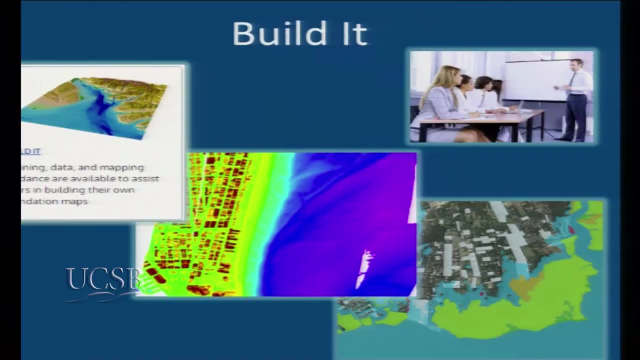 And we use that to build what are called terrain models and we use that to do our mapping, our inundation mapping. So you end up with a map product that you can do some analysis with, And then we actually try to train people how to do this. 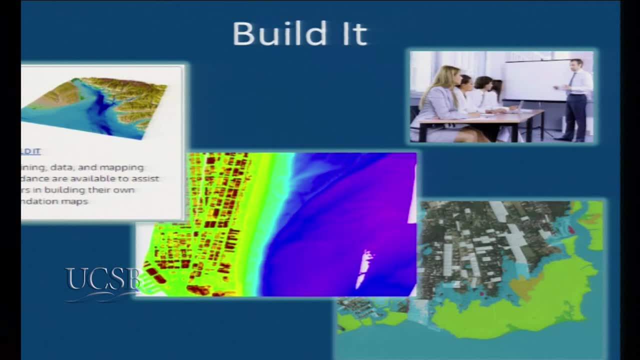 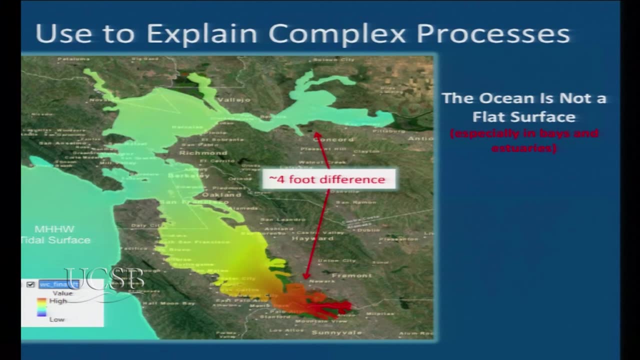 so if they have an issue they want to solve, they can do it themselves, And we want to use the visualizations to try to explain complex processes. This is San Francisco Bay And we use this try to break it down into simple terms. 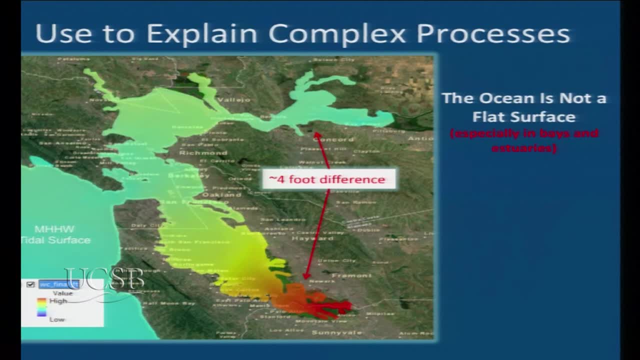 Basically, the ocean is not a flat surface. You go out on a day like today and you look at it: it looks pretty darn flat, But over time- and this is over a course of a month, and you model it- the tide actually has a slope on it. 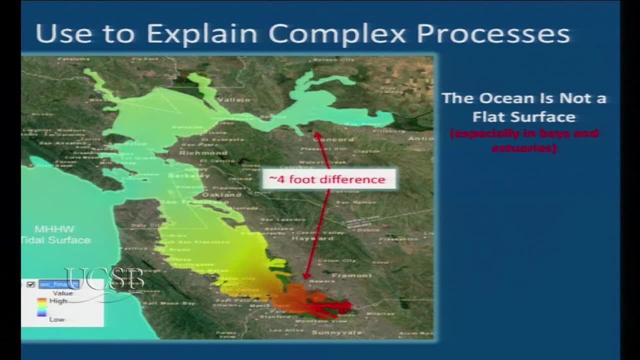 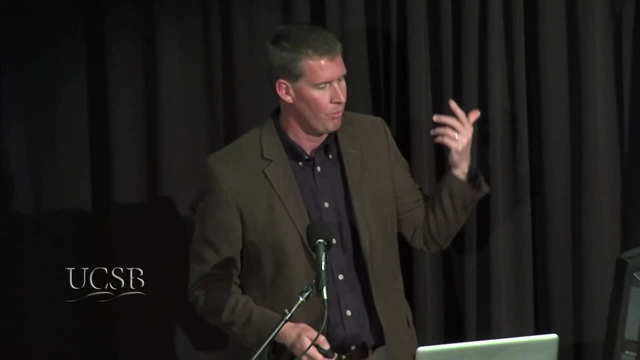 So here, the south part of San Francisco Bay versus the north part, there's an average of a four-foot difference, So you have to take that into account when you do your mapping. So we have models that do all this, but in that, one quick picture. 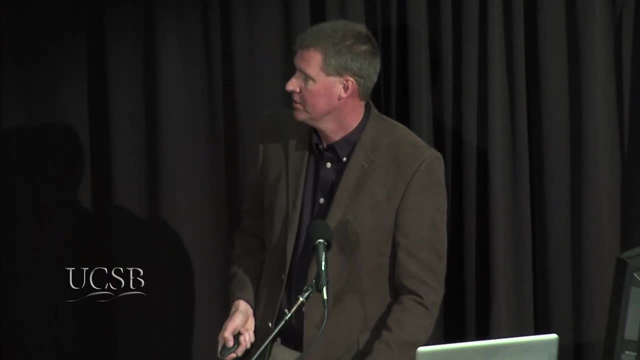 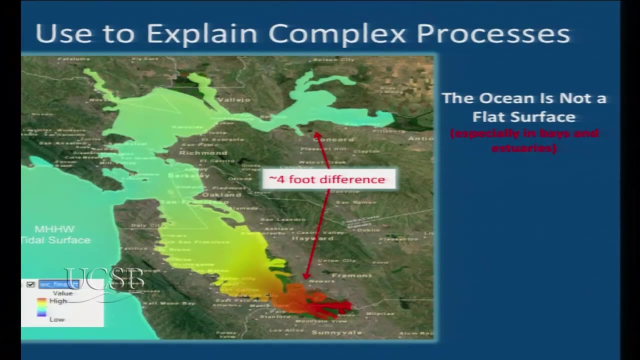 it shows you. yeah, we have a big difference And you can explain that as a complex oceanographic process, but in a picture. very quickly you can make the point And then what you want to do is boil this down and try to get it into. 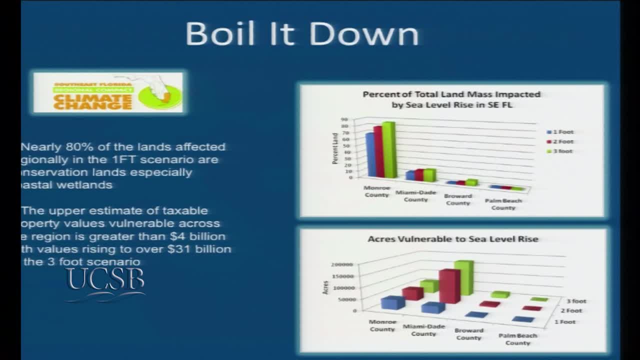 especially for managers. They don't want to know all that stuff. They don't care what data went into it. and then it took you three months to produce this. Usually they ask you: it took you three months to do this. You can't just go. 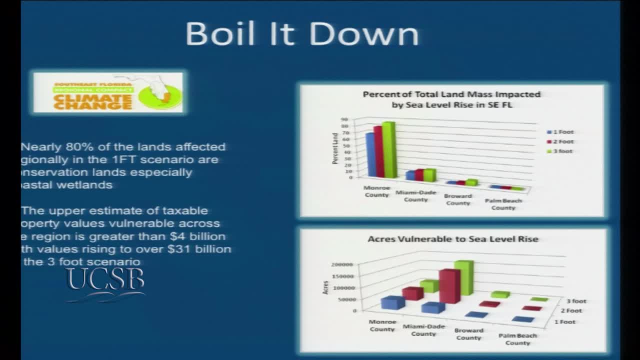 oh, and then they make a change and you're like I can't do that and it's going to take two weeks. But this is an example. In South Florida we worked with Climate Compact there and now it's an initiative called 750.. 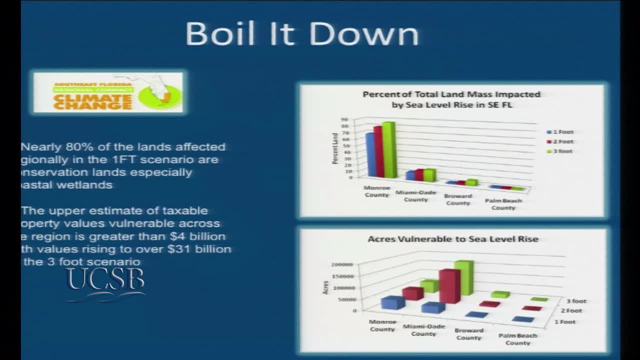 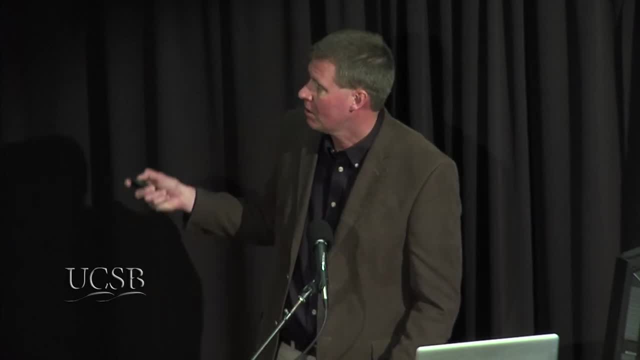 It's seven counties in 50 years. It's a major HUD grant that they received and they're looking at vulnerability, of sea level rise up to three feet- And so they did all this analysis, but they basically boiled it down to some of these simple graphs. 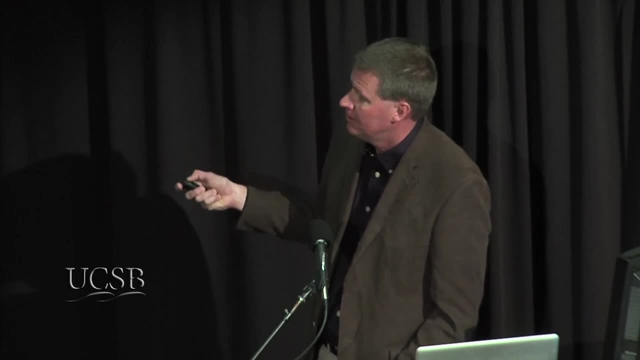 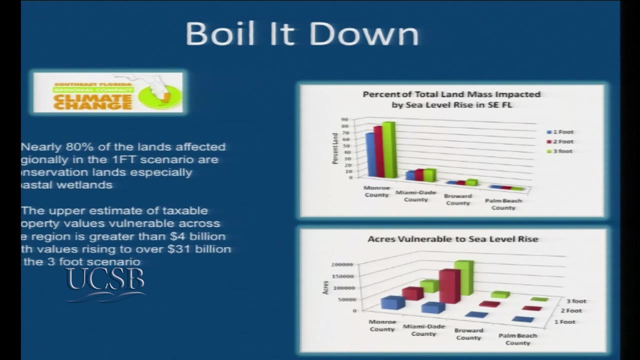 looking at the percent of total land mass impacted, Nearly 80% of the land's affected from a one-foot scenario in South Florida and upper estimate about 4 billion to over 31 billion at the three-foot scenario. So South Florida's in a lot of trouble. 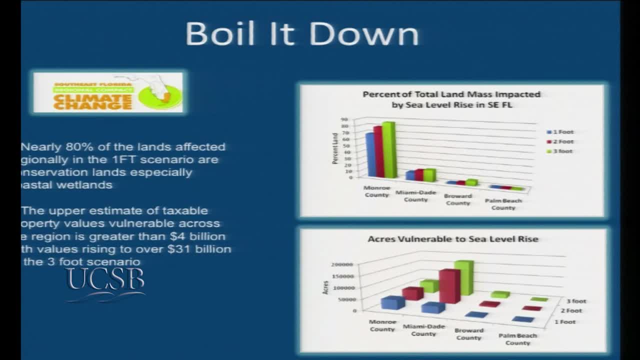 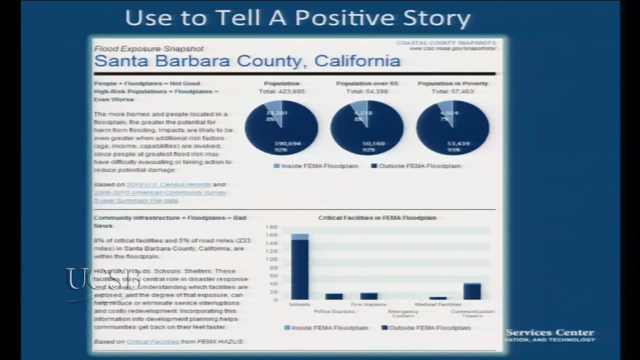 Especially Monroe County, where the keys are. you can see the percent land loss is going to be phenomenal. You can use the data and the graphs to either tell a positive story- and I picked this out for you guys, This is Santa Barbara- We have a tool called the Snapshots. 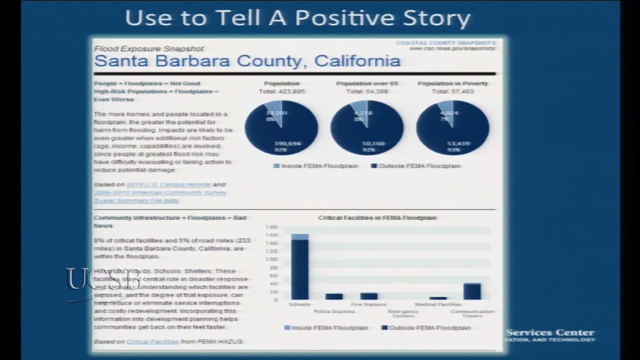 County Snapshots and we can just quickly look at the FEMA National Flood Insurance Program, the floodplains, the 100-year floodplain, and look at how much population lives in that floodplain and then look at some of the vulnerable population. 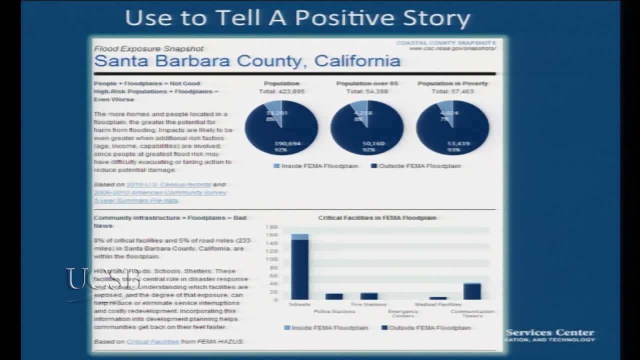 And you see pretty good shape here. This is inside. the floodplain is the light blue. so not that much, not that many people live in the floodplain, because there's not that many floodplains here and not a lot of critical facilities. 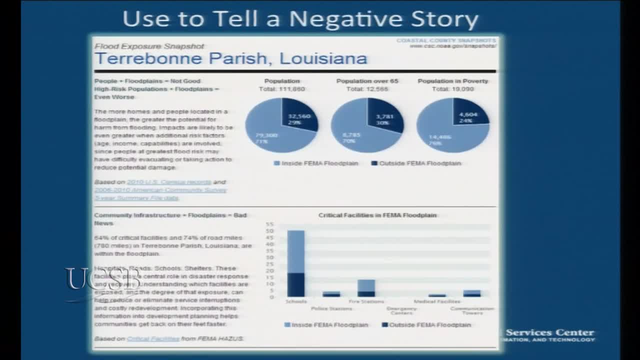 are in the floodplain Or you can use it to tell a negative story. Terrebonne, Parish, Louisiana. A lot more people live in the floodplain, The floodplain's a lot larger and guess what? A lot of the schools, fire stations. 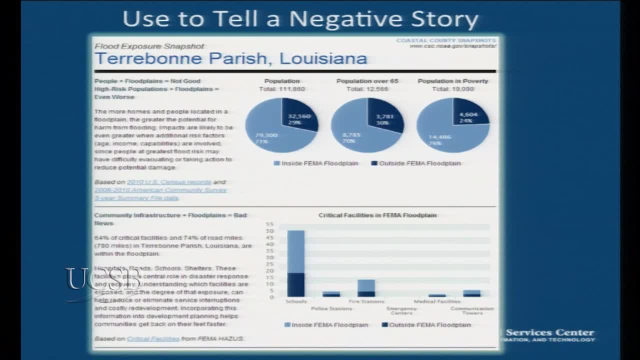 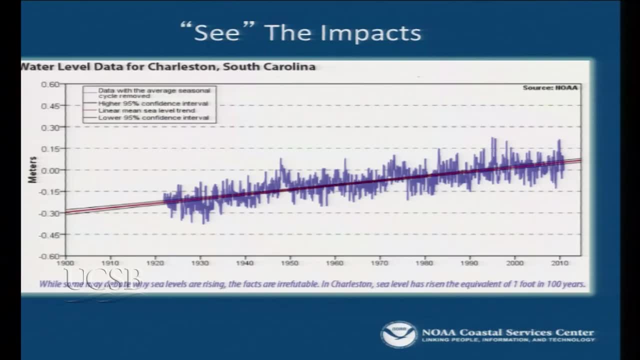 they're in the floodplain. So in a quick two seconds people can figure out the difference. And again, this comes down to being able to see the impacts. You start out with a graph- pretty complicated- and you want to make a point about something like: 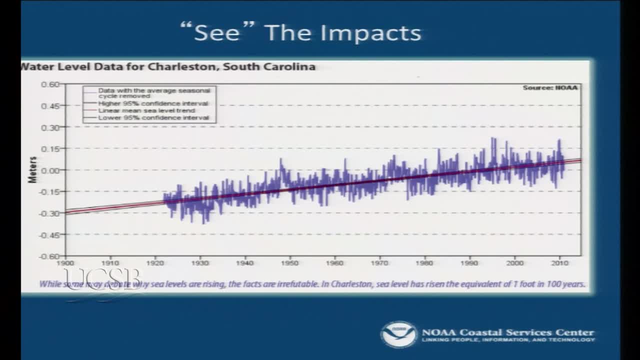 yeah, sea level rise is a big deal in Charleston, South Carolina. okay, I can show someone a graph like this and try to make that case, And then you kind of look at it. okay, what is all the squiggly lines? 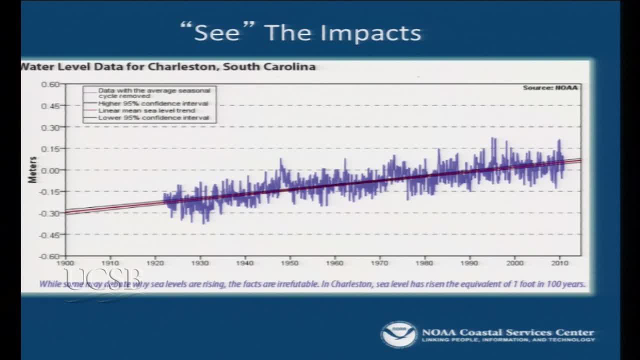 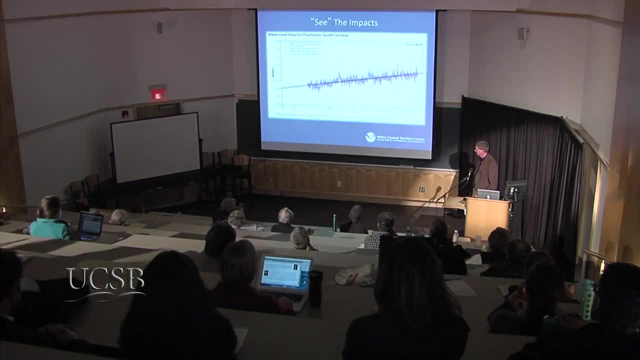 and you got lines doing this and that and then you go: okay, the higher 90% confidence interval it gets. it seems kind of it seems kind of easy to understand, but then when you start getting into it it's hard to explain. 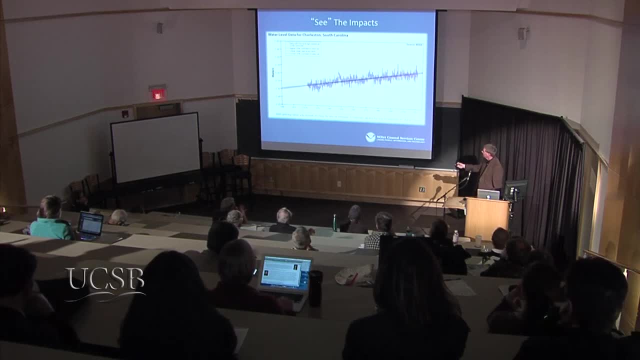 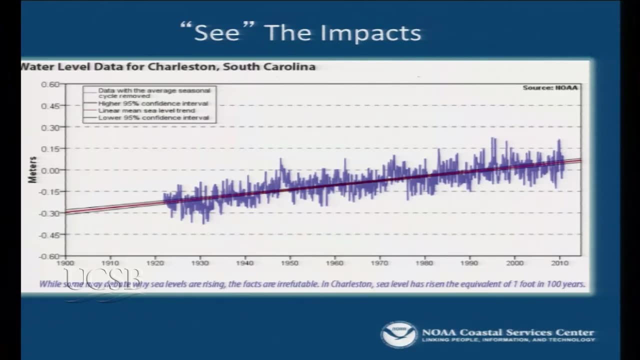 But basically the gist is here. this is observed data, The blue line. it goes up and down and there's seasonal variability, all kinds of difference in the water levels, but the overall trend is sea level has risen a foot the past 100 years in Charleston okay. 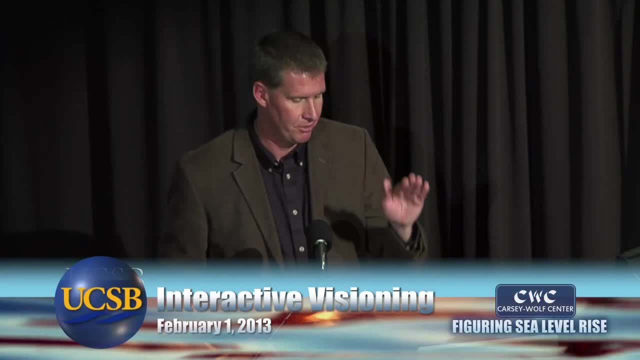 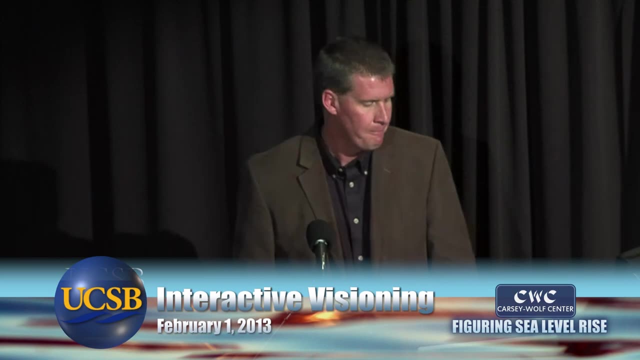 Now, that is relative sea level rise. That means the land is also changing in elevation too, But overall, one foot in 100 years. Well, how else can we tell this story? Okay, well, so we can get elevation data. 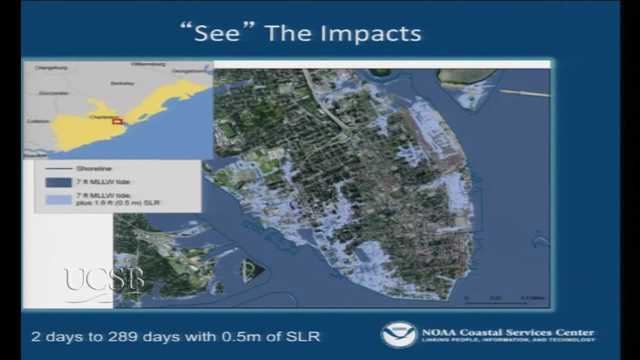 which I talked about earlier, and we can start mapping. okay, And we actually did this. We got in touch with our weather forecast office in Charleston and we said, hey, when you guys issue coastal flood warnings, how do you do that? 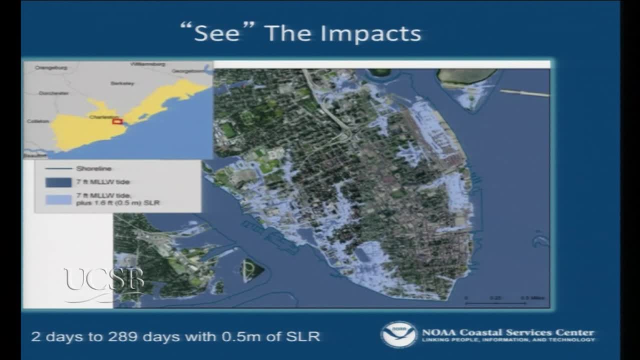 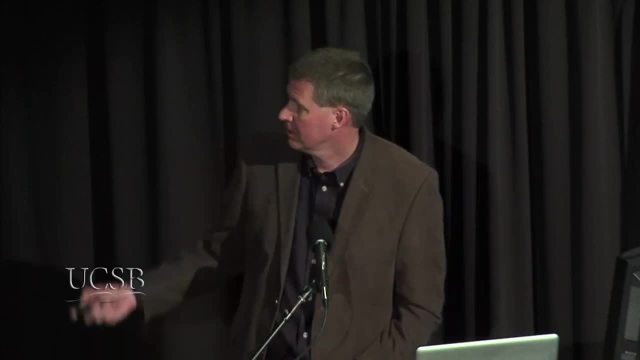 And they said: well, we use a tide gauge and when it gets over a certain threshold, or predicted to go over a certain threshold, we know stuff starts to flood. And it turns out their threshold is seven feet above sea level, because the datum which they use 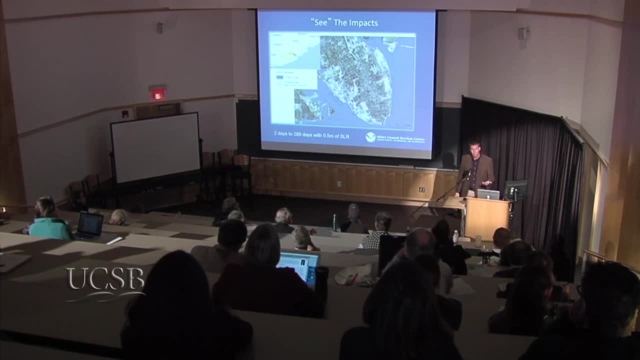 is mean low or low water, So when it gets above seven feet you have a coastal flood warning. So we said, okay, well, let's map that and see what is the impact going to be. and that's the darker blue areas here in Charleston. 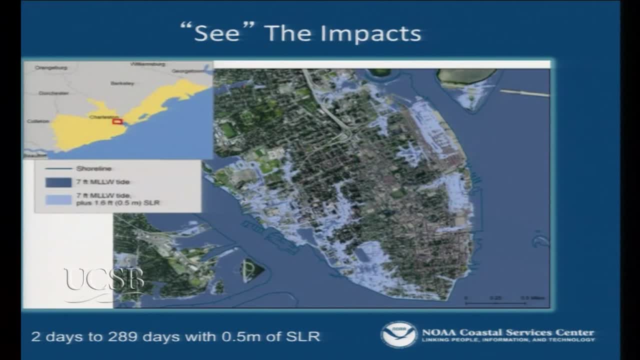 And then we started looking at: okay, well, let's add a half a meter of sea level rise on top of that to see what it might look like, And then we can also go, and we did this back in 2008,. so it's a little older now, but we looked at how many times was the tide, the astronomical tide, the predicted tide, going to go over that threshold, And it turns out back then only two days did it go over seven feet. you know, predicted. This isn't with storm surge and all that, It's just predicted tide. When you raise it half a meter, it starts to happen. 289 days And some days, 66 days. it happens twice a day because we have a semi-diurnal tide. 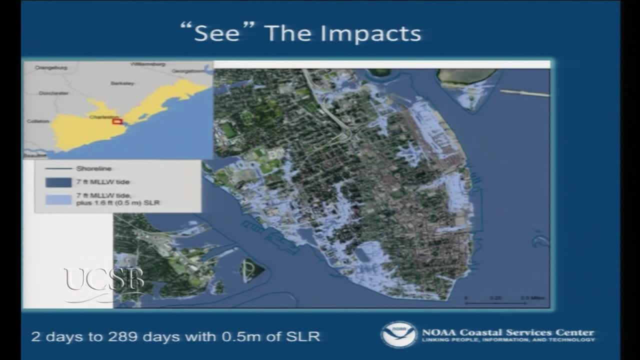 which means we have one high and one, two highs and two lows each day. So that starts to tell the story that these are the areas where we're going to have to start getting, where we're going to flood so often, And I can tell you. 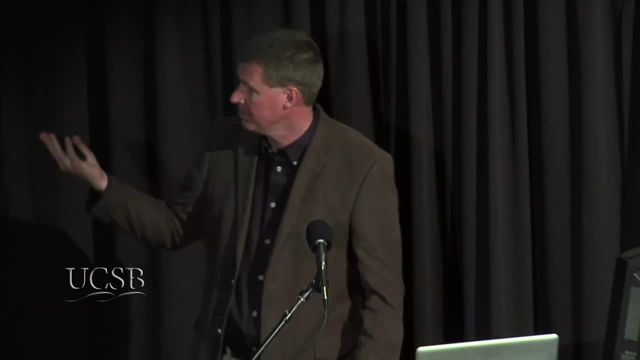 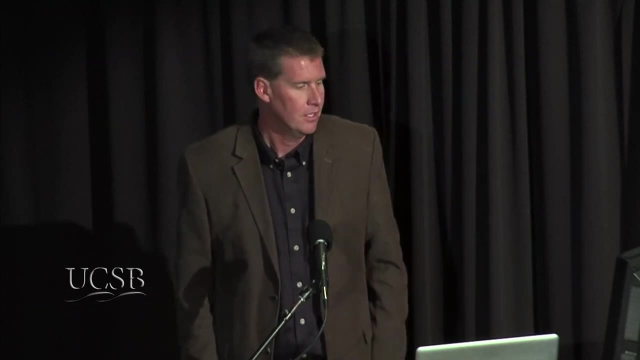 there's places down here, during really high tides, that there's two issues: It starts backing up into the streets and then, when we have excessive rainfall on the same days, we have high tides. the water can't drain, And so it's a real problem. 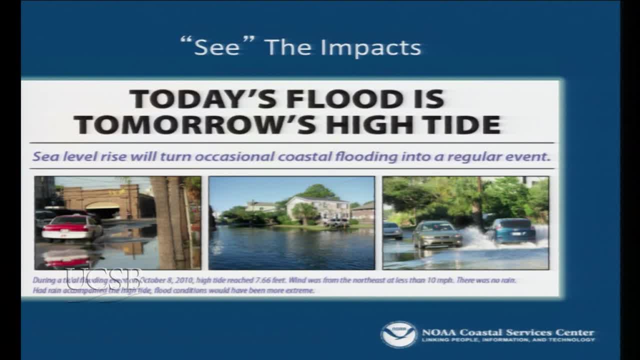 So then we try to coin it to. you know simple phrases like this: Today's flood is going to be tomorrow's high tide. And then you have pictures, actual pictures of the high tide in Charleston to illustrate this. So you've effectively tried to tell. 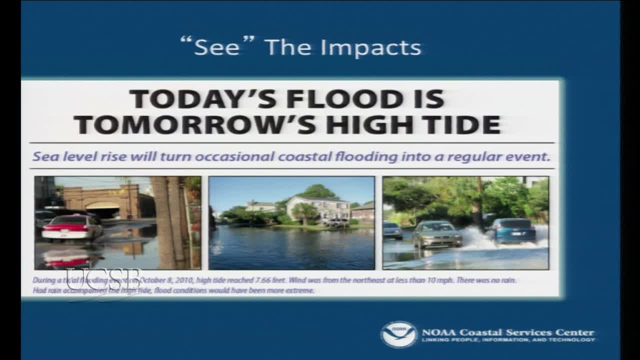 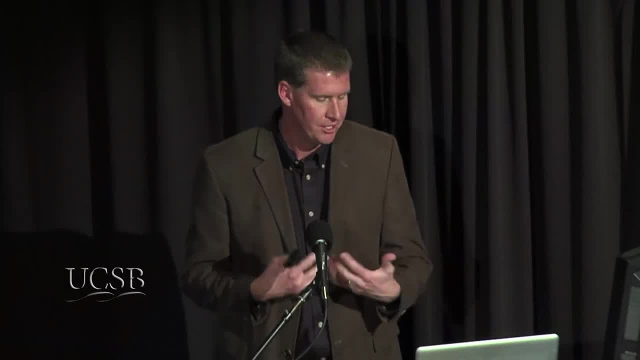 a community that they have a problem. And we actually did this. We took that map and this information to the city of Charleston. They're going through a stormwater revitalization plan, trying to redo their stormwater system, And they know they have a problem. 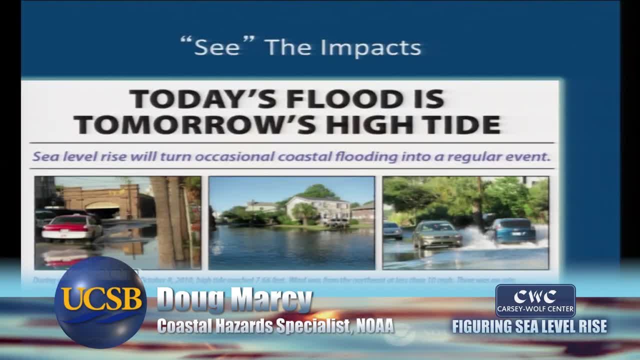 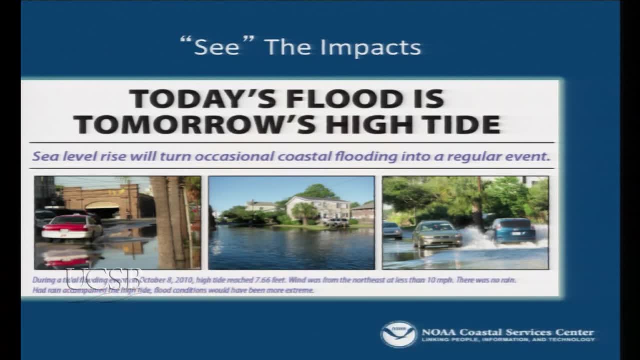 but until they saw the map, yeah, And they were able to verify the places where it does flood and they really saw the issue. It really brought it home to them. So we're going to switch gears a little bit now and get into the sea level rise science. 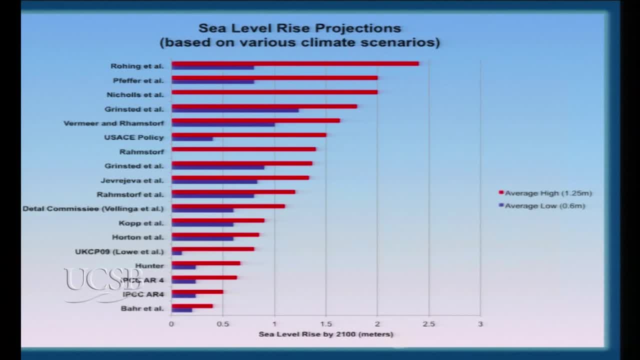 And I don't want to steal Jeremy's thunder too much. He's going to talk a little bit about this, But there's been a major effort going on in this country to try to get a handle on not only climate change in general but also sea level rise. 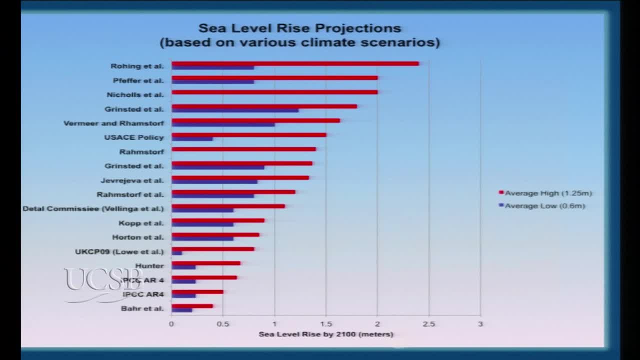 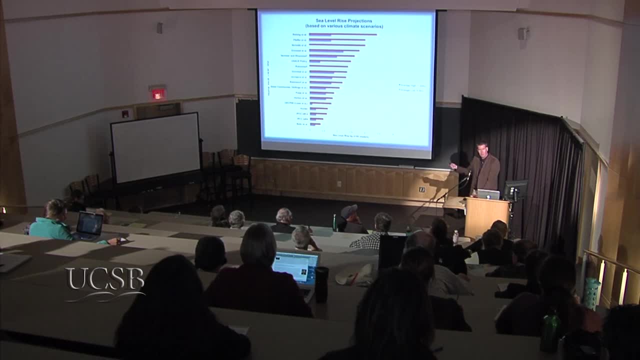 It's called the National Climate Assessment And the results of that report will be coming out. The final, I guess, will be coming out this year. Is it out now? I can't remember The draft's out now. yeah, But it's the same group that actually Jeremy was on. 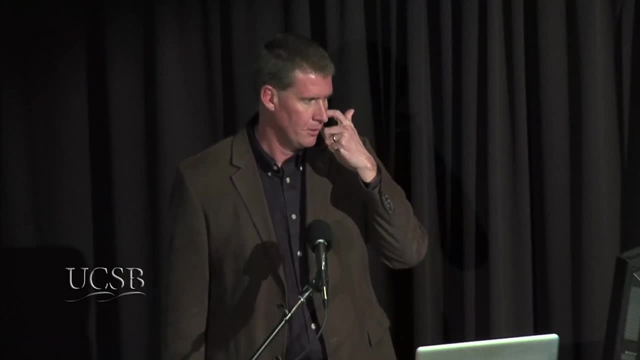 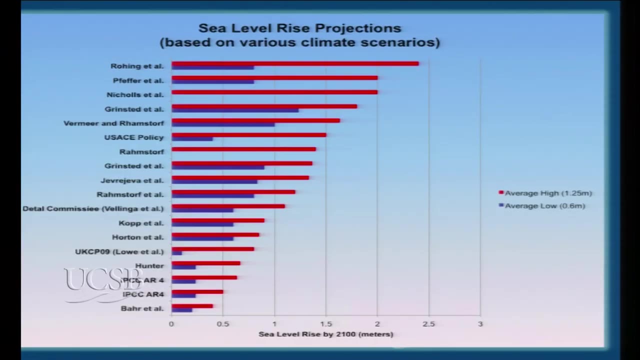 that basically sifted through all the literature on sea level rise projections from various scientists, And what you see here is a graph of a lot of those- I don't know if it's every one of them- And you can see they range all over the place. 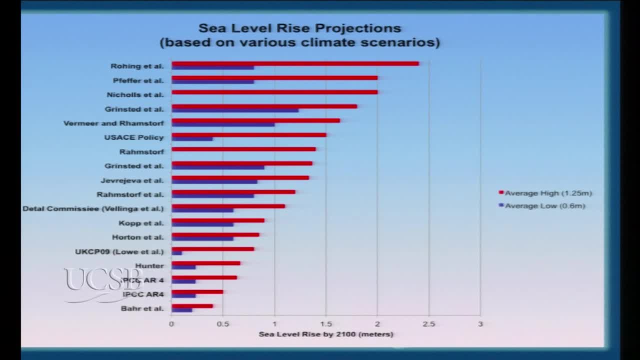 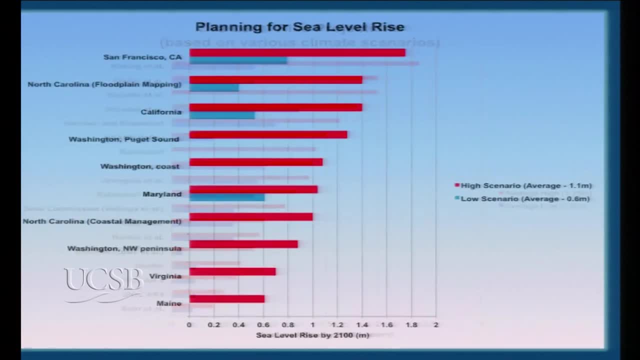 from 2 meters above 2 meters all the way down to 0.5 meters by 2100.. But with an average of about 1.25 on the high side and 0.6 on the low side, And we also kind of 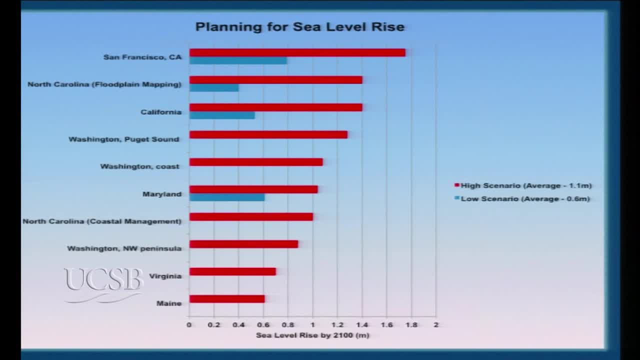 started looking at what are different cities or states doing, And it turns out they're using different ones as well. San Francisco is using some of the higher side, But it does vary. Some are using a low and a high, Some are just using a high. 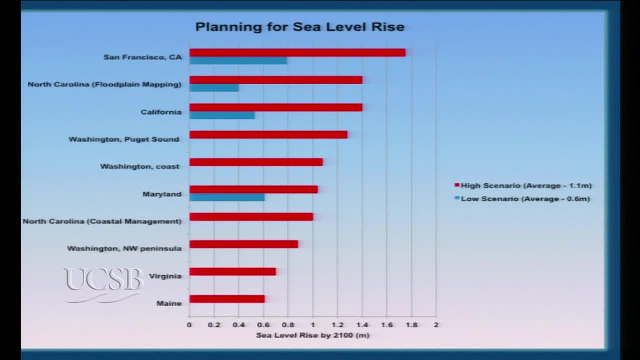 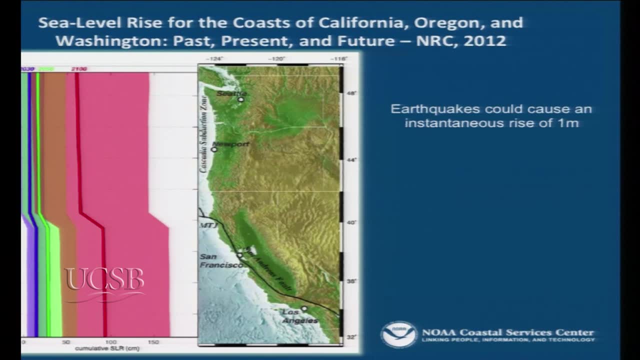 And some aren't doing anything, But again about 1.1 meters, And this was all going on. This is where we were. We were trying to help ourselves and the science community because the public was like: well, there's no consensus on sea level rise. 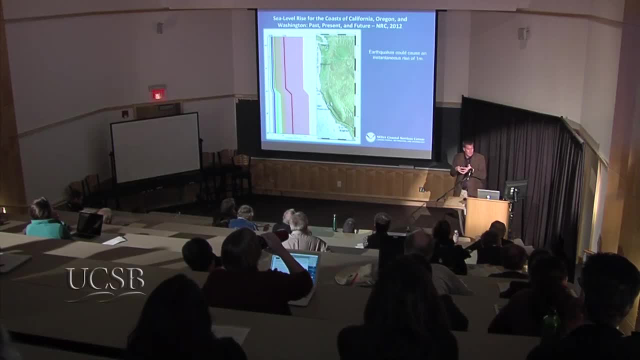 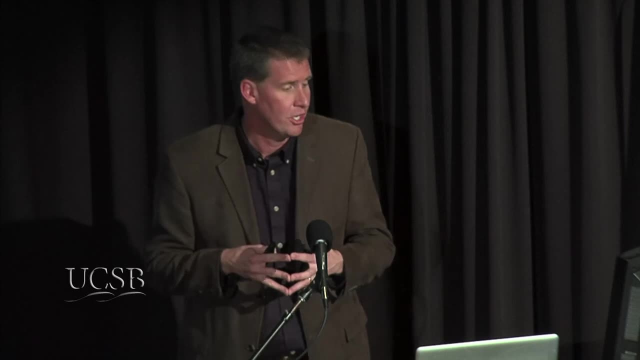 It's all over the place, So we don't know what to believe, But it's actually starting to converge now, And that's what this report that just came out. There's a couple of them. This one is the National Research Council. 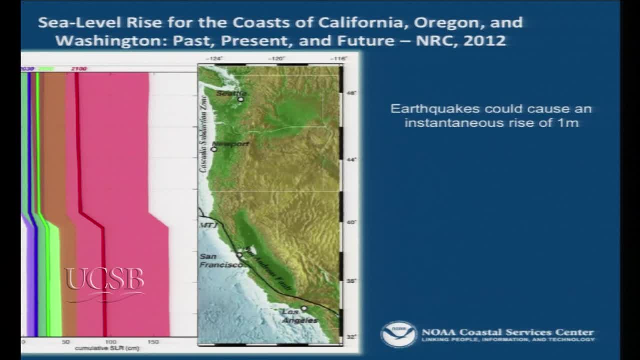 This did this for the West Coast. You can see, this red line is 2100.. So it's about a meter. Here in Southern California it actually jogs a little bit, a little less, But of course earthquakes can cause any kind of sudden uplift. 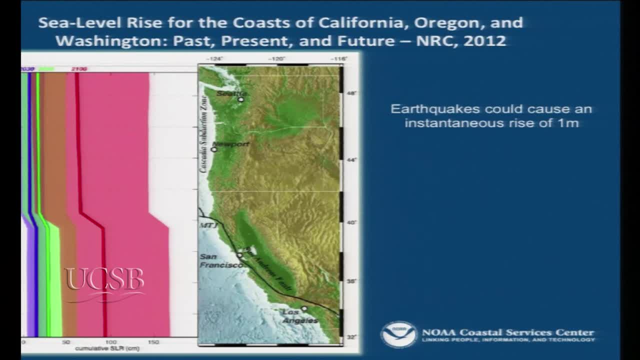 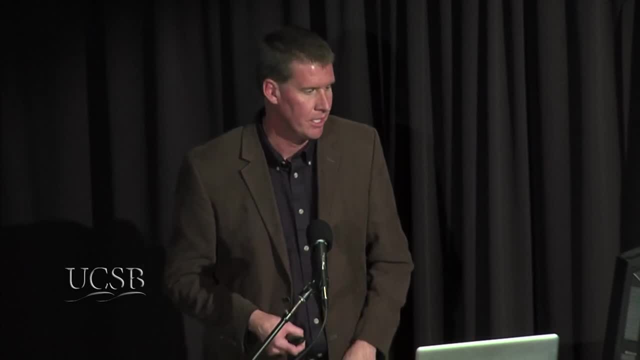 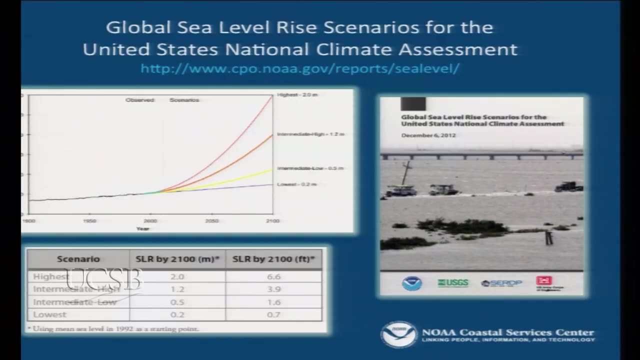 or subsidence could cause instantaneous rise. in some places, Like the earthquake in Alaska, caused up to two or three meters of subsidence and flooded a lot of estuaries there. Now this is the report that kind of pulls it all together And has pretty boldly 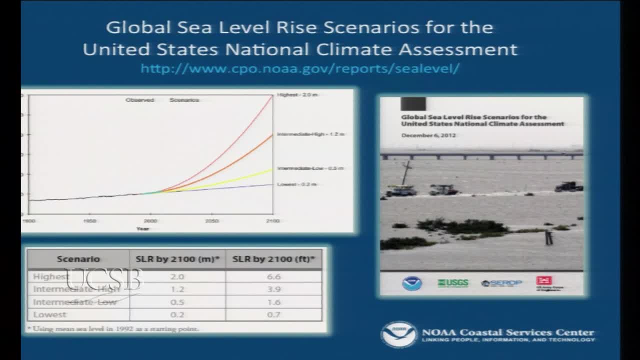 come out with some four scenarios, The highest being- and this is the highest that I've seen so far- 6.6 feet by 2100.. And the way they preface it in the report is by confidence. The lowest is basically just an extrapolation. 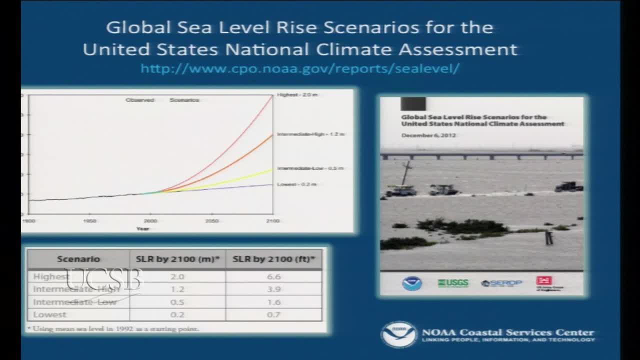 of the existing sea level rise, curve, But they pretty much recommend not using that one because of low confidence. So somewhere in here and it basically tells communities to choose. it's basically a risk tolerance: What risk are you willing to tolerate? And then choose your scenario. 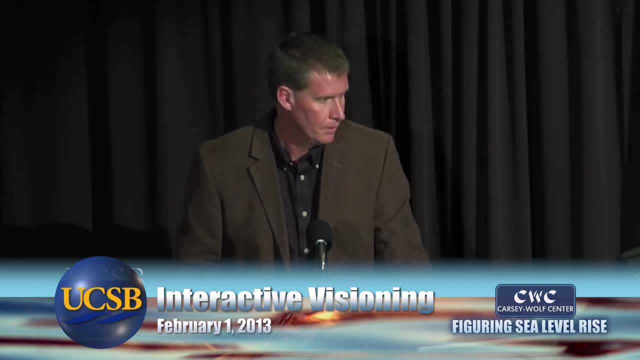 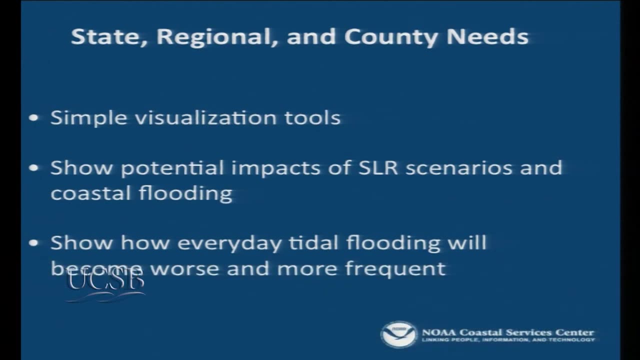 for that tolerance. So we've been working a lot with, and our audience is state and coastal management, coastal resource management community, and what they have been asking us is for simple visualization tools, show potential impacts of these sea level rise scenarios and coastal flooding and also show us how the everyday 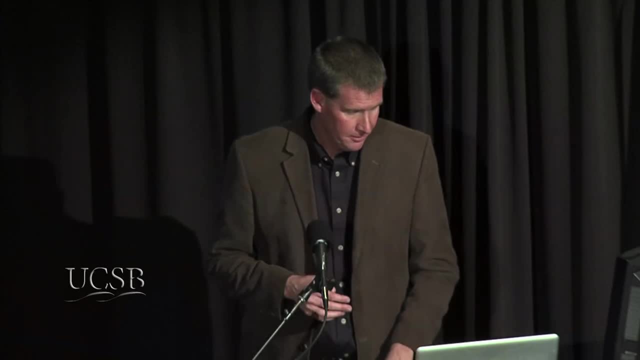 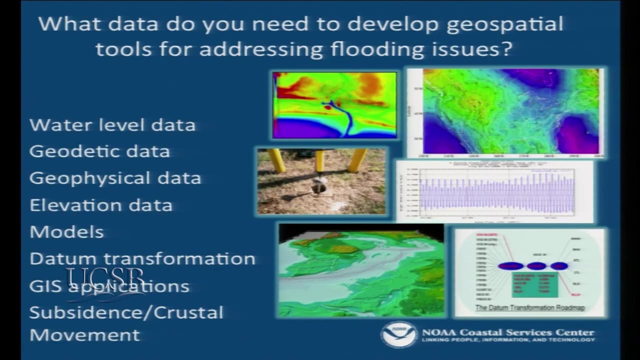 flooding is going to become more frequent and worse. To do that it requires an awful lot of data. The end product, the visualization you'll see when I get to it today, looks pretty easy. it looks pretty simple, and that's the whole point. 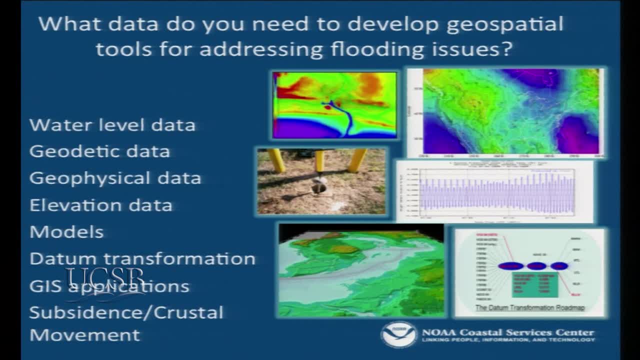 You try to boil it down to that point, but there's an awful lot of work that went into it. You have to have water level data. you have to have geodetic data- that's how high the earth is. you have to have geophysical data like gravity field. 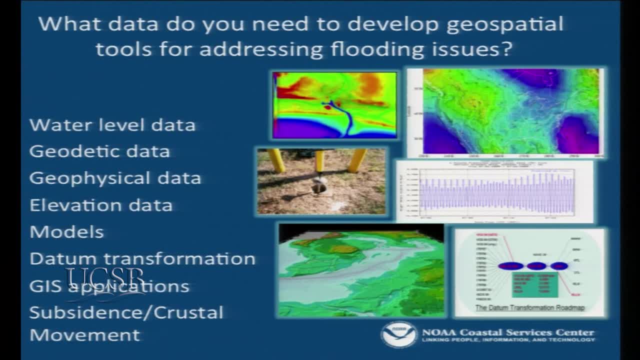 to be able to determine that and model the earth's surface in what they call a geoid. You have to have the elevation data, you have to model the tidal surface, you have to have tools that let you transform from one datum to another. 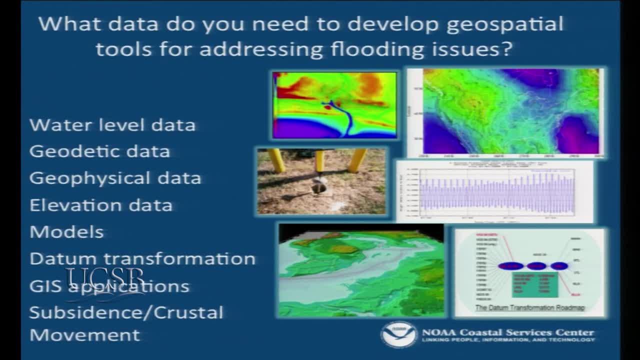 you have to use GIS applications to do a lot of the analysis and also some knowledge of crustal movement if you're going to take into account subsidence. So there's an awful, and you notice, this is not. this is interdisciplinary right. 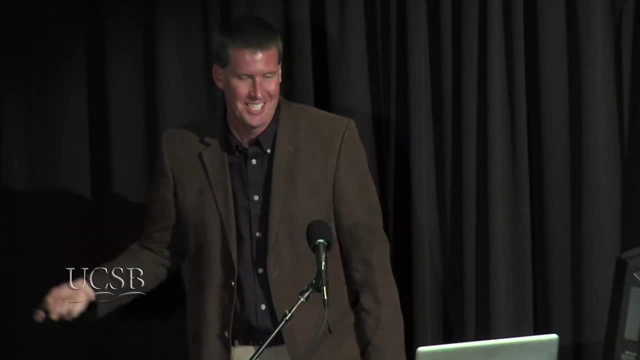 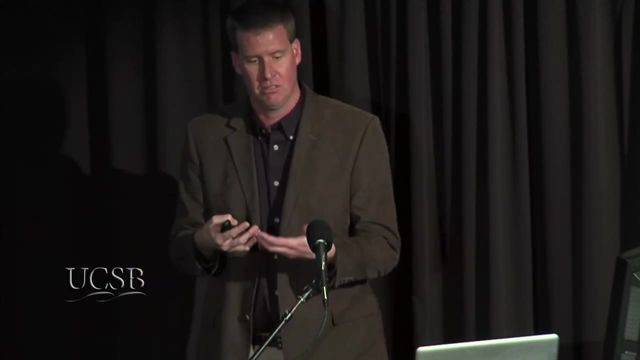 You don't go to college and do all this. You don't. One person's a geodesist and he may be sitting there and he's going to be like, oh, I'm a geoid. It requires you to really get a group of scientists together on this. 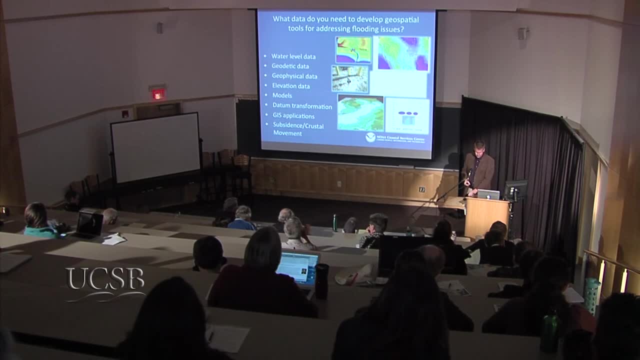 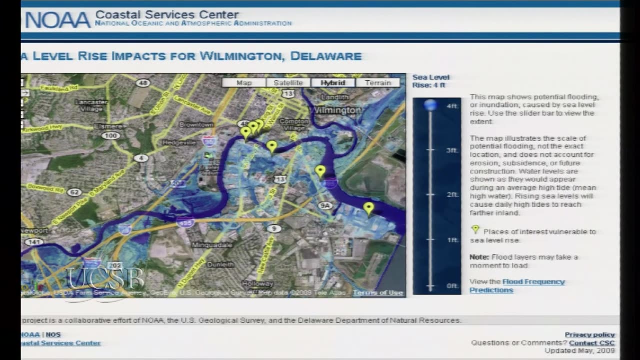 and share data. that's the key is sharing data, because you have to have it all. We started out with some really simple tools. This is one that we worked on with the USGS up in Delaware. This is Wilmington, Delaware. 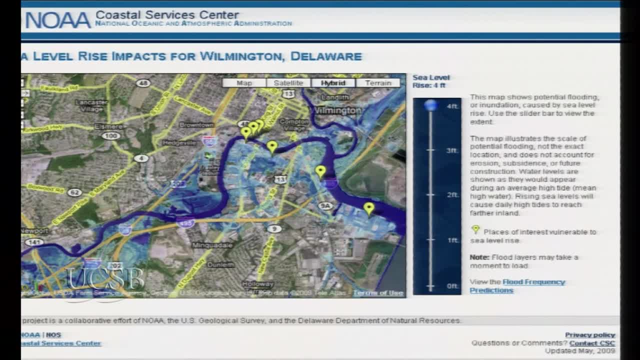 And it was very much okay. let's just map different levels of sea level and have a slider you can go up and down. This is like the infant stages of trying to do something like this on the web Using Google Maps. This was back when Google was becoming very popular. 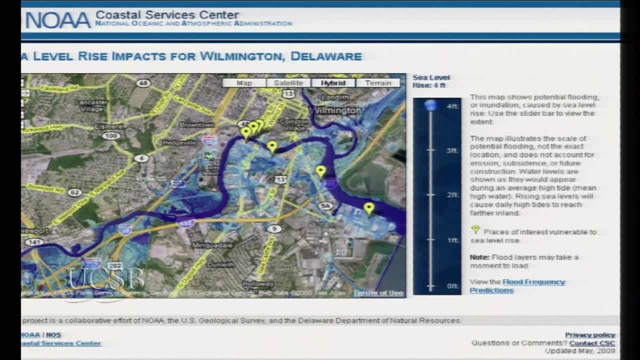 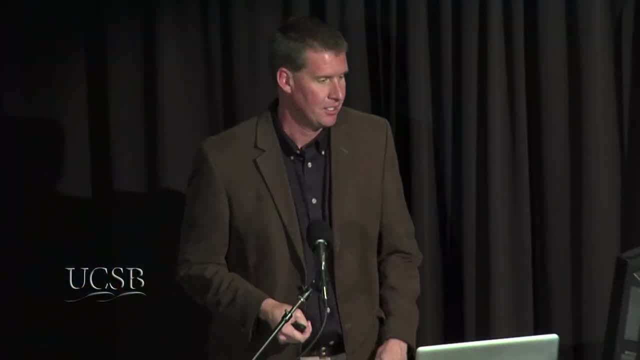 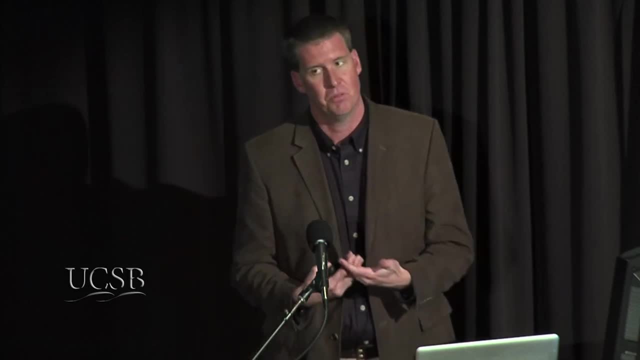 and so the term mashup was born, where you could take a map and stick it on top of Google imagery and it's fast and people can access it. It really made much to companies like ESRI's chagrin. it made GIS very accessible to people. 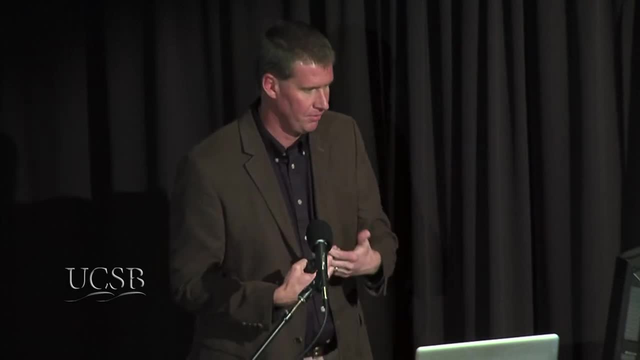 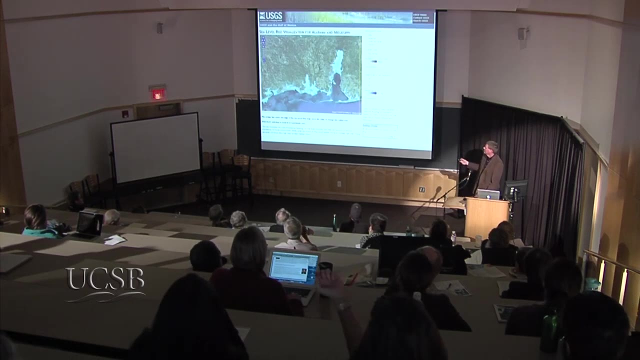 There are caveats with some of the Google stuff as far as the accuracy, but so we were able to take advantage of these types of tools. Then we did another one in the Gulf Coast with the USGS. They actually took the lead on that. 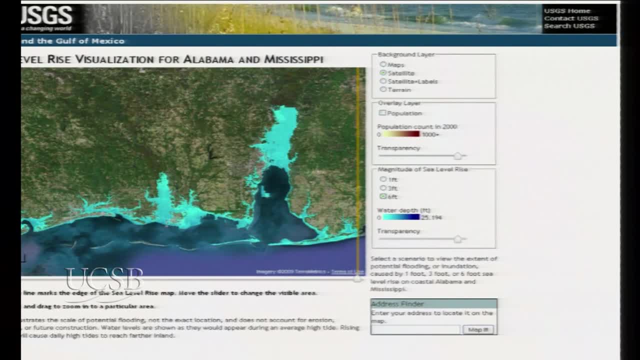 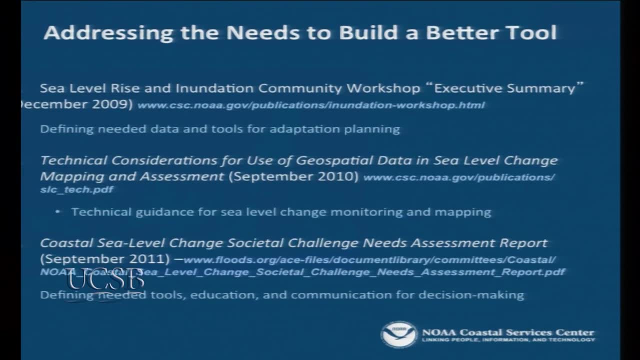 and that was to try to look at different sea level rise scenarios. So we tried- different viewers, different kind of ways of looking at it- And then, back in 2009,, they had what they called an inundation community workshop, and there's a great executive summary out of that. 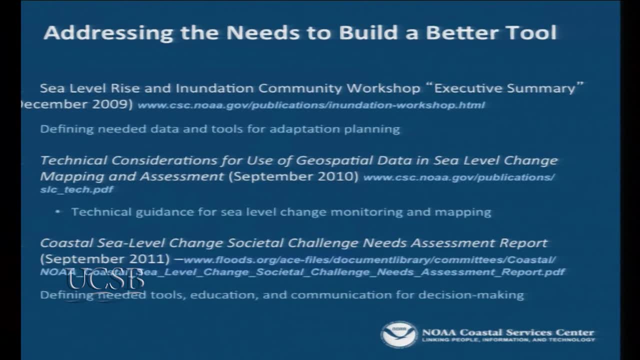 that it brought together about 60 or 65 folks from academics, non-profits and government together to try to figure out what the data needed and what are the tools needed for doing this adaptation planning that we were striving to do, And out of that came a lot of recommendations. 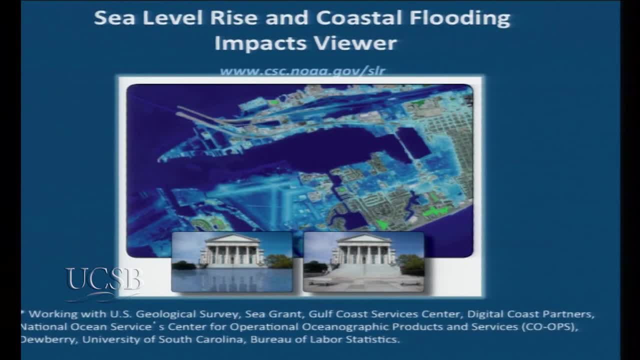 we tried to use to build a better mousetrap, which is essentially what we're doing, And so I'm going to give you some examples of this tool we call the Sea Level Rise and Coastal Flooding Impacts Viewer. There's a whole host of partners. 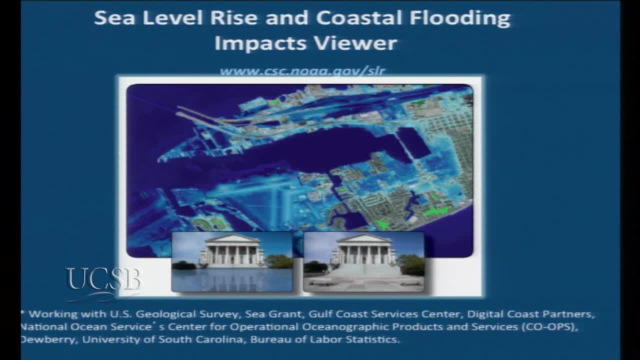 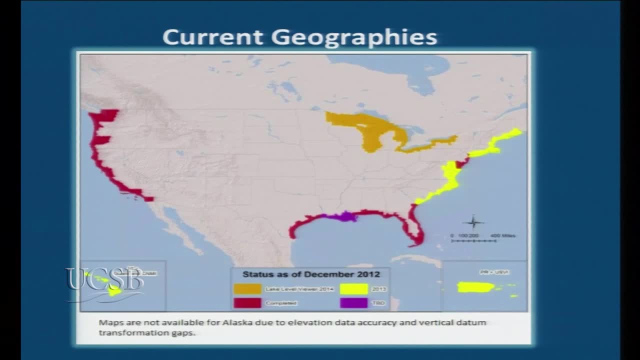 we've worked on with this tool. I'm not going to mention them all there. This is where it's currently available. so you can see we have the West Coast mapped now and we have most of the Gulf of Mexico. We're having some issues. 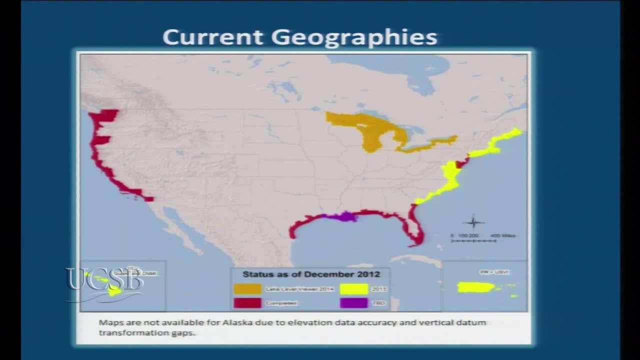 in Louisiana. as you might imagine, That's a very complicated state. There's a lot of levee systems there. We don't necessarily have the levee height information we need and the elevation data there is pretty old. The state collected LIDAR back in 2001. 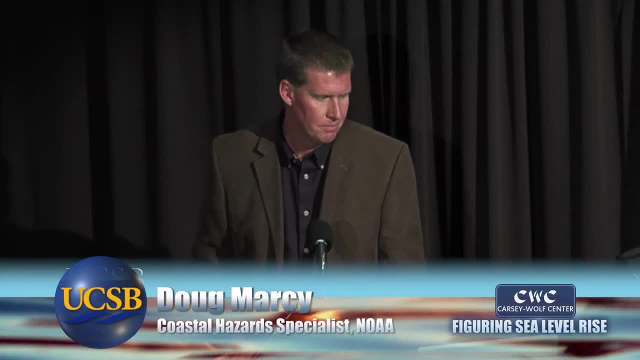 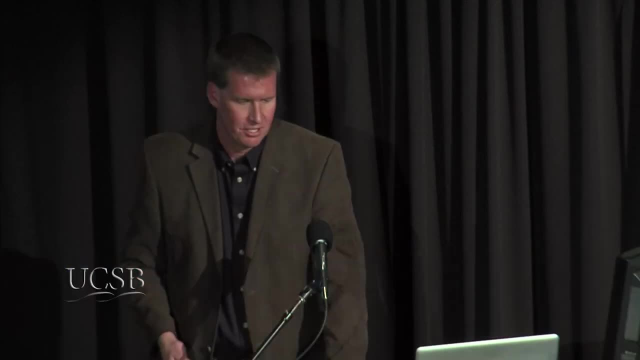 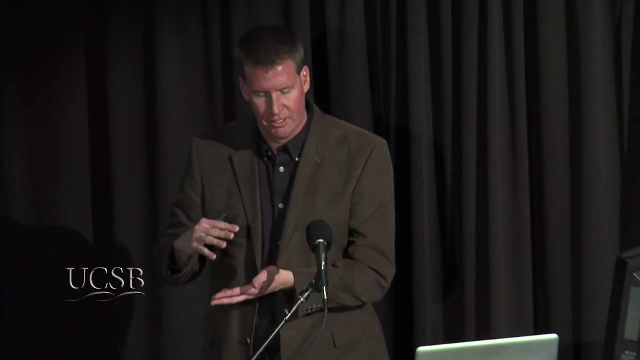 but it's not the quality. you really need to do sea level rise mapping. The scientists argue over inches sometimes of sea level rise and when it gets down to it, when we go into the mapping world, the elevation data that we're using really only has an accuracy. 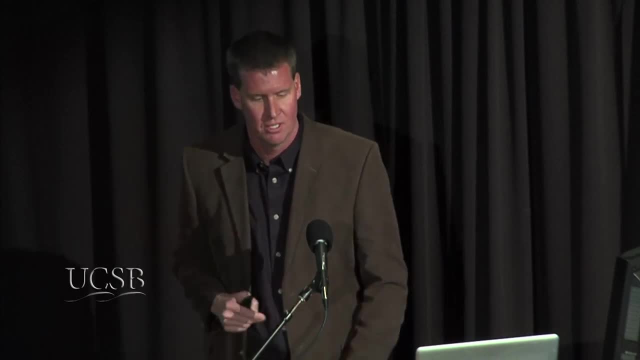 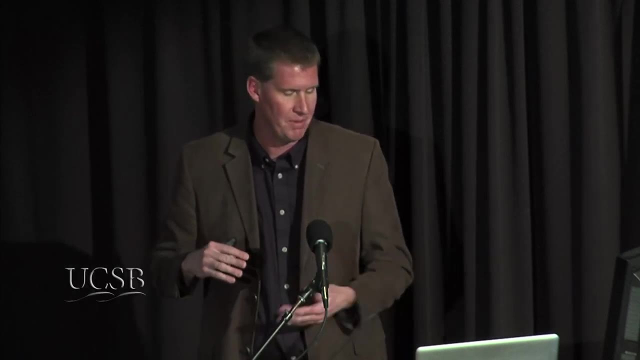 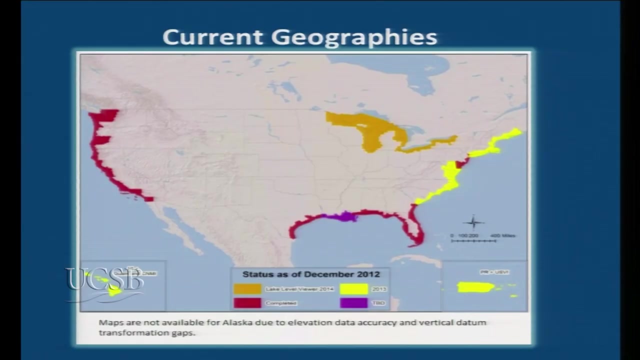 to let us do one foot increments for the most part. So we can argue all day long about inches, but really what it boils down to when we do mapping, it's all lost in the noise of the elevation data sometimes, so it's not an issue. 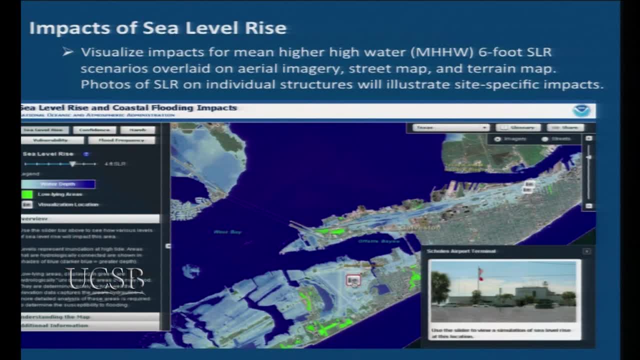 It's an important part of that. So I'd like to try to take you through a series of screen grabs to try to visualize what this tool does, and I invite you to go check it out after the show today, so to speak, The first thing it does. 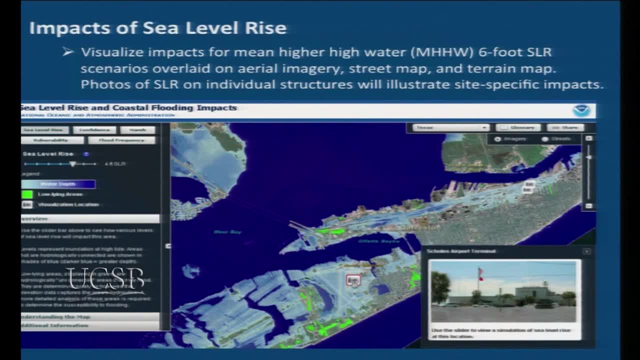 when you come into the tool, it lets you visualize the impacts of water level rise. It could be coastal flooding, it could be sea level and you have a slider bar that lets you go up and down. Now, we're not tying this to any one of those curves. 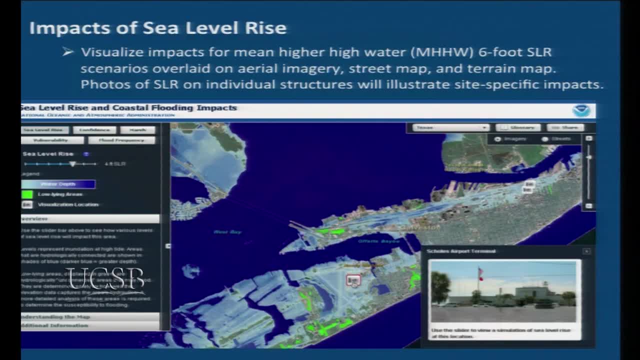 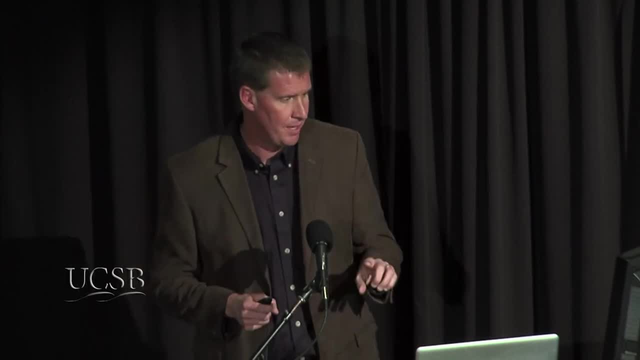 we let the user decide that. We let the user pick: by 2050 I want to look at three feet or I want to look at two feet, and you can go do that In the future. we might be trying to tie it to this NOAA report. 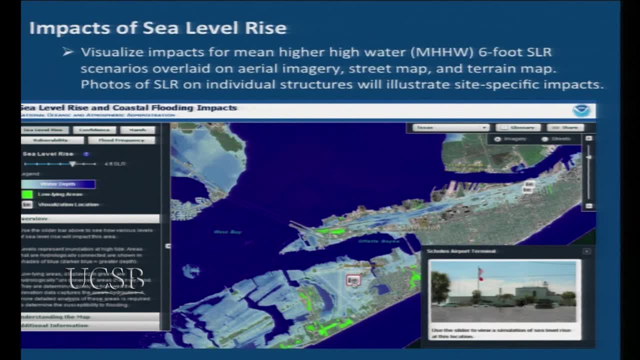 but right now it's not doing that- And then you can click on these locations here. this is Galveston, Texas. in case you didn't know, there's a big seawall that runs right along here, So you go to one of these locations. 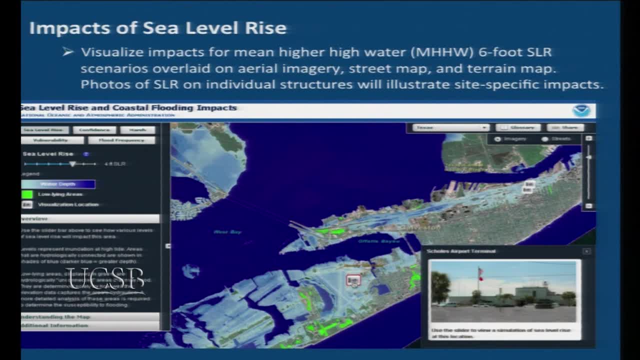 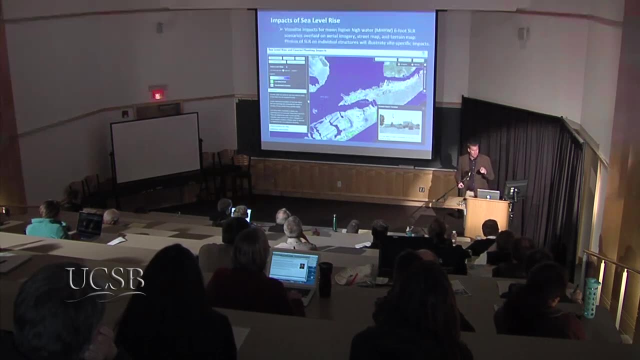 and it pulls up a picture and as you slide this, the water level goes up and down. on this it's interactive, So we know the elevation data at this location and we can determine what the water looks like using that Canvas software. So again it's trying to pull in. 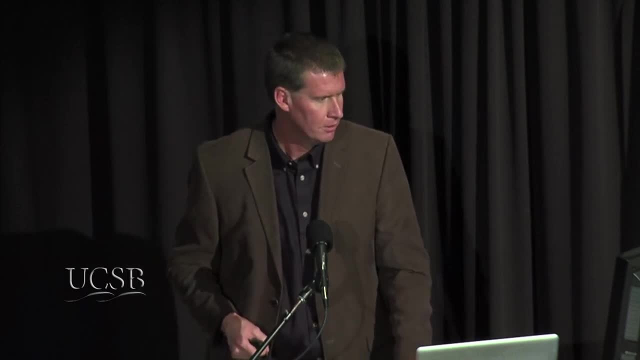 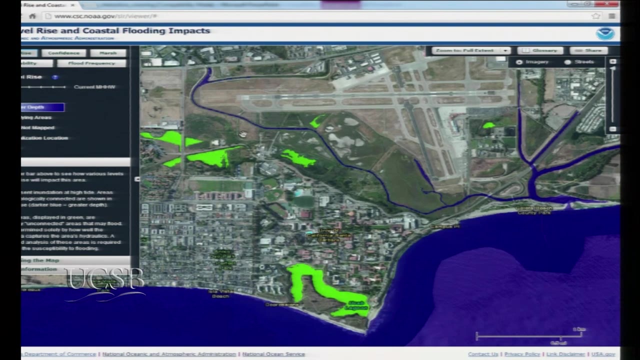 the different pieces of map and a photograph to show people a location and say, hey, I know that airport and I know that's going to be a problem. So I took a map and I was telling Janet, I kind of flew in and I was looking out the window. 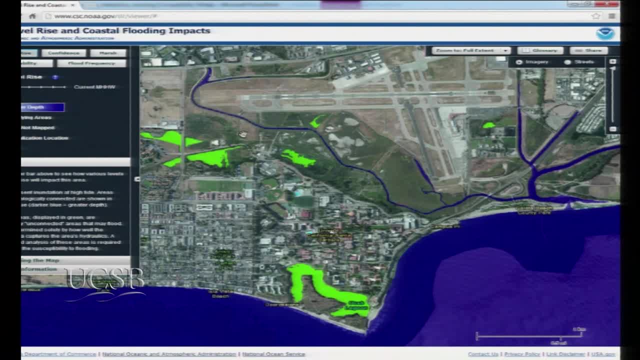 and sort of the high side over here and I know this area is vulnerable. then I was like, wow, did I mess up the mapping? And then I looked and the plane turned and I saw the estuary right there and I was like, oh, okay, So I want to start out. 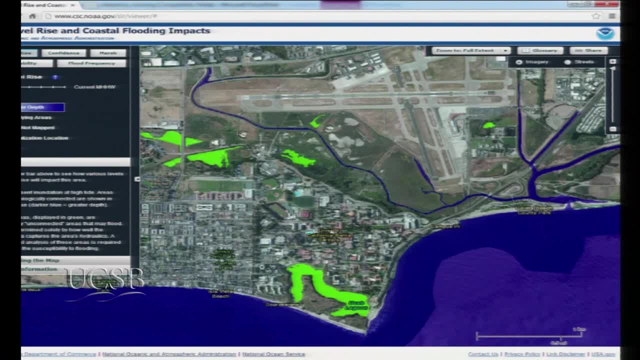 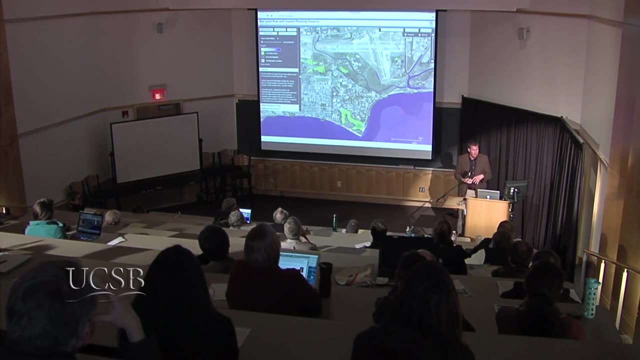 this is at mean high, high water, and you'll notice the green. this is the blue areas that currently would have water, and this all comes down to how you present information too. there's two schools of thought when you start doing mapping. there's these unconnected areas. 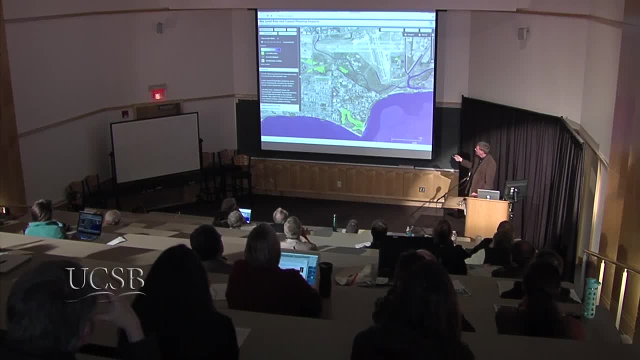 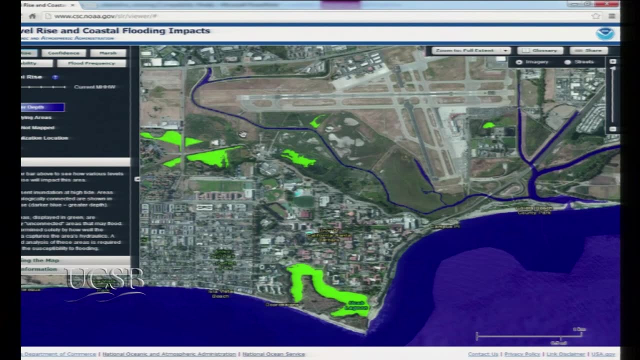 when you start doing inundation mapping. and what do you do? Do you leave them in? Do you take them out? If you leave them in, people will say, well, that doesn't flood, that's not connected to the ocean, it doesn't flood. So we decided to color them differently. 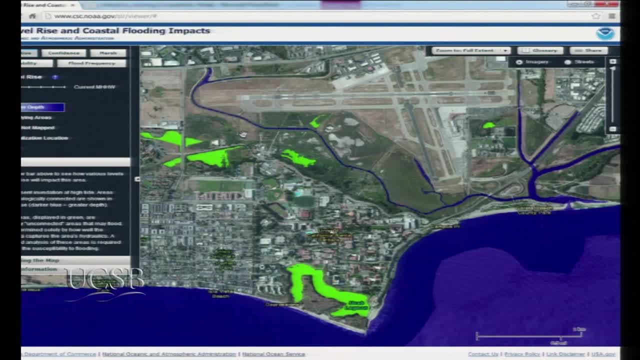 and we call them green in this case because it's a system or a pipe system. so it's better to show it as an area of interest than to leave it out and the lagoon you guys have here. we were just down there looking at it today. 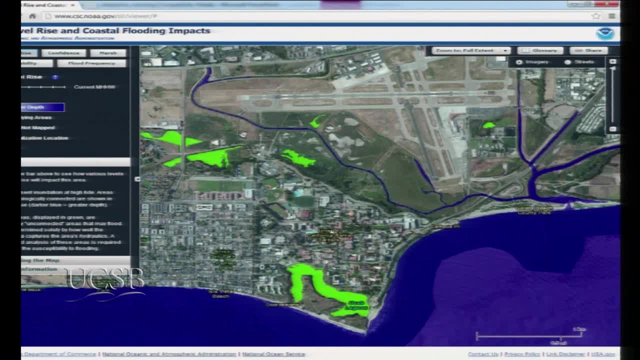 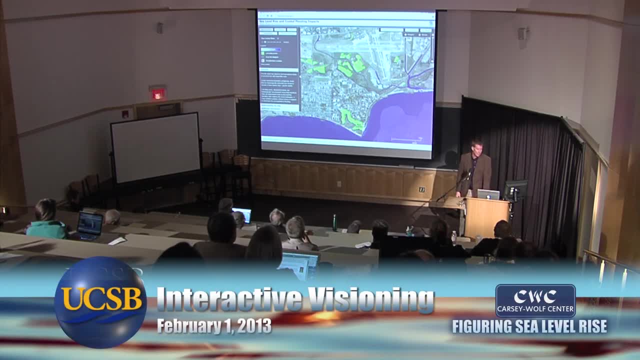 so it's not connected right now, so it shows up as green. let's scroll through this. so one foot above mean high or high water. by the way, mean high or high is sort of the average of the highest tides throughout the year, not the highest of the highest. 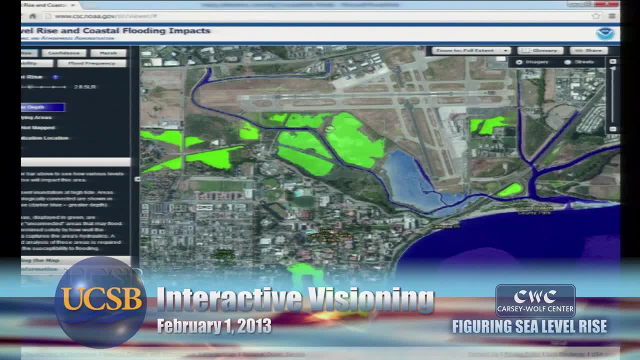 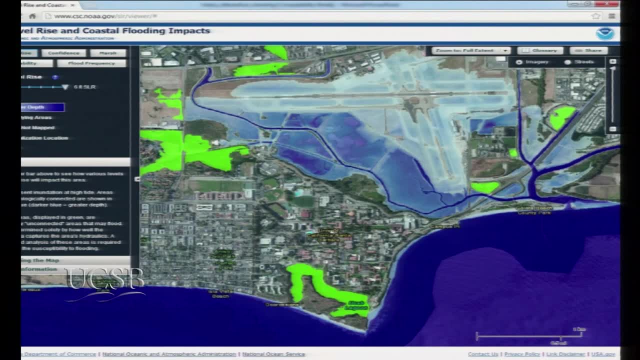 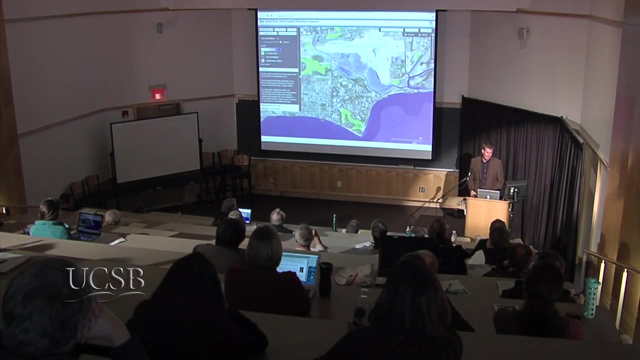 but an average two feet three feet. so that's about a meter four feet, five feet, six feet. so the runway, this runway might be okay, maybe not so much. so yeah, and this isn't just so, this is sort of a- if you want to call it a- sentinel example. because many of our infrastructure, especially if you think about our ports, especially airports, a lot of them are vulnerable. San Francisco airport does the same thing, Oakland airport does this, Philadelphia airport does this, JFK does this, LaGuardia does this. they all flood within the first six feet. 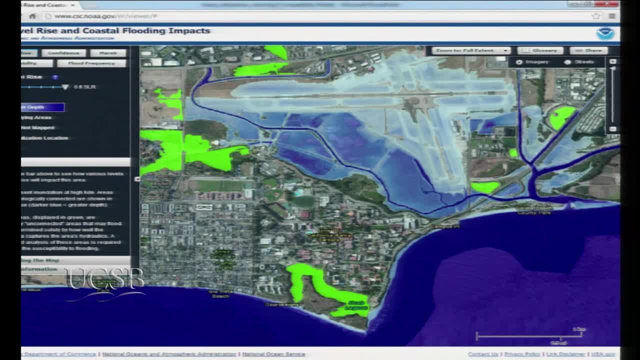 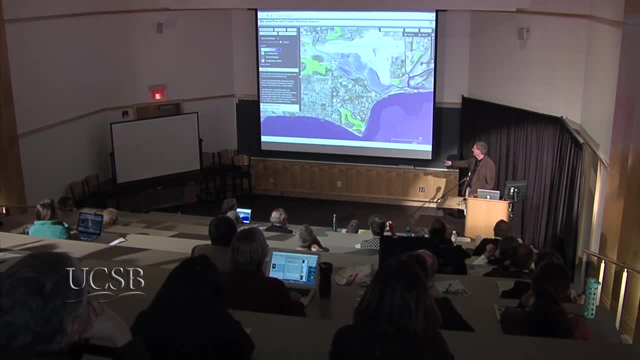 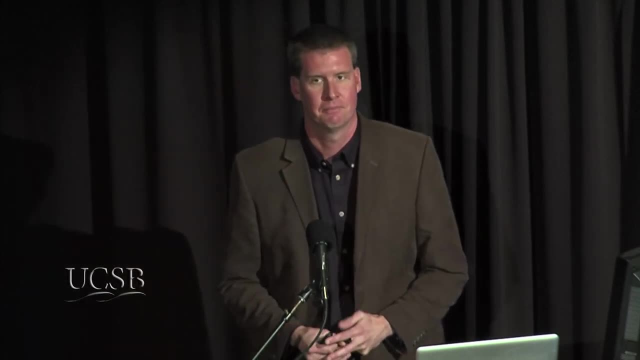 so we're going to have some major, and you saw what happened in Hurricane Sandy: LaGuardia was literally under water. yeah, USD is going to be fine and it doesn't even flood the lagoon. so you guys are up on like a little mesa here. so, yeah, 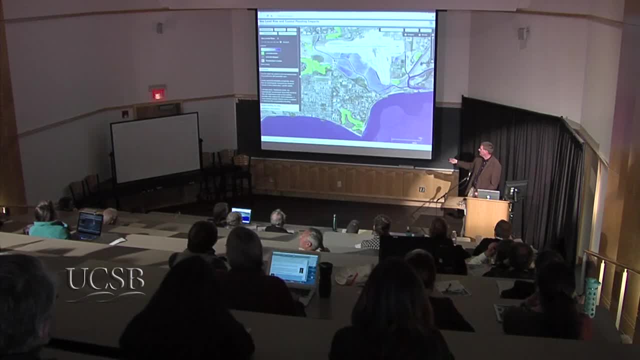 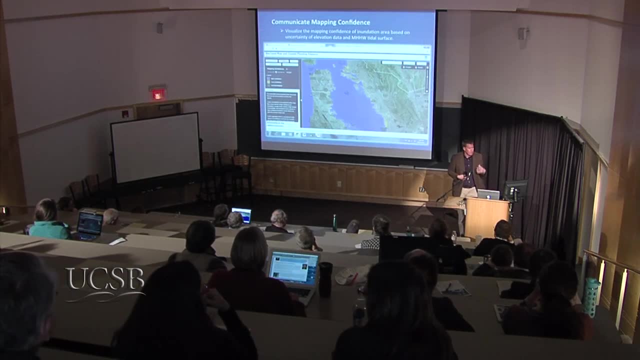 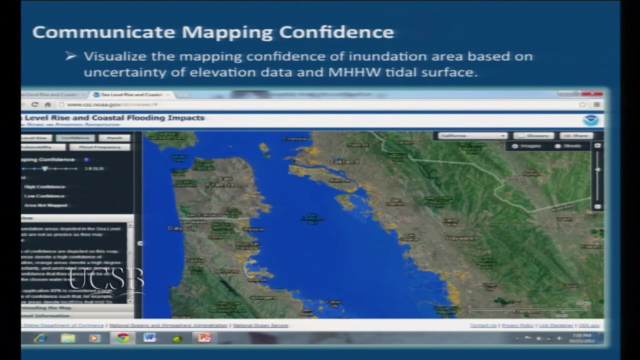 no, the green is wet, but it's not connected to the ocean at that point. so another thing we try to do in this tool is to communicate the uncertainty in just the mapping. I mean not sea level rise uncertainty, because that's a whole different thing, but this is actually the data that we use to create the maps. 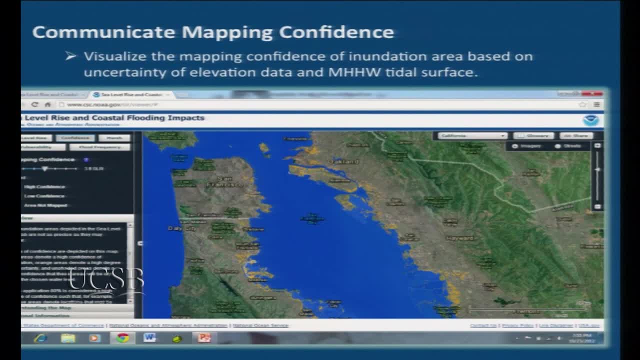 the elevation data and the water surface that we get from. if we know how, what the certainty of that is, we can map and show you how confident we are. it's going to be wet. it kind of gives you the idea it's not just a line in the sand. 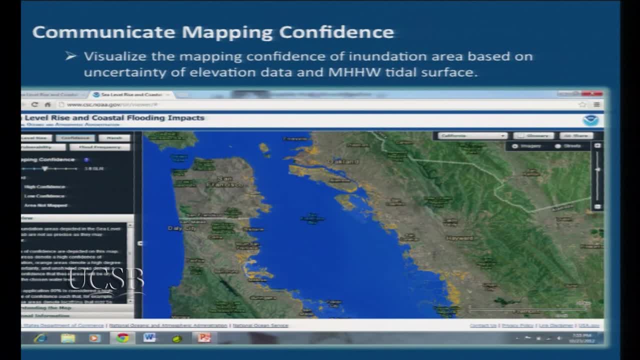 as most maps are. it either shows you wet or dry. you sort of have this zone and you can see it's kind of hard on this screen, but there's an orange area. we have low confidence and we show you we're pretty much 80% sure. 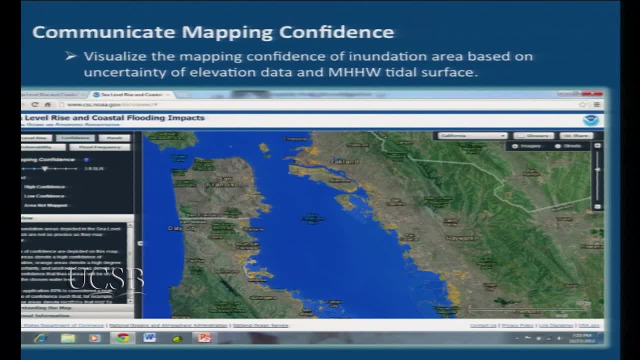 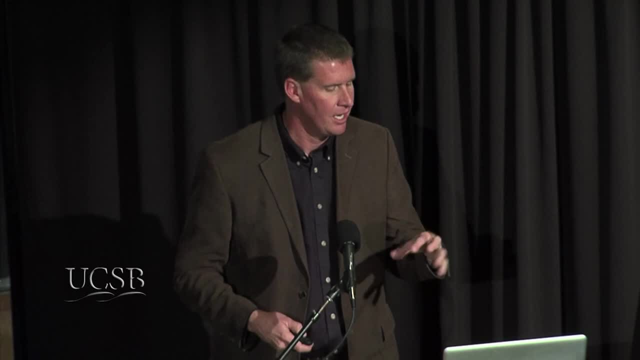 that this blue area is going to be wet and there's an area that we're not quite sure, but we can capture that micro topography in the data. so I think in the future, a lot of this visualization, we need to be communicating some of that uncertainty. 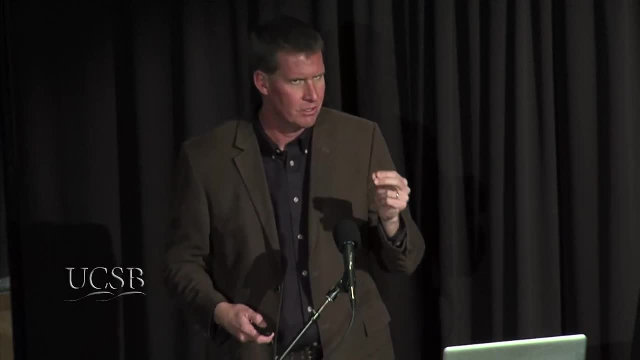 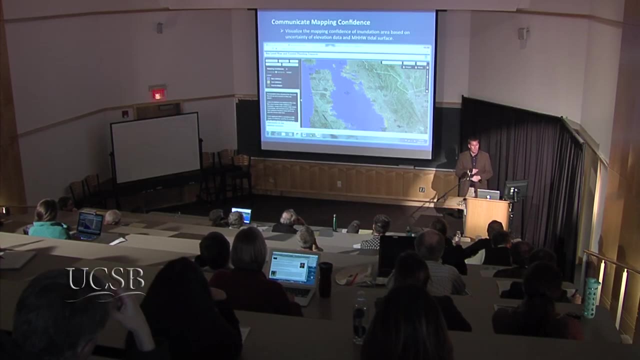 now that's like two way street because you start throwing out: oh, we're uncertain, people don't like uncertainty. but yeah, you think about it and I think it's the word they don't like. so we've actually flipped it around and said: mapping confidence. this is how confident we are. 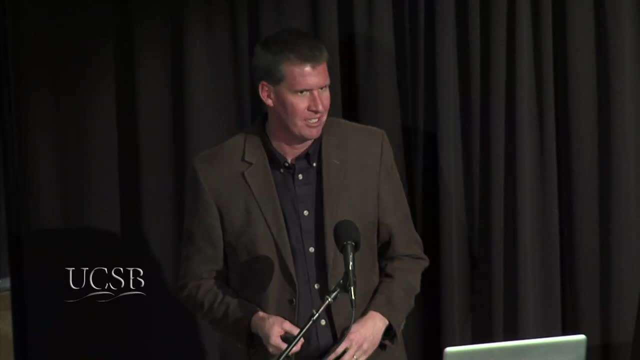 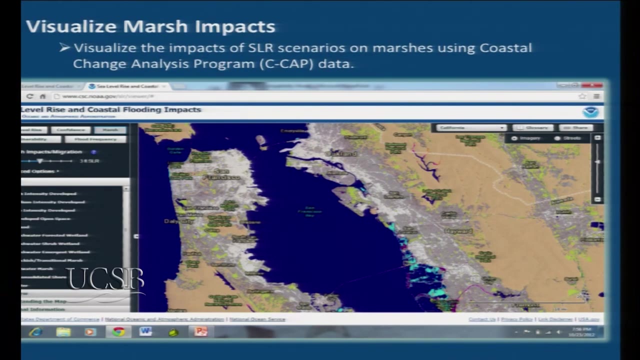 and they like that better. you don't want to be uncertain, so. and another thing is the natural habitat. and how is the marsh going to? is it going to migrate, is it going to be able to keep up, or is it going to run into infrastructure and not be able to migrate? 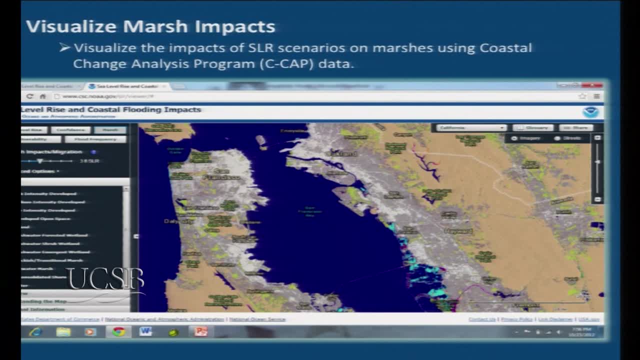 so what this part of the tool does is tries to model the idea that certain vegetation types live at certain elevations and as we raise the water level it will migrate inland, based on sediment rates and what not. so when you do the slider, you can start to see open. water starts to move. 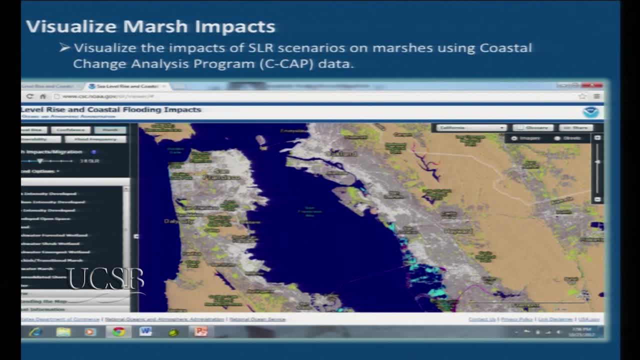 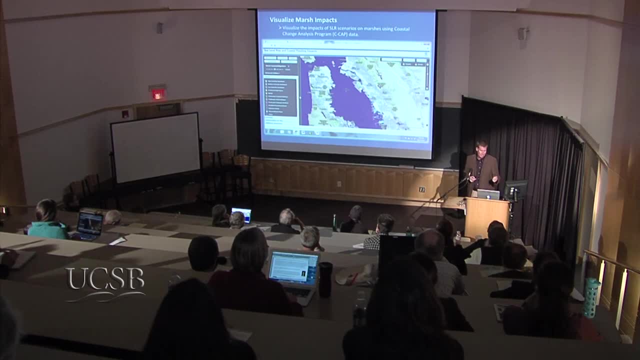 and some of these marshes. but when you have a highly developed area like the bay area, it's not going to be able to migrate. you're just going to hit those. that's what that high and medium density development, those grays and those whites in there. 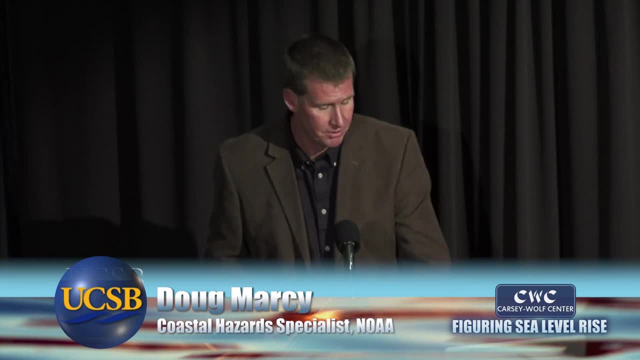 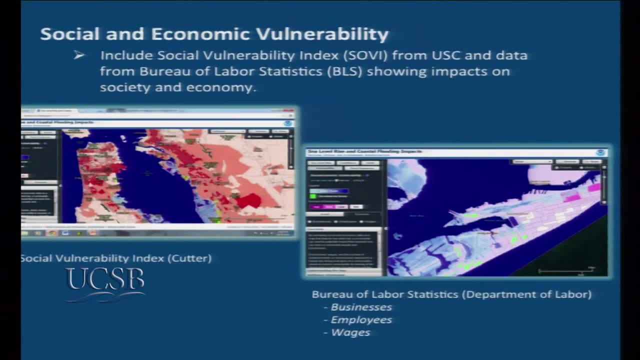 are not going to be able to. we're assuming we won't abandon those areas. we're going to probably sea wall them. and then another key component is to look at the data sets under here that let you see where is the social vulnerability. for instance, this data called the social vulnerability index. 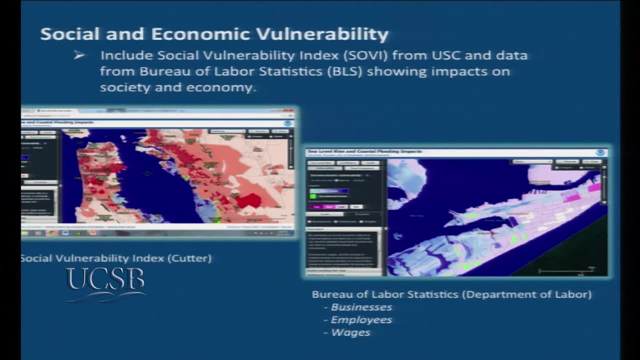 is put out by the University of South Carolina, Susan Cutter, and it looks at 31 different census variables and comes up with an index of high, medium and low. so you see the block groups in here that have more social vulnerability and you can see the areas. 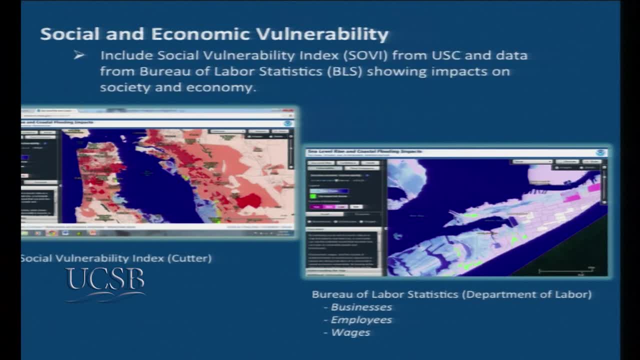 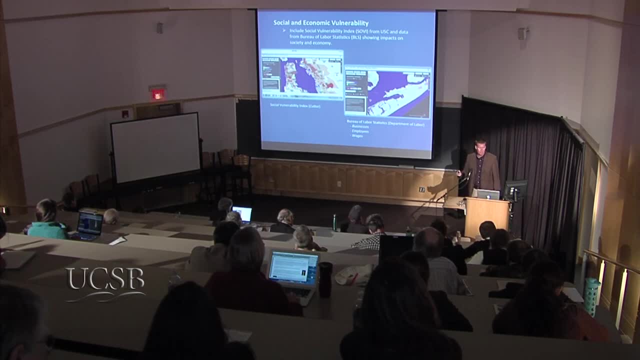 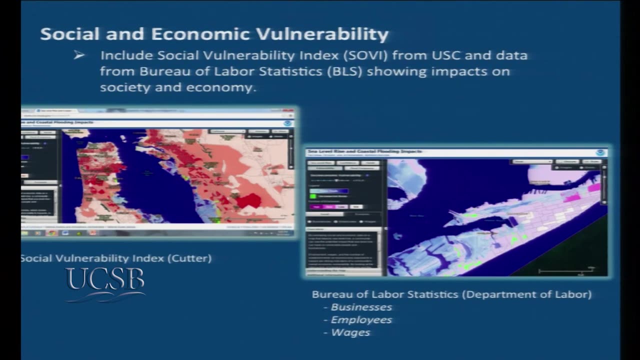 that are going to be impacted and at the same token, we can get data from the department of labor on number of businesses, number of employees and the amount of wages in some of these block groups. so you start to see where are the real impacts going to be. 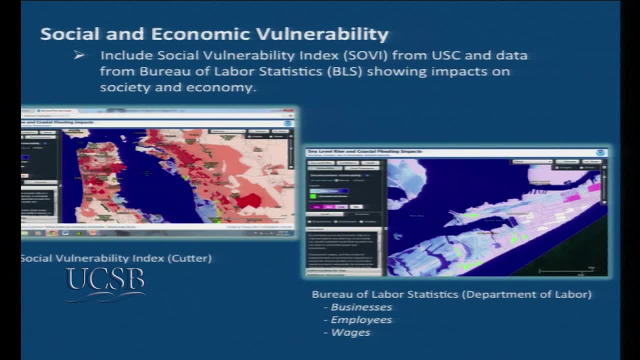 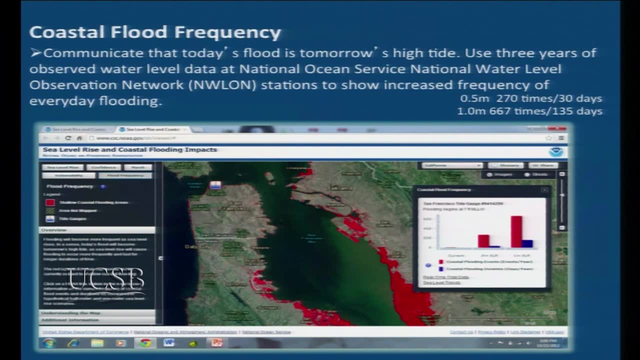 we start impacting businesses and they have to relocate, then that impacts the whole economy and then the last component of the tool is going back to this flood frequency and that is at some of the tide gauges, most of the tide gauges we have. you can click on the tide gauge. 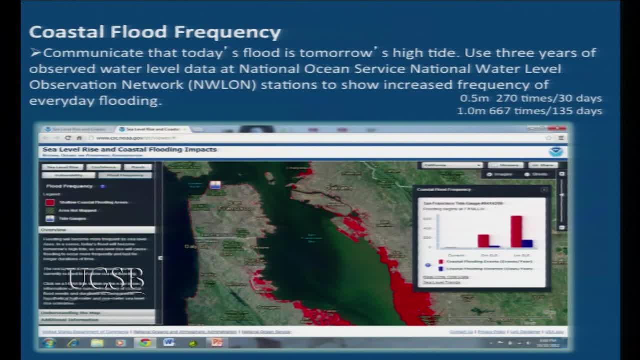 the oldest tide gauge, by the way, in the country is in San Francisco. it's about 150 years of data, so you can click on that and you get a graph. so again, we're using multimedia here and it shows you that, basically, going from now, we barely have any events. 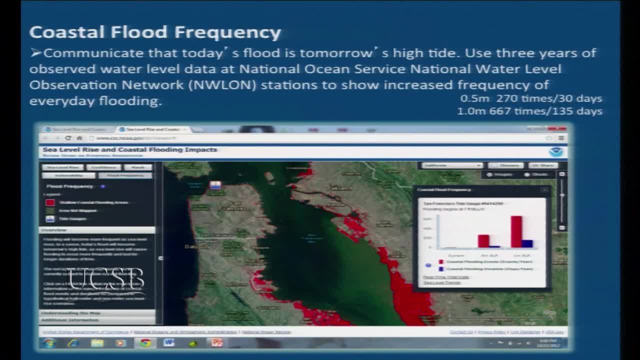 we barely cross over that threshold. this is 7 feet mean low or low water, very similar to the Charleston example I told you. but if you raise it up a half a meter, it happens 270 times, equivalent to 30 days of time. and then a meter it's. 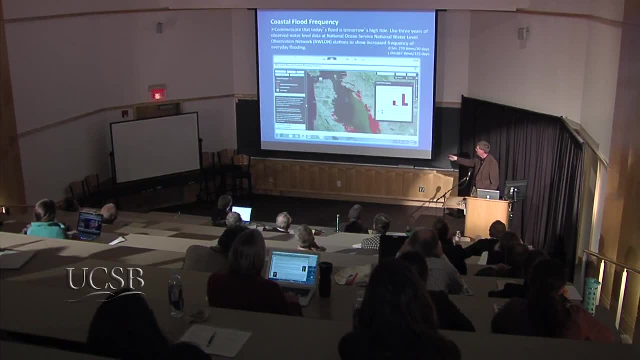 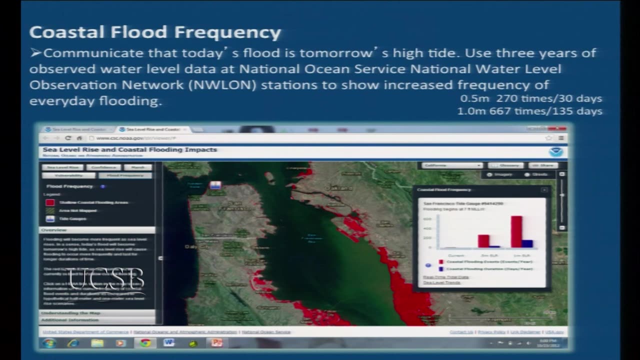 667 times, or 135 days of duration. so these red areas here, that's what would be flooded that often during the year if you raise it a meter. so again, it's pointing out, and this is Oakland airport, so it's pointing out that San Francisco airport 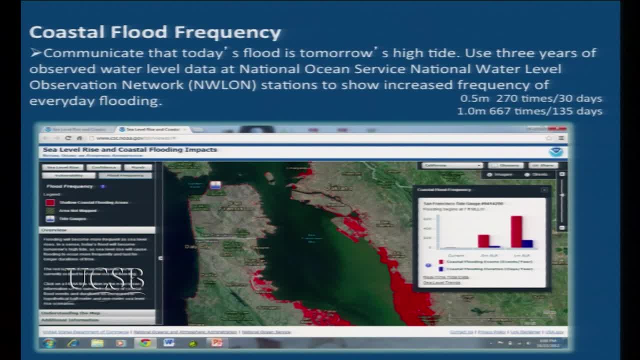 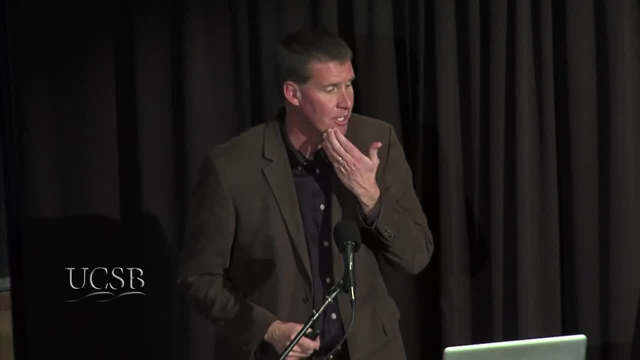 right here. so we have. we're really going to have to start dealing with this and it's going to be. it's not the storm events, we're going to continue to have those and they're going to be in the news, but it's going to be the daily flooding. 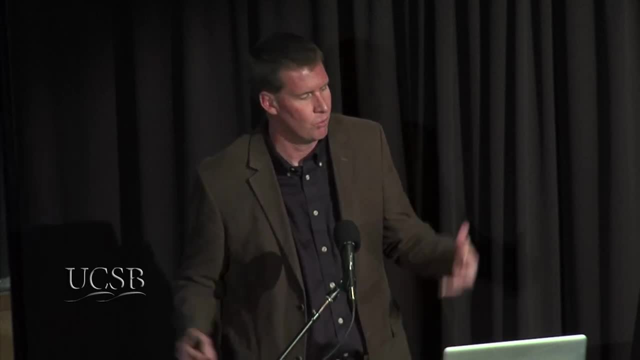 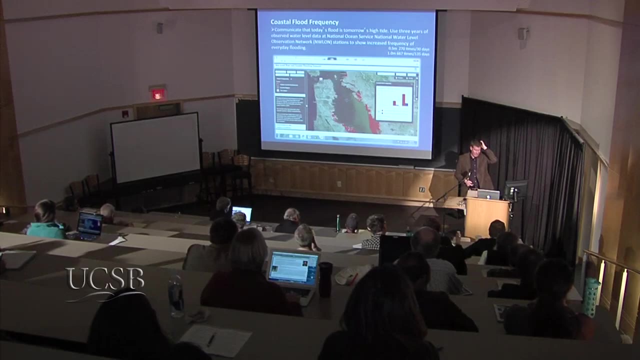 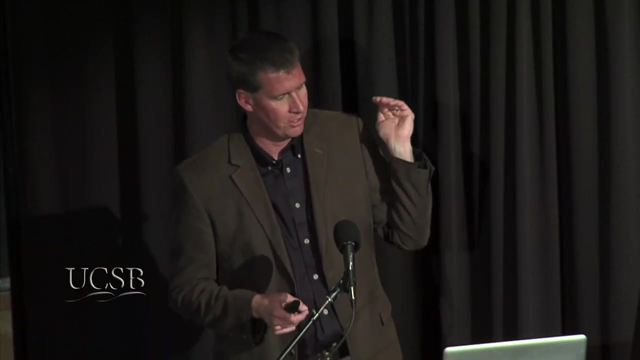 we have to start closing roads and changing our storm water systems and everything else. the water won't drain anymore like it used to when we designed it 50 years, 100 years ago, which is with the case of Charleston, where I live. it really needs to be looked at. 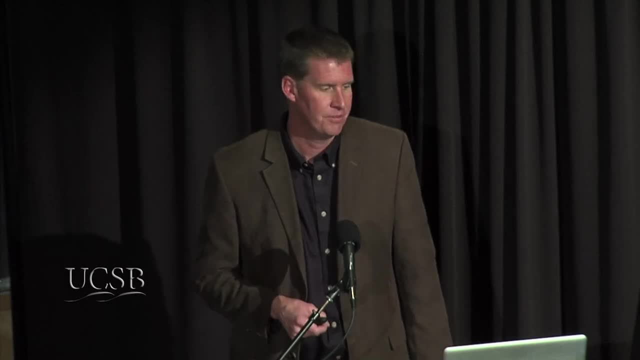 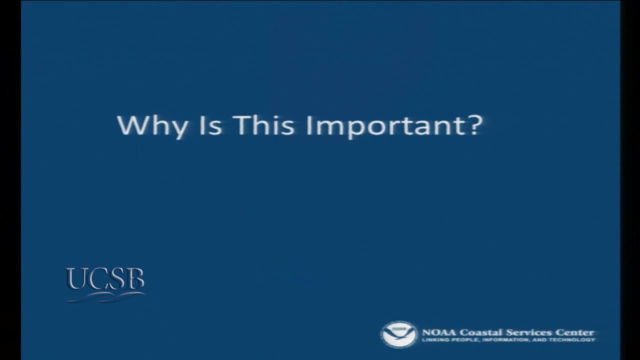 are we going to have to start pumping the water out and putting some head on it? head is kind of a slope, so that the water will drain. so why is all this so important? I think there was a press release done for this and a reporter was asking me. 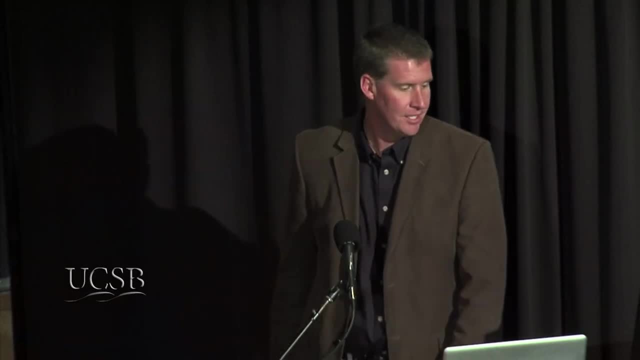 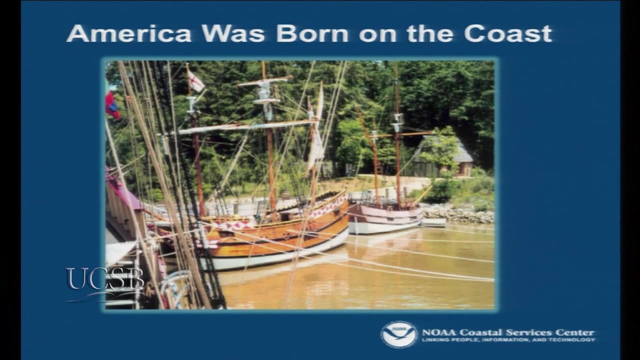 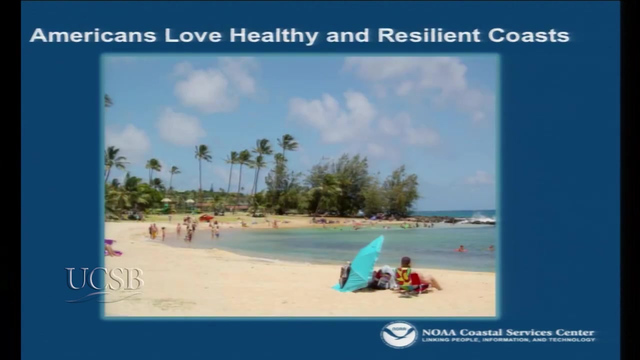 why should we care about all this stuff? and it's because, inherently, as people, America was born on the coast. our first settlements were on the coast. we rely on the coast for so much- and I'll show you another slide- and we love healthy, resilient coasts. tourism is such a major part. 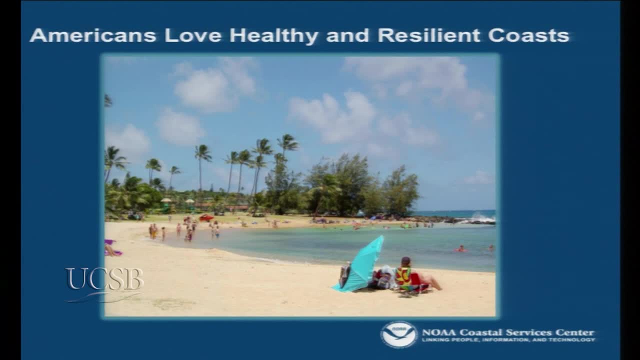 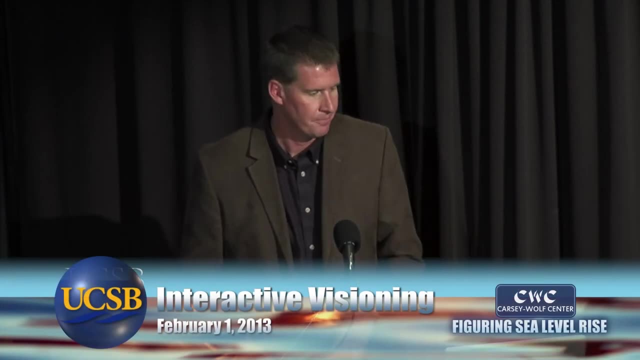 of the economy and a lot of our coastline and coastal states. we love to go and enjoy the beach and as this phenomenon starts to happen, those beaches are going to. they want to roll with sea level and if we put sea walls and what not, we're going to lose our beach. 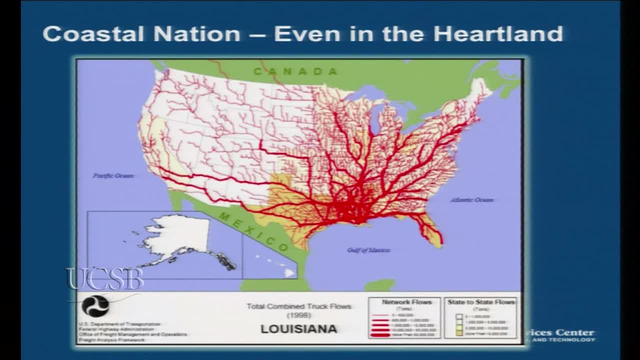 and this is even more important, we are really a coastal nation, even in the heartland. this is the truck traffic that comes into New Orleans and where it goes- and you can see this is by volume- it's literally an artery system. so you start shutting down the ports. 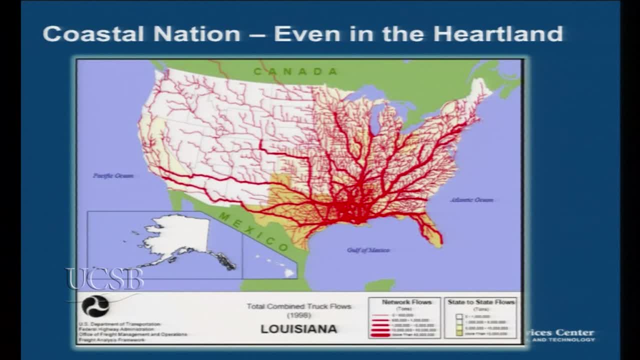 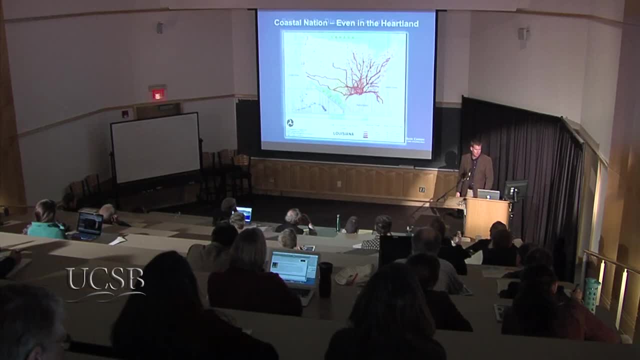 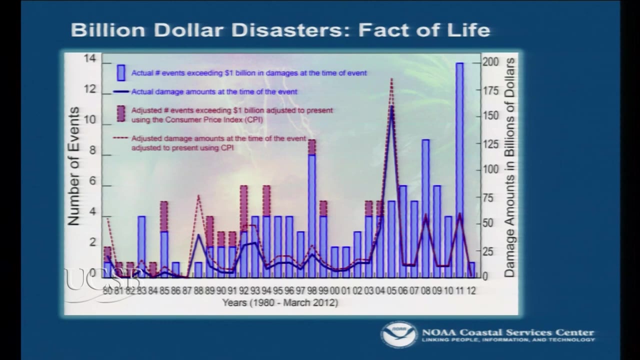 we start losing Long Beach and LA. that's the biggest port we have in this country. if you shut that down even for a day, the economic impacts are phenomenal. and then we keep adding this: we've had more billion dollar disasters. is that because we have more billion dollar things to get damaged? 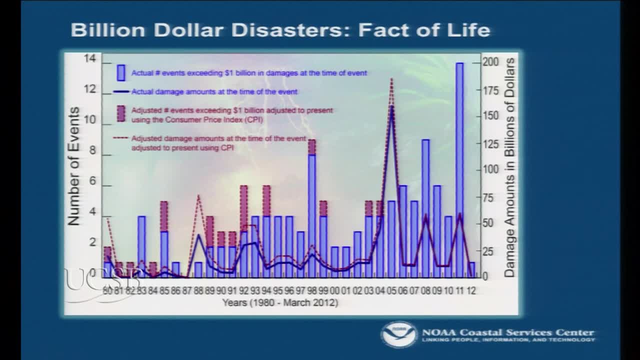 or is it because the frequency is going up and the storms are more intense? I guess that's a debate that we don't- we probably won't get into today, but the fact is, this is starting in 2012 and, of course, we're already through 2012. 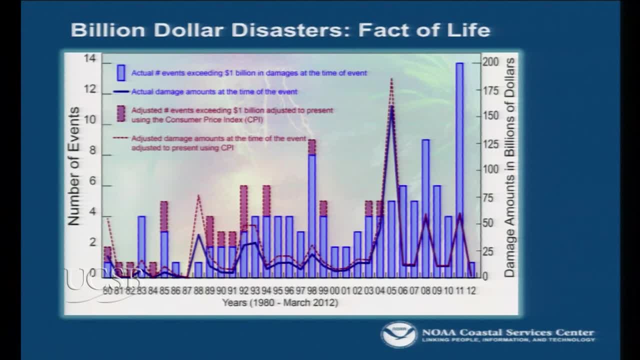 they haven't done the numbers yet, but they're thinking that 2012 is going to surpass 2011, which last year was 2011- was the highest number of billion dollar disasters. we're probably going to supersede that this year, so are we on a trend? 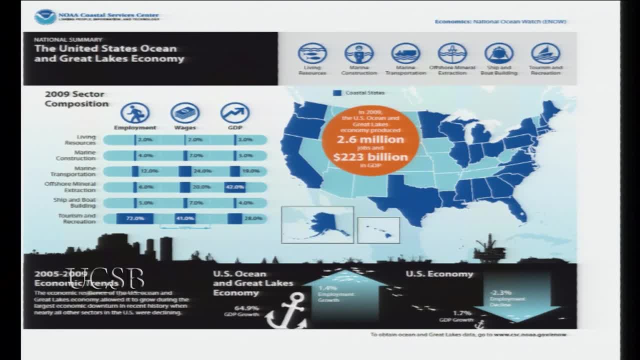 potentially, and if you look at the ocean, jobs- the jobs that the ocean and the coast create is divided up by living resources, marine construction, transportation, anything having to do with relying on the ocean. it's just going up and up. it's 2.6 million jobs. 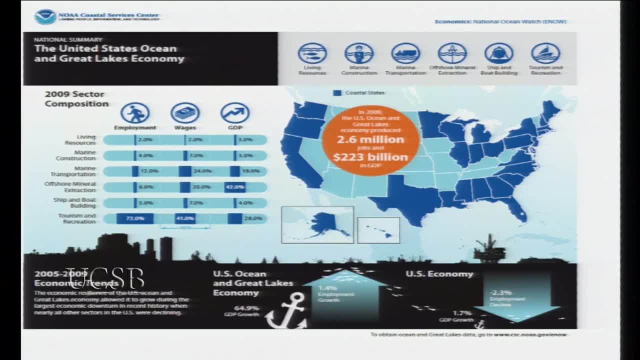 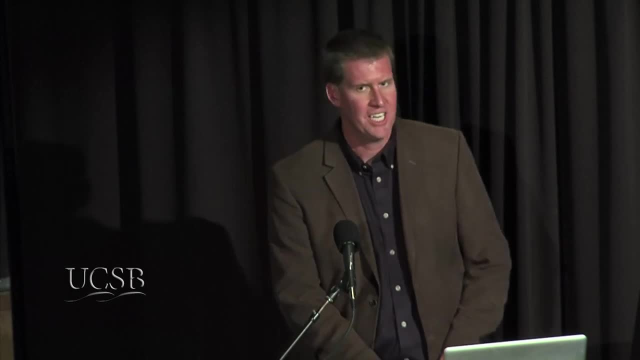 generating 223 billion in the gross domestic product. you can see that as overall the economy slowed, this sector has continued to rise, so even more and more people, and a lot of that is tourism driven. so, with Sandy a turning point, it certainly did wake up a lot of folks. 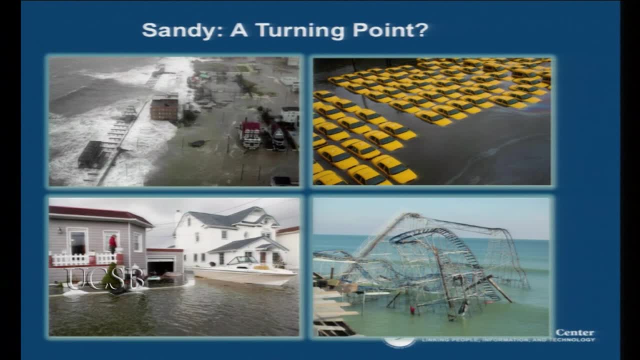 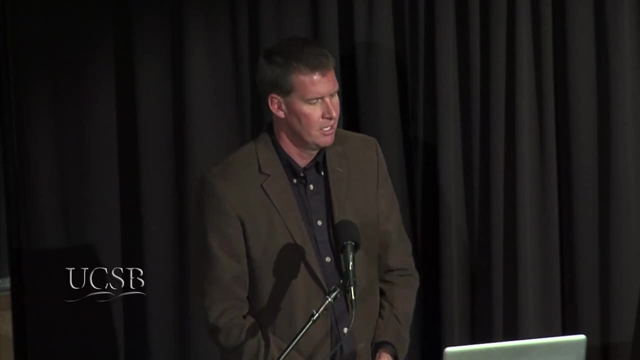 I think it hit such a populated area of the country. there was a lot of discussion that they weren't ready. they didn't understand the risk that was going to happen. but it also got people to start thinking, hmm, this climate change thing might be a real deal here. 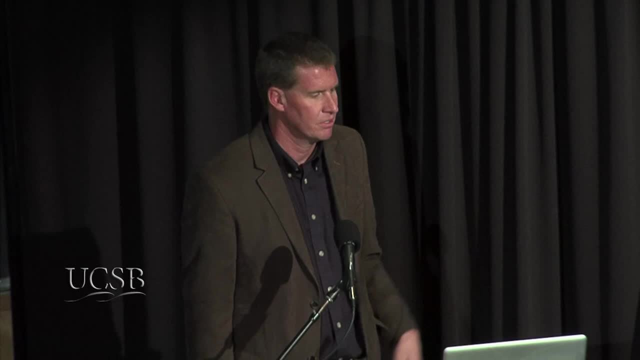 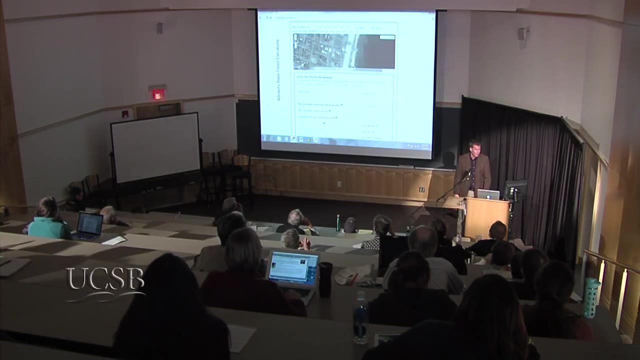 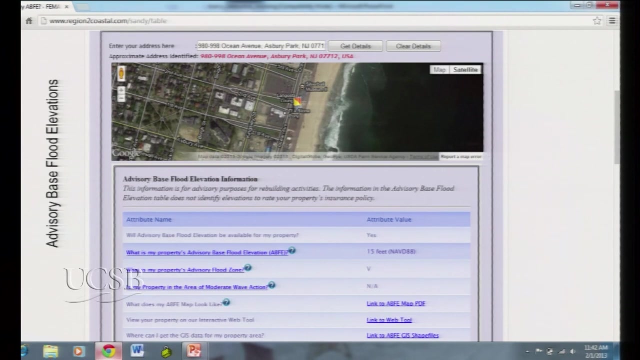 because it's actually impacting us and I don't remember storms, especially different generations, and storms being that bad and causing that much damage. so what FEMA has been doing up there- and I'm happy to say that we're trying to help with this effort- is to put out 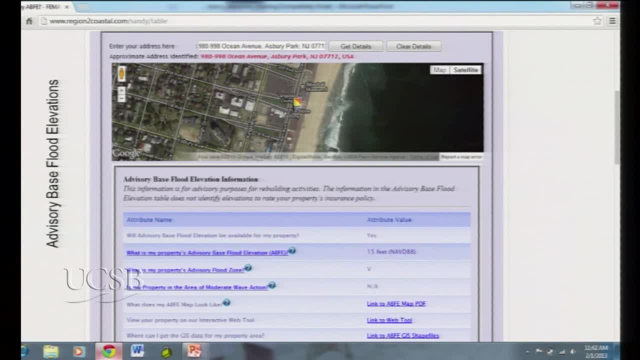 advisory flood maps. the New Jersey and New York area had really really old flood maps, about 20 years old in some cases, so the elevations they tell people to build to were based on older information, older models. so they're in the process of updating those maps when Sandy 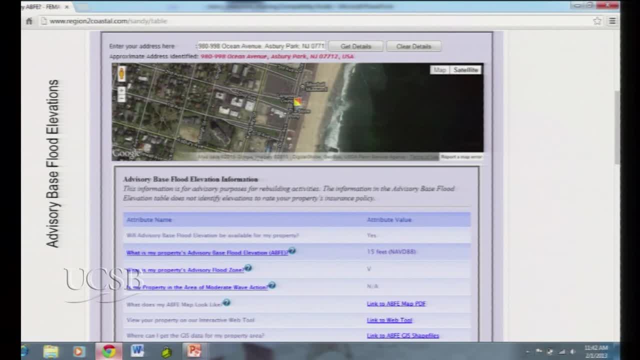 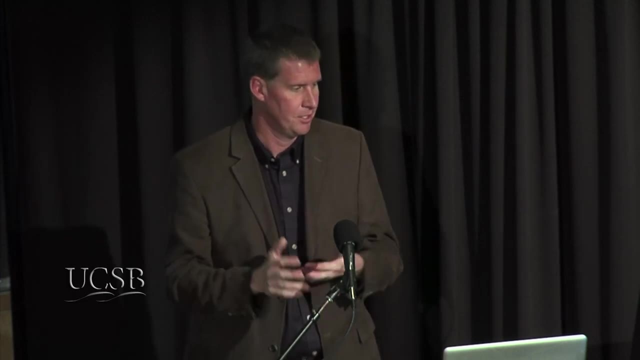 hit. so in the meantime, they've put out what are called advisory based flood elevations and they're telling people: please build back to these heights if you will, so that you're going to build yourself out of the risk zone and build back smarter and better. that's the whole idea. 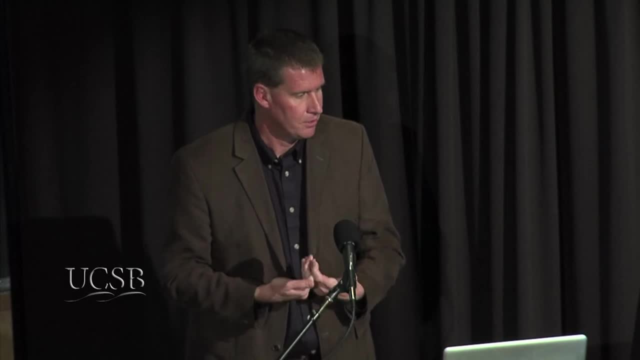 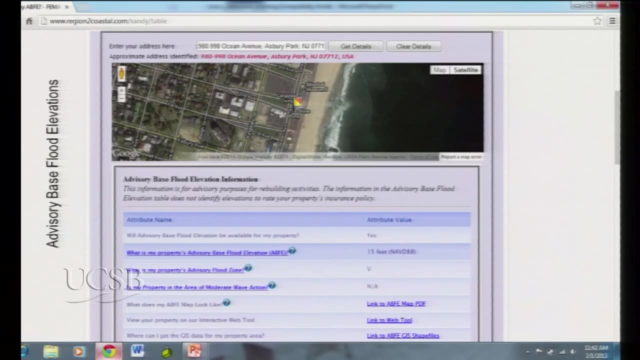 next time, instead of just building back to the existing footprint. so what they've got here? this is just a simple tool that you can go in and locate. this is an Asbury area in New Jersey. you can type in your address, get a location, and it tells you. 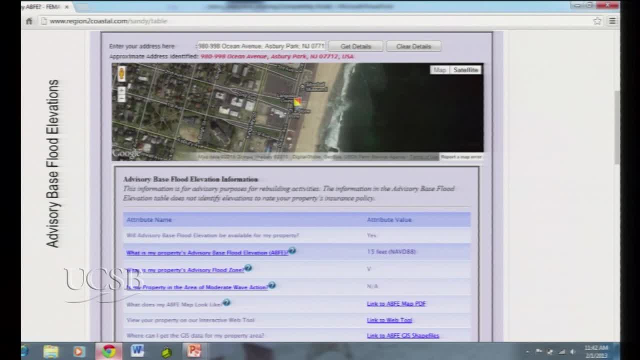 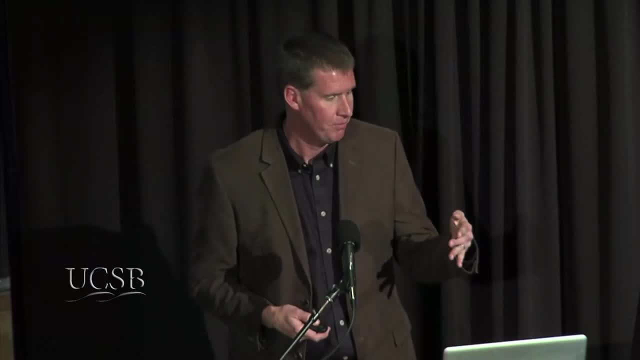 it's very easy. these are the type of tools that people want to see. will advisory based flood elevation be available? yes, is my property. what's the elevation going to be? it's 15 feet. the next thing they want to add is: you want to actually know what the elevation. 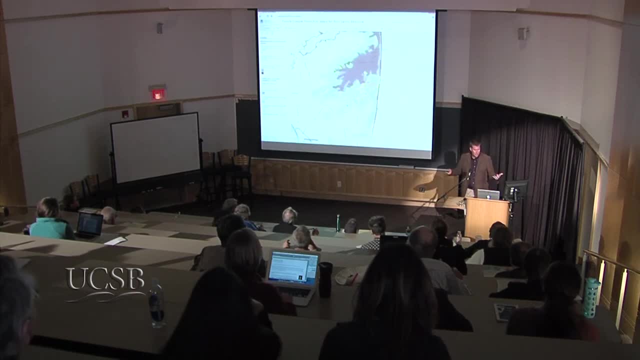 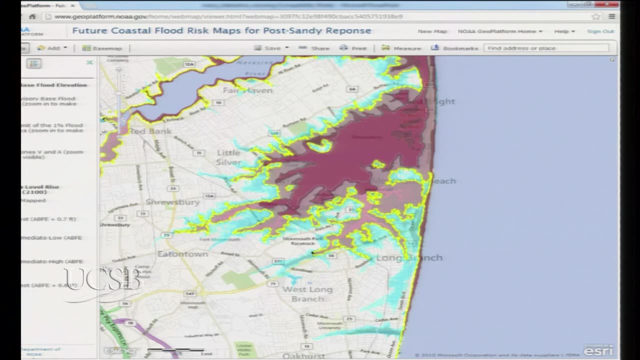 is of your first floor. so easy tools like that. and then guess what? a map, of course. so they're mapping the advisory flood layer. here you can see the yellow- this is what they call the velocity zone in red, and then this is the. these are areas where waves are going to be impacting. 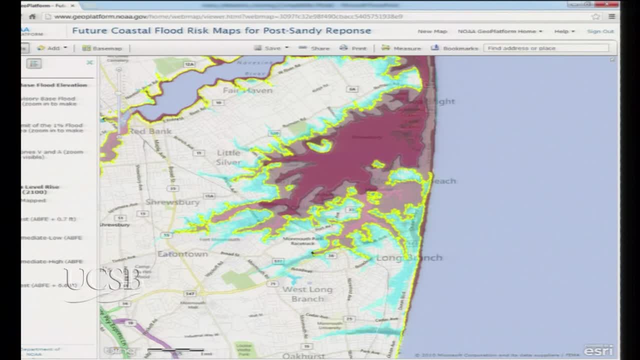 and then the other pink is just going to be still water. but then we project the different scenarios that we were just talking about out of that NOAA report- lowest intermediate, low intermediate, high- on top of that. so you can start seeing: this is what the 100 year floodplain is going to look like. 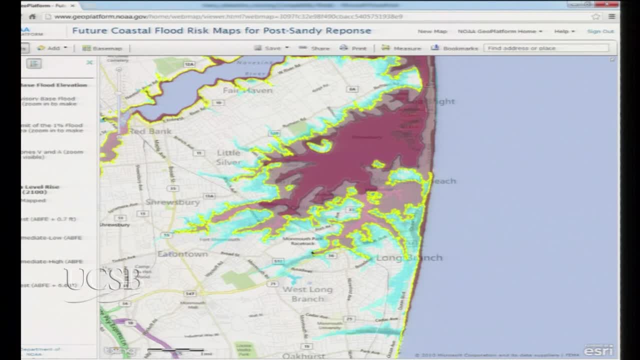 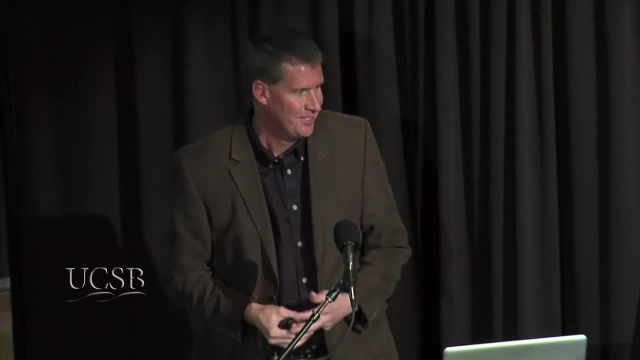 you know, by 2050 or by 2100, because people go: well, I'm not in the floodplain, so I'm not going to get insurance. well, you aren't, but just wait a few years. so yeah, we're trying to communicate. so this is an effort. 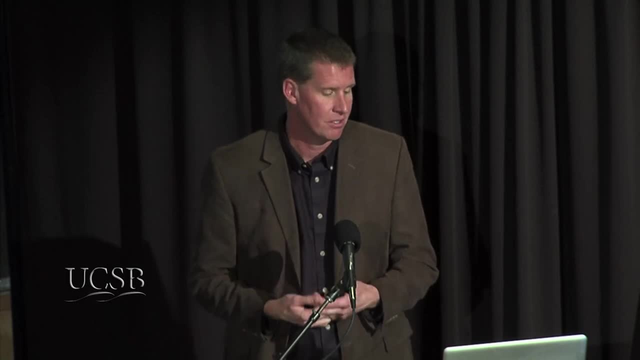 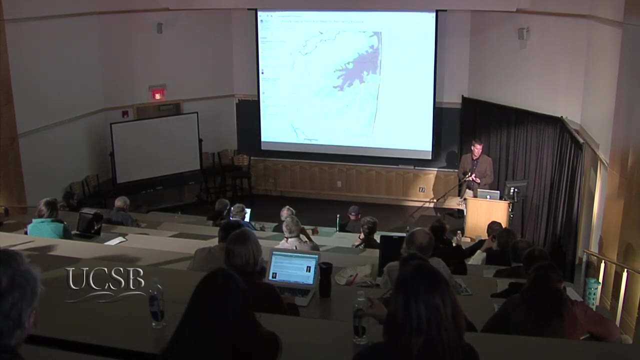 it's the first time it's actually being led by a White House CEQ, that's the Council on Environmental Equality, and so we have FEMA involved, the Corps of Engineers, NOAA, working together on really trying to communicate that there is future risk. currently, the National Flood Insurance Program, 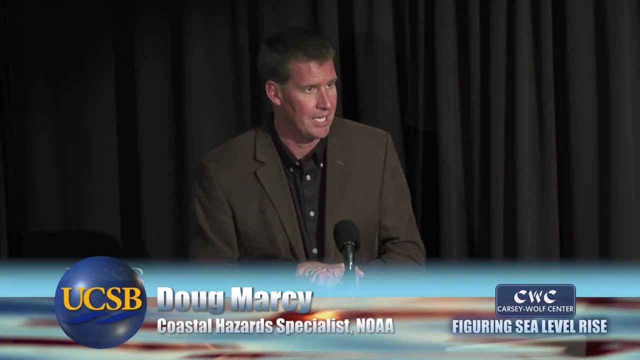 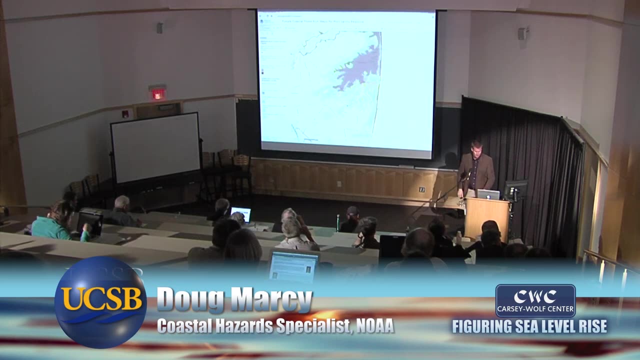 doesn't take into account future risk. it only maps the hazard today. it doesn't take into account sea level rise. so we're really trying to change that and put out some products that do let people know, because people do start asking if I'm going to invest an amount of money. 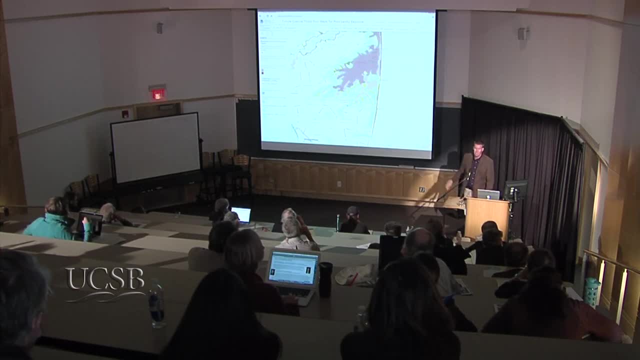 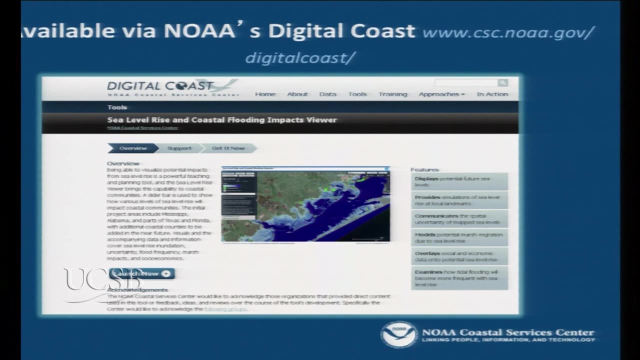 to rebuild. you want to get it right. you don't want to have to do it again in another 20 years or so. a lot of these tools and things that I've mentioned today are available on our website, Digital Coast, kind of a resource for a lot of. 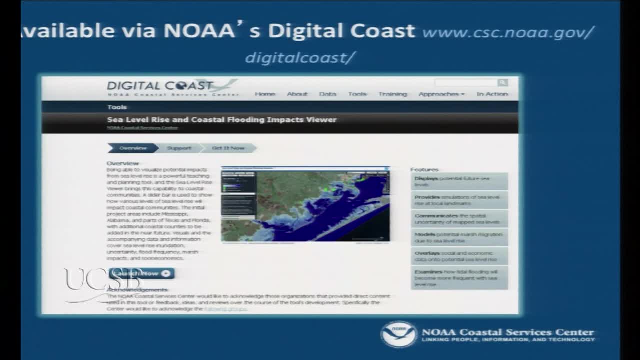 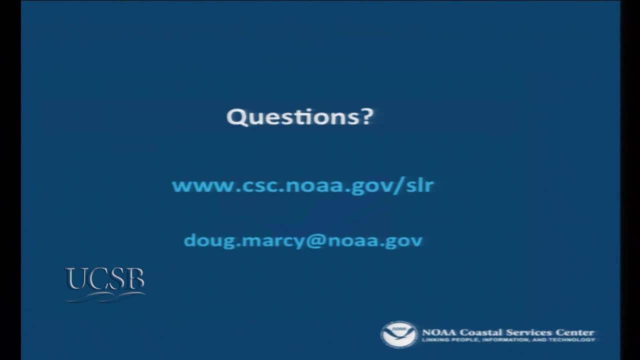 you can go in there and get data. there's also a lot of the tools I talked about, so I encourage you to go there- and our sea level rise viewer is there too, and there's the URL for the actual tool- and go in there and play with it. 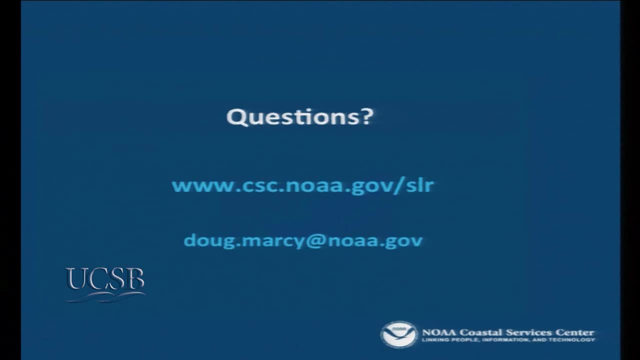 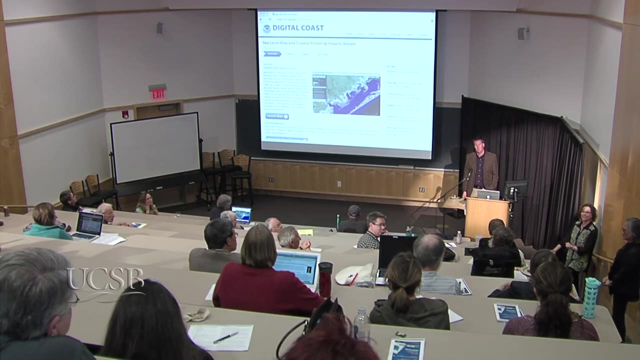 I don't know how much time we have. I could actually pull it up and do a demo, or we can just take questions. you kind of got the gist. You've got these tools out there. how has the public responded to them? again preaching to the choir using these kinds of tools. 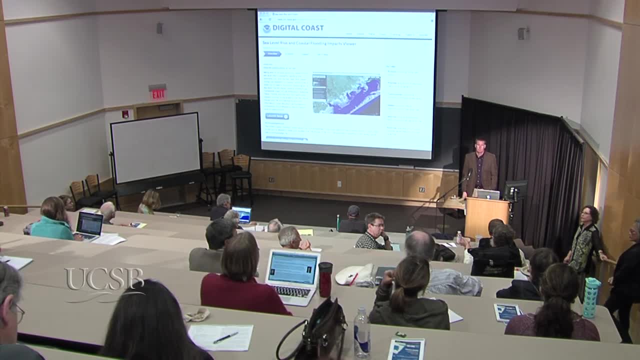 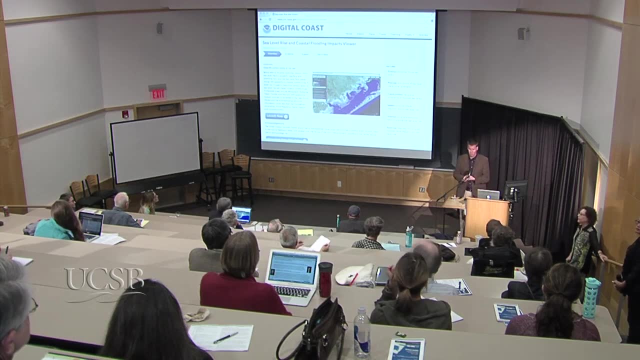 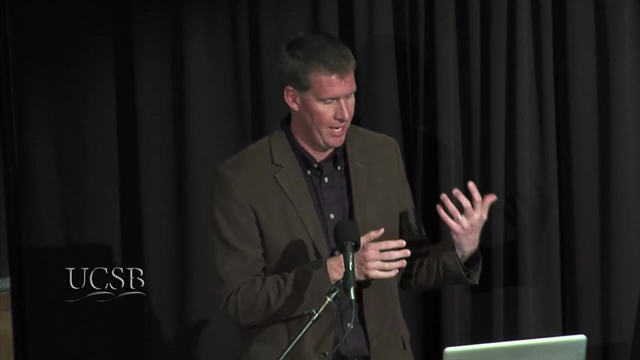 if not this specific one. has this been useful? has the public seen it as too technological? have they embraced it so initially in the design of the tool and the usability was not really designed for the public we don't tend to. our audience is more managers, coastal resource managers. 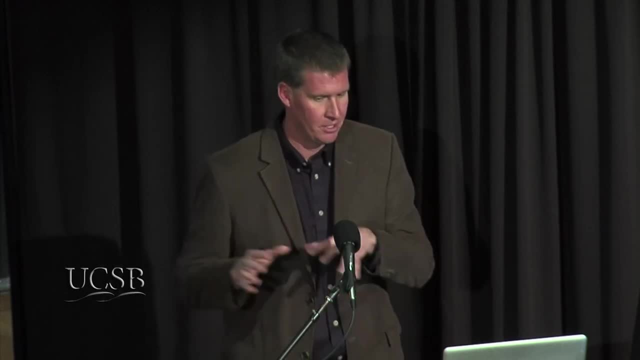 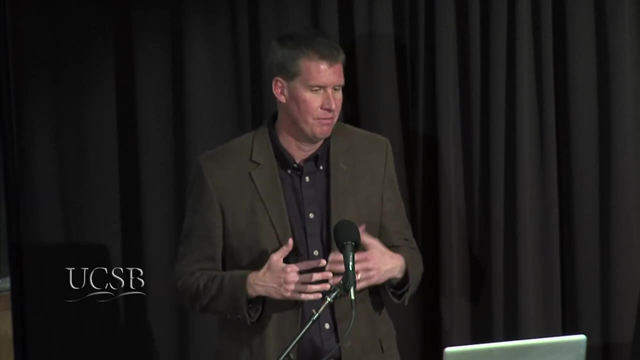 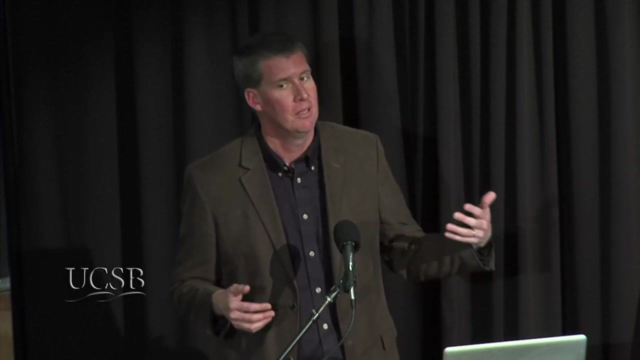 floodplain managers. so I think there's definitely a market for this, for public outreach, and as we we're in the process right now and technology changes so fast, the actual software that our tool is developed in has kind of become obsolete. so we're looking at different options. 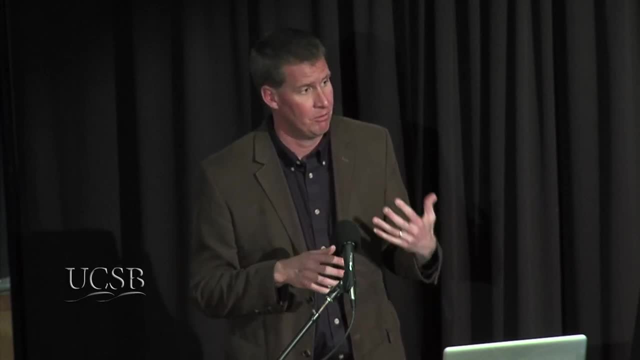 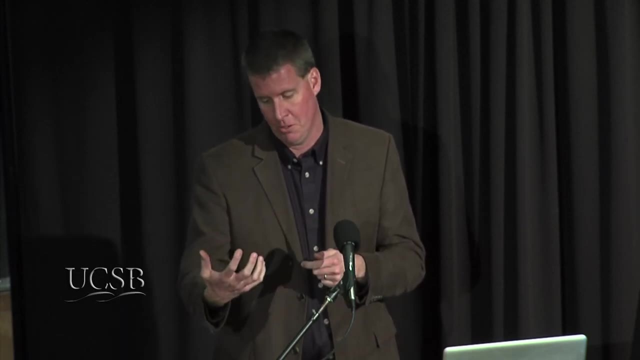 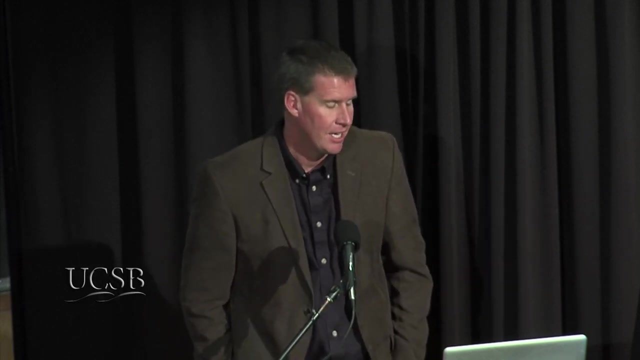 people want to see this stuff on mobile and on their iPad and right now we can't do that, so we're looking at stripping out components of the tool. potentially, you could have your smart phone and it tells you your GPS location and where you are, and you can slide the thing up and down. 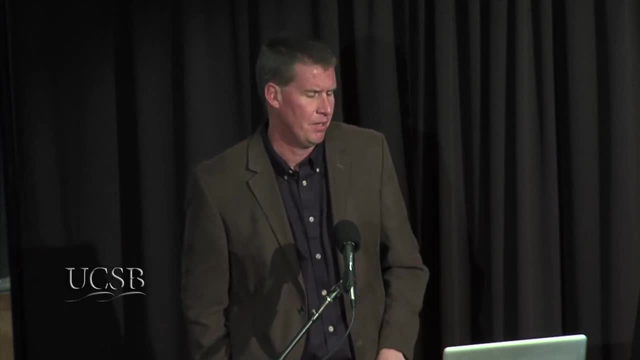 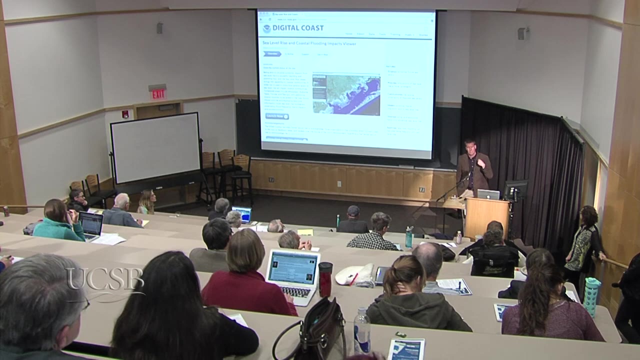 so right now it's not really a general public. we don't have that many comments coming from the public. most people that want it are using it for the visualization, but they actually contact us to get the data. they want to be able to use the data to do analysis. 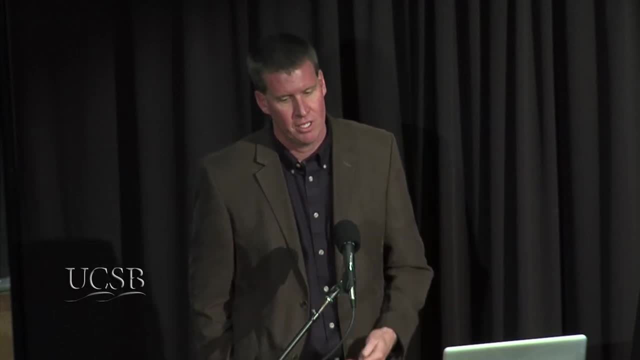 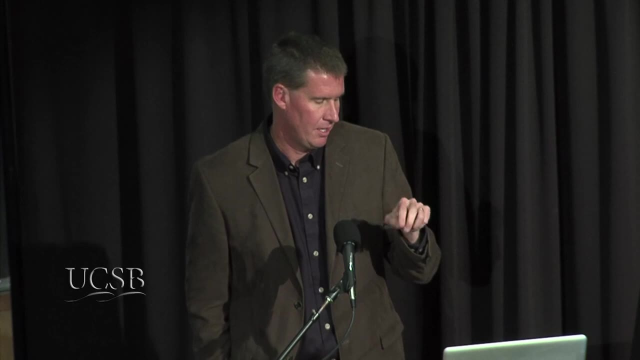 so they're usually trying to do an adaptation plan. we have a lot of other federal agencies. for instance, EPA is trying to locate their outfalls point- source solution outfalls- and look at how many of those are going to be impacted and use the data it's been mapped. 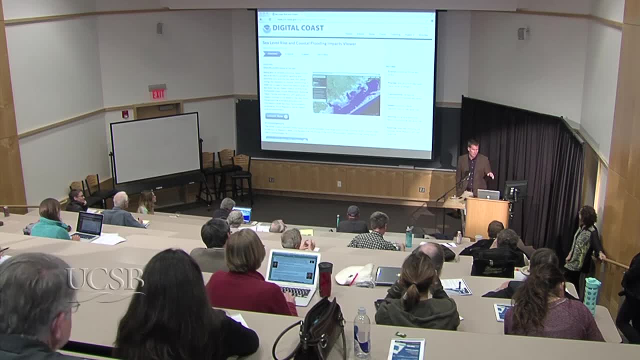 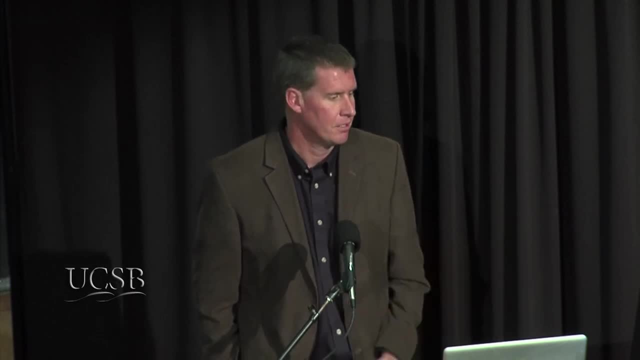 it's consistent. the core of engineers is interested in their federal projects, so that's more of the application when we designed it. but I think there is an outreach component. some of the derivative products, like the tide, some of the tidal flooding stuff: today's tide is tomorrow's. 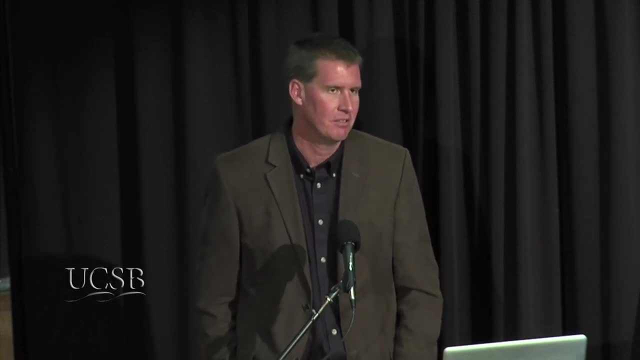 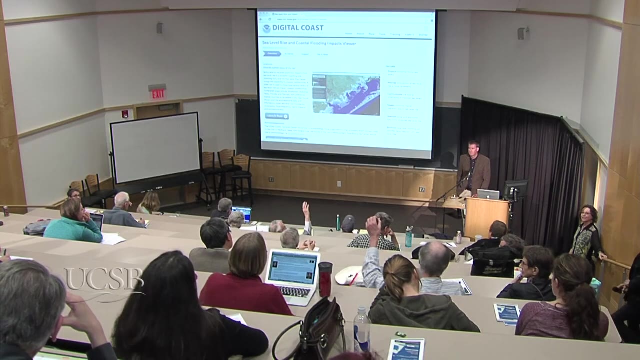 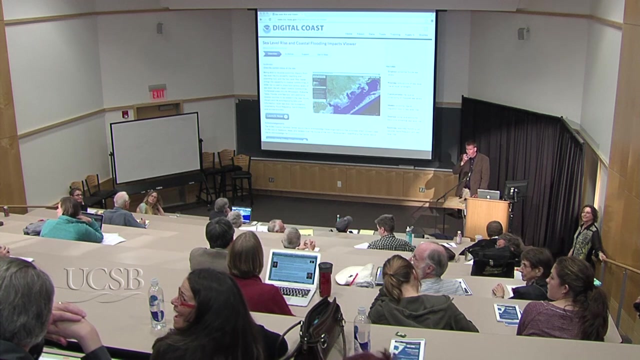 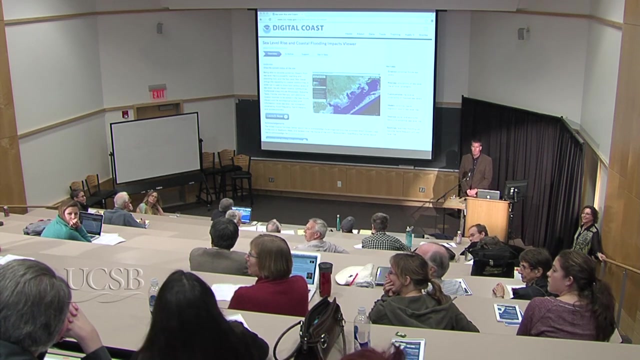 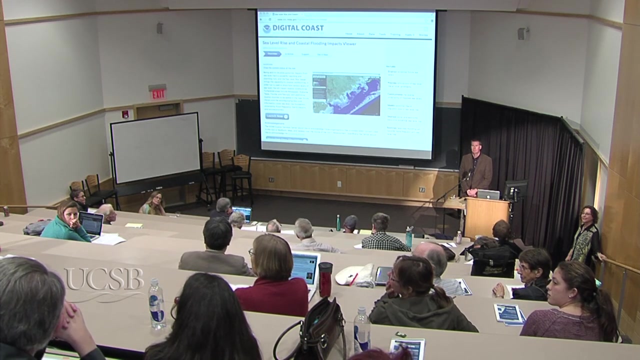 whatever it was, that's more for the public to start thinking this might be a problem in the future. so so yeah, those of us who have been thinking about climate change for a long time, I think there's a level of frustration with the acceptance of it and the way it actually 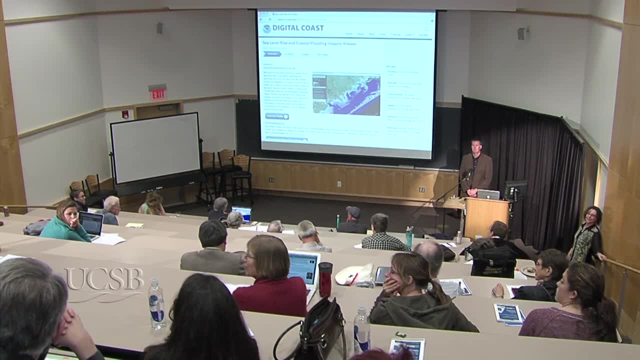 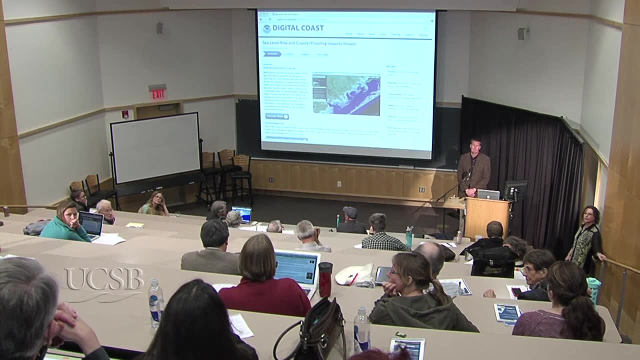 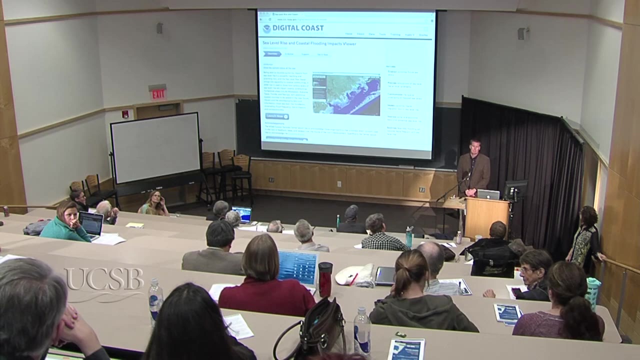 as the data have accreted that the public is actually doubting, it has actually increased. have you, at NOAA, seen any change, significant change? I mean you mentioned it anecdotally, but what have you seen as a significant change since Sandy and do you think that is, in fact, the watershed moment? 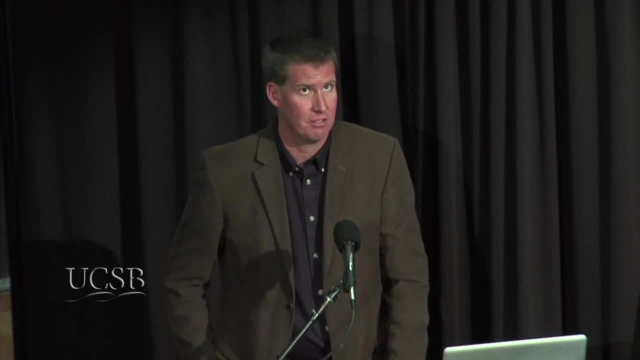 that might actually shift the debate from what I have seen since Sandy. yes, now the general public, I don't know. like I said, we don't work directly with the general public. we don't do a lot of education, outreach for the public. the federal agencies anyway are in a big way. 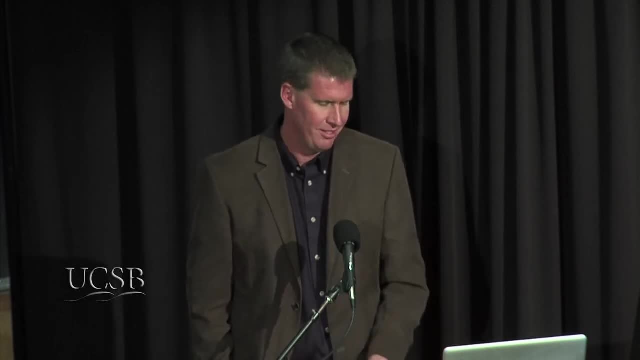 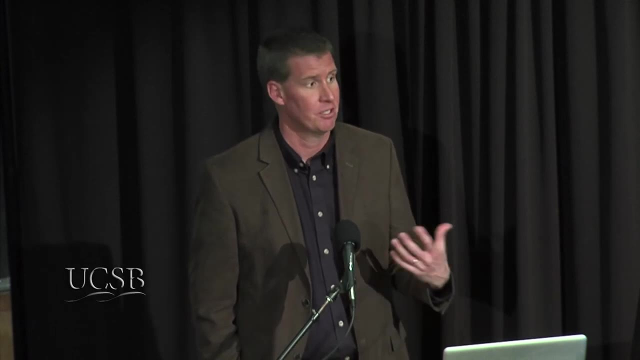 starting to do this. we were doing it on our own anyway, but when the inauguration speech, you know, they came right out and said: yeah, we're going to head on climate change. you know, that's like the green light, like go ahead. there was some with the previous administrations. 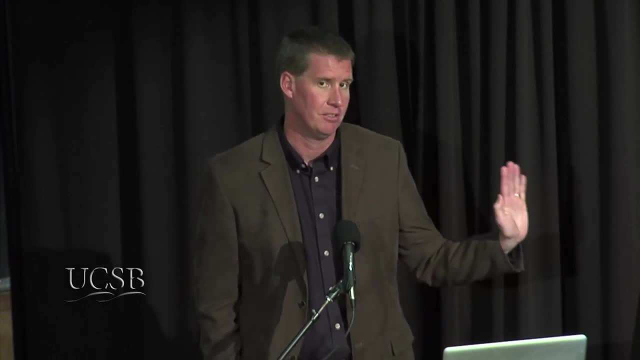 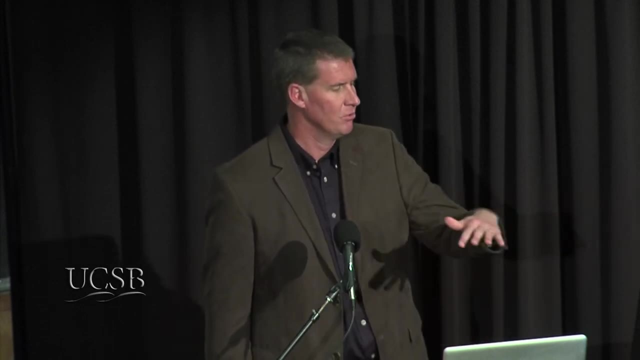 we had started this project- you know we weren't really advertising so much we were doing it- we were afraid, oh no, we're going to put the kibosh on this. and then we said: let's just call it sea level rise. and the director she's like: your title is too long. 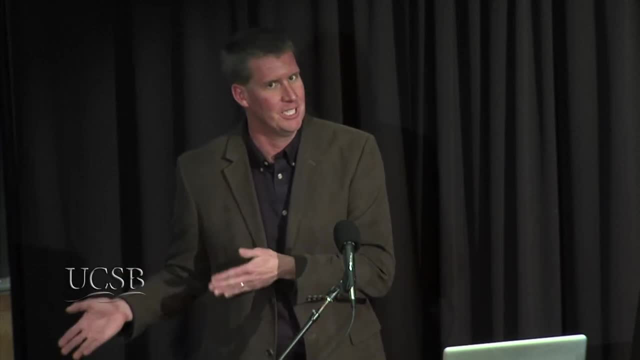 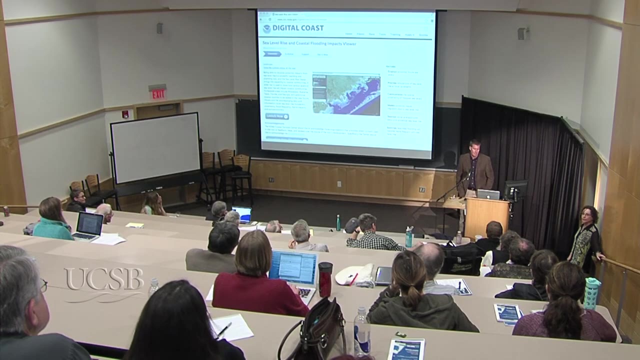 that's never going to work. sea level rise- that doesn't roll off the tongue. let's just call it sea level rise. and I said no coastal flooding impacts. if you don't believe in sea level rise, it's still coastal flooding impacts. it's all about how you market it. 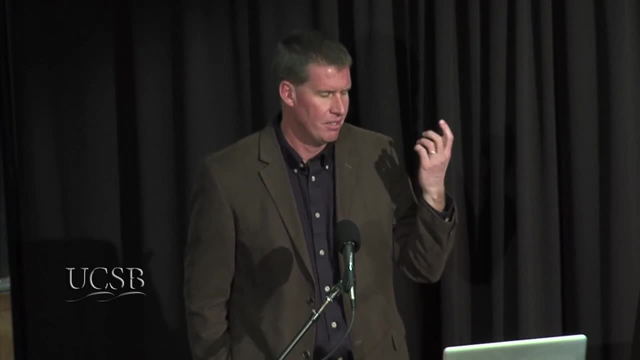 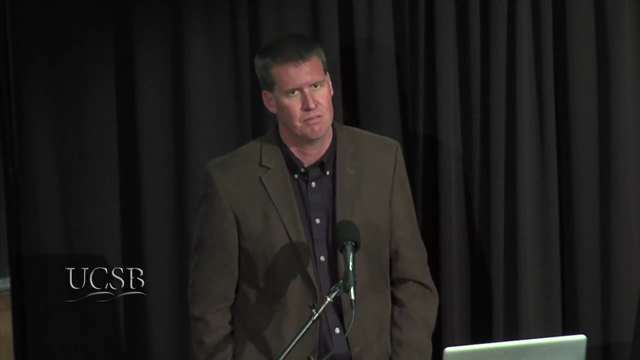 but no, I think there's definitely been. it could have been the watershed moment. I think that it's one of those just was I mean order of magnitude of more destruction than they've ever seen. So I think they're thinking something's behind this. 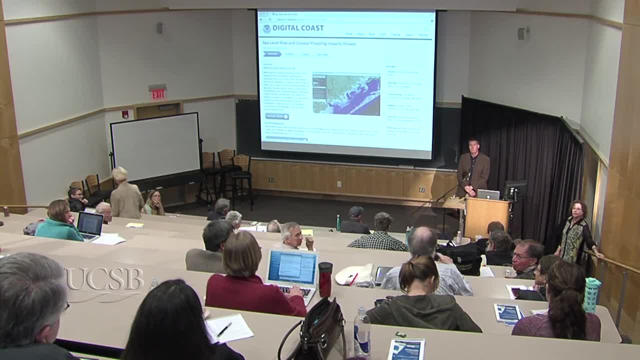 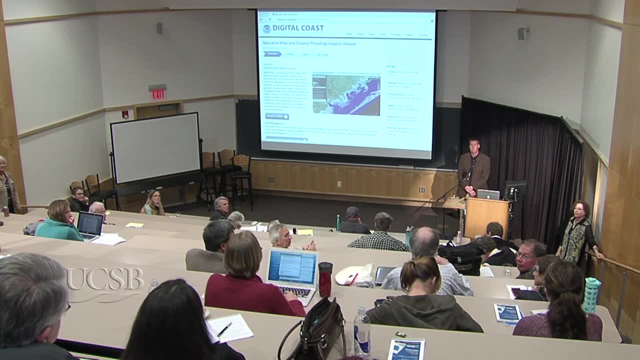 I really like your effort with FEMA on the 1% lines, the 100-year flood lines, because a lot of people understand the 100-year flood concept and have accepted that if my house is there or my property is there, I ought to do something about it. 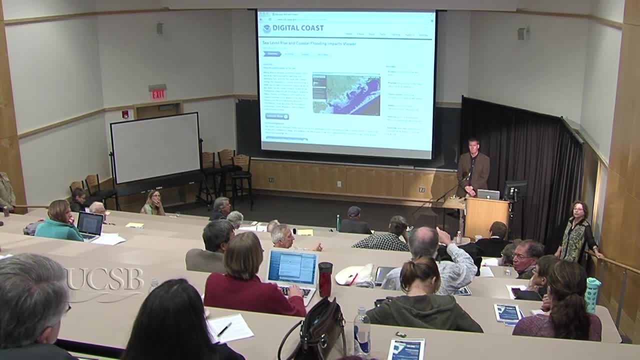 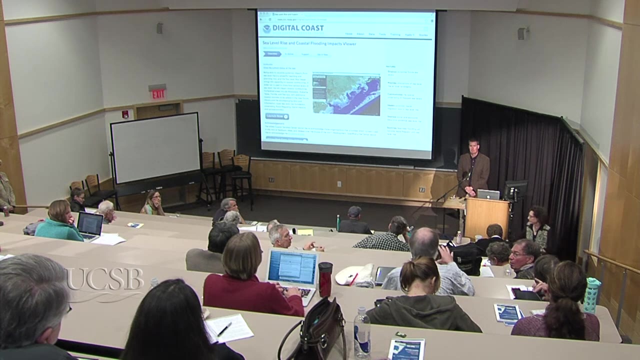 And if you could have a tool that would show those the line for each sea level rise, then people could see what property is included. Because the other thing reaction I had is it looks as if a lot of the time the areas that you project to be flooded. 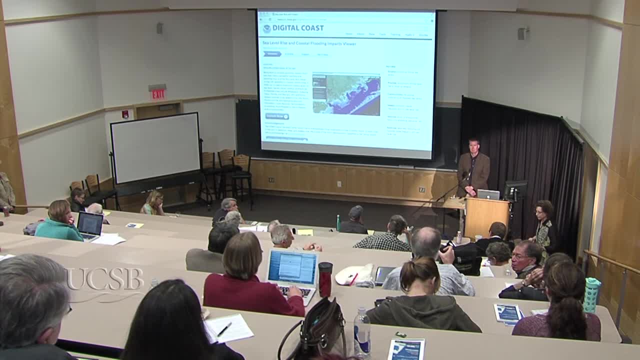 or hit by high tides or whatever. you reduce the contrast, They're sort of blue. They might have some models modeling to show where the buildings used to be, but it's then much harder to see the buildings that are lost. So the eye goes to the buildings that are high and dry. 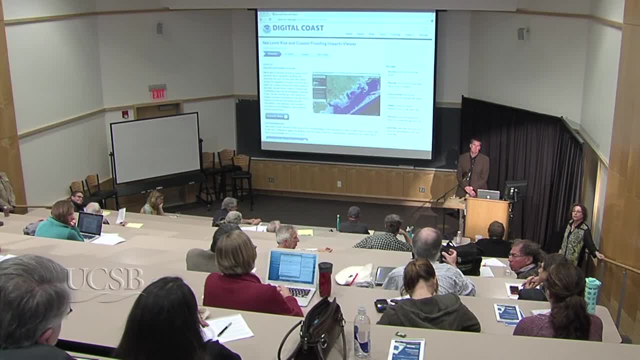 which are not the problem. If maybe, instead of reducing the contrast, just switch the color so you've got brown and white inland and blue and white in the flooded areas, then it's much easier to see. okay, that's the airport, that's my house. 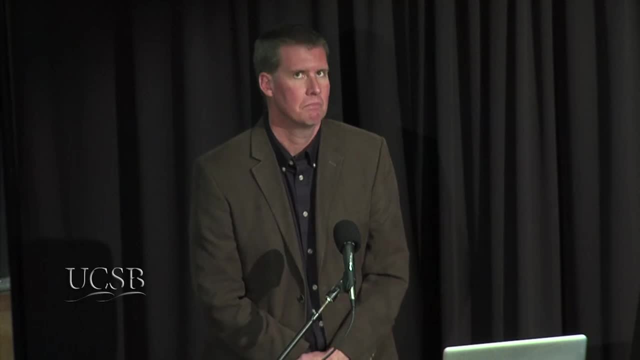 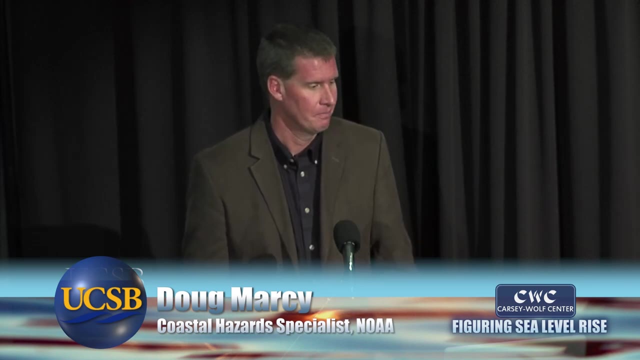 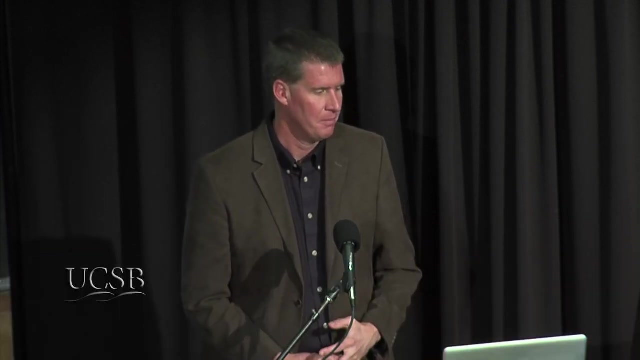 that's the UCSB campus. So yeah, absolutely, that's a good point. You know, the funny thing about colors is we agonize over them sometimes and then it's like you can never make everybody happy. My, when we first started doing this. 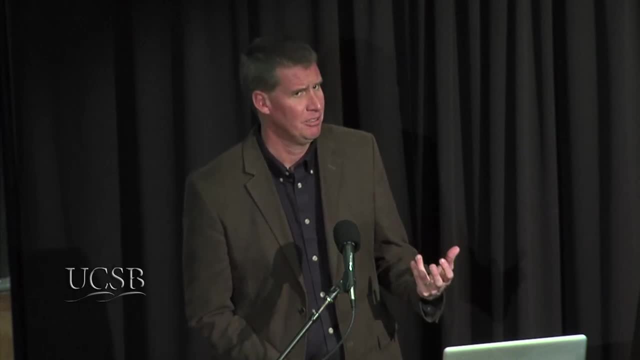 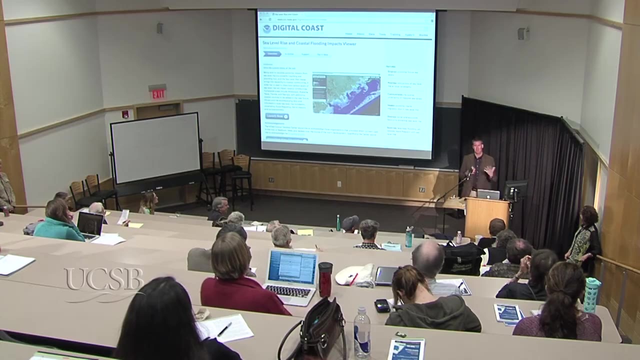 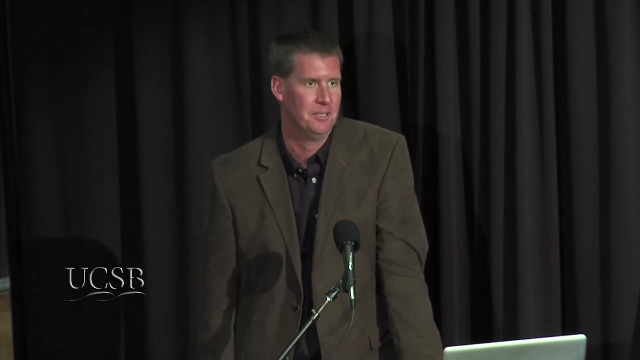 well, we shouldn't do this. water doesn't look that clear. It should be brown water, right? So yeah, especially storm surge, It's not nice pretty blue Caribbean water, so But that's a good point. Yeah, it does cover up what is actually impacted. so 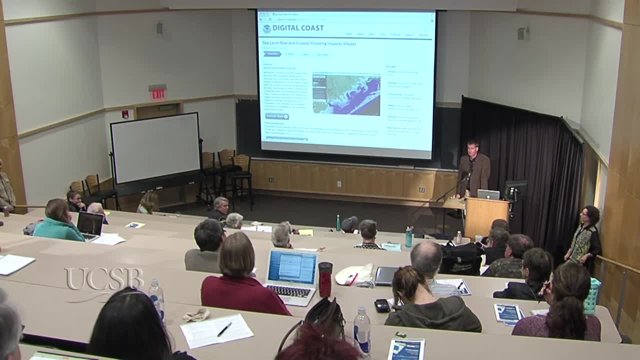 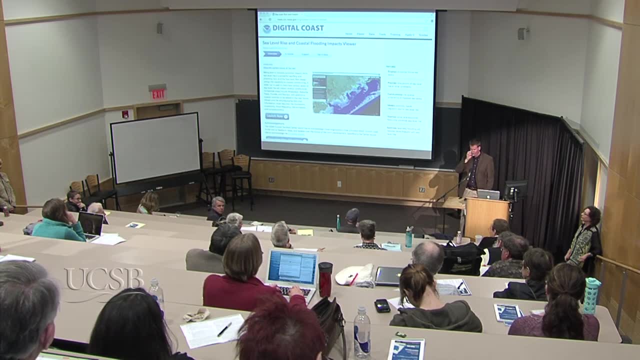 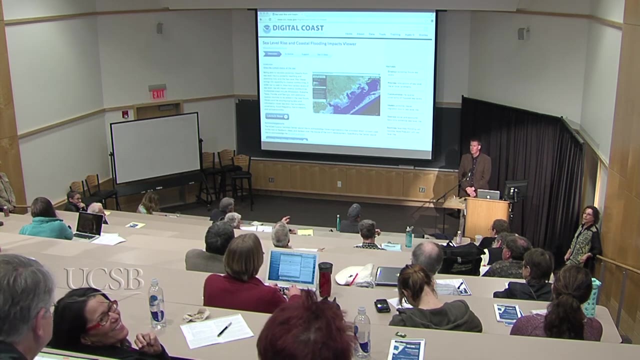 I wanted to come back to the impact of Sandy Watershed. moment pun intended. I grew up in the area that you were showing in New Jersey, Long Branch. The good news that was, my childhood home was out of the danger. It was on fairly high ground. 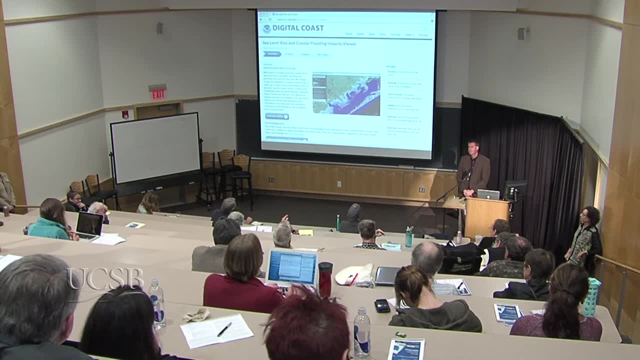 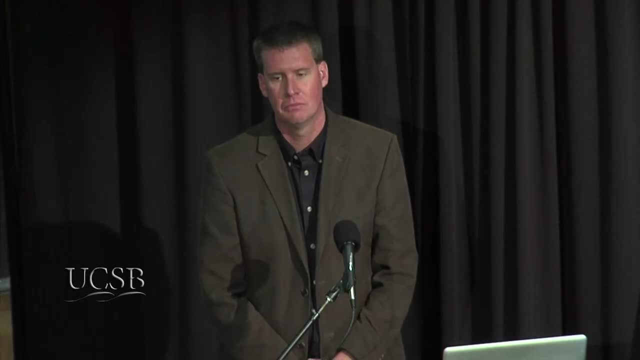 But the bad news was that my cousins they had a restaurant which was the largest restaurant anywhere in the area. it was in Asbury Park and it looked like he might have real trouble. So what I wanted to suggest and do, I'll email him some information. 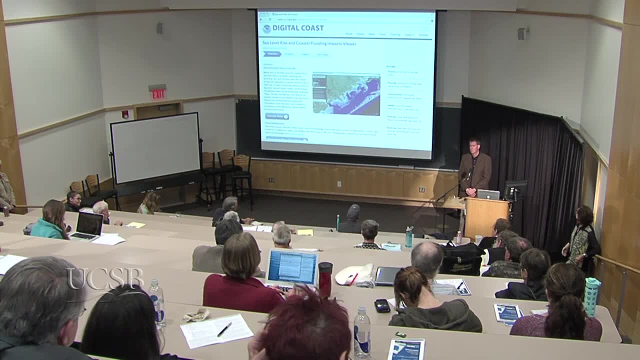 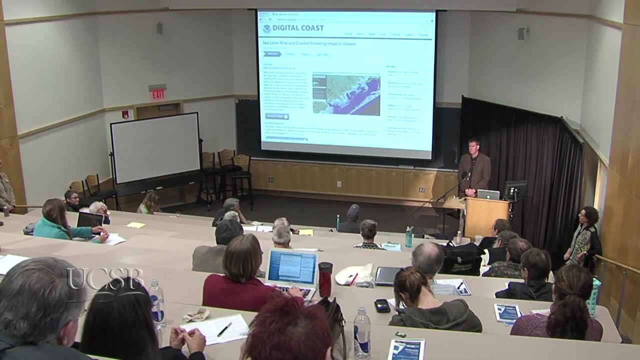 He can plug in the address of that restaurant in Asbury Park and tell his friends. and you know, the business community, it seems to me, are the people that need to get busy on this. I don't have a restaurant, I could care less. 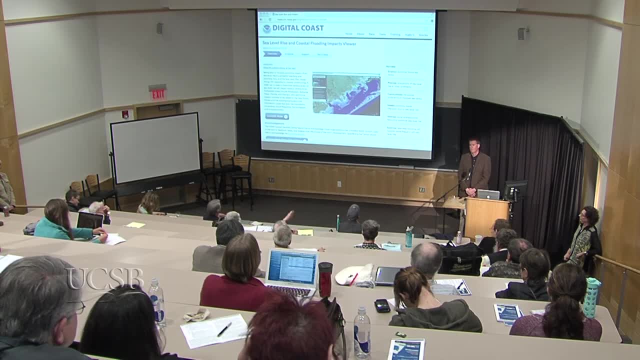 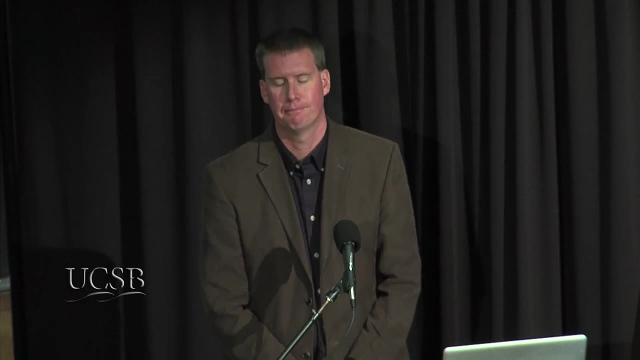 Where I am, the land is rising, But that whole area is just full of businesses, small businesses, tourist industry, and once they get onto this picture, I think you'll get some public action outcry. So I would just suggest that that's where the outreach. 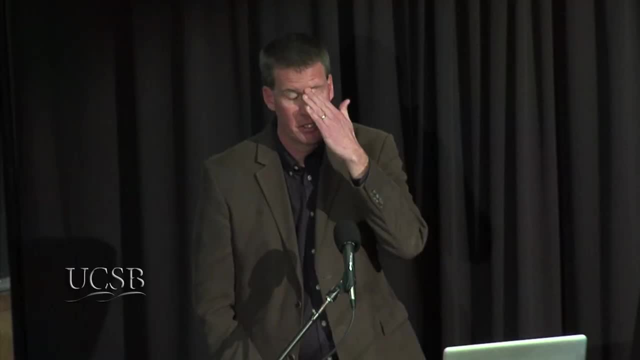 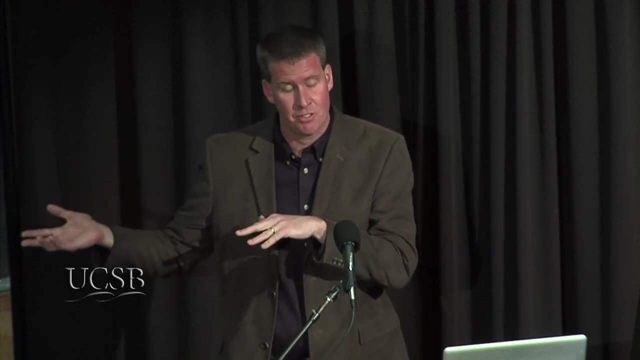 needs to go to that business community And you know, and the carrot it really is with the flood insurance program is that if they build back to these advisory-based flood elevations, they're eligible to get hazard mitigation grant funding to do it. so, in other words, if you're gonna build back, 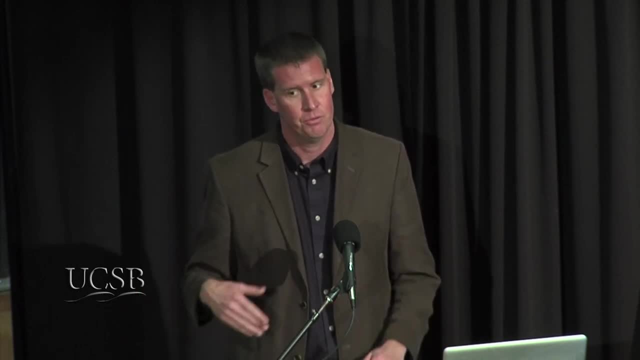 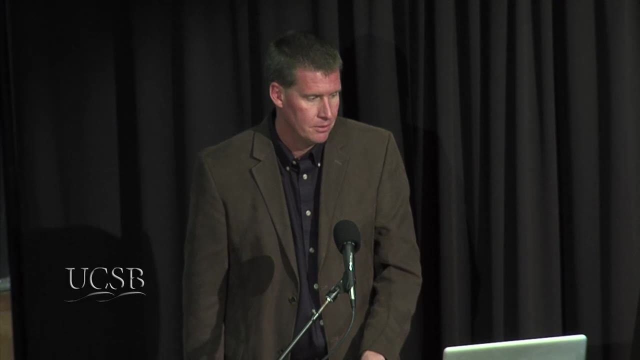 to your existing elevation, you gotta do it on your own. If you want government help, you need to build back higher, And that's definitely a good thing. So yeah, and that's the thing about the flood insurance program, and I agree with you adding sea level to that. 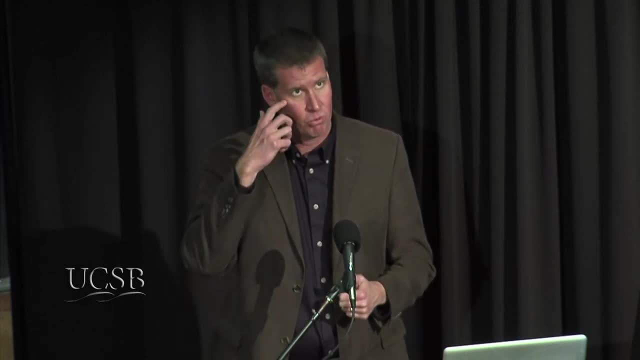 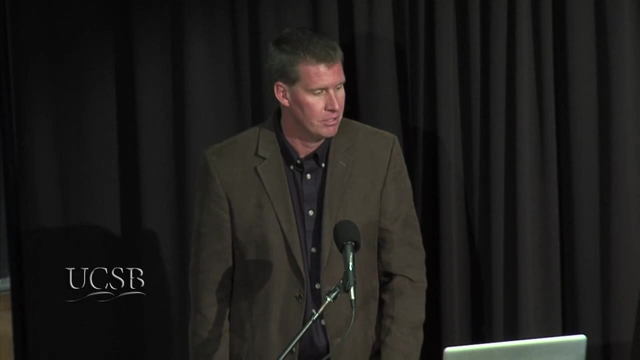 And so this is the first time we've tried to do it and FEMA's very interested in trying to work with us to do this- not just advisory maps, but the effective maps other places and start doing this, because I agree with you. 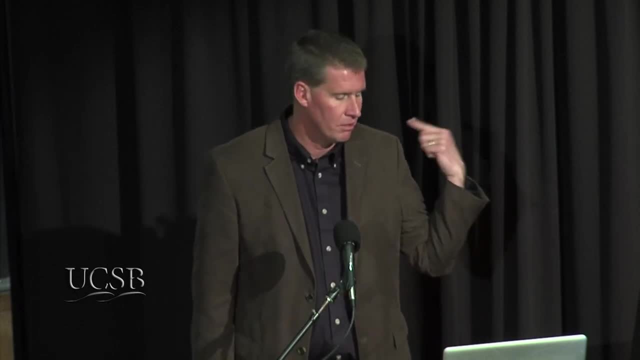 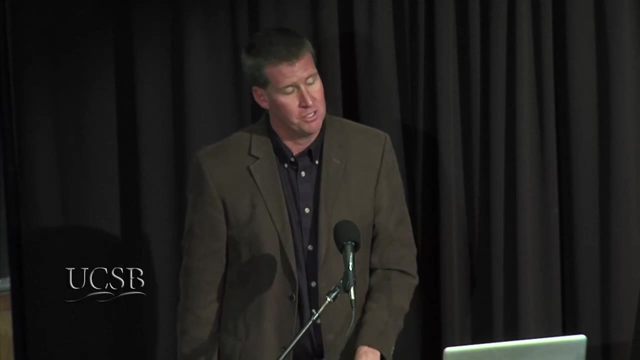 it's the only thing that you can show the viewer all day, but it's the only thing that has regulatory teeth, so to speak. for people it hits them in the wallet. you know, if you get a mortgage and you live in the flood plane. 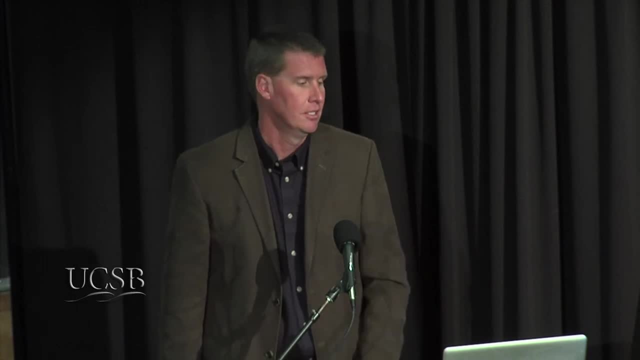 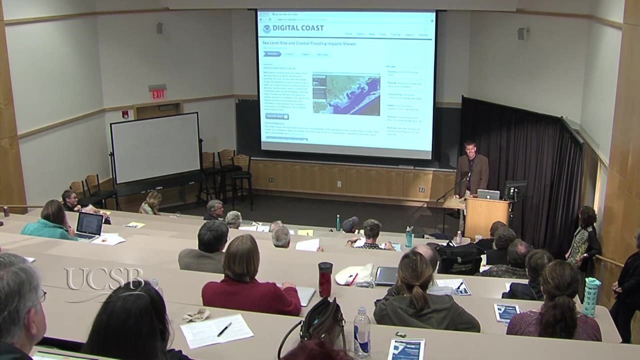 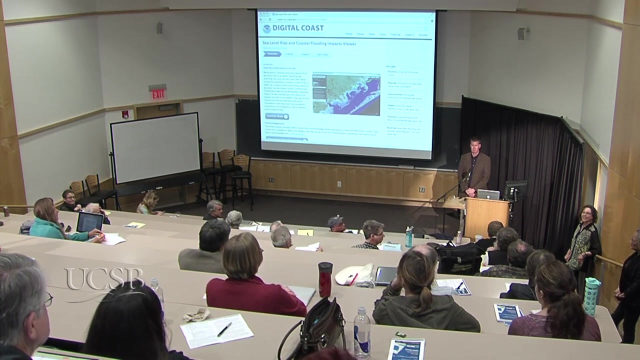 you have to pay, you have to have flood insurance. The bank makes you have to have it. So then you start paying attention a little bit more. When it hits you in the wallet, people pay attention. I grew up in New England and sort of the benchmark. 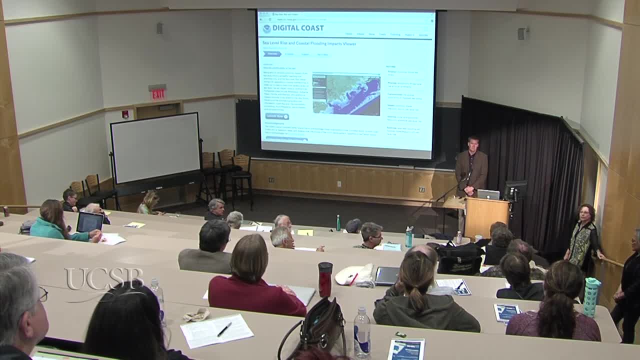 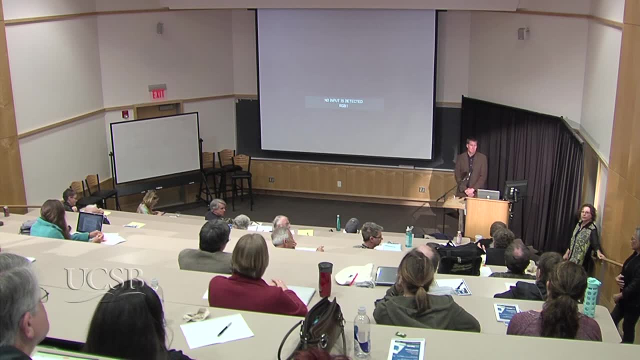 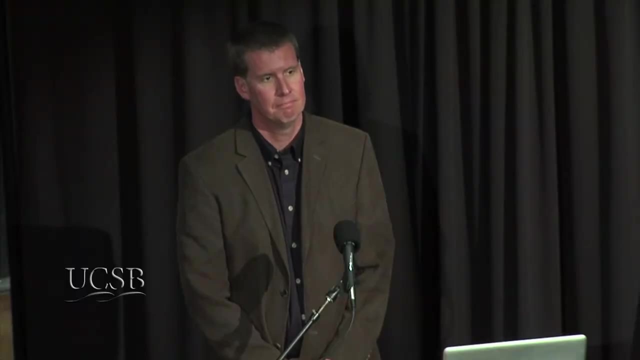 by which we always measured. really bad news in the fall was the 1938 hurricane, And the 38 hurricane was much more limited in its area of effect than Sandy but, I suspect, much more powerful, And I think about the tremendous damage that that did along the coast of the Long Island and Connecticut. 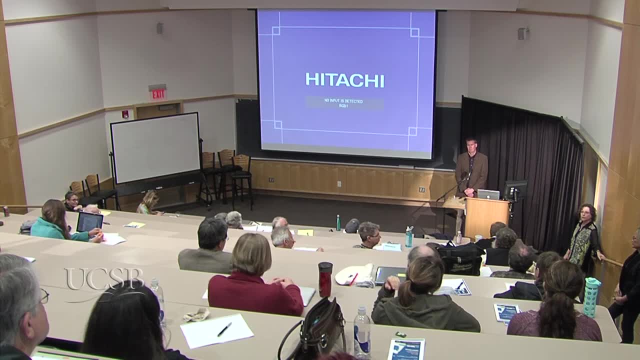 and wonder if one, because people are sort of looking at Sandy as the worst case scenario. It was a big storm, It was a huge tide surge. It wasn't a powerful wind event pushing the water with it. If one could go back and from the records of the 1938. 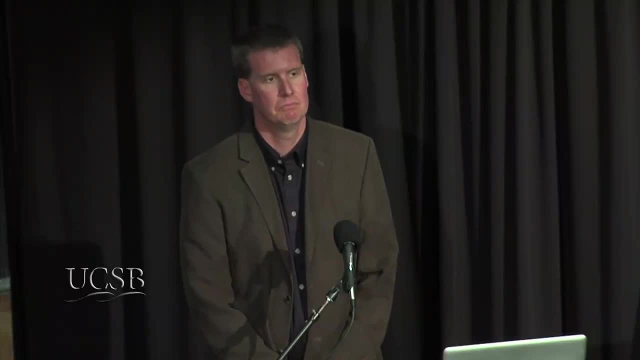 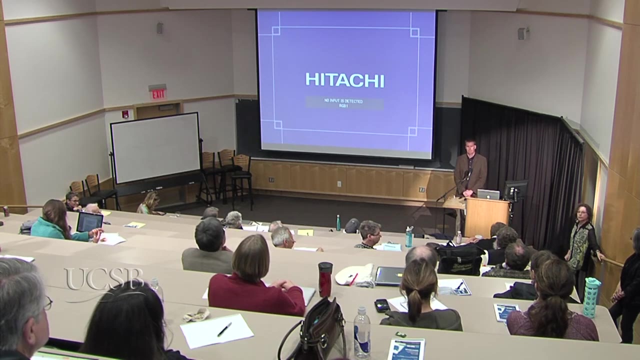 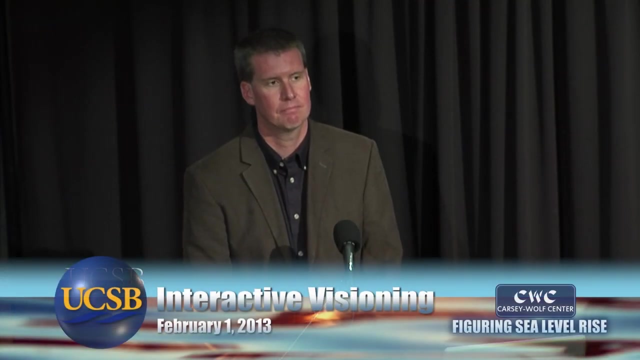 hurricane. look at the high water and that particular limited area, see how much higher it would have been, and build in your sea level rise, thermal expansion, everything else, and come back with a model here which is not simply sea level rise. one foot one, two foot, three foot. 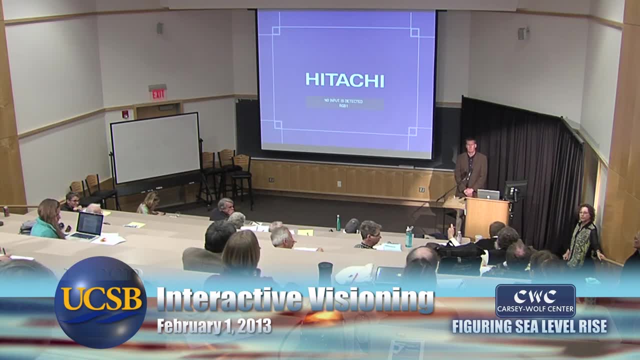 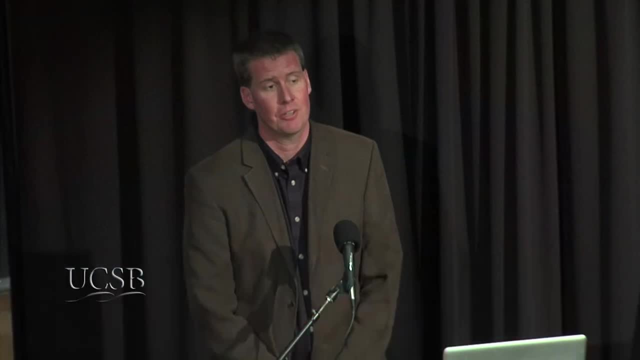 but sea level rise and one of the worst case scenario- hurricanes we've seen, and then back model that on other places on the East Coast to say, hey, you guys think Sandy was bad, You ain't seen nothing yet. Right, That's exactly right. 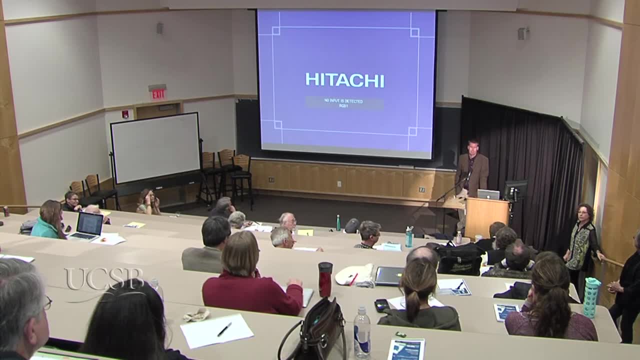 New England has forgotten about, or most people have forgotten about, that moment. This is my opening. I said the problem is Sandy. people are going to put into their local mythology and forget about it. Only if we get a Sandy a year will they start to believe it. 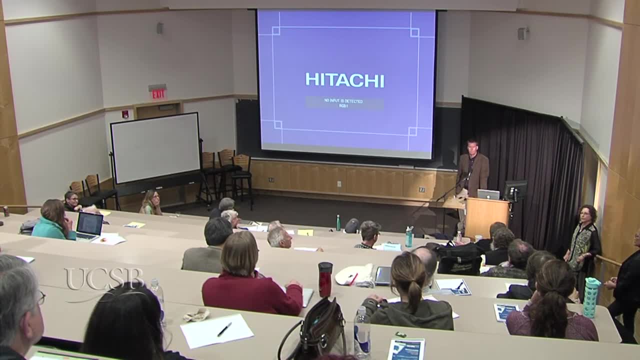 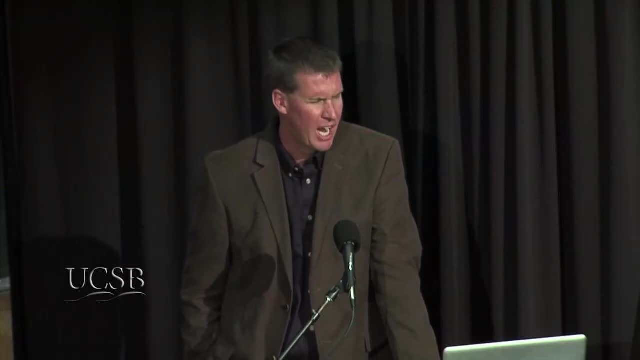 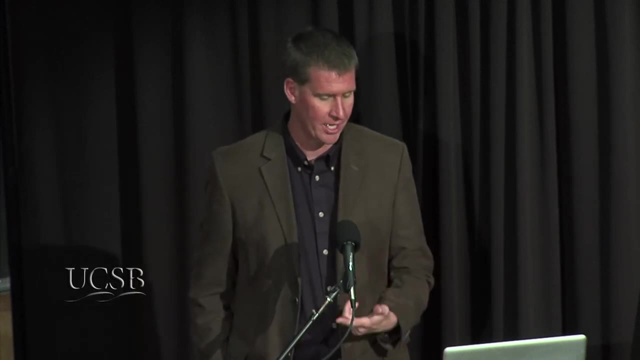 How do we save them the difficulty of having to suffer a Sandy a year to get them to believe it? Yeah, that's exactly right. The Long Island Express. that's what they called that storm, right, the 1938 hurricane. Yeah, I grew up going out to Block Island. every summer for vacation and I always hear stories. I used to have a really thriving fishing community fishing fleet out on Block Island, But after the 38 hurricane it just wiped them all off, wiped them out, and they never really came back after that. 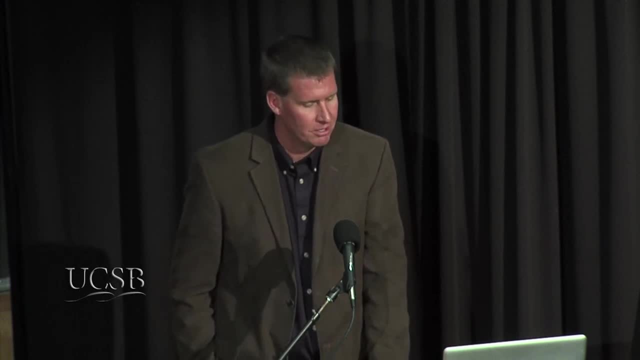 There's other places that have that same problem with memory loss. I was a freshman in college in Charleston in 1989.. That's when Hurricane Hugo hit And everybody says, oh well, we survived, Hugo, That was really not that bad. Well, downtown Charleston only got 10 foot of storm surge from Hugo. Most of the wind was north of Charleston And the worst surge, 20 feet, was in an area that really nobody lives in. It was actually a wildlife refuge. So you take that same storm and move it just a little bit. farther south, it could have been much, much worse. So people think they lived through it. That was a problem with, I think, Camille. A lot of people say that Camille actually killed more people than Katrina, because people say, oh well. we lived through Hurricane Camille, no problem. But Katrina was just a different animal, It was a different storm. The only problem with individual storms like that- hindcasted storms, if you will, and adding- is that that storm will never happen again. 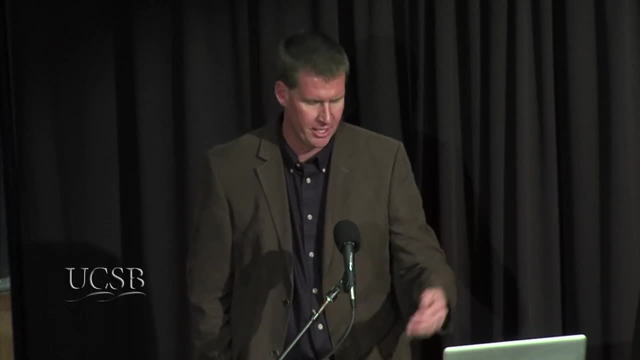 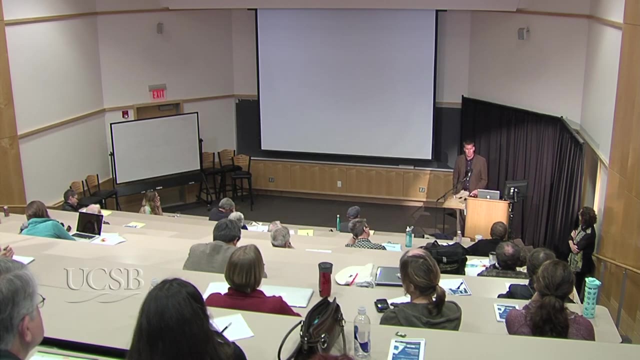 That particular inundation footprint. if you will, from Katrina or the 38th storm, every storm's different. There's always going to be some other factor that's not going to produce the same inundation, So you're always going to have someone. 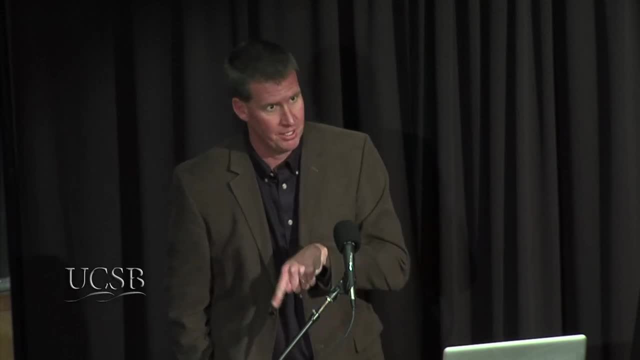 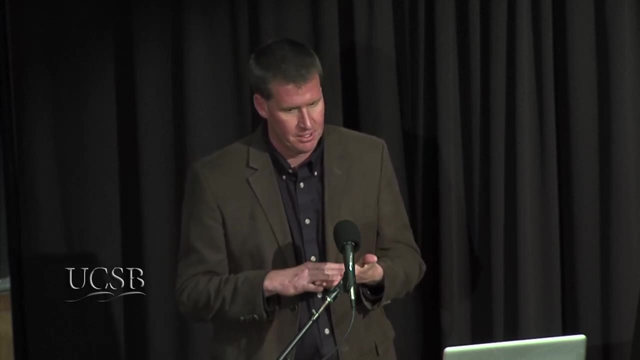 that wasn't impacted by that storm, that will be impacted by the next storm. So that's the only problem. That's the only problem with that. So what you try to do is do probability analysis, And this is what the coastal flood studies now try to do. 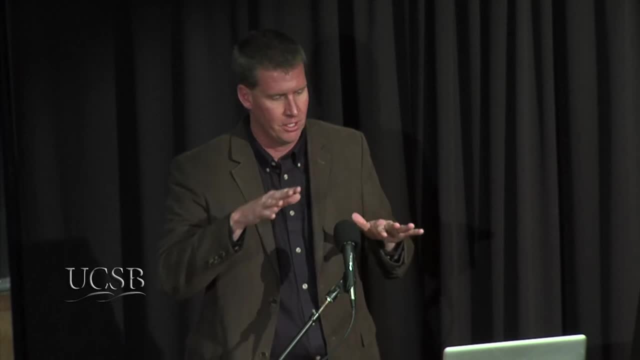 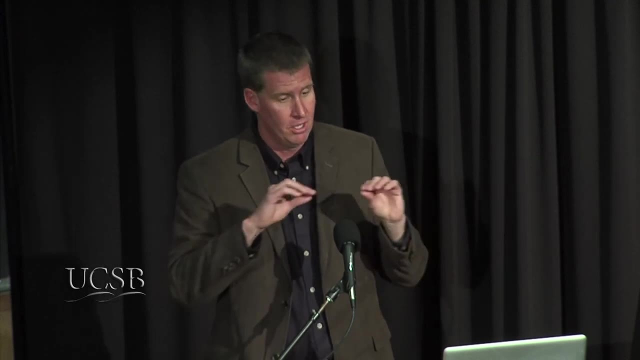 is you mimic all these different paths of storms and all these different combinations of strength, wind, speed and pressure and all that, and then try to come up with an ensemble, if you will, of the possibilities and then do a probability analysis. 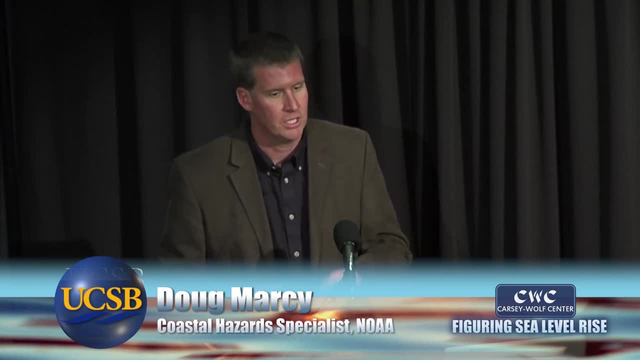 of the 1% chance, which is the 100-year storm, would give you this amount of water, So you sort of get the most out of it. That's the most likely scenario. That's how they try to model these things. 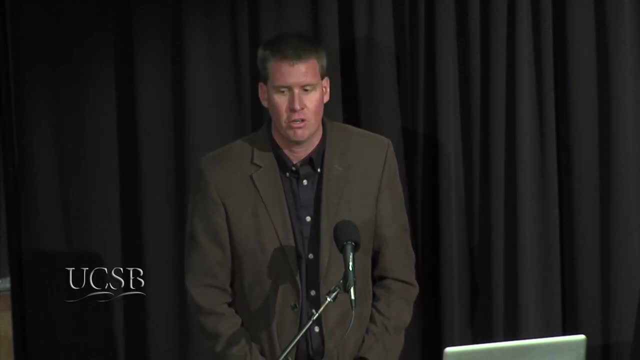 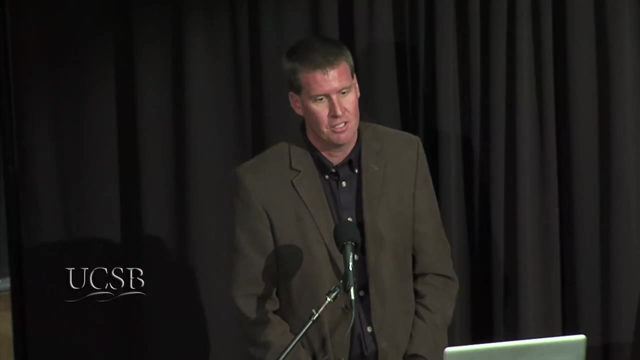 instead of just picking one. So it's hard, though It's still hard. People, 100-year flood. I mean that's something that FEMA tried to steer away from, because people are like: well, I'm good, We had a flood last year, so I got another 100 years. 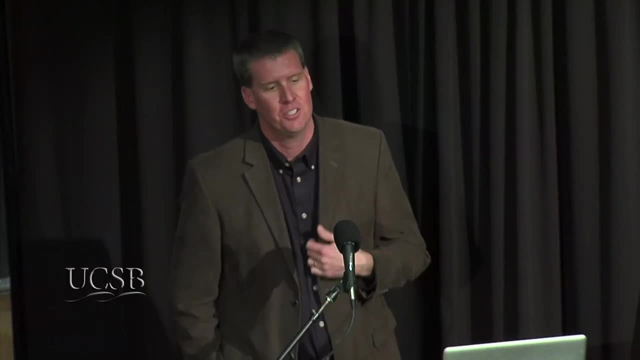 And then they get. well, we just had two 100-year floods in a row, So then they try. well, we'll do 1% exceedance probability. Well, that's great. What the hell does that mean? So 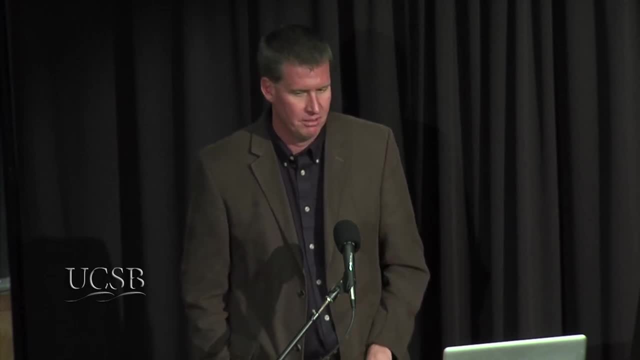 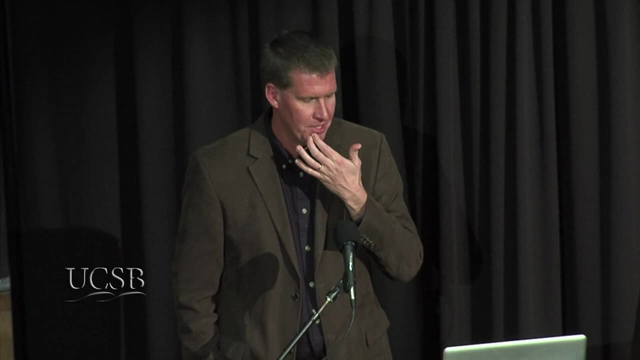 So yeah, it's a hard thing for people to understand. Probability is really people. It's funny because people, it's perception of risk, because I always the folks I work with at the National Hurricane Center. they try to do things in probabilities as well. 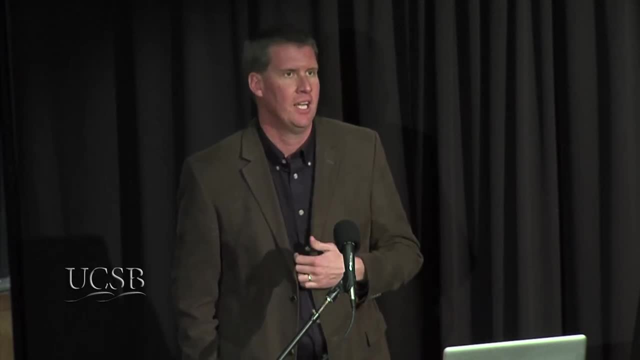 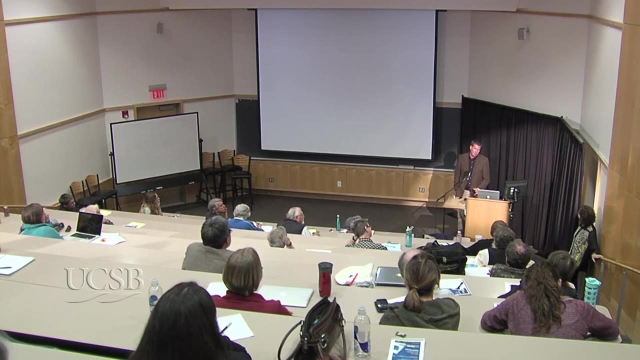 And they try to communicate it like: well, OK, let's see If you had a. there's a difference: 30% chance of rain. are you going to bring your umbrella? Are you going to wear a raincoat? Most people, it might rain, it might not rain. 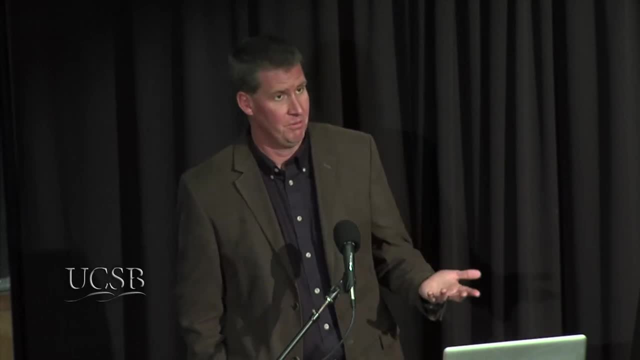 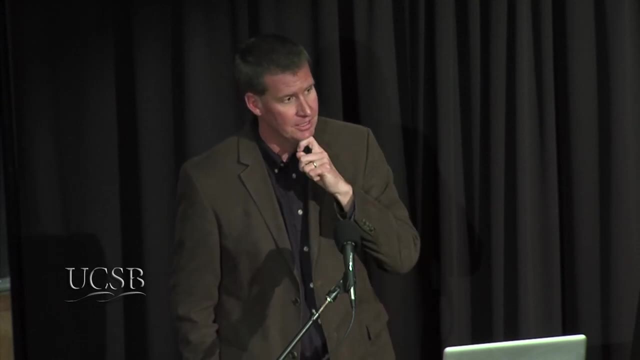 But it's the. it's what you have to lose. If you're wrong, you get wet, But if you have a three- if someone told you you have a three in 10 chance- you're going to get hit by a bus if you cross the street. 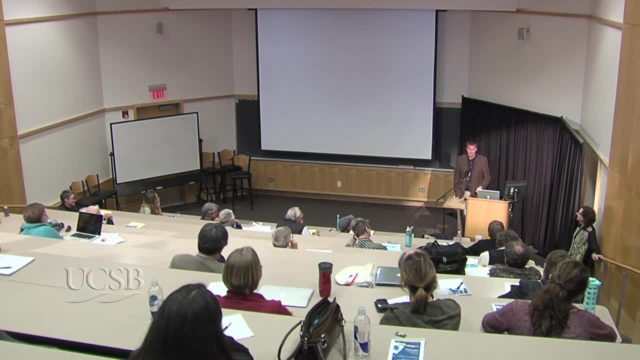 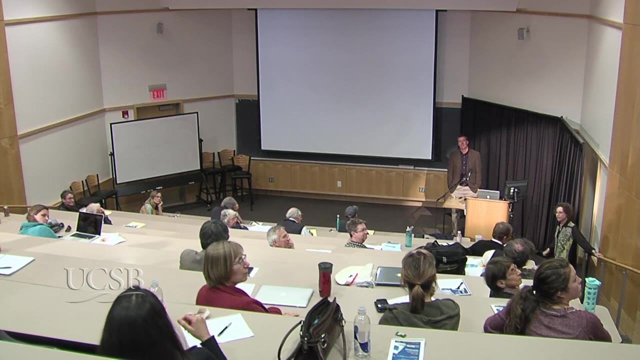 would you do it? So there's a big difference, right? So there's that whole perception of risk, that kind of that's a long answer, but Tied into this, we sort of ask: will Sandy be the watershed event that actually changes attitudes? 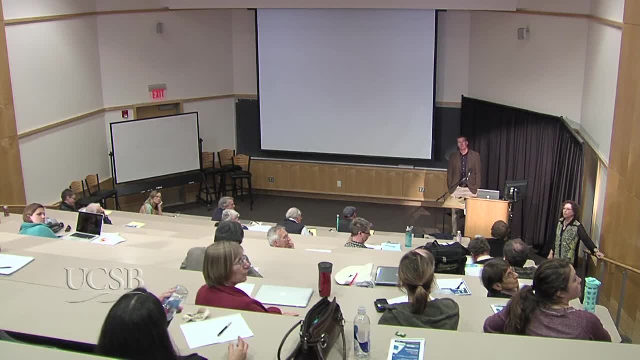 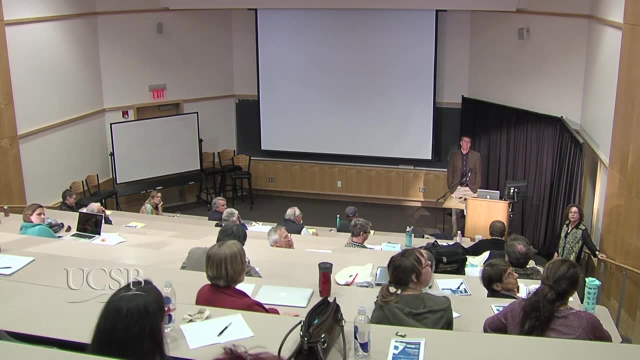 And I wonder whether you think that such events really have that power, Because I look at Sandy Hook, for example, and I don't believe that's going to change gun laws anyhow, despite the shock, outrage and upset that it invoked at the time, in part because of people's 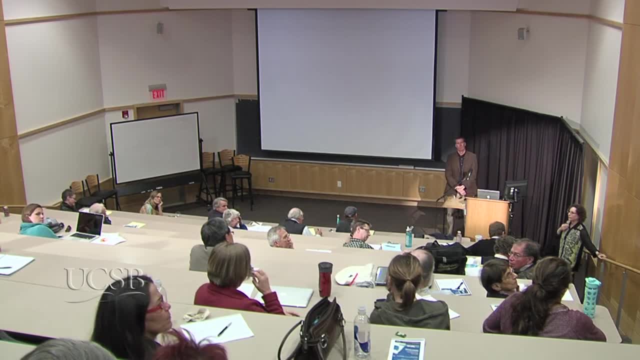 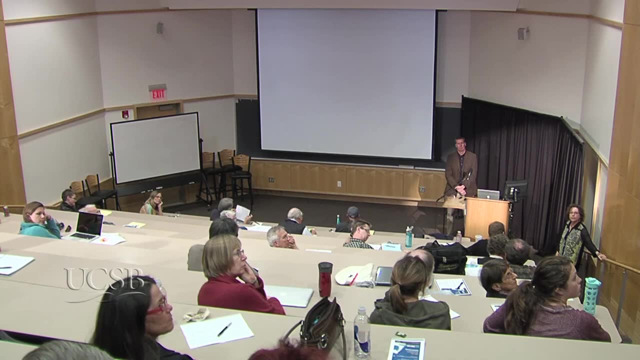 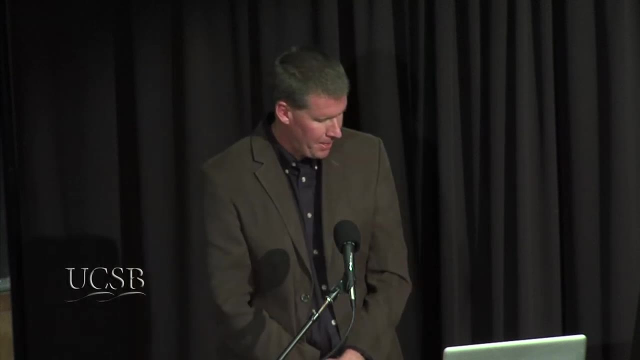 memories and in part because of counterbalancing forces that have more durability. So do you think these kinds of big events really have much power in the climate and the sea level? I think that for public perception I don't know, because they're on to the next thing. 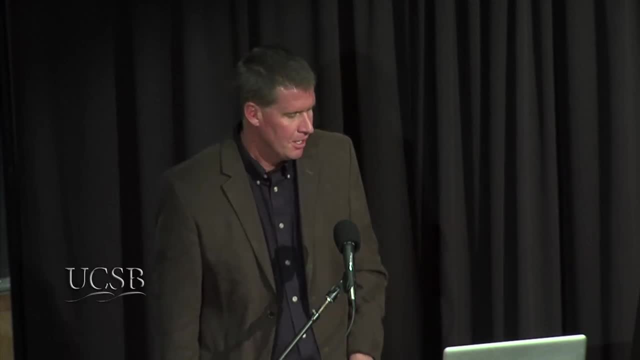 like what's Kim Kardashian doing or something. But I think where it makes a difference- and we've seen it like Hurricane Andrew back in 1992, they made some significant changes to the building codes in Florida because of that. So they really changed the wind code. 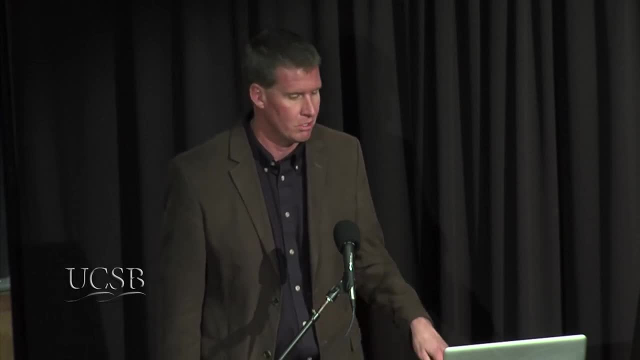 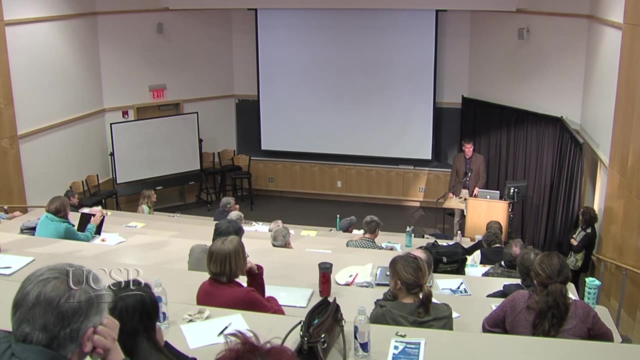 and so the buildings are built stronger. So these events do cause changes in regulations that do make a difference when it comes to building more resilient structures. So I think, in that sense, it's a hard lesson for us to learn, but we do change. 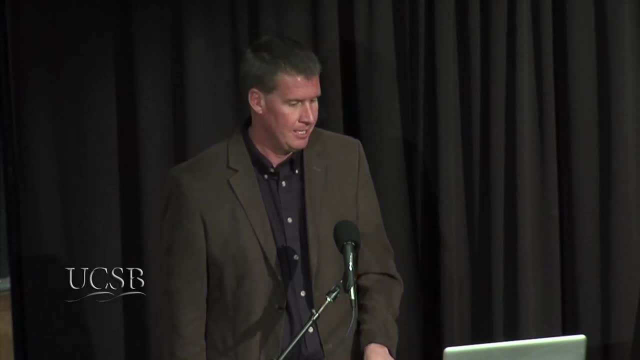 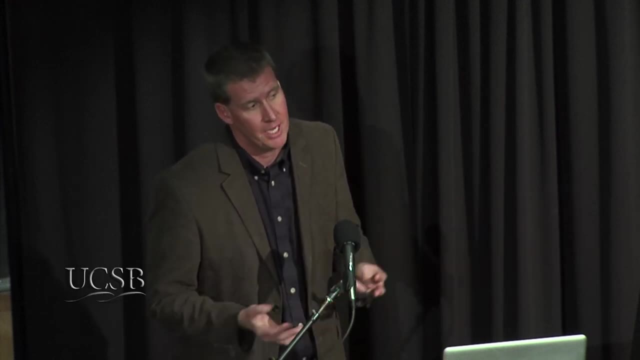 It takes us a long time to do it. What might happen with Sandy is that we do come up. maybe this does go somewhere and we have advisory information on the flood maps now or something like that might come up. I've worked in the government for like 12,. 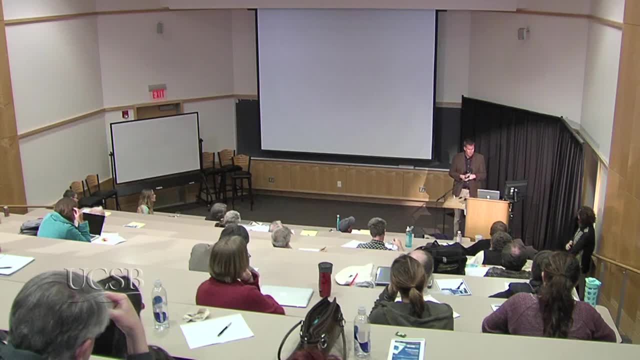 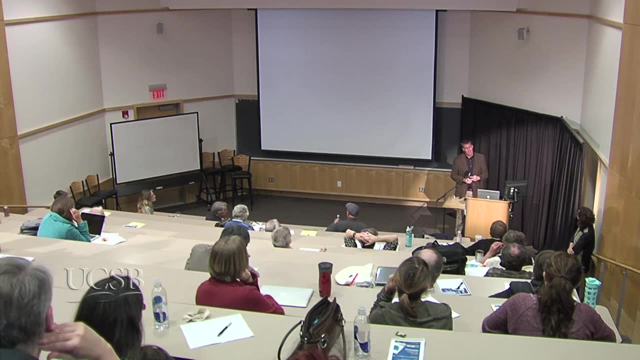 or about 13 years now, And so we have this expression: we're not fast, but we sure are slow, So and we're not cheap, but we sure are expensive. So it does take a long time And sometimes these events, it's reactionary. 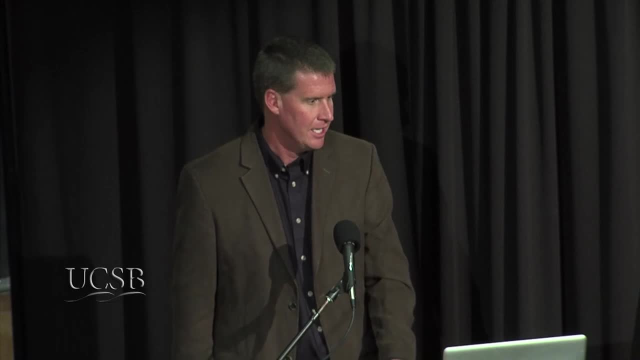 If you look at a lot of the laws we have in the country, it's always some issue that caused it: the Disabilities Act and all these other acts and a lot of the women's rights. It's all because of some events that have happened that eventually change it. 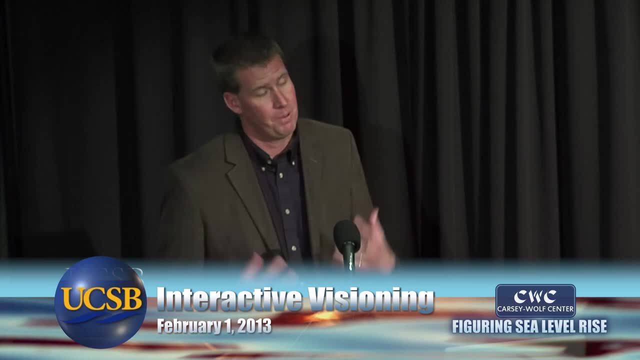 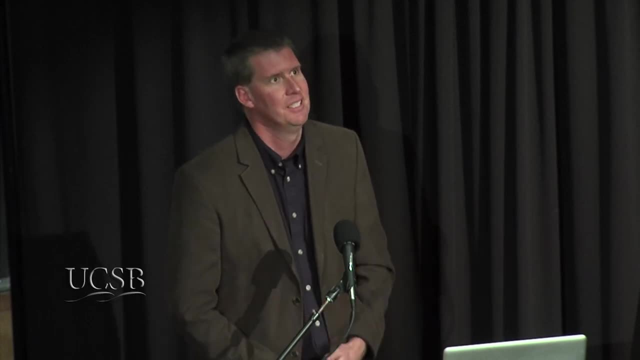 So I do believe that's the case in this one. Now, general public awareness and the gun law thing, I don't know, That's kind of outside. Yeah, It is yeah, But I mean I think we suffer from information overloads. 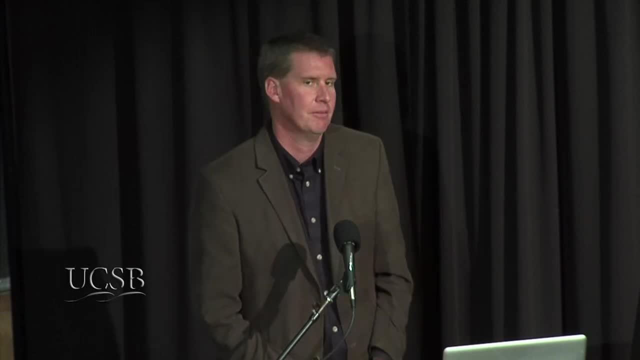 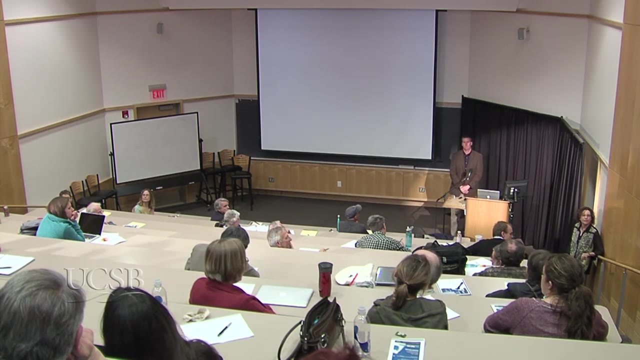 So people are on to the next thing. If it didn't affect them, they're like: well, it's too bad for those people, but I've got my life to deal with. So Thank you. Besides your engineering background and your work with the Army Corps, 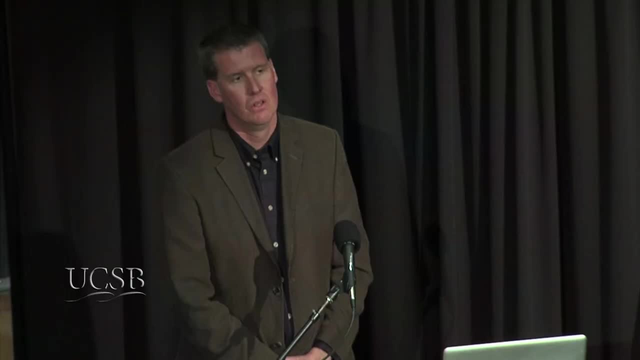 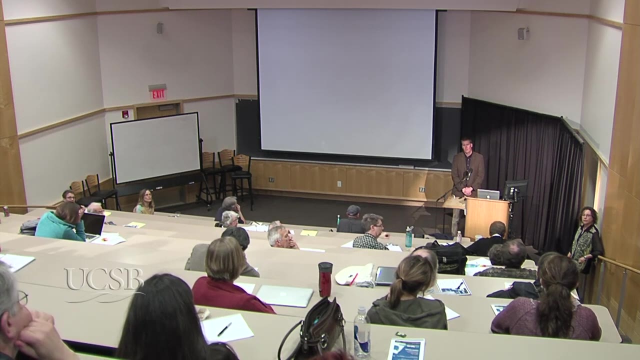 you've been working on this modeling stuff with information display for a long time now. With these two most recent reports that you referenced, what are the single one or two things that surprised you or that you found most interesting in the most recent data sets that you've seen? 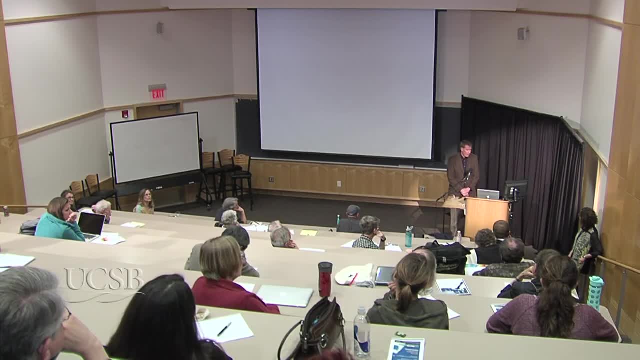 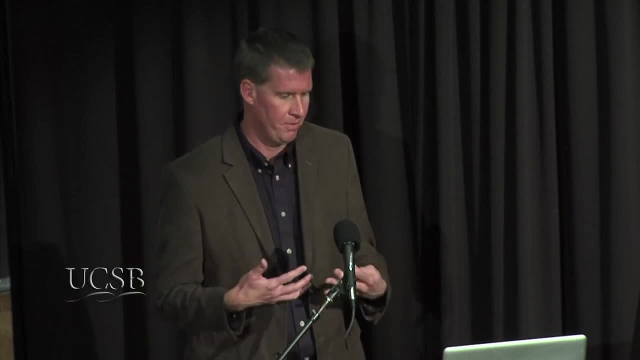 The sea level rise reports you're talking about. I was really surprised that. well, for one- and Jeremy can attest to this when he talks- I mean for an integer agency group to get together- and the climate assessment made this happen- but to agree on these four scenarios. 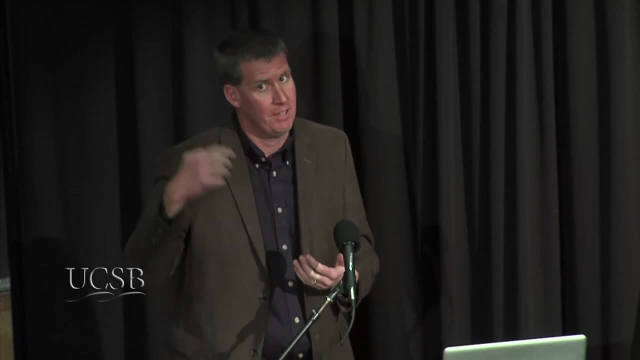 I never thought that was going to happen. And the fact that the upper end of that scenario really does take the rapid ice melt scenario into account and it's a 6.6 foot rise by 2100, I thought, oh Yeah. 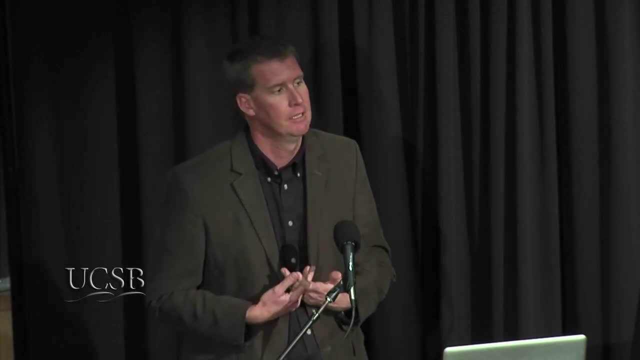 Yeah, Yeah, Yeah. No way the government's going to put out a number that high. So that really did, and I'm proud of that group because that's maybe a risky thing to do at that time, but I think they stayed true to the science. 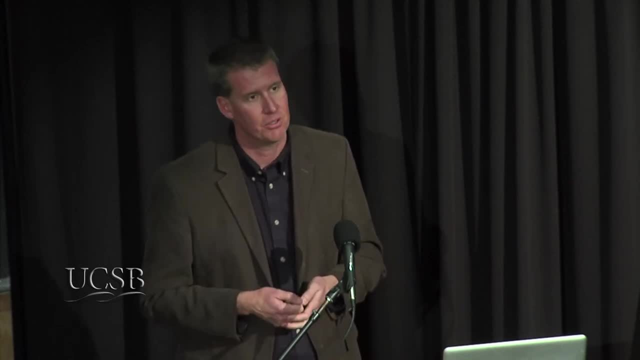 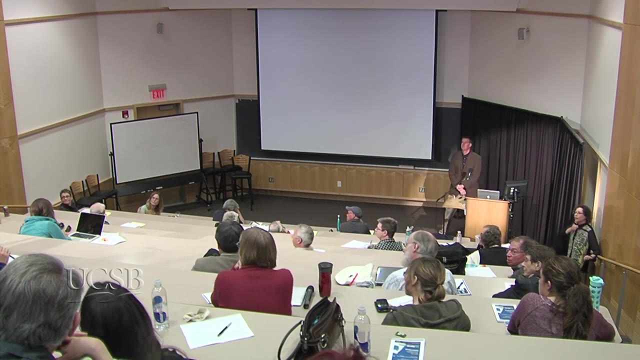 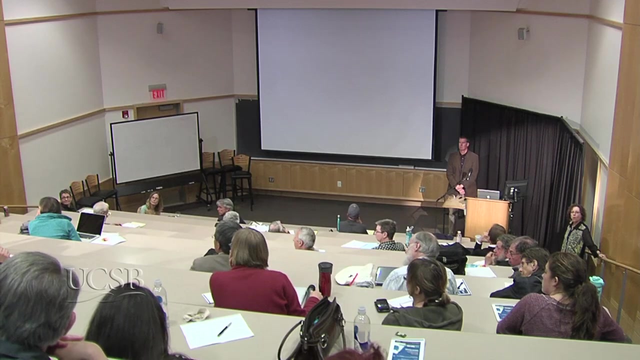 So that answers your question. Yeah, Thanks for your talk. I have a question about. I really liked all of the different layers of data that you showed and being able to link things. I think it's powerful, especially visually, And you also mentioned that you thought. 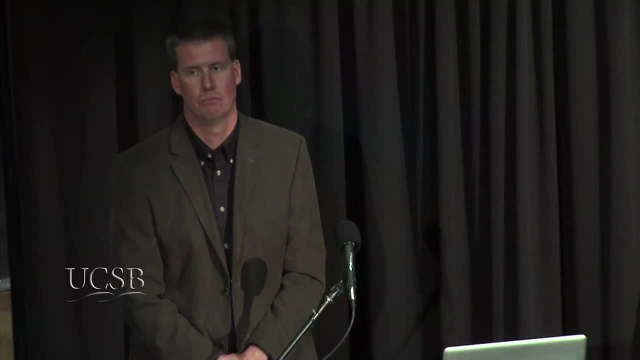 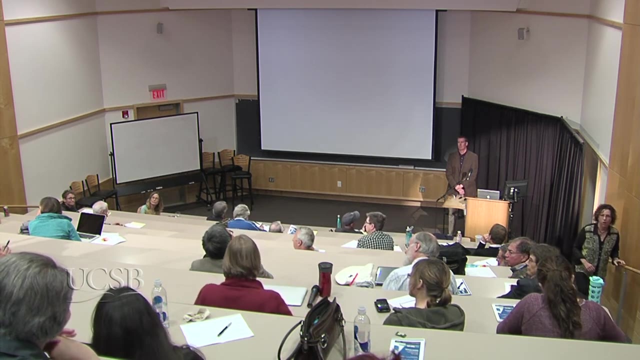 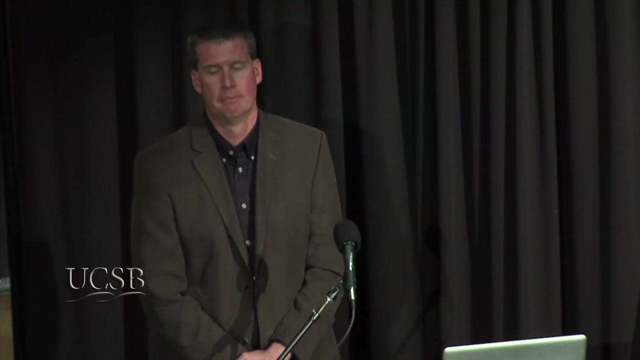 that hitting someone's pocketbook is the best way to go. So, as you present all these different images with these different levels of impacts, are there at least an impetus of some sort to? you talked about insurance, having to get new insurance and whatnot. 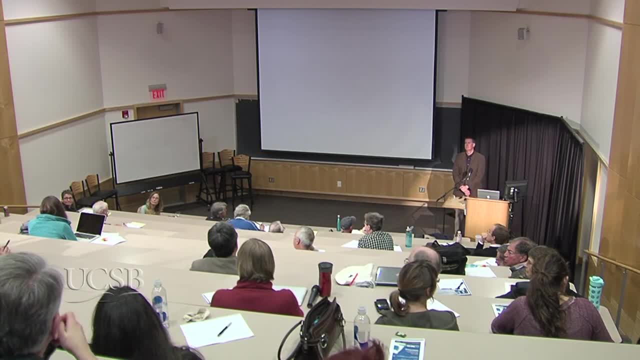 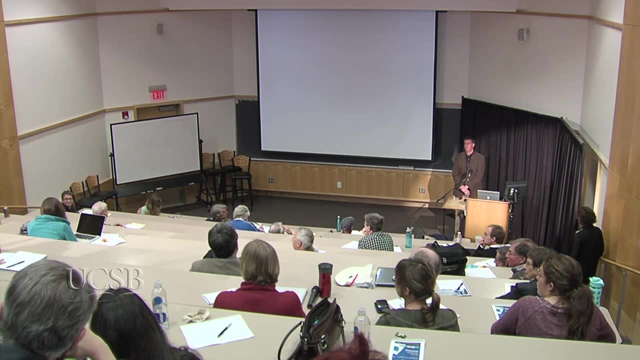 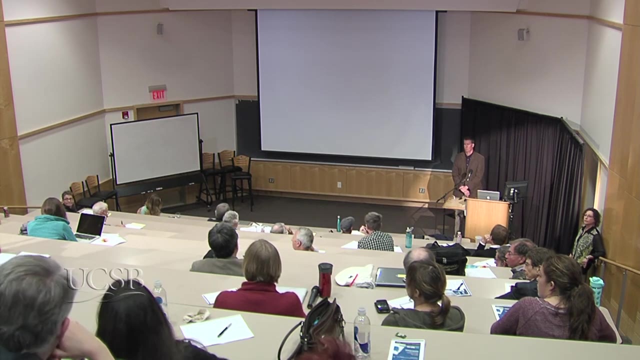 And if you don't get insurance and FEMA has to come in, there's obviously a lot more cost, And so So, whether we have more billion dollar storms or just more billion dollar things, is this the type of tool that the government could use to think about those costs? 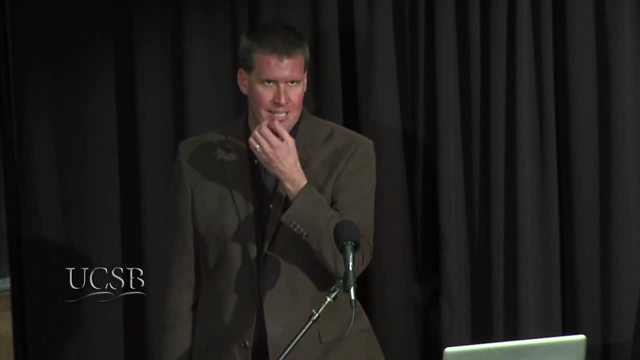 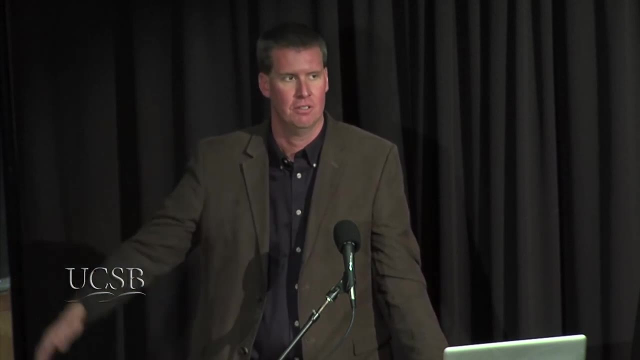 Yeah, The next phase of this, or the next obvious step, would be to do an analysis with these layers and then figure out, well, how much infrastructure is going, actual, real numbers, because that's what politicians want to know: how much infrastructure. 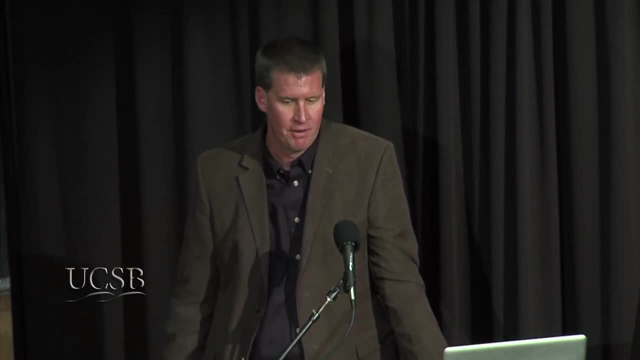 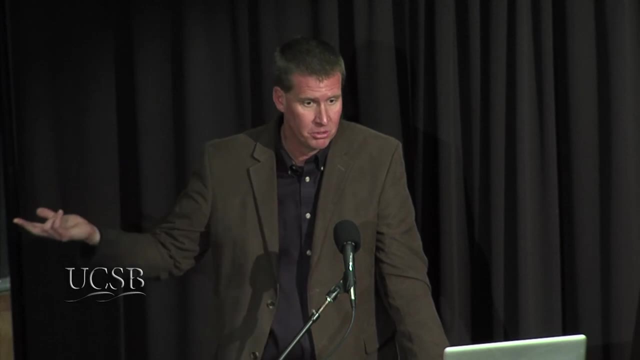 is going to be impacted, And so there's a lot of efforts. As a matter of fact, I'm disappointed Michael Lemonick couldn't be here because Climate Central is actually working on. they have a similar tool called Surging Seas. you guys may have seen. 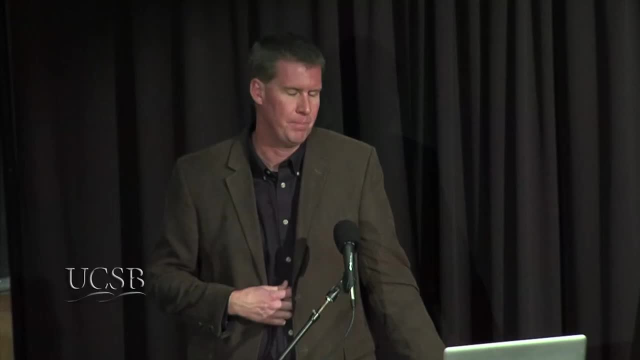 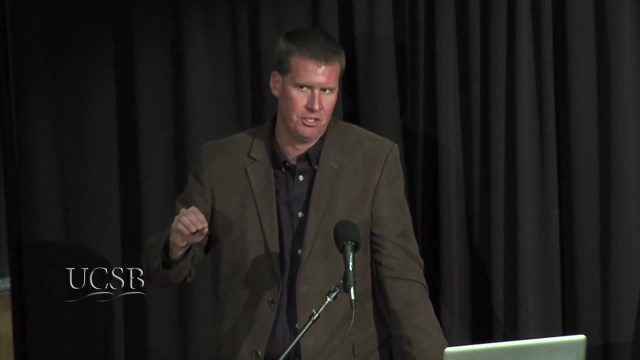 And he's got some Kresge Foundation money. His name is Ben Strauss. The guy's doing it Kresge Foundation money. to go and do this analysis was basically take those layers and overlay on census and come up with the numbers. to look at the number, the amount. 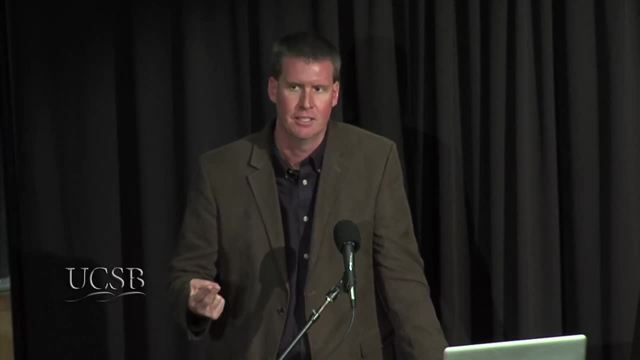 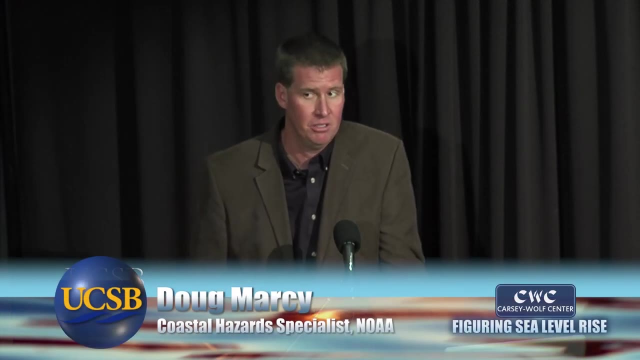 the amount of population, the amount of economic impact. Because that's really again, if you don't do the impact part of the or the consequences part of the risk equation, you're not really doing a risk analysis. So the thing is: insurance companies. 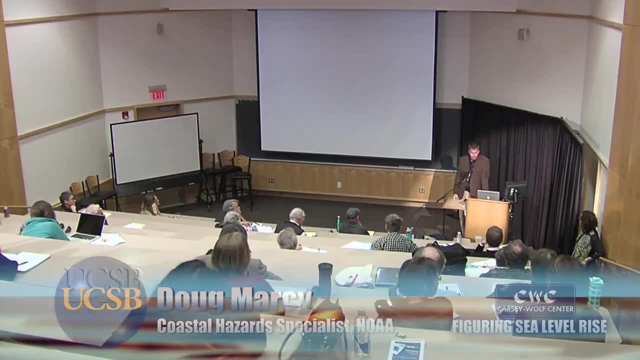 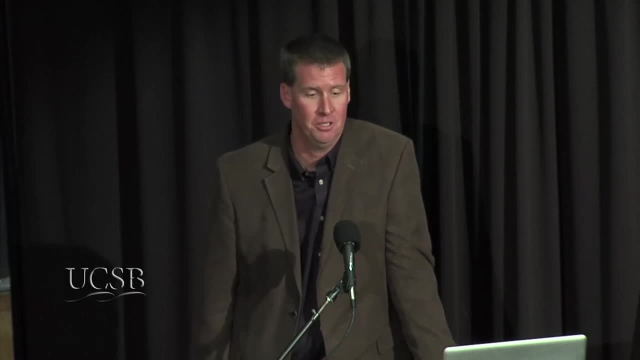 are really good at this stuff And that's how they make their money. And if we could get into their code, if you will. I mean a lot of that's proprietary. They've got this stuff all figured out. They really do. 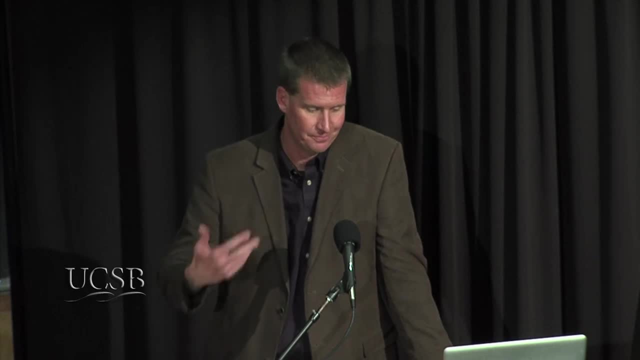 And so, if we could, they could be a little more forthcoming with some of their data. I think there's a lot we could gain from that, But that's like sharing your cards when you're playing poker and saying this is what I got before you bet. 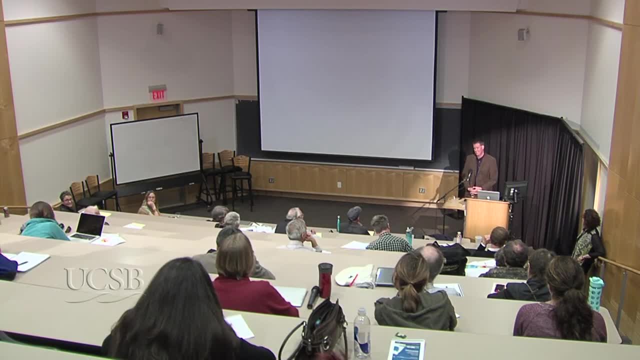 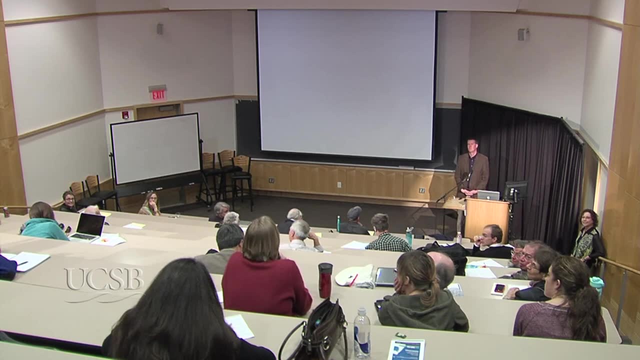 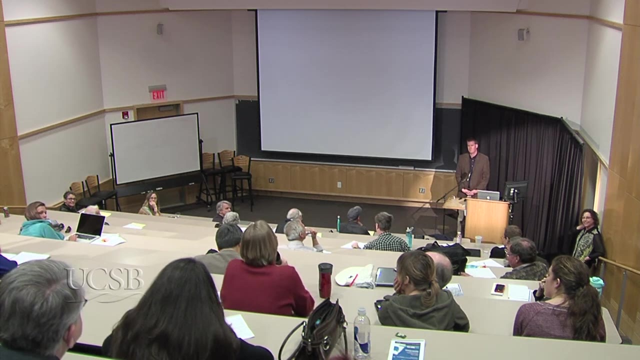 So I don't know if that's going to happen. Does that answer your question? Yeah, I am a risk perception researcher and often take the lone view in these meetings of trying to argue for the sensibility of public jobs, And I think that's really important. 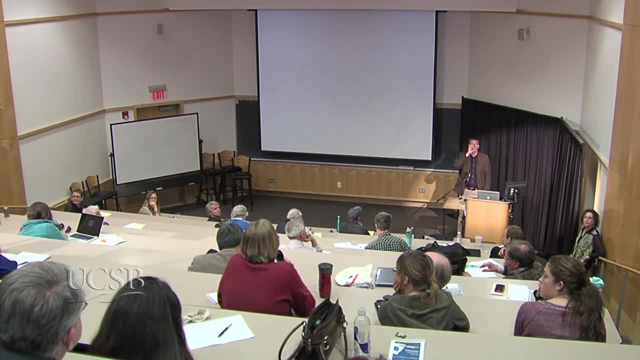 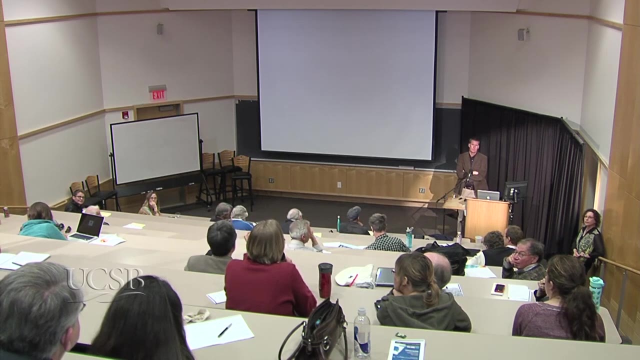 And I think there's a lot of judgment about risk, And so one of the factors that is the biggest driver of risk perception in a lot of technological risk issues is trust, And so, rather than thinking about the sophistication of the models behind the images, I'm 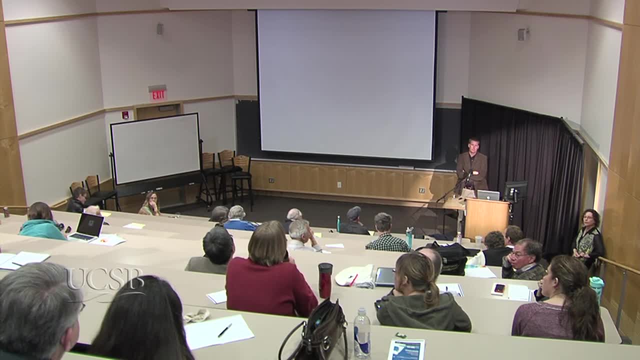 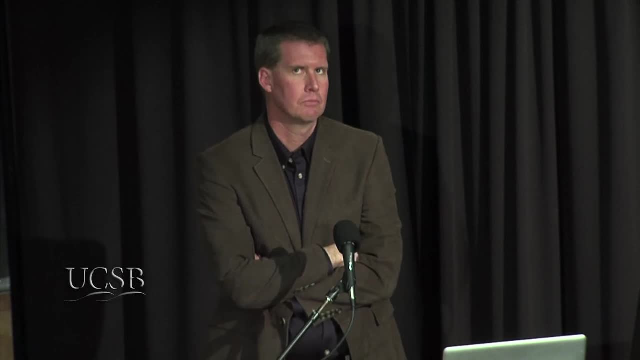 wondering what your plan for building enhanced trust with the public is, which, I would argue, is perhaps certainly more important, and maybe more important going forward. That's a good question. I'm not sure if you did a poll today, how many people would say. 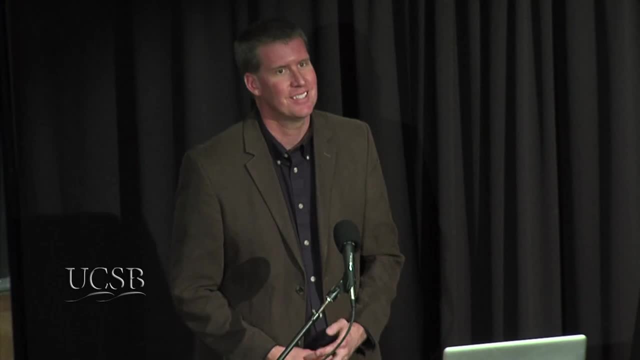 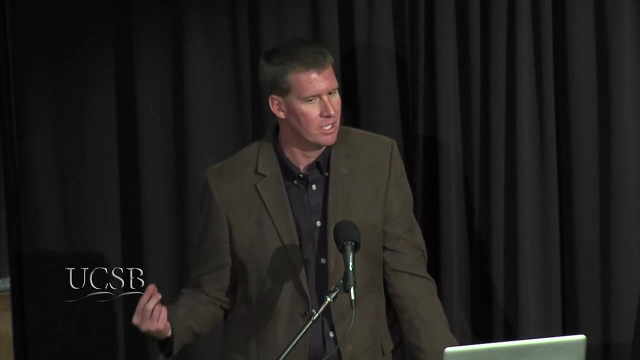 they trust the government. right Is it? And I think for the most part- I don't know, I don't have any evidence or numbers, But I think for the most part we have more flexibility to do this kind of work in an agency. like NOAA, Yeah Than another agency, like a regulatory agency, more like FEMA or the Corps, Because the thing is, with NOAA, we actually don't have a mandate. If you go and look at all the regulations and code of federal regulations that basically started up NOAA. 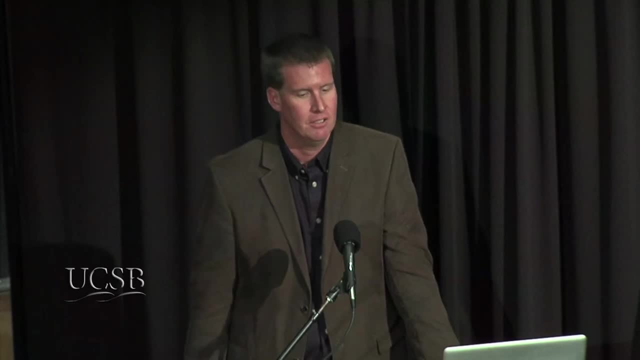 we don't have any authority to do climate modeling, We just do it And we sort of have become the agency that does that. and the weather prediction: We do have authority to do weather prediction and other things, But I think maybe we have more flexibility. 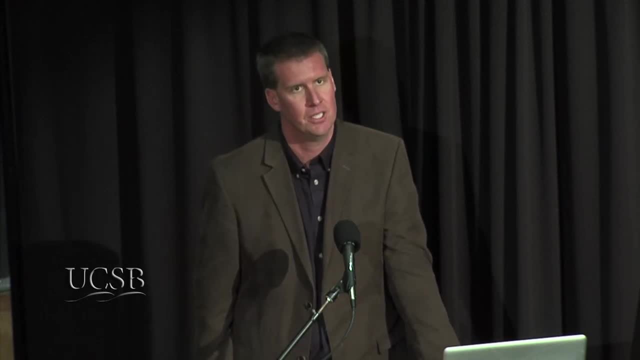 and we have maybe more credibility when it comes to some of this. So we get a lot of questions from the other agencies: How do you guys getting away with doing this, especially back in the Bush administration? And I think it's just something that we have the ability to do. 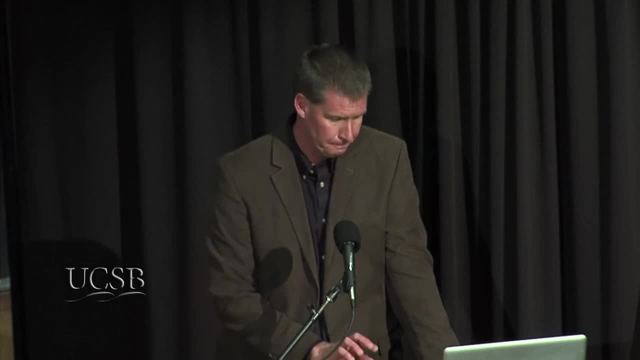 And so I do think that people want- especially the regulators and the managers that we mostly deal with and like floodplain managers and even emergency managers, I mean they want a trusted source. They want to be able to say: we got this data from NOAA. 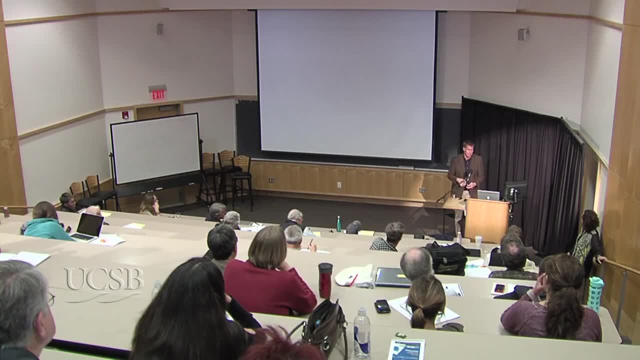 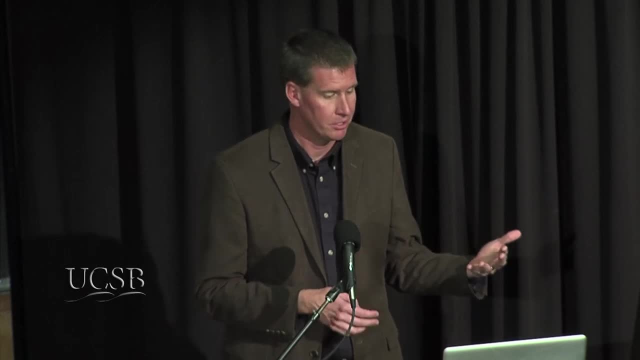 And so, especially like the folks in South Florida I was mentioning, we helped them do the mapping And then they did their analysis. They were able to say in front of their politicals: yeah, this data came from NOAA. They helped us with the methodology. 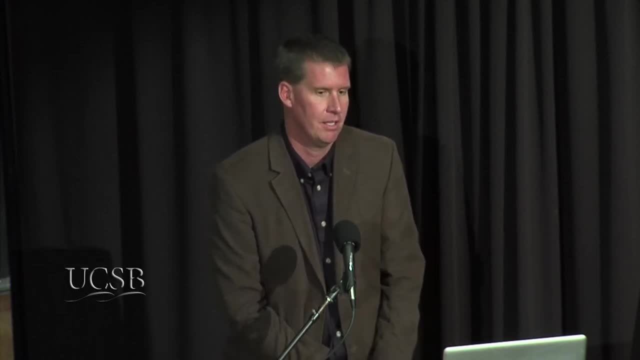 And that gives them a credibility sense that they may not get if they went and said we've got a private sector company to do this for us. So I don't know if that's getting to your question, But I guess if I could just take down some of the 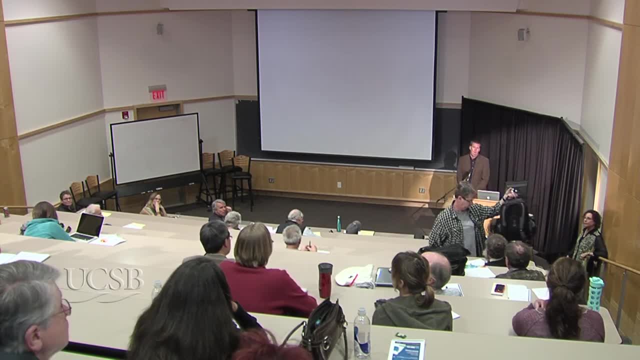 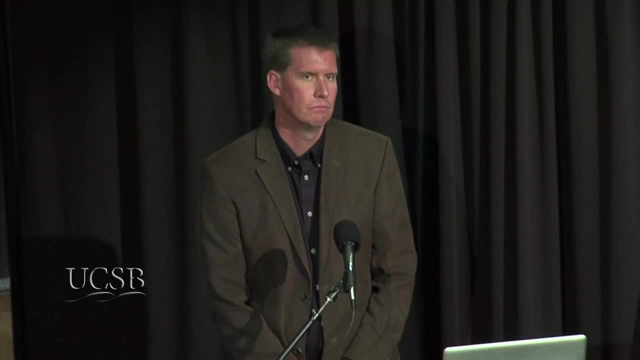 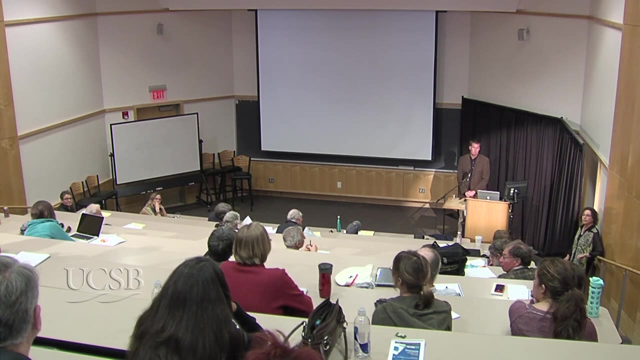 I think this is just a little bit more romantic And I think it's kind of a new conversation And I can't talk about all the facts here, But I think it's a good thing that we have the capacity to do this And I think it's a good thing that we get to just identify. 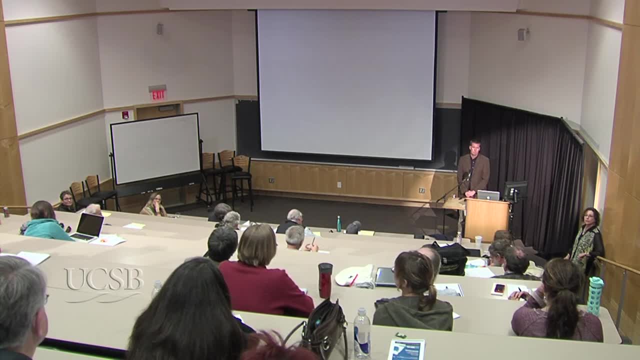 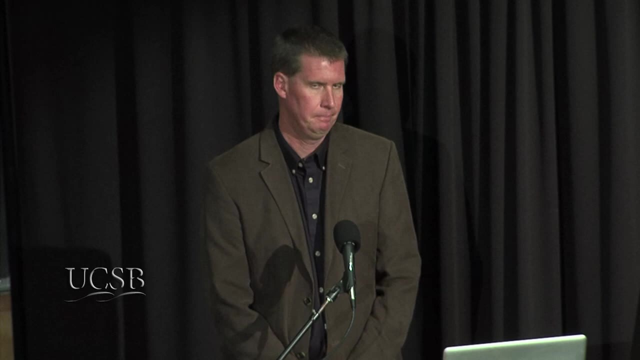 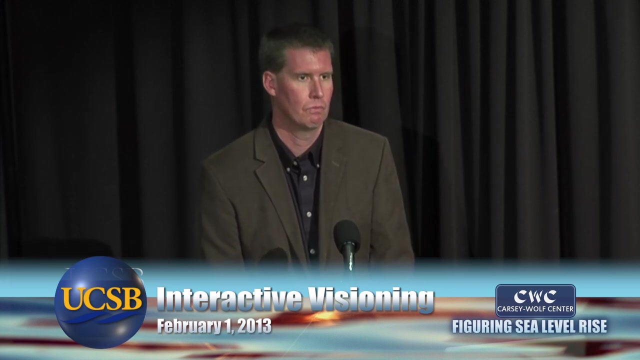 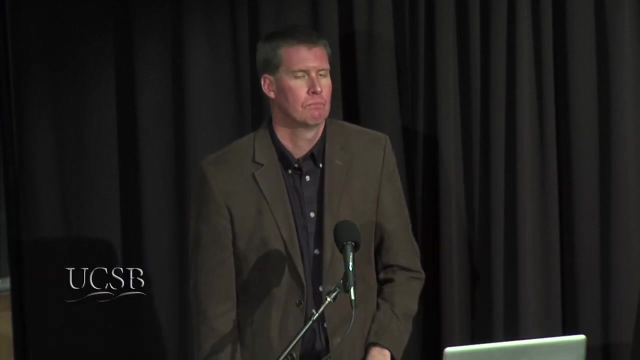 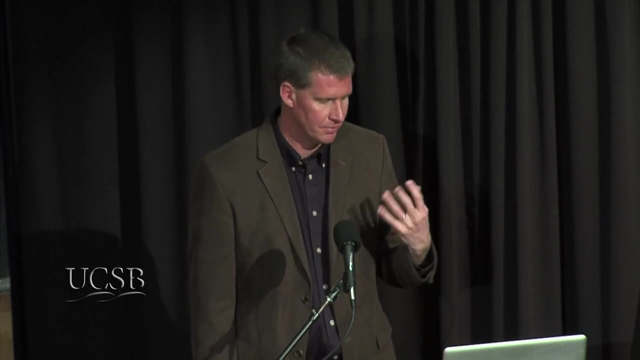 these things and start talking to these folks. Thank you, We'd like to know, Right, yes, there is, and there's a whole outreach component. I didn't go into It's not my specialty, but we have other folks that help facilitate, for instance, communities. 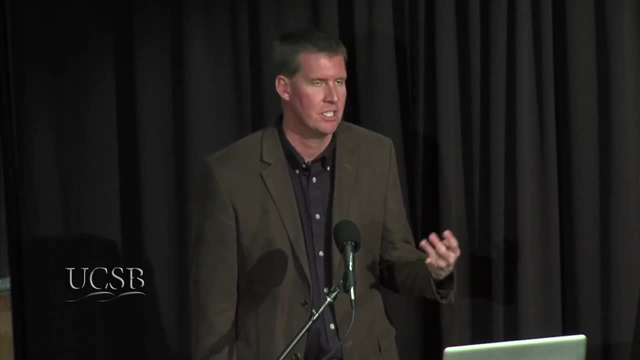 that want to put in. there's a lot of interest. sometimes it's through our Sea Grant program to put together workshops to bring in all the folks together, like this We want to do. start looking at adaptation planning for this particular community. Then we will go and help facilitate. okay, here's all the maps and stuff that you can. 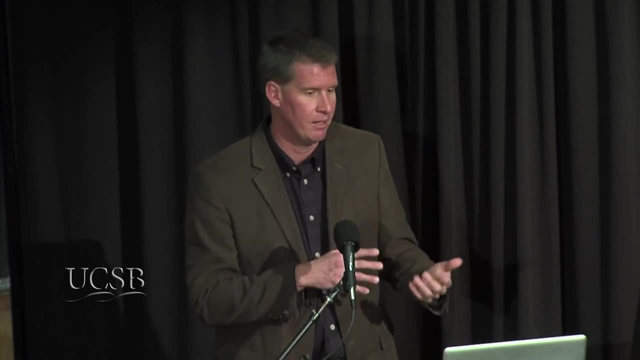 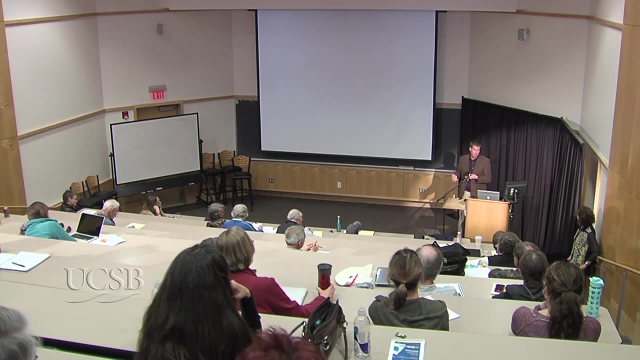 use to figure out where your critical facilities are and get them started in that process, And so we would bring a lot of the tools I showed you here to the table and let them see that, yeah, this can be used to answer your questions. 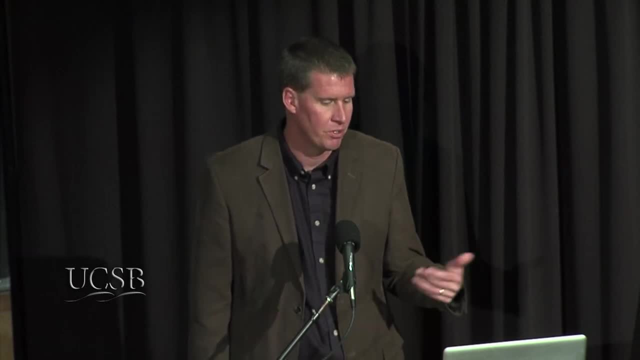 And we have. we have the way we're structured. we have regional offices, so we have folks in just about every district. We have a lot of folks in the city. We have a lot of folks in the city. We have a lot of folks in the city. 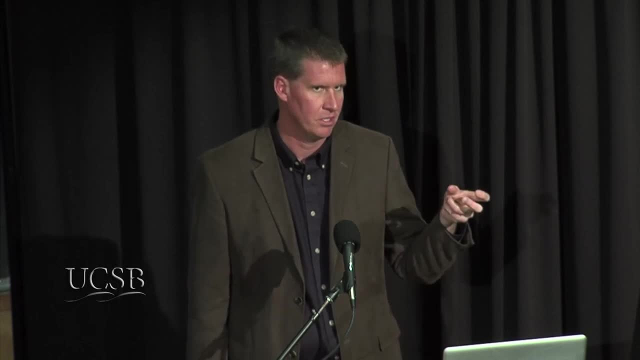 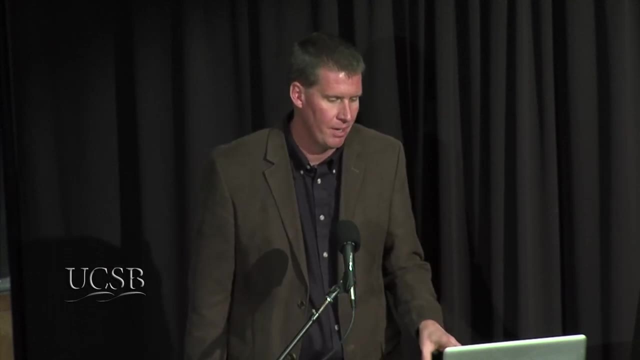 We have a lot of folks in every region that can reach out to local communities, because a lot of times I think the issue is: oh, it's the government. they're up in DC, they don't understand us, So it's trying to. you know again, our audience isn't necessarily the general public, but 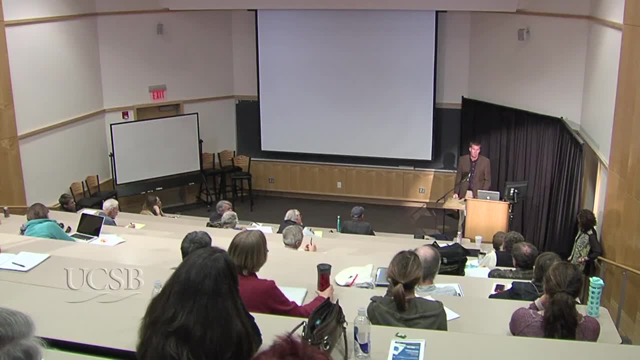 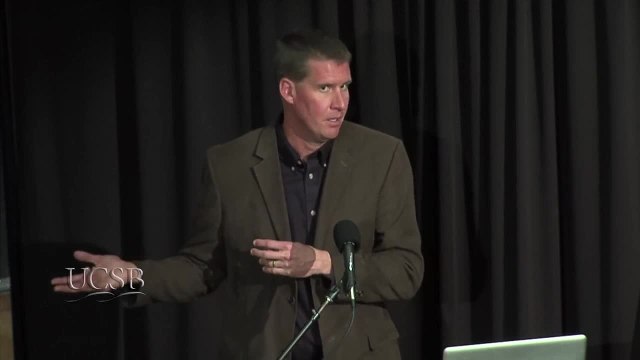 it's the folks that are actually trying to regulate the coast, and so we're trying to get them to use these tools, And also we provide training on the methodologies that we incorporate to do the mapping, in case they want to do it themselves. you know, try to build the capacity. Because, you're right, the agencies don't have the resources. it's tough for us to pull this off for the whole country And you throw a storm like Sandy in and all of a sudden you know it puts you back behind because you're working on something different, and so you know it's a battle of the budgets. 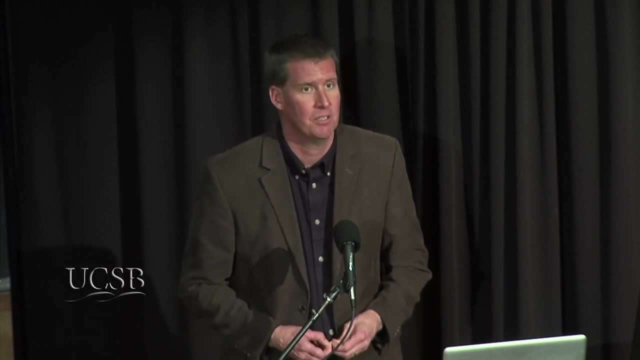 We're still- you know, we're still- looking at really bad budget increases. I had to, I mean just to. our travel has been slashed, so I was lucky to be able to come out here, because our travel's really gotten yeah. 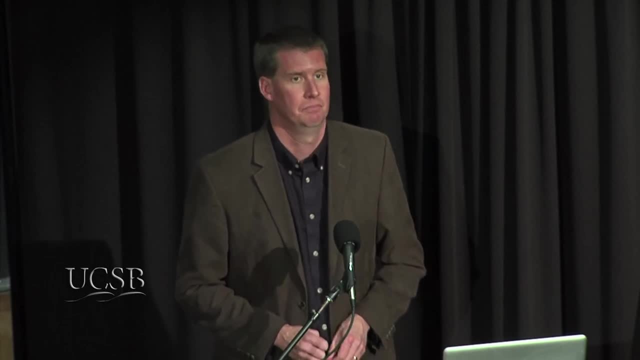 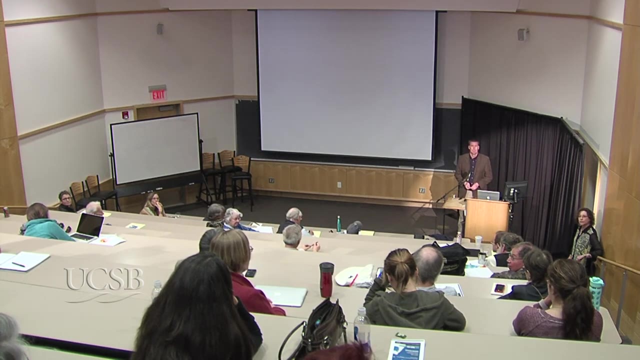 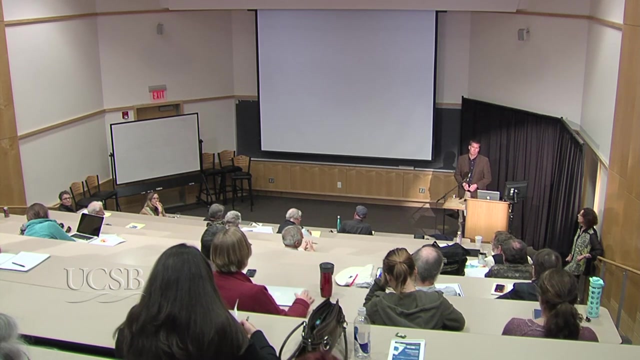 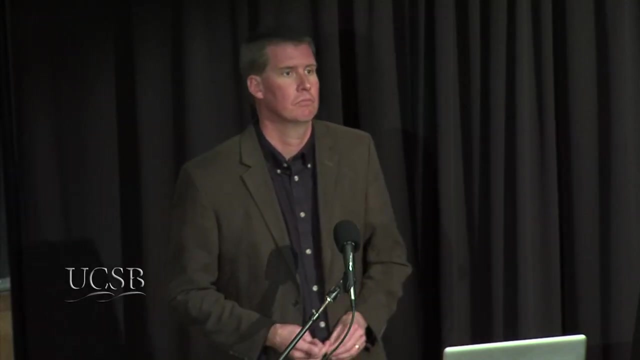 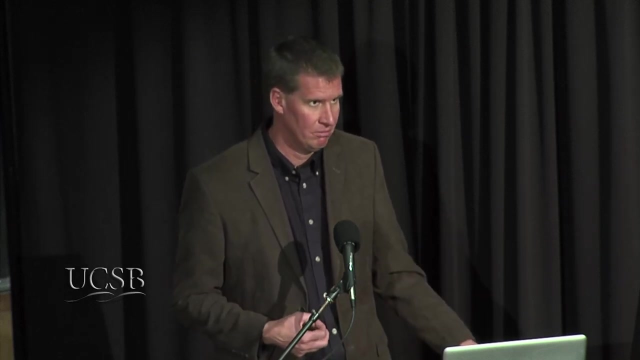 No, you're, you're. no, you're right. Yeah, No, I agree. Yeah, it's. I mean priorities, it's, it's. you know, and especially if you look at the NOAA budget, what we're faced with. satellites and weather take up a lot of space. 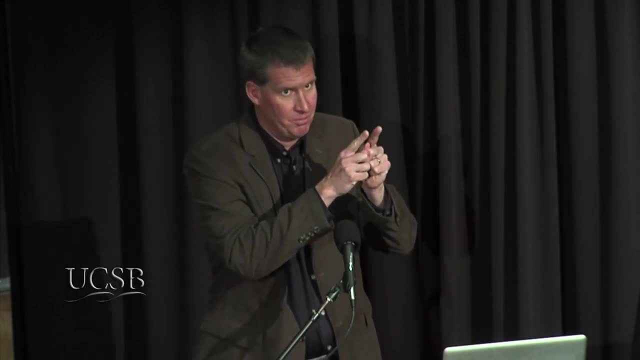 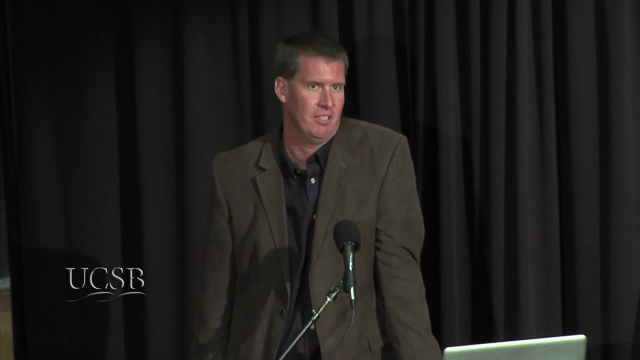 So we've got pretty much our whole budget. then we have, you know this, much left to do the other stuff. So it's, but you can't. what do you do? We don't have satellites, we can't do weather prediction, we can't predict Sandy, to do what? 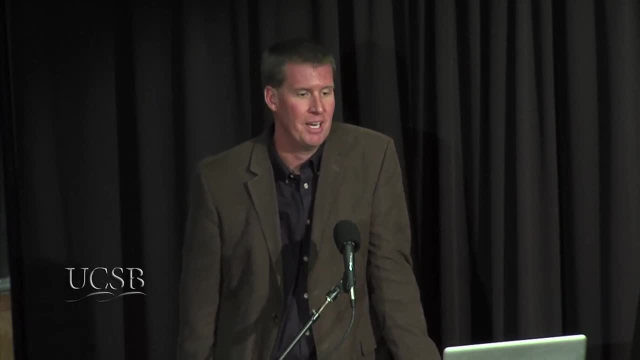 it did. So it's yeah, But I mean there's a lot of. I won't get into the whole budget thing because the cane might come out from you know. I'm wondering if you could talk about some specific cases where communities or state. 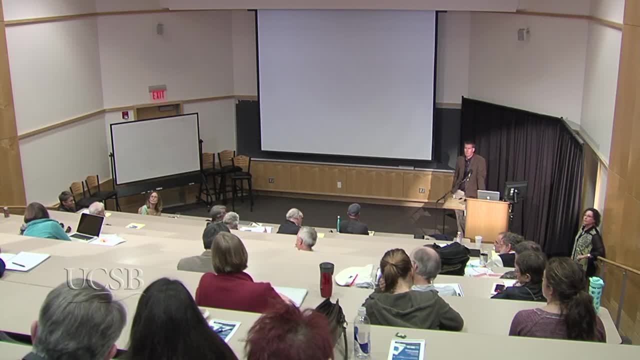 regional level governments have or have come out of the budget. Well, I think it's fairly simple. It's not. you know, we're not in a state where we're not. you know, we're not in a state where we don't have, where we don't have any financial resources. So it's it's it's a challenge, And you know, I think there are some. you know some, you know some. you know there's a lot of there's a lot of you know there's a lot of you know there's a lot of you. know there's a lot of things that you know we don't have, or how they have used that data in terms of planning, long-term planning. And then the second question is: in some ways, it's easiest easy to envision how businesses 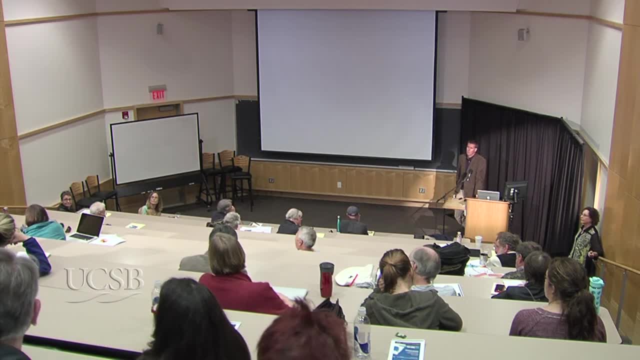 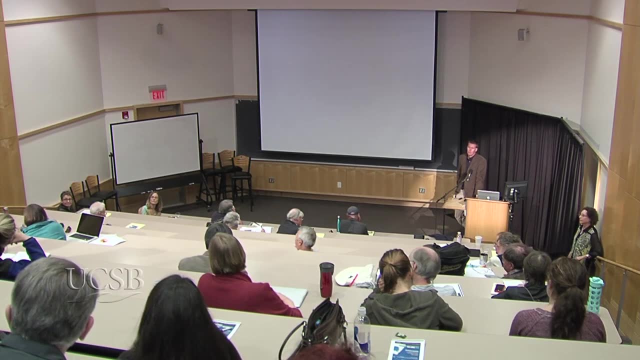 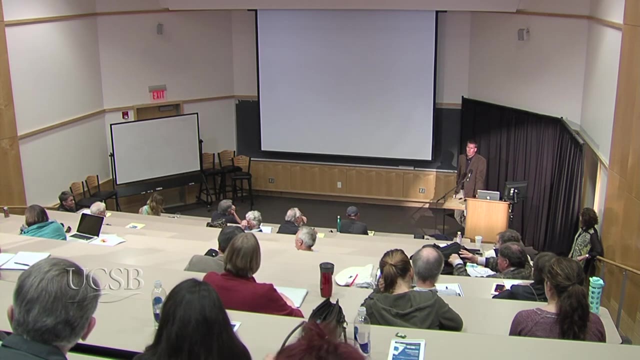 and people with some kind of financial means might use this data to make proactive decisions about the future in a socioeconomic vulnerable place as a community or as an individual, as a family, etc. I think it makes them much more difficult to access the data as well as sort of envision how you might take action for the future, and so I 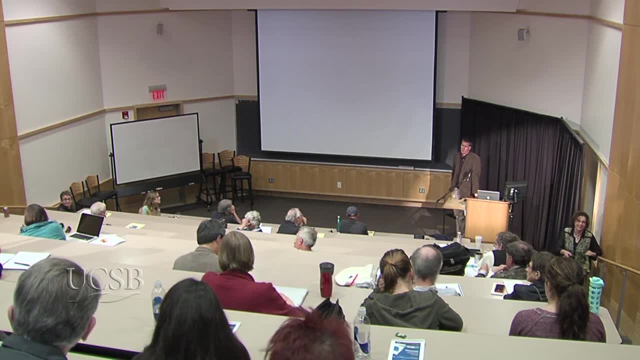 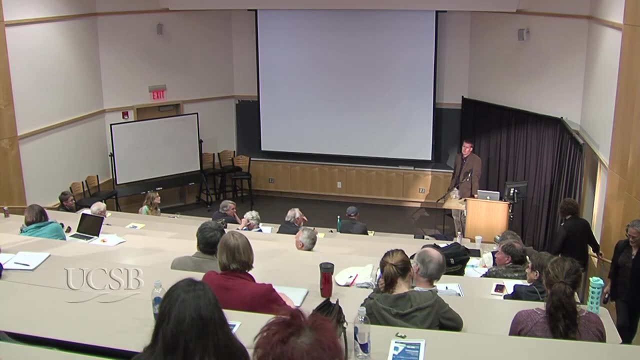 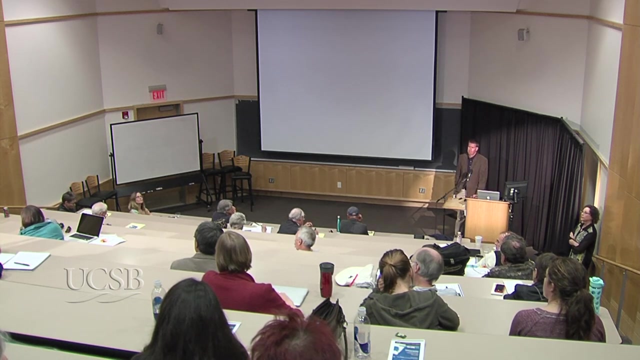 wonder if you could talk about, if any communities are even thinking about budgeting for making some kind of proactive, taking proactive steps in terms of planning for these communities, because clearly we saw the tremendous damage and devastation after Hurricane Katrina and it inevitably you see a kind of alignment between low-lying areas and communities who have, who are 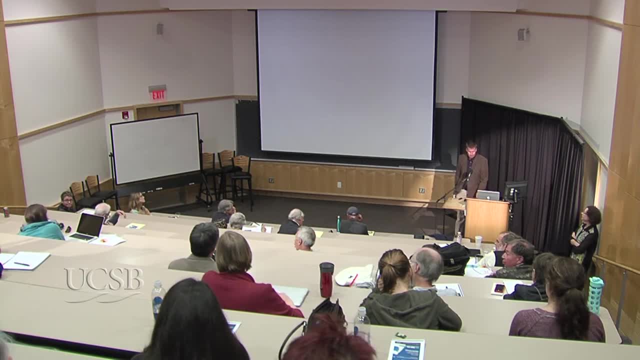 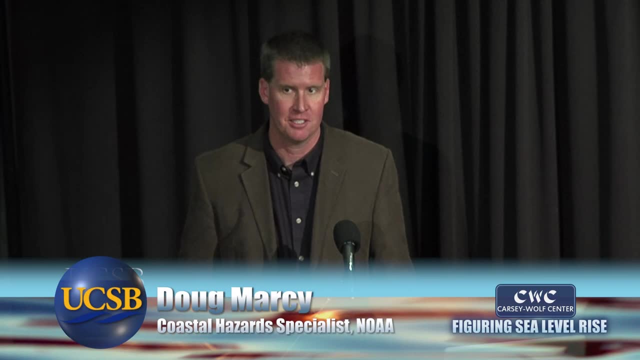 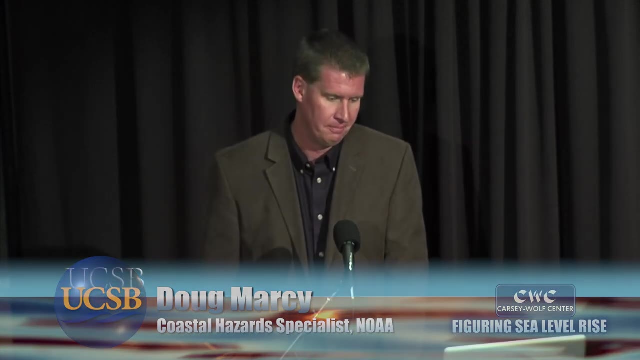 vulnerable in that way, so if you could speak a little bit about that. thank you so much. no, that was. I was gonna actually say that it does seem to be that most of the vulnerable population live in low-lying areas. it's the less desirable property it's, it's not. it's wet more often and and so that that tends to be. 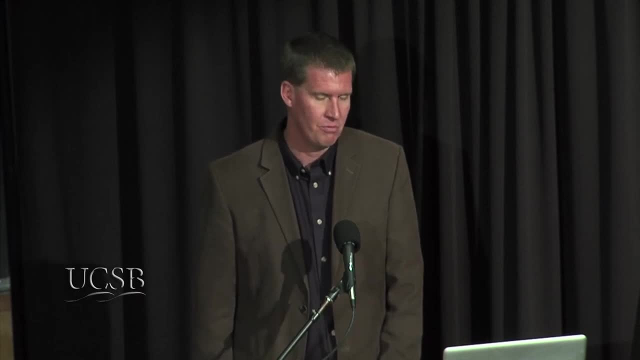 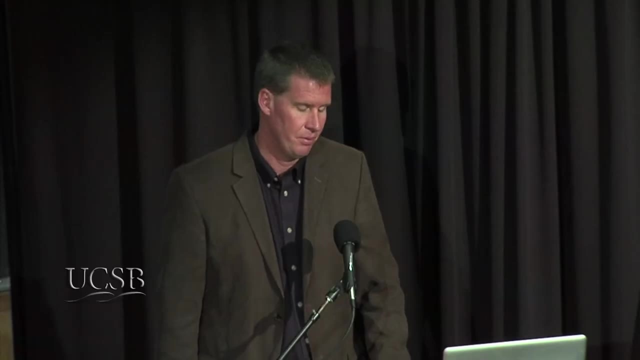 what happens the you. I know that the social vulnerability data, yes, it does get used, and you know the nice thing about that process that University of South Carolina does, is it? it's using all the variables that are in census and so you can get the census. 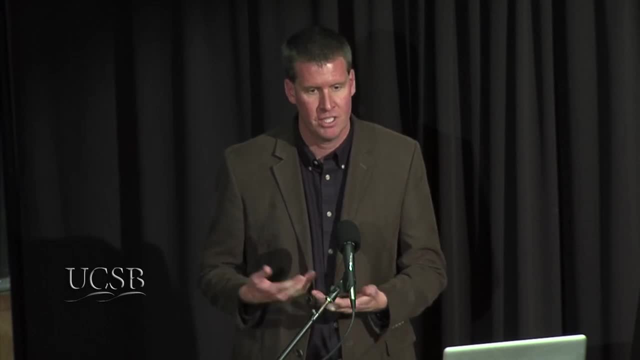 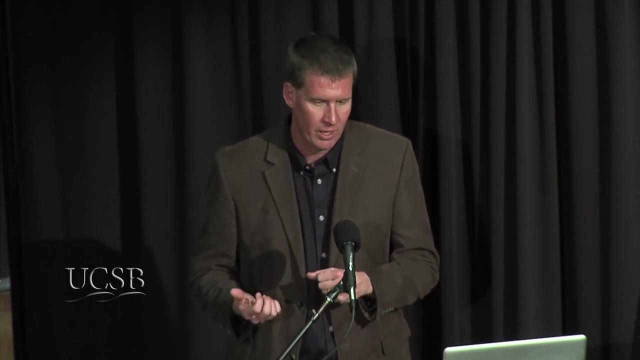 data and do all that yourself, but it it really does kind of give you an index which kind of makes it easier to figure out what's high, medium and low. I know in Delaware, for instance, the coastal program. there they were working on an adaptation plan and wanted that data and actually wanted to go down even finer than a than. 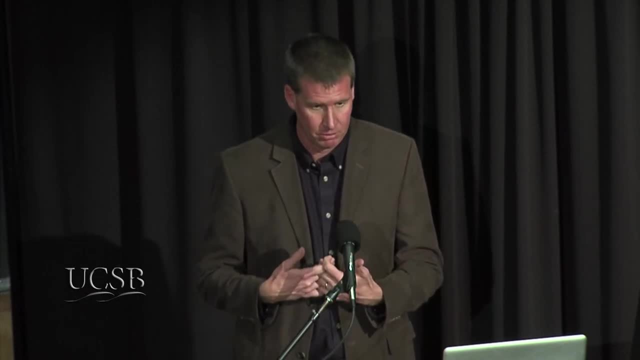 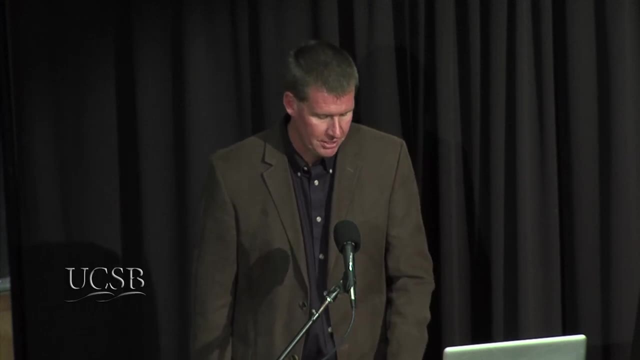 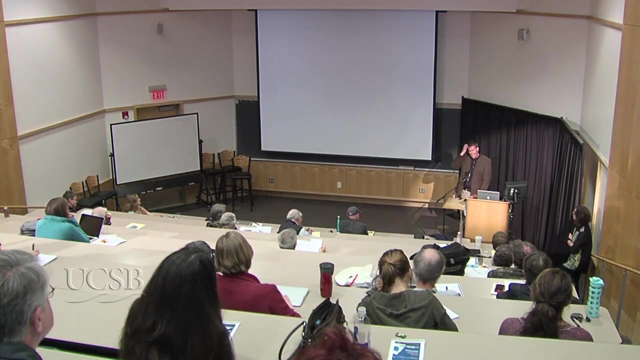 at the block group level, which would be down to the, to the block level which gets even more, you know, specific, to look at the, the population, and there's even interest in trying to do something- some in the GIS world it's called a symmetric mapping, which is to to get it down to even finer resolution than that and try. 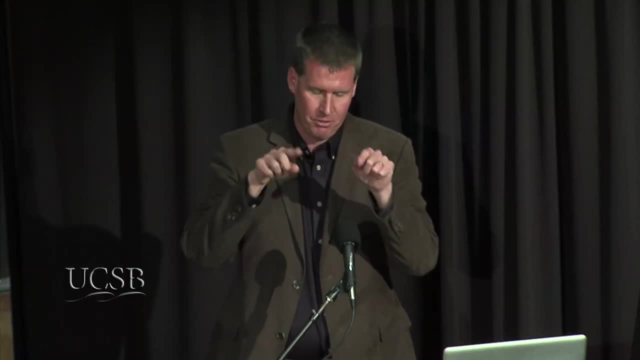 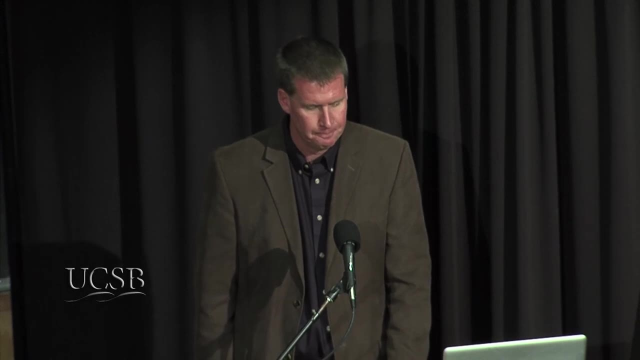 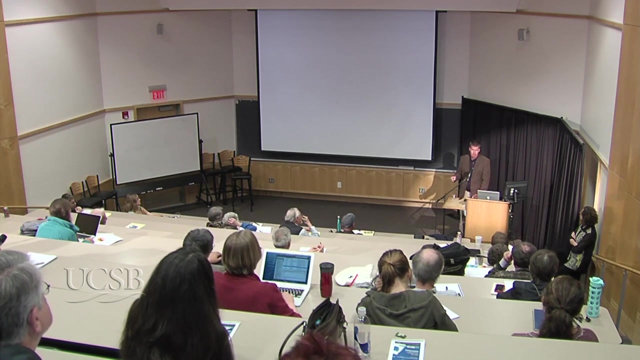 to pick apart where's the people live actually in this block group? so are they in the inundation zone or they are they actually out and there's there's more work to be done on that? but in Florida they definitely- you know some cases- they want to go even to a finer resolution where they'll actually use parcel data. 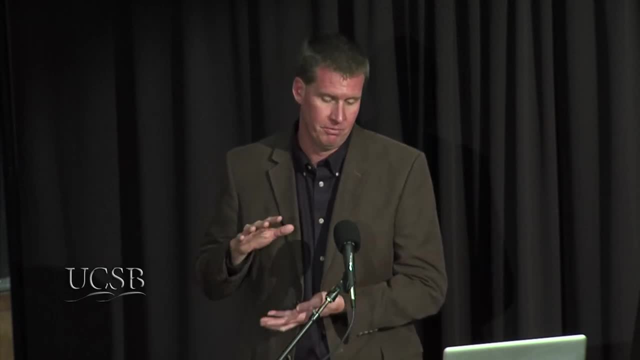 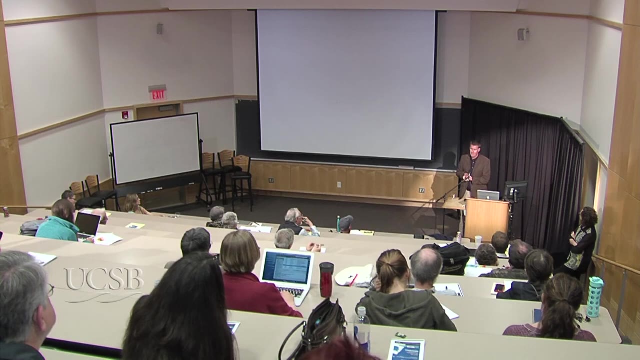 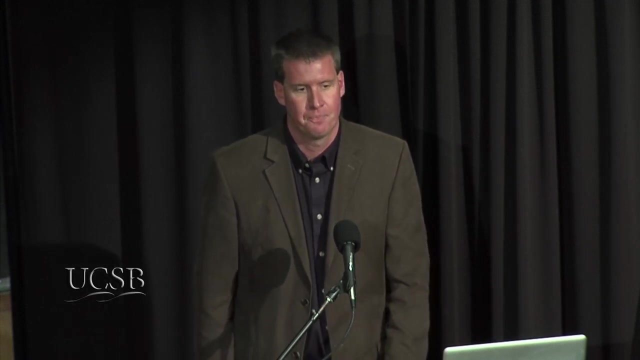 so you won't even use census. they'll go to their actual parcels and figure out the value based on the tax assessors value of that parcel, to come up with dollar figures, and then they can actually get people's names and who owns the property, and then they can, you know, do mail outs and stuff like that. so it's. 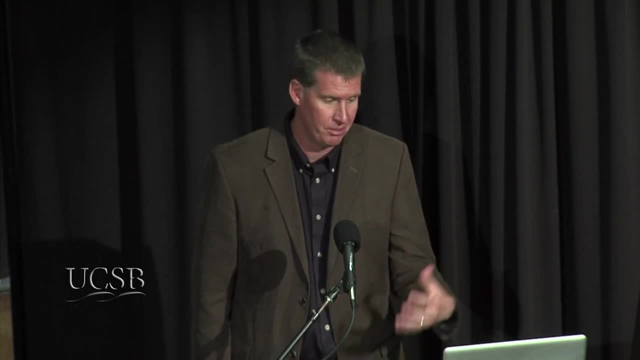 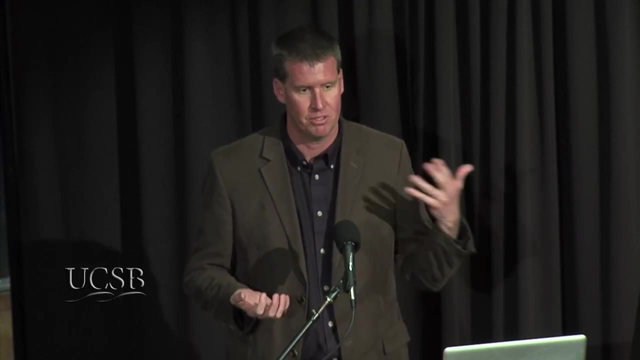 the challenge that at our level is trying to do a national tool like this is it's never going to be good enough, mostly at the local level. right, we can only provide it at a certain screening level and then an additional GIS analysis, whatever has to be done to get there. but I think it's starting to. 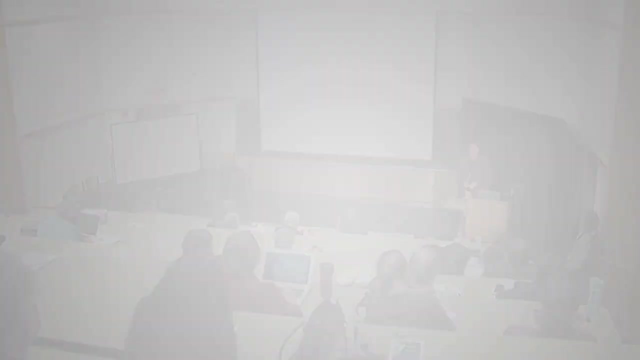 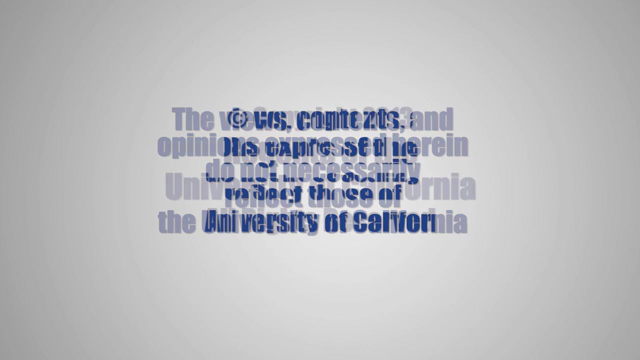 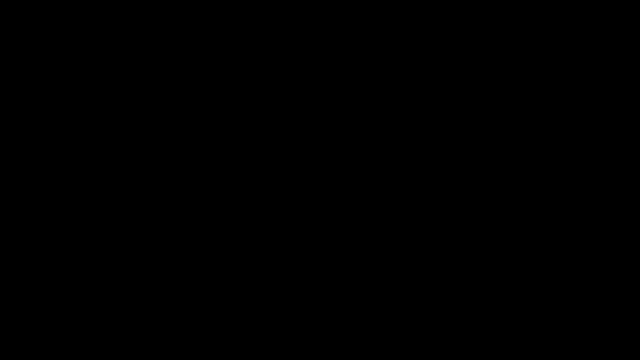 happen. we've seen a lot more capability at that level. you